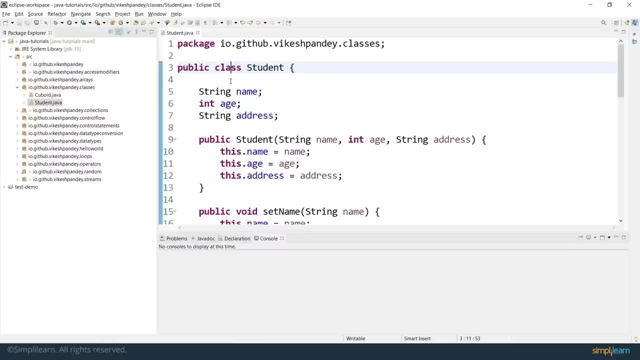 it's always basically some entity. Human beings are an entity, Cars are an entity, Students are an entity, Lecturers are an entity. So who are all the actors? all the actors which you see in the world are basically entities, and you can map them as classes in the Java program. Now, why do you? 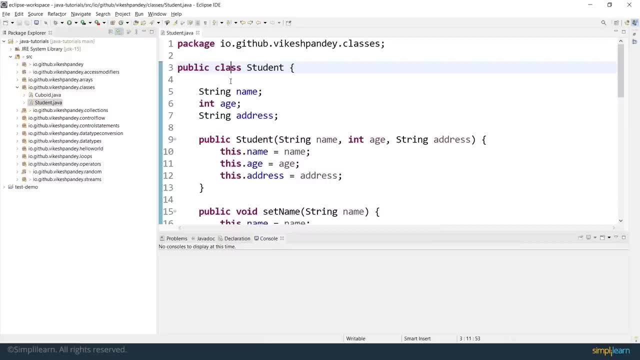 want to map them, Because these entities have basically two kind of specifications. One is, every one has some attributes and it will have some behavior, and actually that is how you identify an entity. For example, human beings have attributes like we have hands, we have eyes, we have ears. 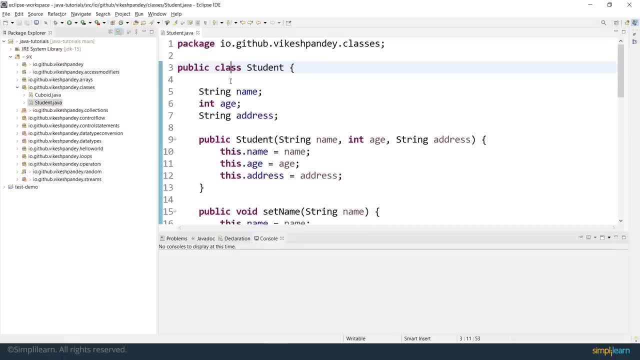 legs, et cetera. These are our attributes. Then we have our behaviors. Behaviors are actions. You can think of them as a human being can speak. So can speak is an action, It's a behavior. Can listen is an action, It's a behavior. Can walk is an action, It's a behavior. Similarly, can 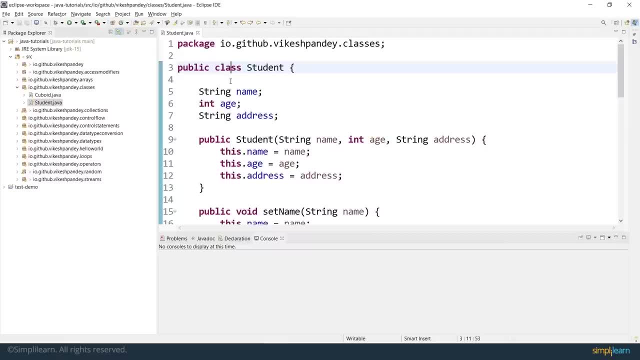 Eat is also an action or a behavior. So that's how you basically represent an entity. That's how basically you identify an entity, That an entity will have some attributes and some behavior. If you see those two specifications in any entity, you can map that entity or you can write that entity inside a Java program as a class. 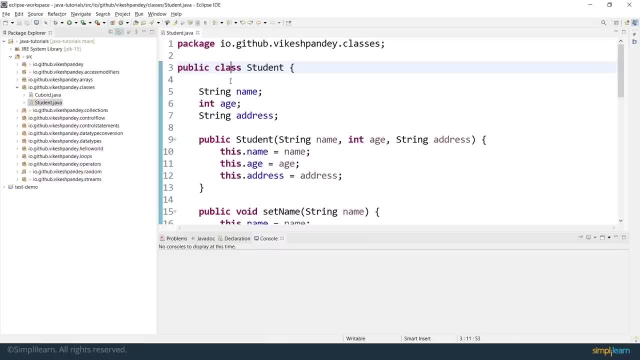 Because a class in Java will exactly have these two properties. It will have some attributes which we call as properties and it will have some behaviors which technically are called as methods. So it will have attributes and it will have properties and methods similar to real world entity, where we have attributes and behavior. 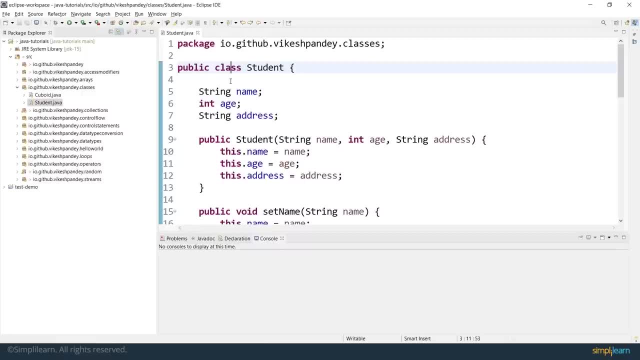 Behavior are methods and attributes are properties. That's how it is So if you, if you apply this simple philosophy, whenever you are taking requirements from a customer for a particular project, always try to identify these entities, These actors, in your program. once you have identified those, you will be able to write a corresponding Java class in the Java program which can represent those entities without representation of those entities. 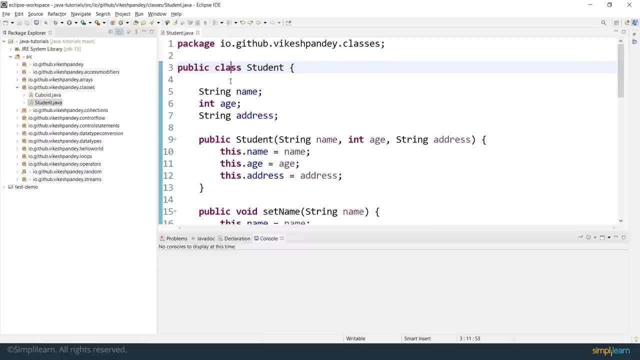 You cannot write the program, So Java will kind of force you to think in this direction, to find entities which will have attributes and behaviors. So, taking that philosophy further and taking that example further, here for you I have prepared an example where I am creating: 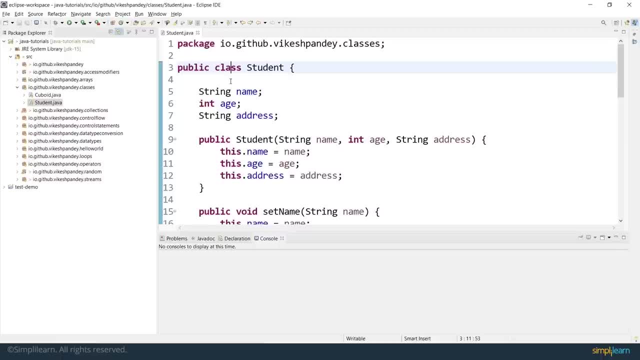 A student class. So basically, let's say, if you have to build a college management system or a student management system, then student is probably one of the main entities which will be talked about when you take the requirements. So if you think about the attributes and the behavior concept, a student will have a name, will have an age, will have an address. 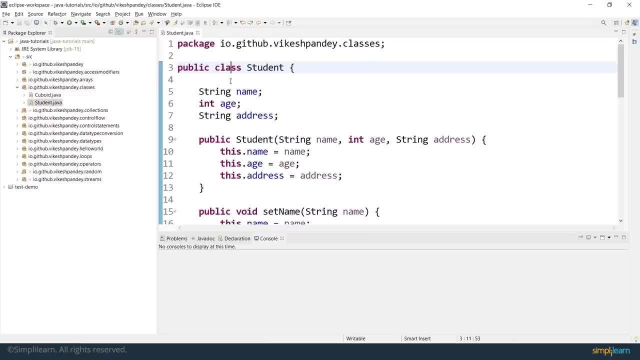 And, at the same time, a student can also have some behaviors, like can enroll in a particular course, Can Attend a lecture, can take a leave, can take exam, et cetera. These are all behaviors. Let's understand this in a more detail with the help of this example, where I've created a class which is named a student. 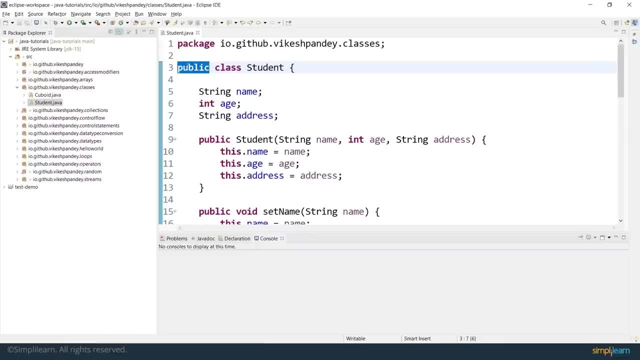 And you see the public keyword. here Again, I will cover access modifier. public is basically an access modifier and I will cover this in very detail in the upcoming sessions. For now, let's focus on this part. So we have created a class to represent our entity. 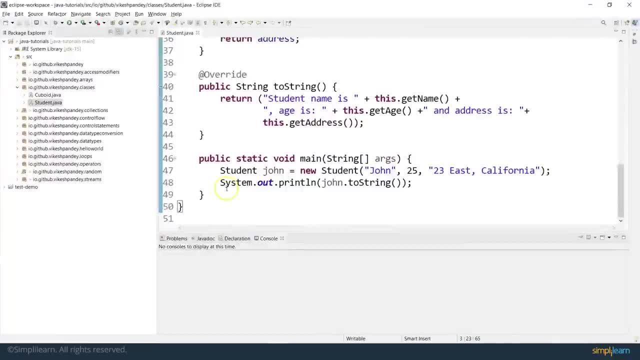 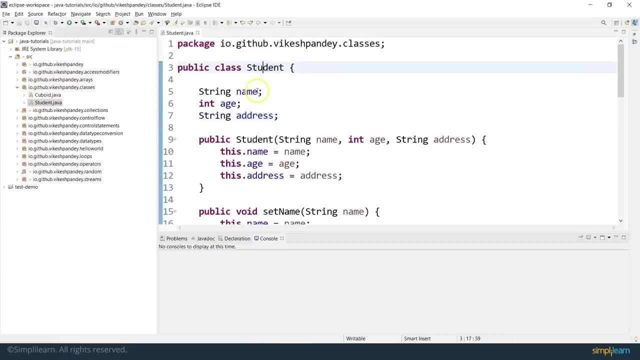 You put a curly braces around it. It ends here, And after that you provide the attributes. So here I'm saying that a student will have a name, It will have an age and it will have an address. It has three properties. 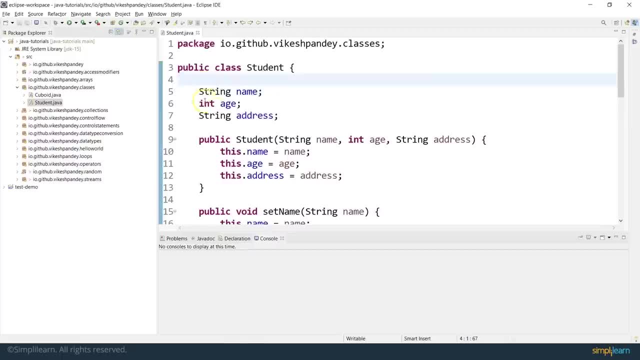 So the technical name of attributes is properties. After that, let's skip this part, and I will come back to this part. Once you have declared these properties, you would want to provide a way for the name to be filled or replaced or received. 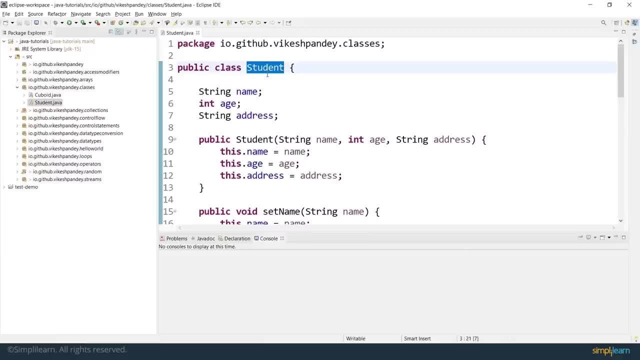 For example, If you have created a student class, how do you insert the name inside the student class, But how do you insert the age or how do you insert the address or modify the age, name or address properties? for that We have these setters and getters methods. 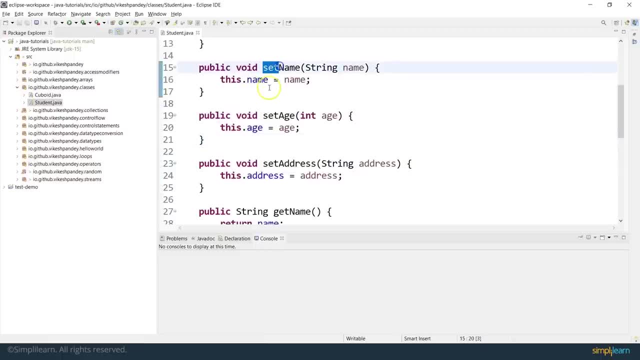 We call them setters and getters because they start with this keyword, not keyword, but they start with a string called set. It is not a keyword. You can actually write it as anything. You can call it as modify name, That will also be absolutely fine. 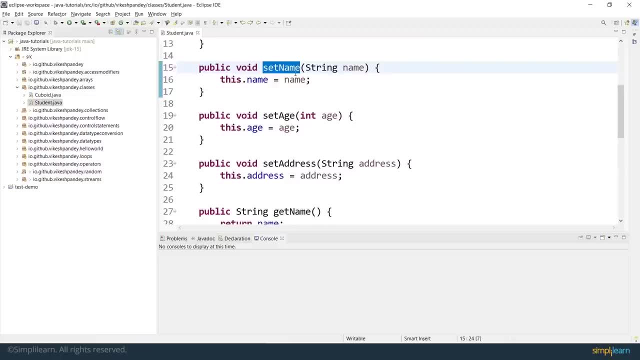 Java will not give you an error, But the standard naming convention given by Java is to start the methods as starting with set and get. This is the standard naming convention And, like I said, it's a naming convention, It's not a compulsion. 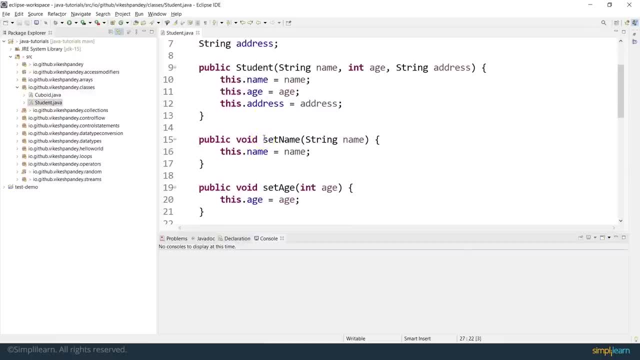 But if you write this way, your core developers and the people who are going to maintain this project in the longer run will be very happy. Otherwise, they will be very angry if you use strange methods Because, like I said, this is the standard naming convention. 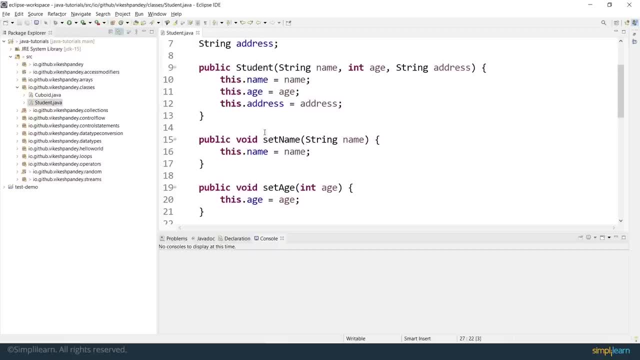 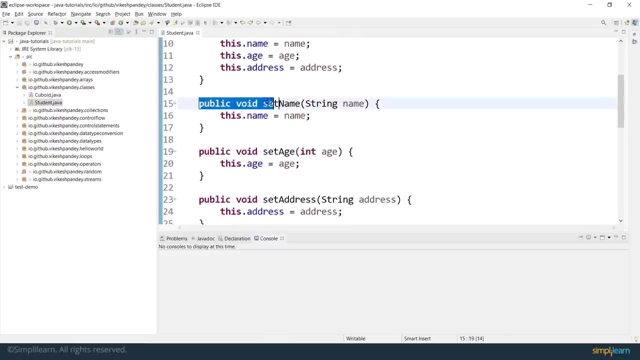 So now you are going to write a setter method for each of the properties in this particular class for name, age and address. So we call set name. Again, you put public void because this is not supposed to return anything. This is just supposed to set the value of name with whatever value you specified. 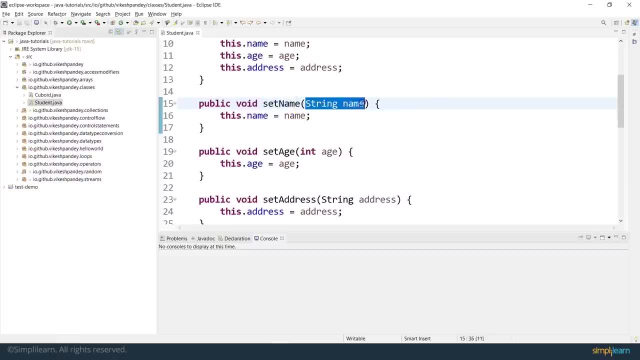 Then you call set name And then you provide the value which you are supposed to set against the name. So whatever value, Like any random name, John or Jane, whatever- You need to supply that name here while you call this method And that name, whatever name you supply, will be set against the name property of this particular class. 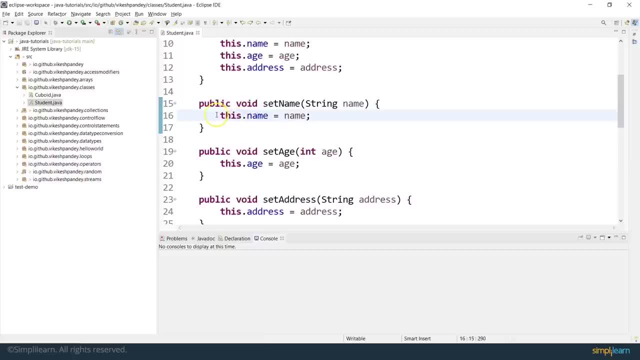 And remember, I use the word this here intentionally, because the way you are going to represent this is with the help of this keyword. This keyword means current object, It means that you are. when you use this dot name, It is referring to the current object. 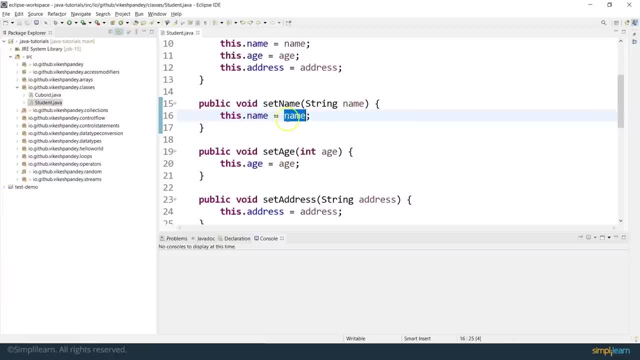 Current objects, name property, And this name is basically corresponding to the name which is coming in when somebody is trying to set a name. Similarly, for set age, age is a numeric number, If you, if you observed, it's basically an integer. 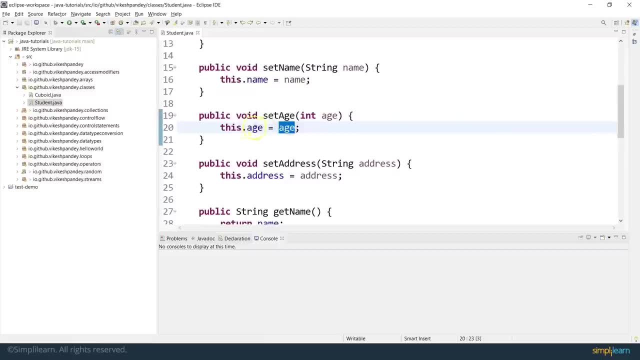 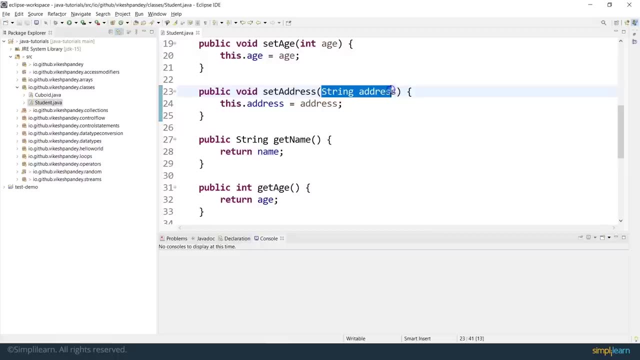 Then I'm saying int age, and whatever value of age will be coming will be set in this particular object's age. Then, similarly, for set address, we have a string address argument being passed into into this method And this gets set inside the current objects. 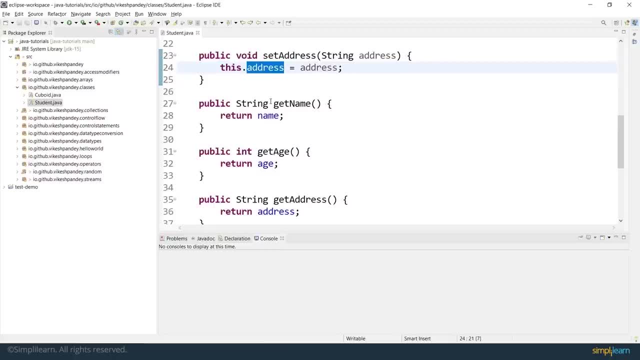 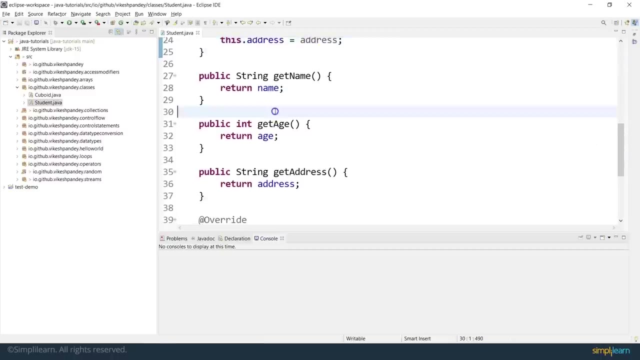 And this is the same thing for the set address property. So I've provided a way for the external world to set the values of name, age and address, because for each student you would need to set these values. Now you also need to provide a way to receive the values or to return the values or to read the values for reading operation. 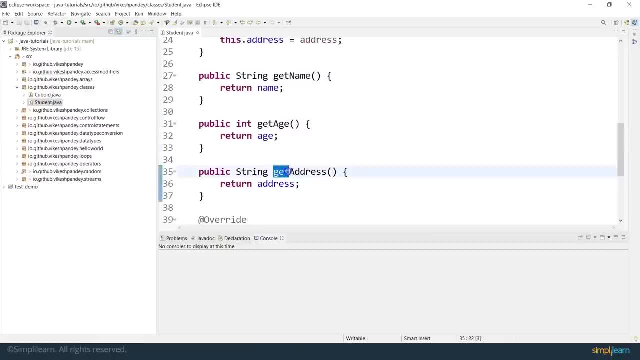 You need to provide the getter method. So you see this: get again. This is not a keyword, It's a standard naming convention, So similar when you, when you wrote set name, Similarly you will write a get name. This method is supposed to be reading the current objects names, properties, value and will return that value, since name is a string. 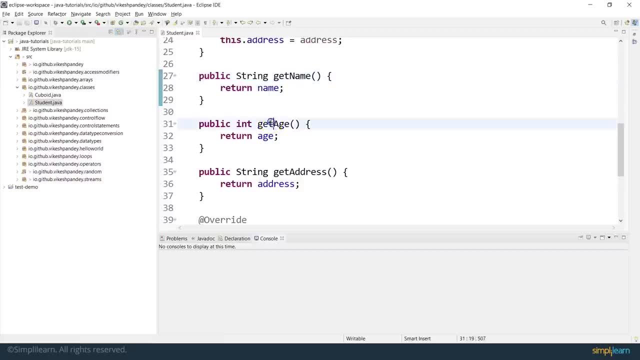 That's why you see the return type as string here. Similarly, get age is going to return the age, which is an integer, and address is going to return the address. You can also write it like this, which is absolutely fine: It is not going to complain because technically it is returning the current objects: name properties and age property and the address property. 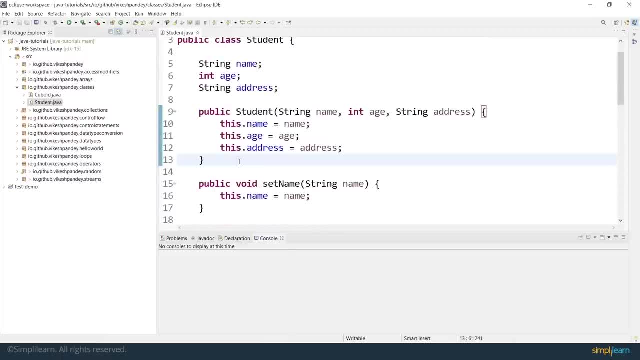 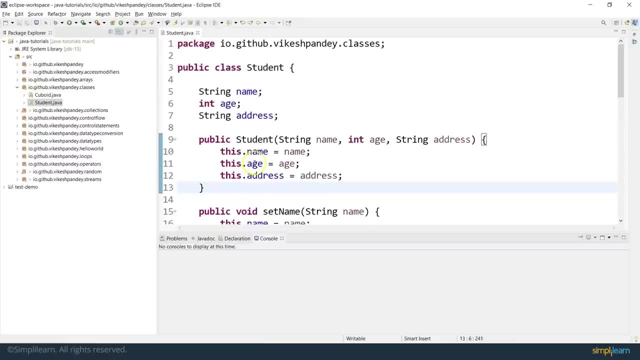 Now let's talk about this. What is, what is this section? So this section is basically called a constructor, and I have a whole session dedicated on the constructors. But let's understand why we need this. Remember, when I told you the definition of the class, I said that class is a blueprint of an object. 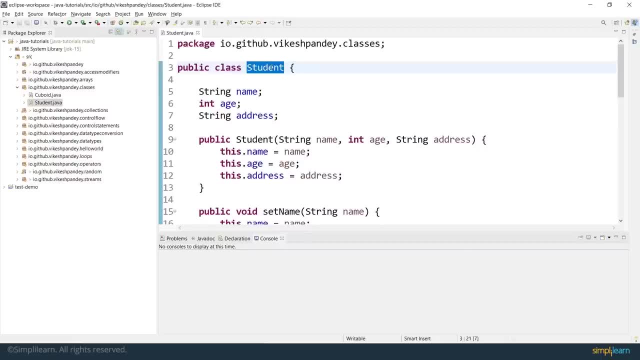 So you have created a student class and you have 5000 students in your college. Now you need to create a new student object for each of those students. You need to initialize The student class 5000 times. How do you do that? 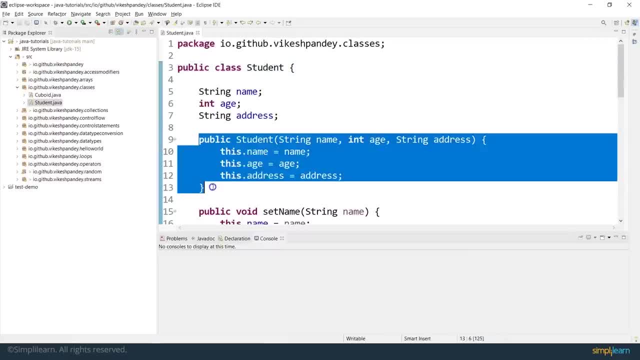 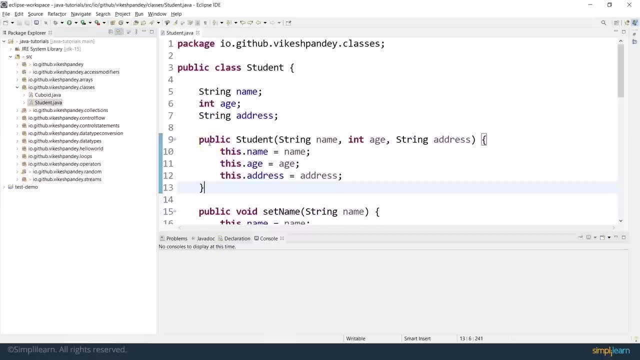 To do that. we do that with the help of constructors. We call this constructor. This is a special type of method- Remember this is a special type of method which is provided by Java to initialize any classes objects. If you want to create multiple objects of the student class, you can repeatedly call this student constructor. 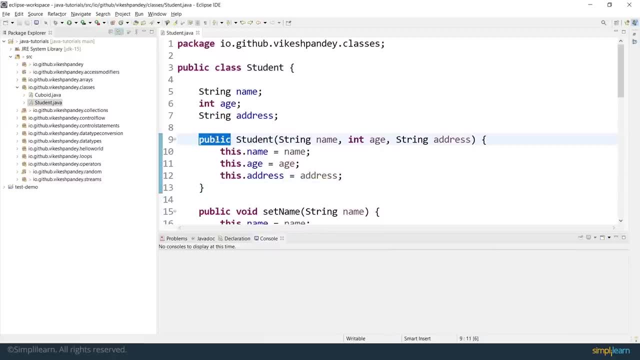 We call this constructor. So you put public here, because we want this constructor to be accessible to the outside world. Then you put the exact class name. So whatever class name you have provided here, you need to put the exact class name here. If you don't do that, Java is going to raise an error. 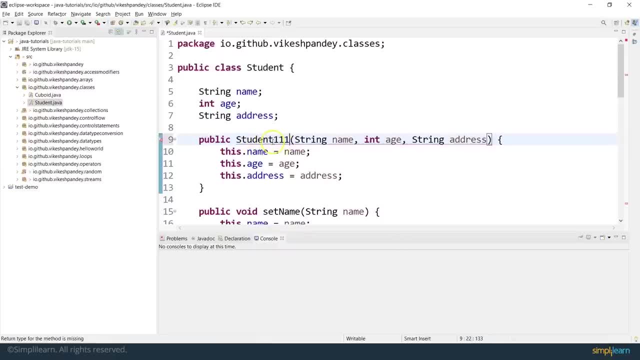 If I do this here, it is going to you see a red line here because Java failed to compile this constructor. It does not understand what a student triple one, but it does understand what a student. So this is how it is going to be. 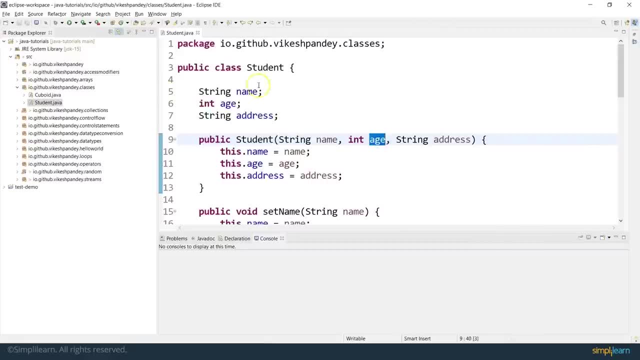 And then you provide all the properties which are going to create the student object. So you're going to create the name, The age and the address, So the name, age and address, And then you set those values, again similar to the setter methods we have seen. 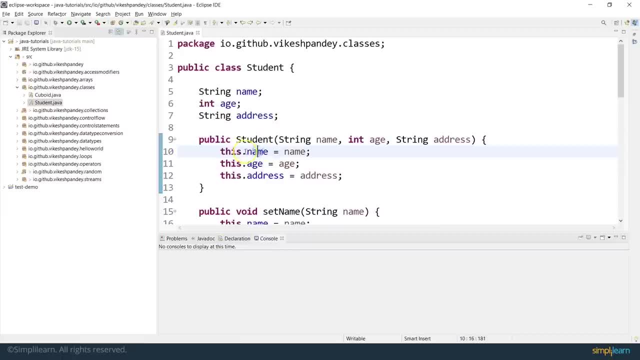 The reason we need to use this here? because if you write it like this, then Java doesn't understand the difference between the current object's name and the name coming from the argument, So to differentiate that you need to use this here. If you use n here and if I just use n here, then this is fine, because there's only single name variation. 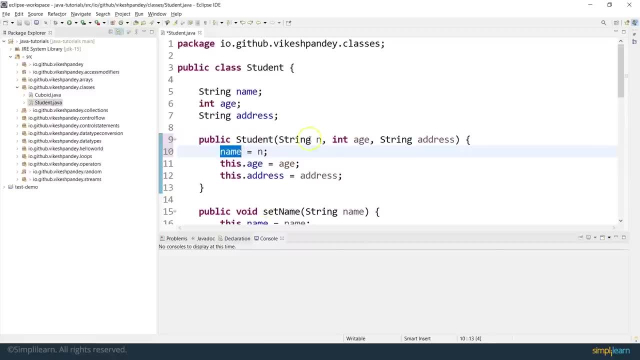 So if you use n here and if I just use n here, then this is fine, because there's only single name variation. So if you use n here and if I just use n here, then this is fine, because there's only single name variation. 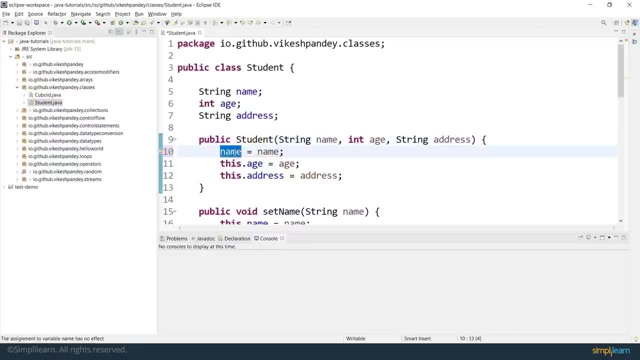 And then Java doesn't know if this name is basically the student class' name. And if I write it like this, then Java doesn't know if this name is basically the student class' name. And if I write it like this, then Java doesn't know if this name is basically the student class' name. 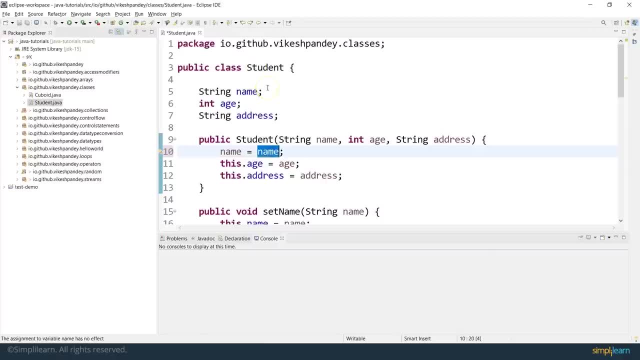 Or this name is the student class' name, It will get confused. it'll get confused like you're getting confused, If you try to just find this in a Mind Mapping. So that's why we need to write this here, so that it's clearly differentiable. 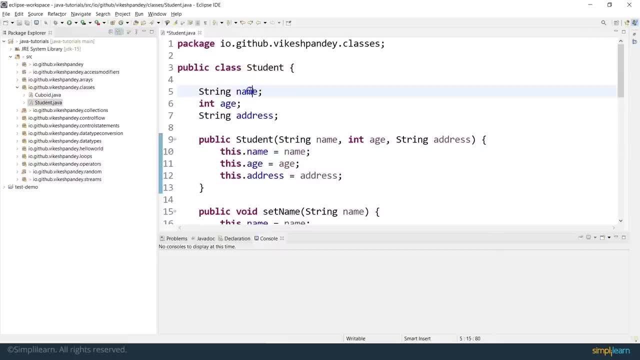 that whenever I use this dot name, I'm referring to the classes name property And when I'm just using the name, I'm referring to the method arguments. So, for example, let me write Bear fyba in the parameter Take. that's what we do in doing this in this constructor, so you basically initialize. 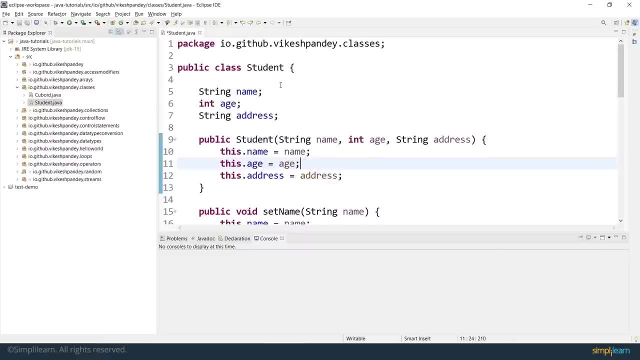 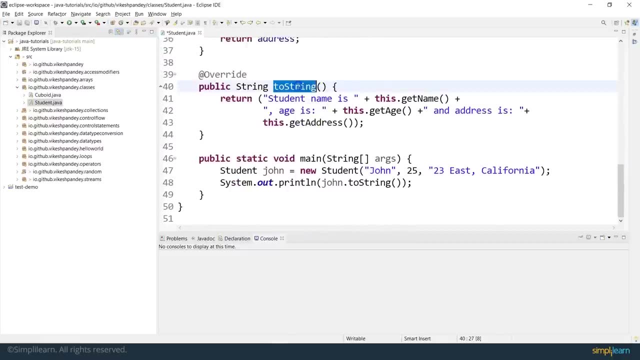 all the properties of your class, with some values, with the help of constructor. so we have the constructor, we have the setter, we have the getter. we can cover about this two string. basically, this two string is to print, print something. but we can cover that later. now let's initialize this. 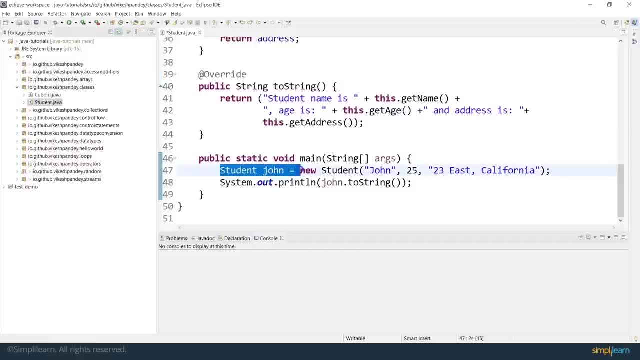 particular class. so i'm similar to the initialization we have seen so far. you just write student, you write the object name- this can be anything- and then you use the new keyword, which is used to initialize anything in java. new is a keyword in java which you can use to initialize. 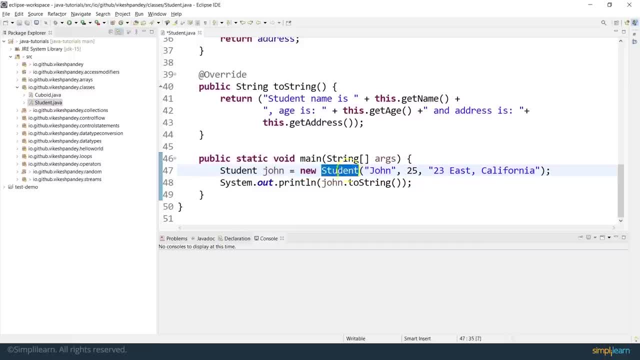 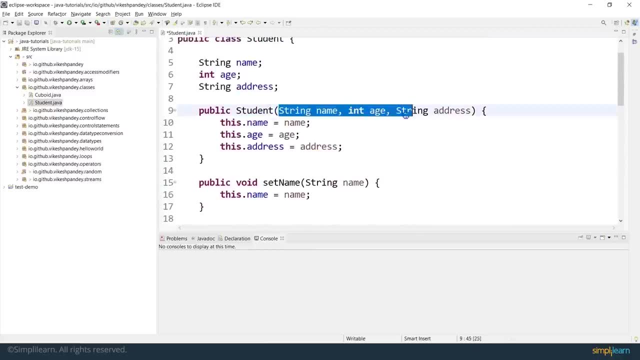 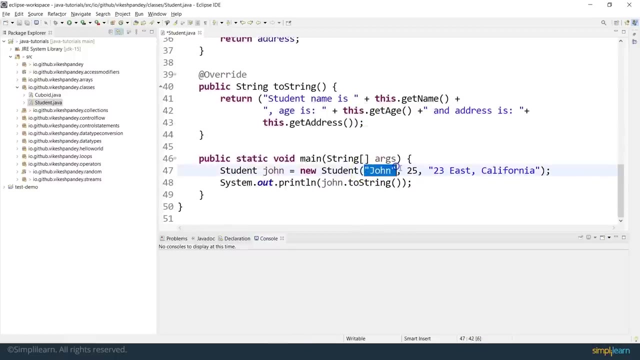 literally anything in java. so you use new student and when you say new student, you can provide all the values which should match its constructor. so here we have three values: string, integer and string- and here also we are supplying three values: string, integer and new string again. so remember to match this exactly with one of the constructors which is available. 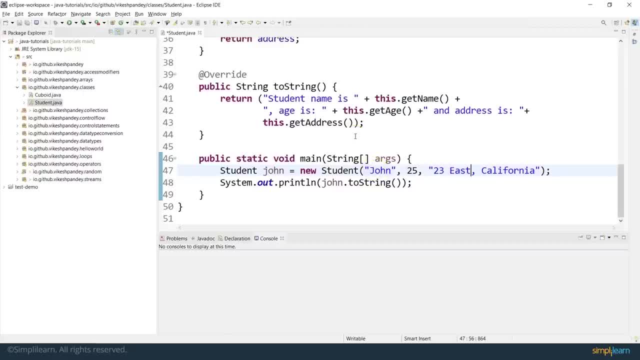 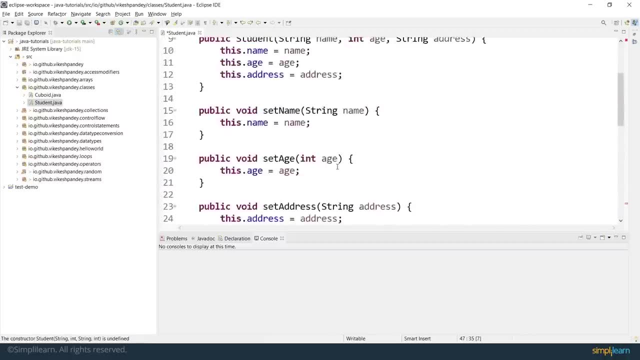 in the class. if it doesn't match, it is going to fail. it will not work. so if i, for example, if i do this, then i'm supplying four arguments to the student class, but there is no constructor matching for argument, so it is going to complain. you see this red line and the code is not compiling. 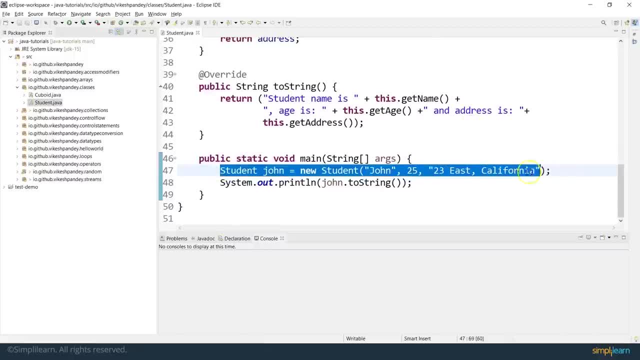 if i remove this, then it is matching it and that's how you basically create a student object. so an object is basically an instance of the class. remember that very well. an object is an instance of the class. once you have created an instance of the class, then you can call any. 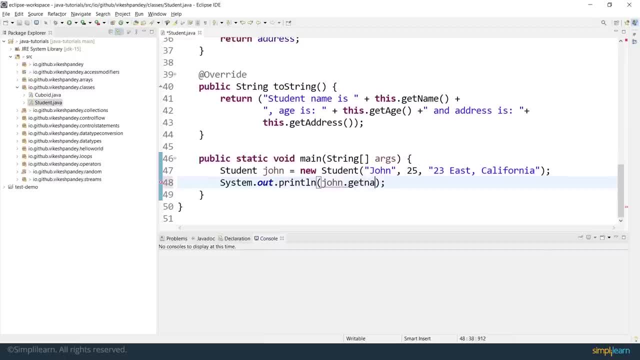 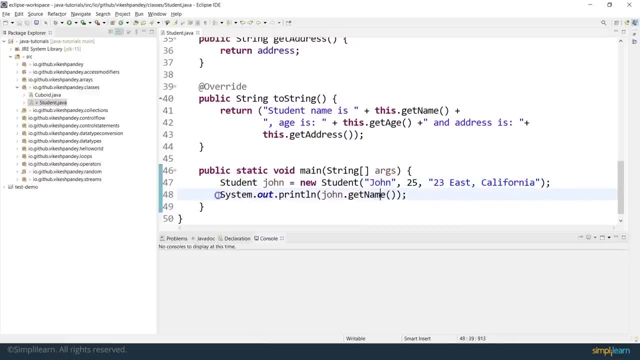 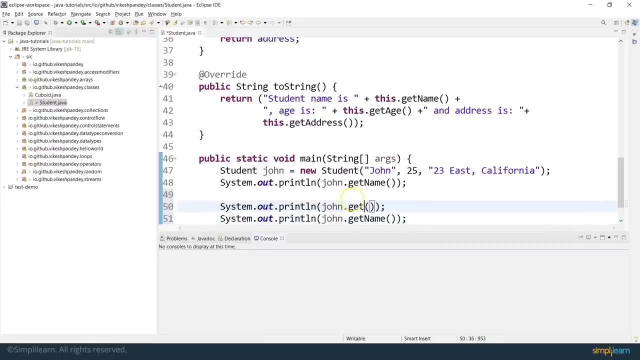 method like say, let's say you want to read the name, so you can call get name, you can read the name similarly if you want to. so if you, if you want to read the age of the student, then you can do that as well. so let me just copy this and do this: let's call get age, i want to print the name. 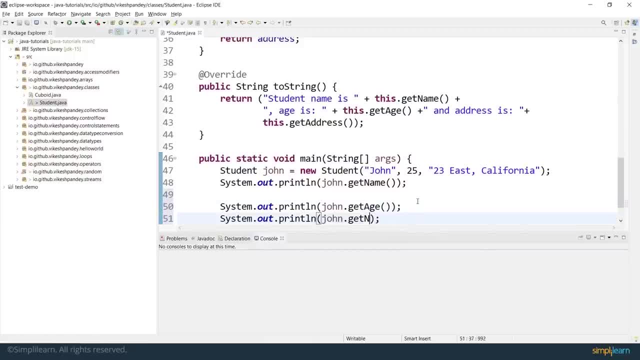 i want to print the age and i also want to print the address. so get control space. i get suggestion address. yep, so i'm printing the name, i'm printing the age and i'm printing the address after i have initialized the object successfully by using this constructor representation, using the new keyword. 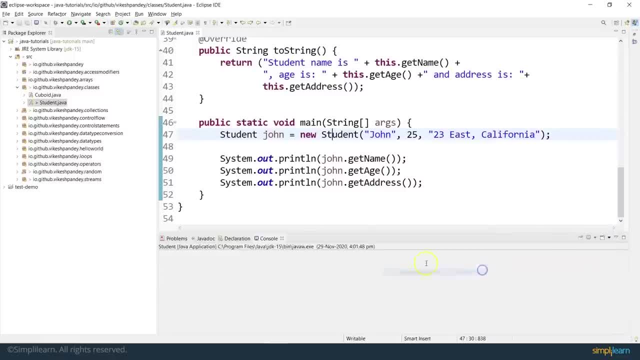 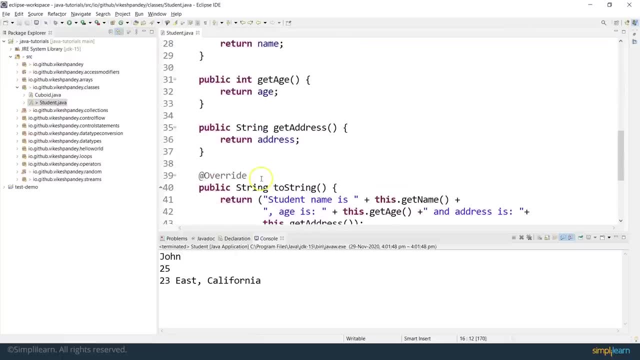 so now let's run this method or run this class, basically okay. so when i run this class, the whole class got compiled: the constructor, the getters and the setters and the properties and their types, everything was set. then the main got called and i created a new object from this. 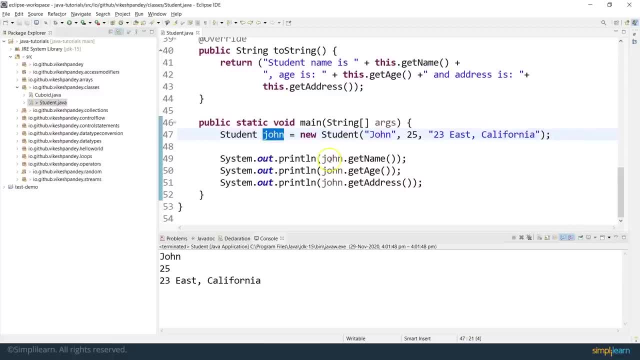 class's blueprint. the object name was john. then i called johnget name to print the name which is stored inside this particular instance of the student class, similarly the age of age which is stored in this particular instance. so we stored the name as john. so when we call johnget name, 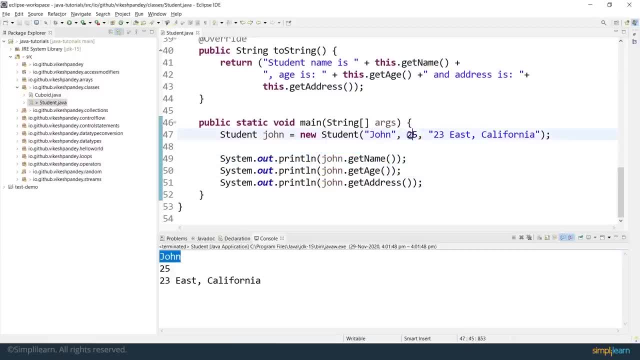 we get john we got. when we call johnget age, we get the age to the class 25 and we call johnget address. we call we get this particular address, whatever values you specified here. the constructor got called here and the name john got set to the student's name. 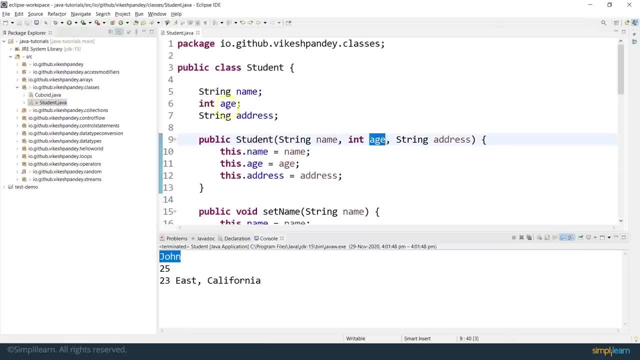 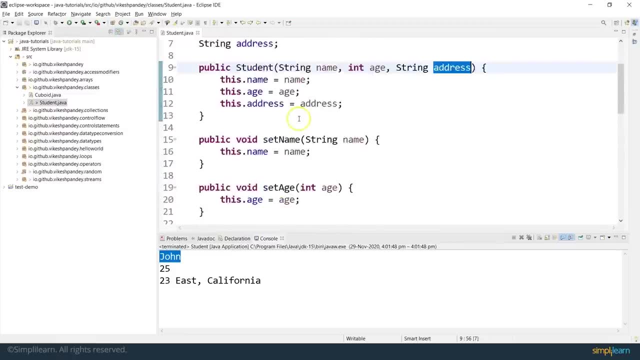 value. the age value which you supplied got set against the student's age and the address value which you supplied got set against the student's address, and that's how you're going to create a class. so remember, whenever you create a class, identify the properties and the behaviors like 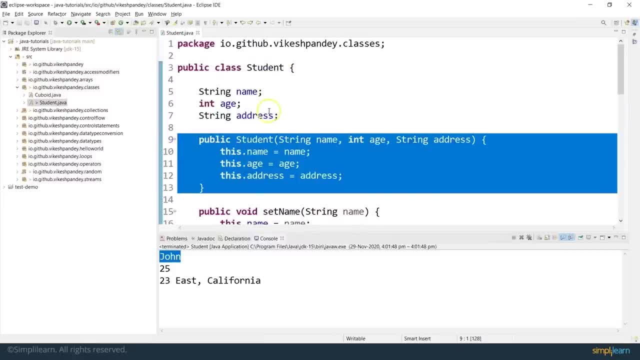 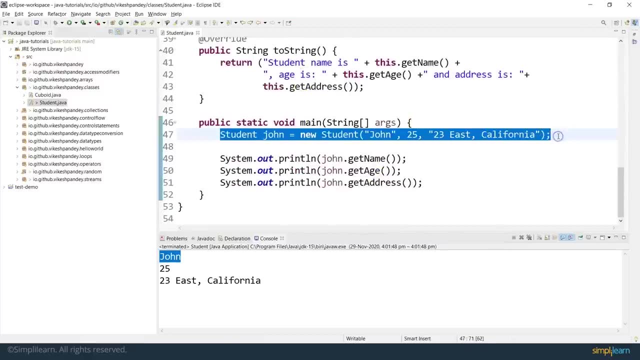 setters and getters. write a constructor which can cover all the values which you want to initialize and after that just initialize that class, create an object of that particular class, basically, and once you have the object, then you can call getters. you can also call this in this way: 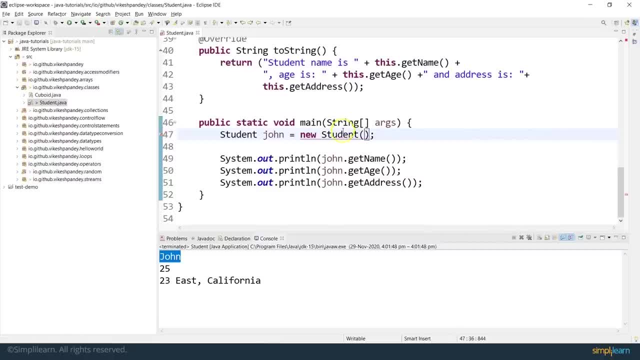 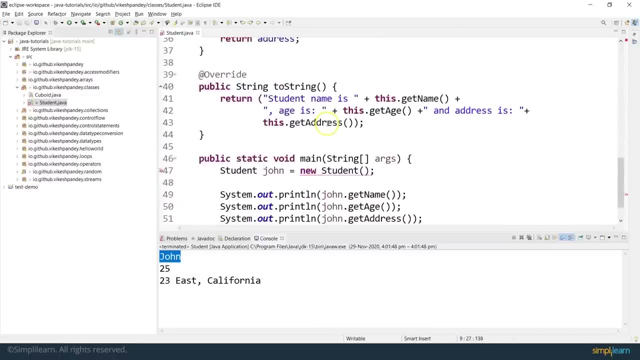 if i don't supply any of this, then it currently it complains. and why it complains. i will cover that in the following session. when, whenever, when- i will cover the multiple constructors concept. but remember, you see this behavior here that if you have created a constructor which accepts some arguments and if you supply this kind of 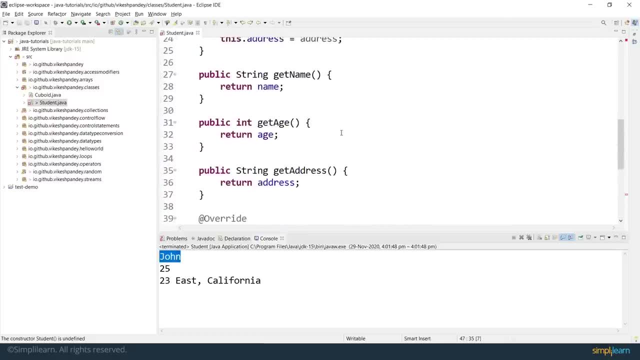 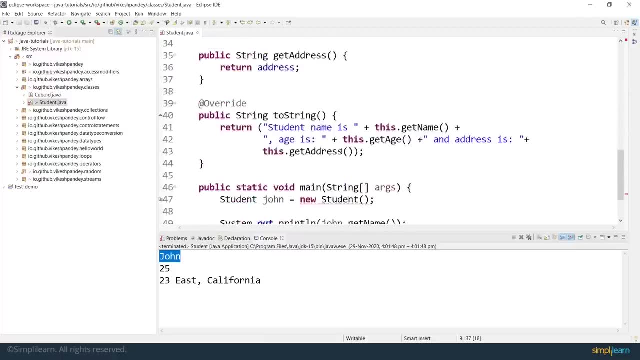 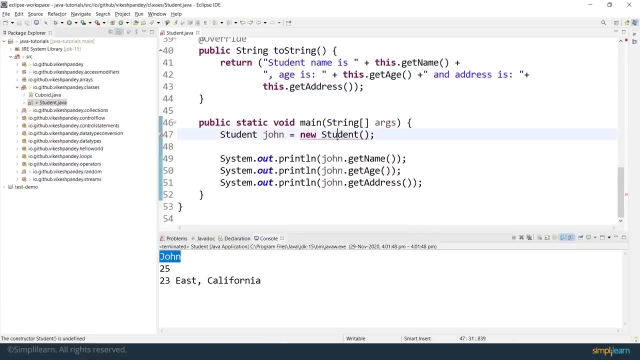 initialization, then student class does not have a constructor which is parameter less. student class has only one constructor which is taking three parameters and that's why java complains, because it is not able to find a representation of a constructor which accepts no parameter. but, like i said, we will cover this. we will find a solution to this particular problem in the in the coming in. 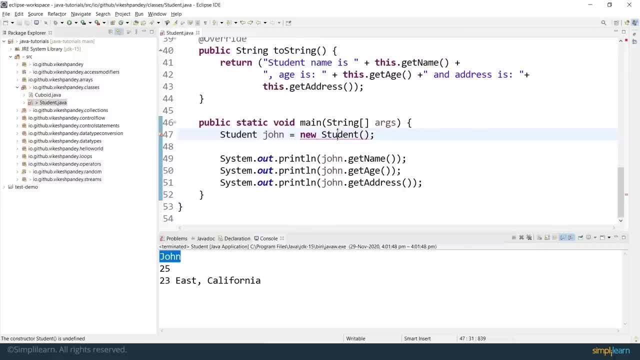 the coming session, but for this session. this is also a solution and it is going to be absolutely very important. all we are going to cover. We covered about classes, we covered about objects and we also saw how we can write getters and setters. 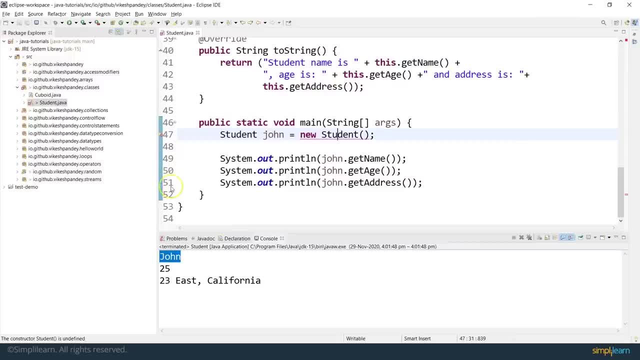 We can initialize those methods, initialize those objects, and we can access the properties of those objects using the getters, And we can also call the setters to modify the values as well. similar to this: Choose from over 300 in-demand skills and get access to 1,000 plus hours. 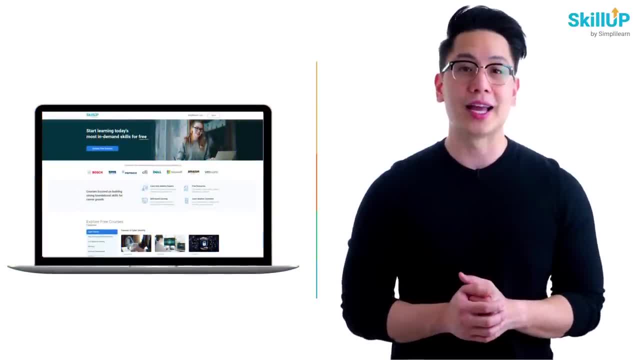 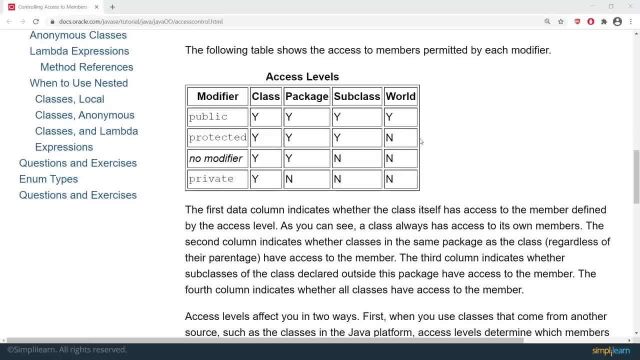 of video content for free. Visit SkillUp by Simply Learn. Click on the link in the description to know more. Let's get started with access modifiers in Java. So when we talk about access modifiers, let's understand what is the underlying philosophy of the reasoning behind this. 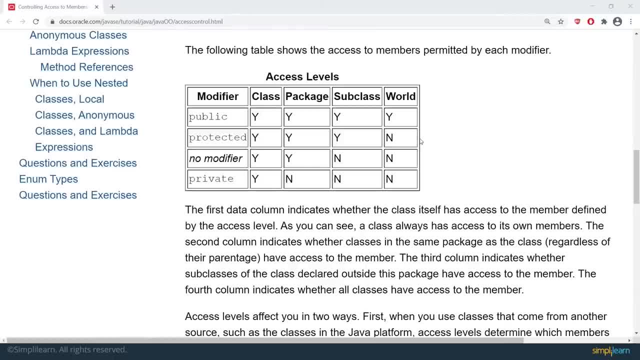 And the reasoning is very straightforward. It can be even wrapped into a single word, which is called security. The reason is that you will be creating multiple kinds of objects and variables while you write your Java program, And you should always write your Java program. 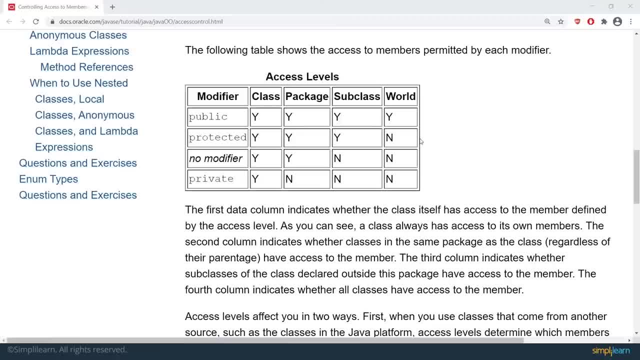 or any program in a manner that only the intended classes, packages, modules or applications should be able to see what they are supposed to see. So as a consumer application, I should only be able to consume the variables which I am expected to consume. 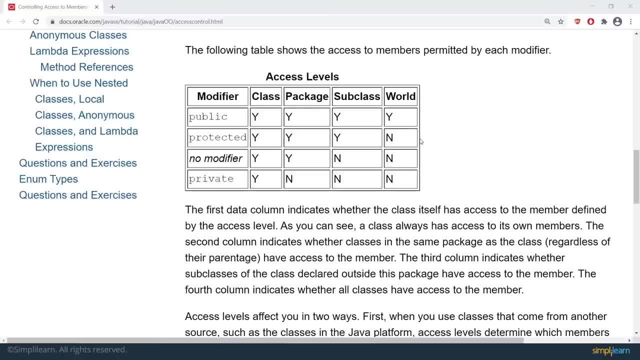 I should not get any variable, or I should not even have access to any variable which I am not supposed to access. So the idea is providing the least privilege principle: Give me the least privilege, Give me the least privilege, Give me the least privilege. 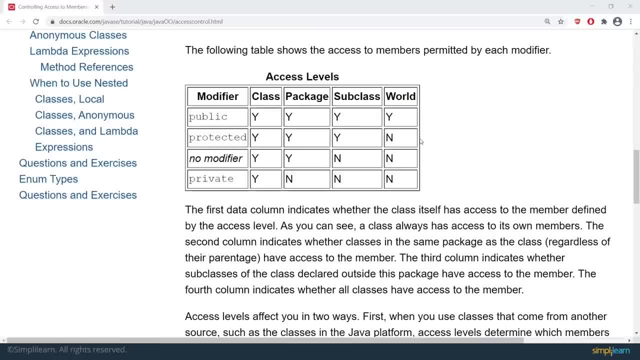 Give access to different functions, different variables, different programs only by providing them the kind of access which they need to run efficiently and do not give them complete access. So with that notion in mind, Java created the concept of access modifiers and it created these three modifiers which 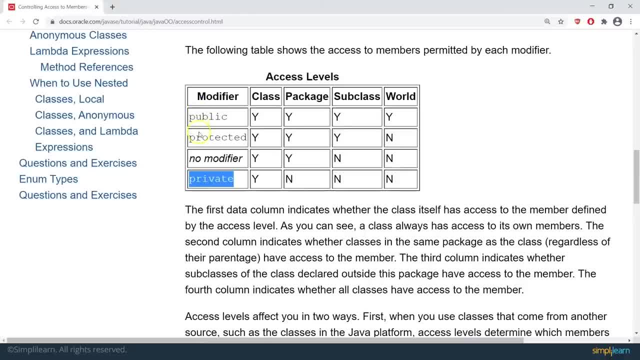 are called public, protected and private. If you do not provide any modifier, then it goes to no modifier, or some people also call it as default modifier, which is also a type of access modifier. So let's understand theoretically first how it works. 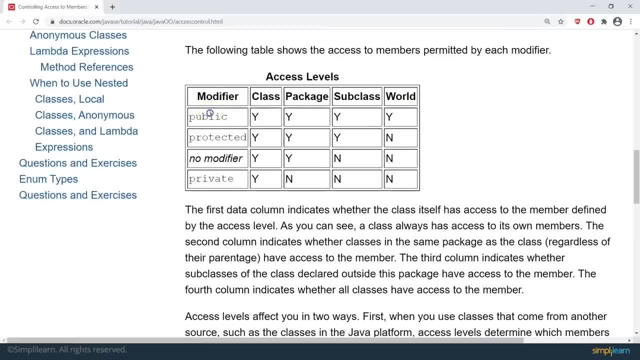 and then we will try to have a look at an example. Let's understand the first one. First of all, these modifiers are keywords, and you can use these keywords in front of classes, in front of variables and also in front of methods. 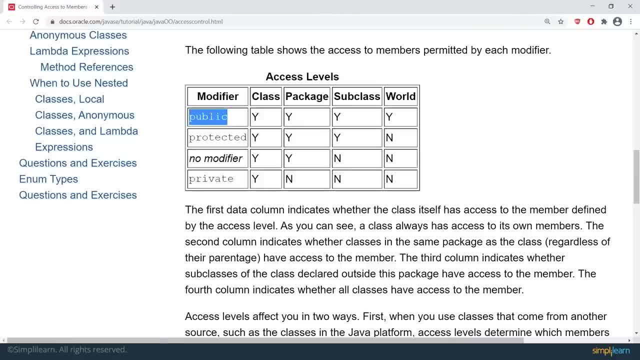 And you might have already noticed this particular keyword called public in front of all the classes I've created, or even when we talked about the public static void main method, we saw this public as a keyword. It is basically an access modifier And whenever you put public in front of a class or a variable, 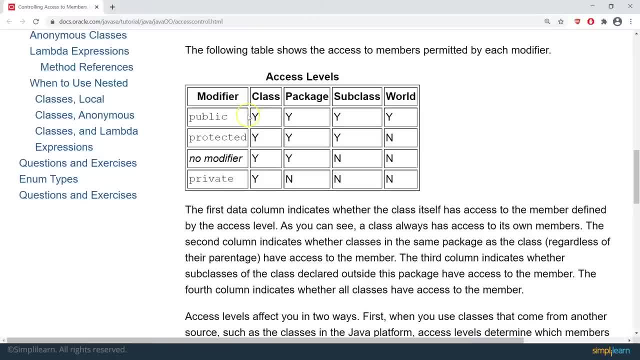 or a method, that particular component becomes available to the whole of the program. It will be available to the whole world. basically, Any subclass or any package or any other class which might have been written in your Java program will be able to access that particular class or variable. 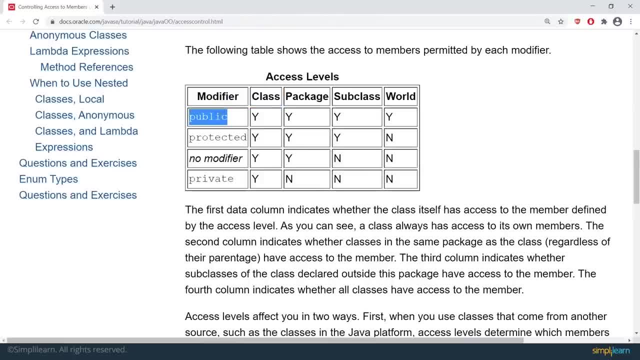 or method. if you put public in front of that, The second modifier level is protected. One of the other things which you will understand as I explain this is that as you move down into this particular table, the access level will start getting more and more restricted. 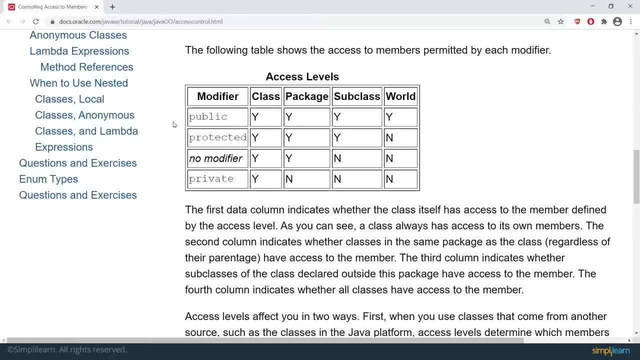 And by restriction I mean that less and less components will be able to get access to those modifiers. So if you write protected in front of a class or in front of a method or in front of a variable, then everything within the class will be protected. 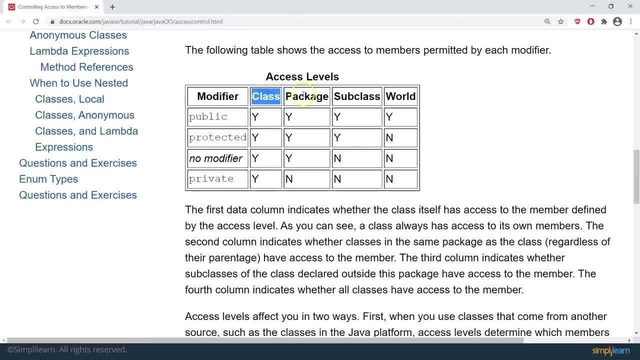 In that particular class, we'll still be able to access it. Everything within the package will still be able to access it. I still haven't covered the concept of package, but I briefly touched upon it, showing you whenever we write a class, we have a package in front of it. 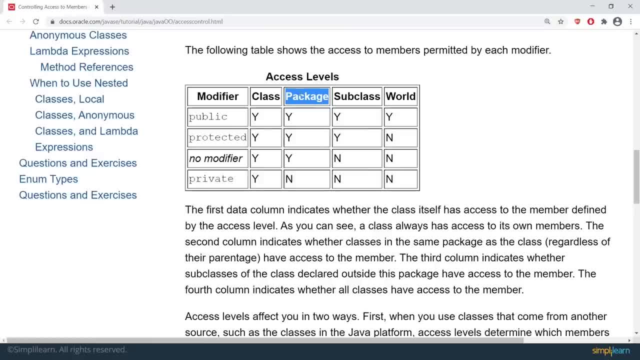 And package technically is just an aggregation of the classes. If you have to write multiple classes and wrap all of those classes into a single logical bundle, that would be called a package. Just to show you an example, these all are packages. 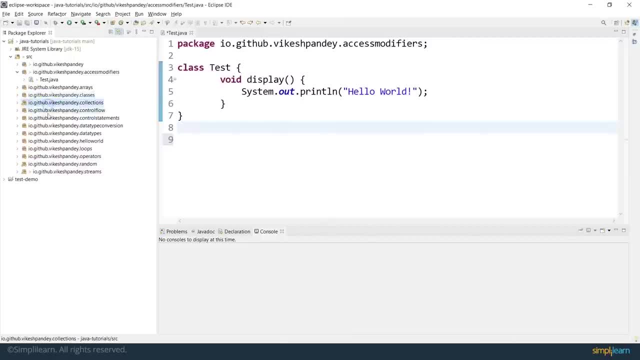 which you see here, You see this square box here and you see that these names, these all are packages And these packages contain multiple classes And technically, that's all. the packages mean that you can wrap multiple related classes into a single package. 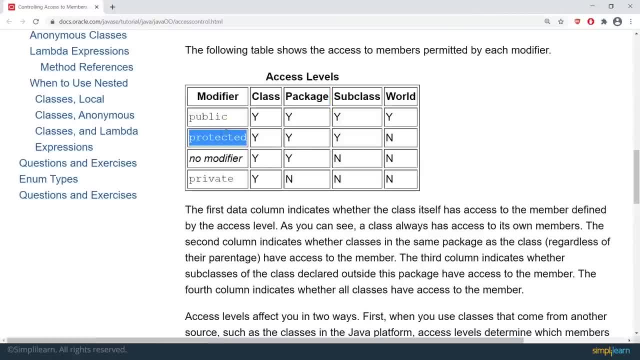 So, coming back to the access modifier, whenever you write protected in front of a class or a variable or a method, then that particular component will be accessible to everybody within the same class, everybody within the same package. It will also be accessible to everybody within the same class. 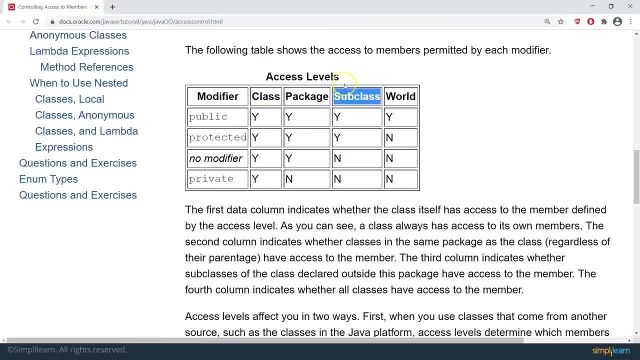 It will also be accessible to everybody within the same package. It will also be accessible to everybody within the same package, Which is a subclass of the class. This is again a new concept which I have not covered, But this basically means a child of this class. 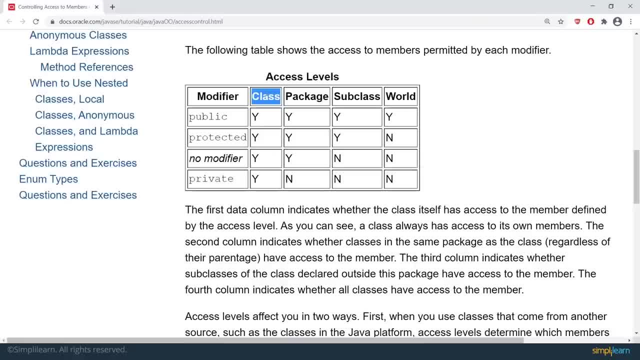 Now, what is a child of the class? We will cover that concept in detail when we will talk about inheritance, But for now you can understand that it is basically an extension of the class. So the moment you declare something as protected, it can easily be accessible within the same class. 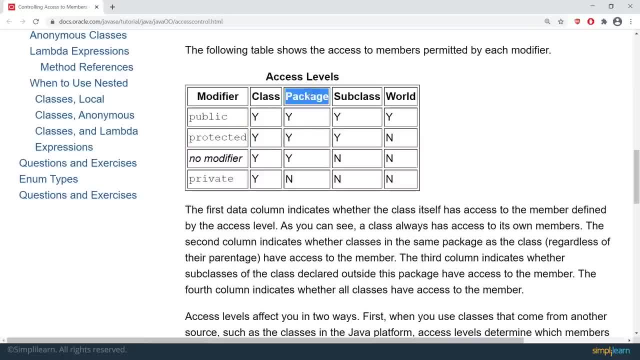 in which this protected component was declared. It can be accessed in the package. It can also be accessed in the subclasses of the class, But anything outside the package will not be able to access it because you see an n here. Then we have the default access modifier or no modifier. 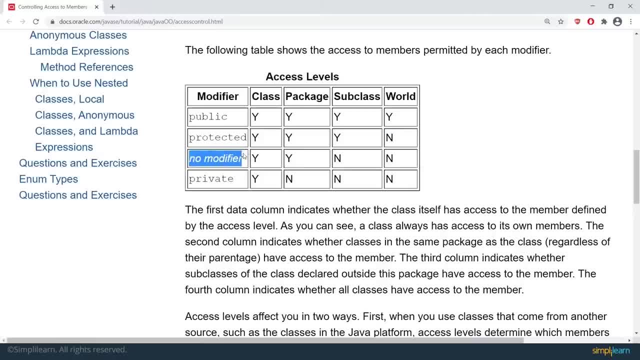 If you do not write anything in front of a class or a method or a variable, it gets the default access modifier privileges And that privilege means that anybody within the same class will be able to access that default variable or a default component. 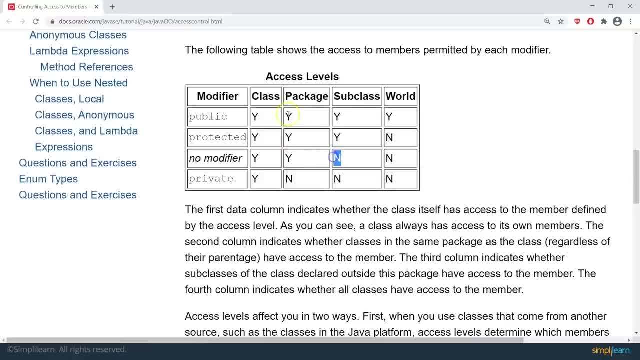 Anybody within the package will also be able to access it. The subclasses of the class where the default component was declared. those subclasses will not be able to access it, And anybody outside the package will obviously not be able to access it. Then comes the last one, which is the most restricted. 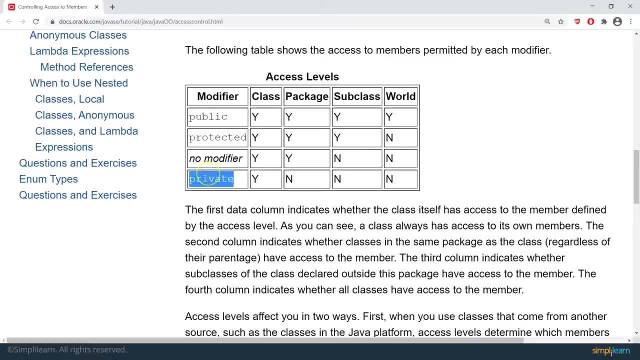 privilege which is called private. So if you put private in front of a class or in front of a method or in front of a variable, that component will only be accessible within the class where it was declared. It will not be accessible in the package. 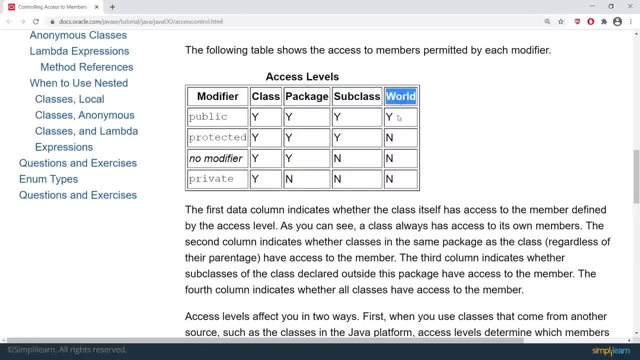 It will not be accessible in the subclasses and definitely not be accessible to anybody outside the package. So private is the least privileged or least access permission level you have in Java. Once you write private in front of any component, that only the class's other variables, the same class, in. 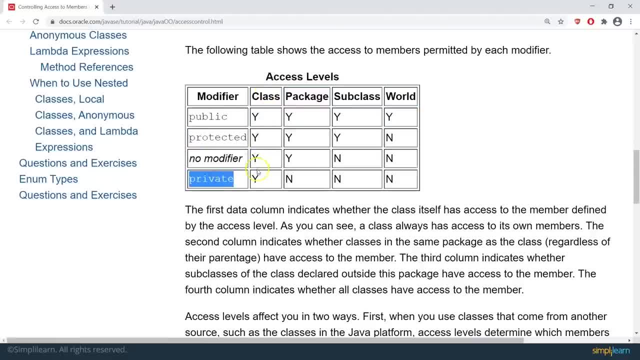 which you declare this particular private variable, only that class itself will be able to access it and nobody else will be able to access it. And as you move above, the accesses become more and more lenient. You can see there's just one y and three n here. 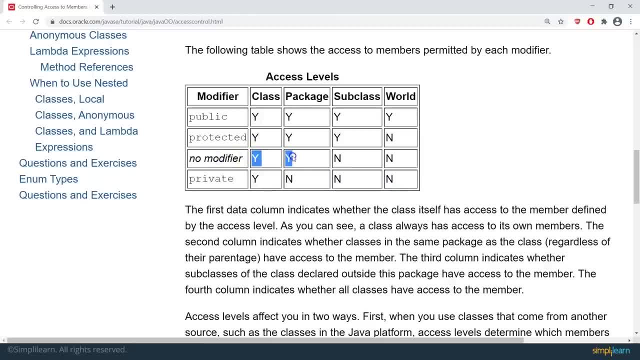 The moment you move a bit above to the default modifier, you get two y's, So everybody in the class and everybody in the package will be able to access that particular component. For the rest of the other world it is still unknown When you write something as protected. 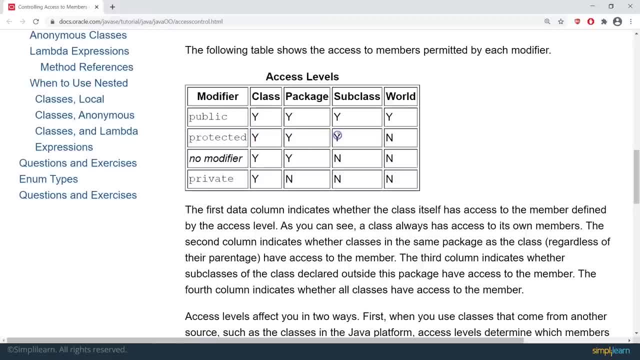 then everything in the class, everything in the package and everything in the subclasses will also be able to access it. Rest of the world cannot access it, And if you write something as public, then anybody can access it. It's like y everywhere. 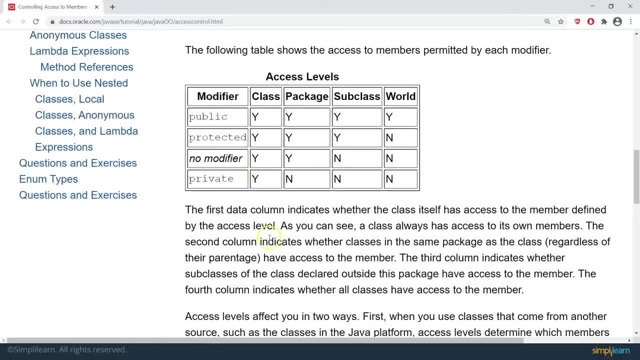 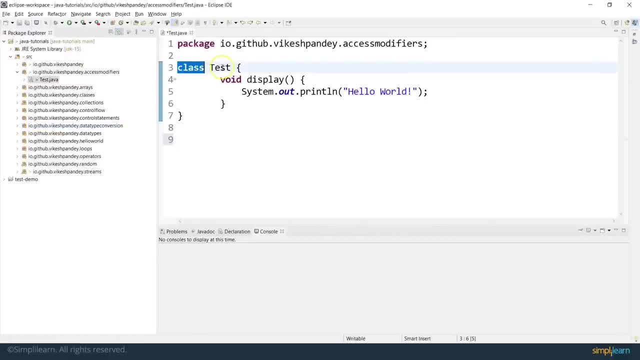 So that is how the access levels work. Now let us understand this with the help of example. So I will go here and I've just written a very simple dummy class here, which is a class called test, And I have a method here which is a display method. 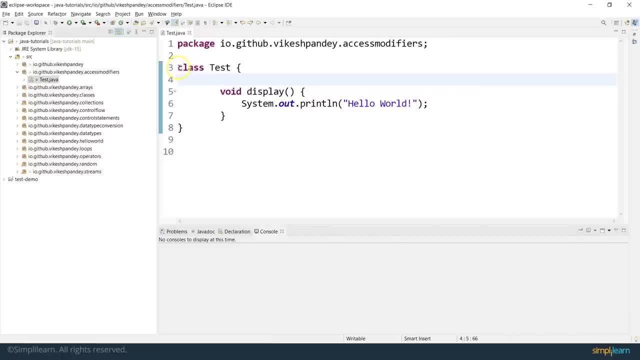 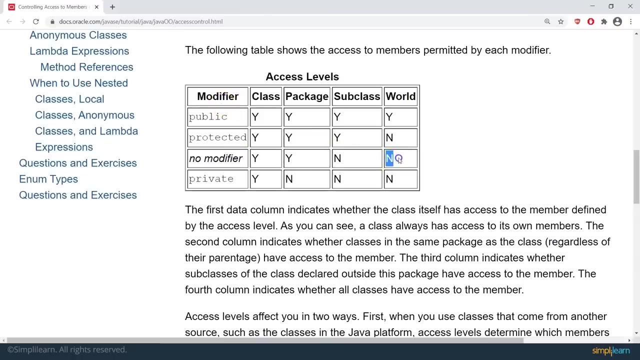 So very simple class, nothing fancy here And, if you notice, I have not put any kind of public, private or protected modifier in front of the class. So this will get the default privilege. If something has default privilege, then the whole world will not be able to access it. 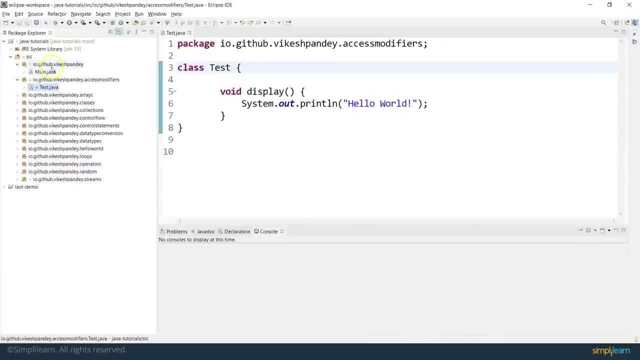 So let's go to a different package. Let's go to this package which is here, And let's try to access this particular test class. So we will try to access this testjava here in the main class. So let's try to do that. 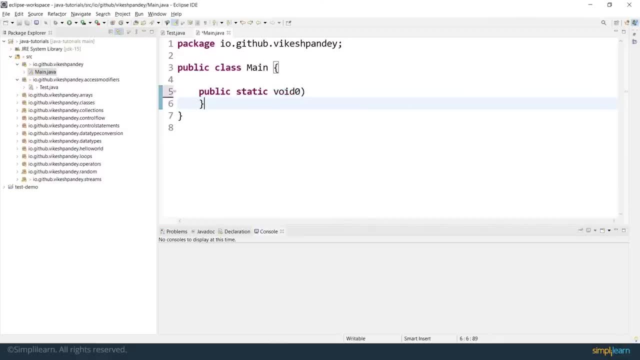 Let's say test t equal to new test. I'm just initializing the same class. So what do I get? I get a compile error. Let me try this. Let me try to fix it if I can, And I cannot fix it. 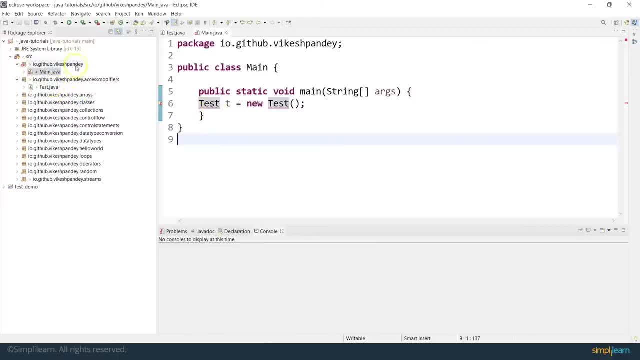 If you see, I'm just trying to use this particular test class into a different package, But that package is not able to see the class at all. I'm getting a compilation error. And if I try to click on the error, generally, Eclipse provide me suggestions. 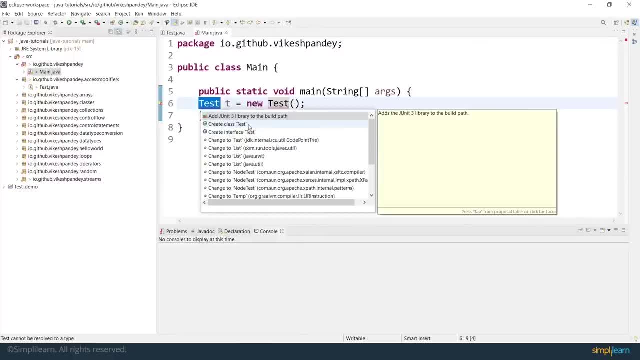 to import this particular class, But Eclipse is not able to find any class with the name of test which can be imported in this package, which is a different package than the one of the test class. So we cannot access it because it's. 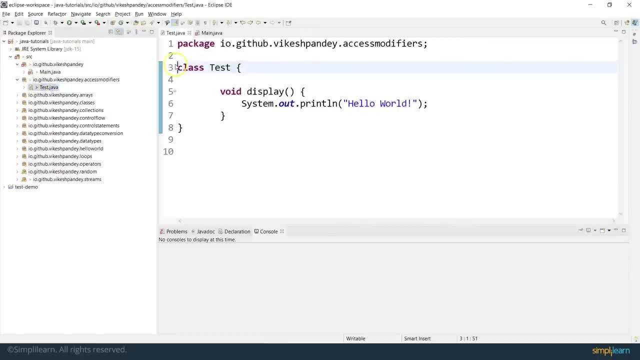 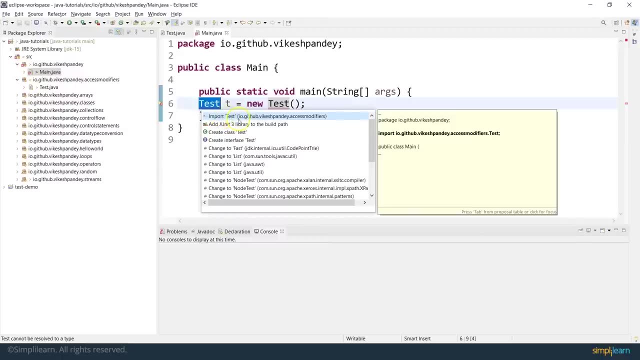 the default access. Now let's go back to the test class and let's make it public. So I've just made it public here And now, if I click on this again, I get the suggestion. If you see, the suggestion was not there earlier. 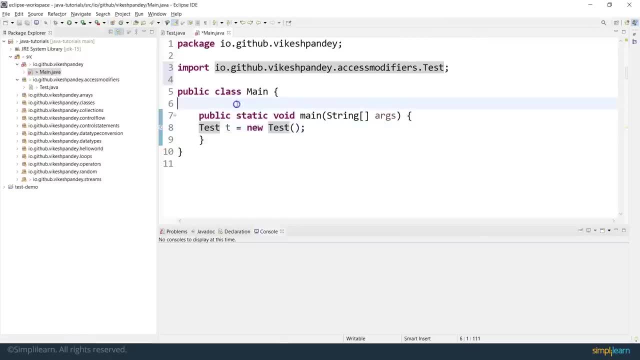 Now it says import test And if I click on this double click it gets imported and everything is happy. So you can see the whole access modifier in effect here, the default versus public. You can also try the other kind of access modifiers. 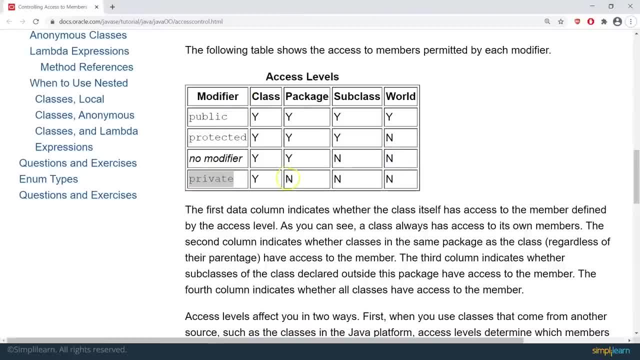 Let's try private as well. I think private will also have the same effect, because it will still not be accessible from the package or from the subclass or from the whole world. We already saw this particular in effect, But we'll see the private in a different way now. 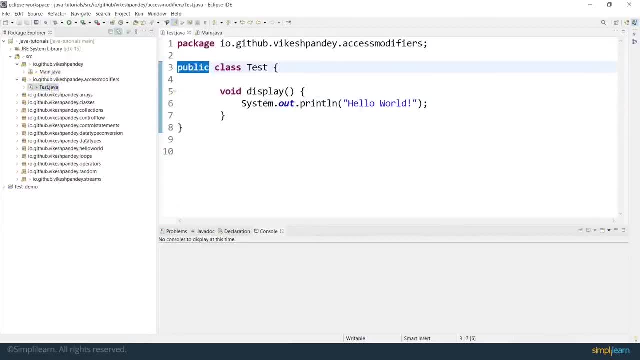 So, going back to the test class, I've made the class as public, But the method here is default. I've not exposed this method to be used outside the class. Let's see what happens if I try to call this display method from the main class. 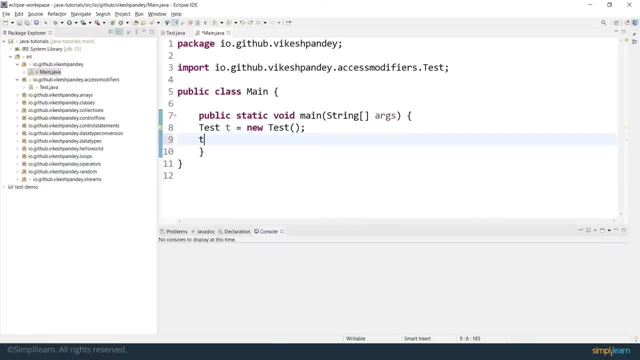 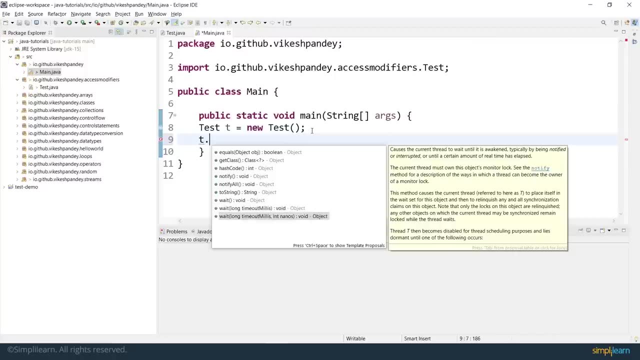 So I have successfully called it, I have successfully initialized the class And if I say t, dot, and if I look at the suggestions here, I do not get the suggestion of the display method. Why? Because it is default. If I go back, make it private. 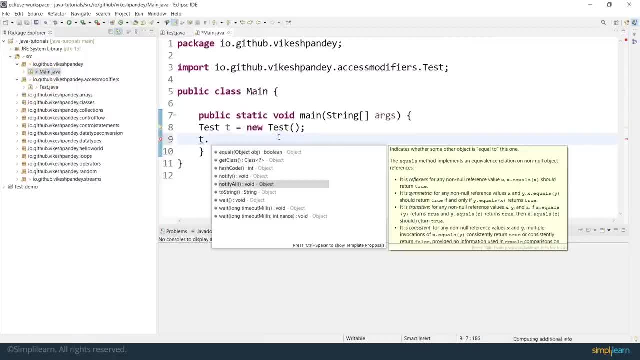 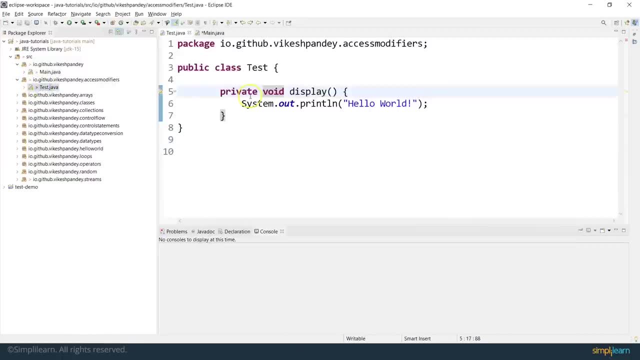 can I now access it? Let's try again. Nope, still we can't access it. Eclipse is not even able to find it inside this package because it is private. Let's go back and make it public. So I've made it just public now. 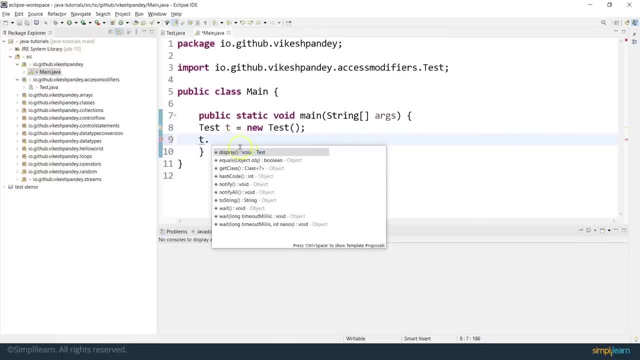 Going back to the main class and again saying t dot. now I get that display suggestion as the first suggested method here And now I am able to use the display method once I have made it public. So you see the moment you change the access modifiers. 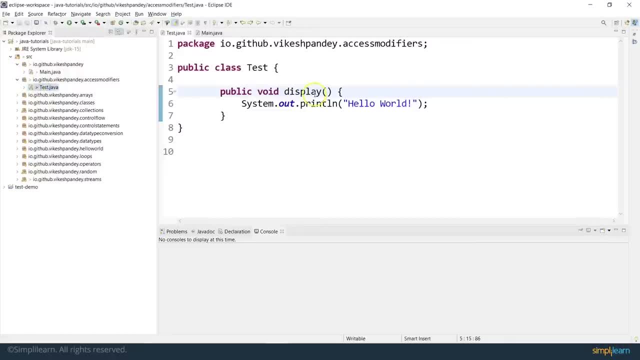 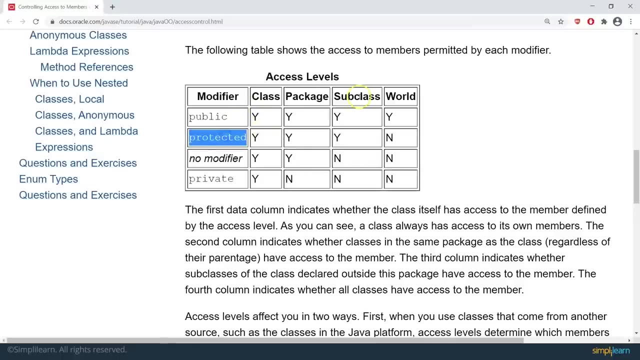 the changes are propagated immediately and you can see the public versus default versus private in play here. We can even go into further detail by using the protected. but for protected I have to explain the concept of subclasses. So I will cover this protected versus subclasses concept when I talk about that in the next episode. 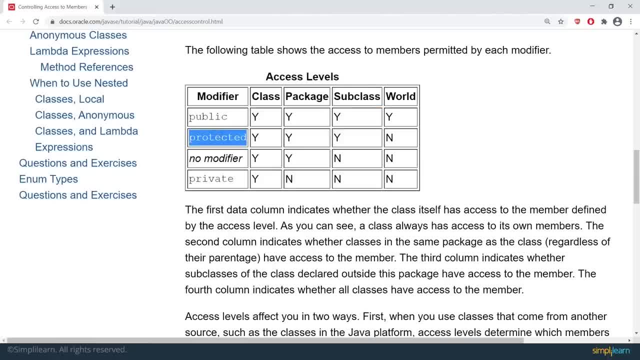 about inheritance, and there we will see the usage of protected variables and the protected access modifier, but we saw the usage of public, the default modifier and the private modifier. do check out the documentation for these access modifiers and i would strongly suggest you to play around with this. get more comfortable with this concept of different kind of modifiers. let's also run an 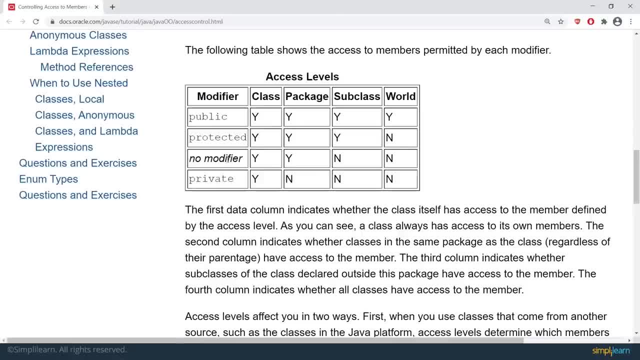 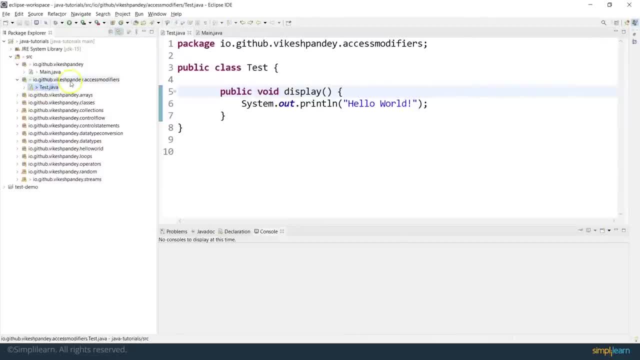 example, for for understanding the default modifier in a better sense, because we can see that for the package it says y right, so let's go back to eclipse and within the same package where we created test class, let's create another class. let's call it test demo. so i will just click. 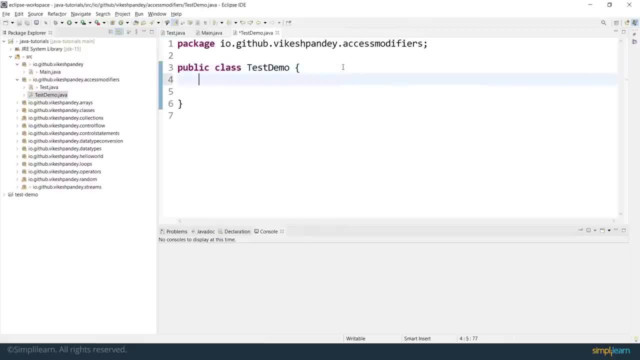 finish, i get a new class. let me also write the public static void main method here. so i get the public static void main method here and let's try to access the test class here within the same package. so let me again go back to the default privilege here. 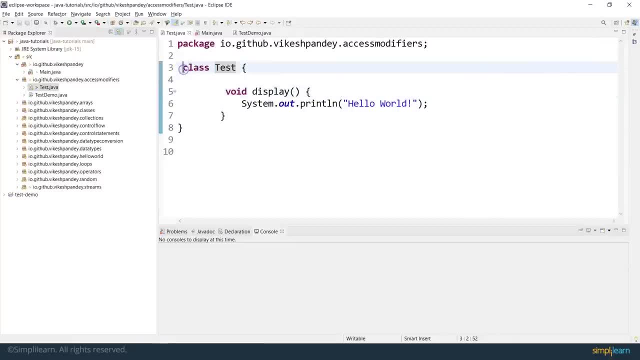 so i put the test class access as the default class or default access, and same goes for display. so can other classes in the same package access the test class. now let's see that if i go to test demo and here if i try to get the test class initialize, does it work or does it give me a 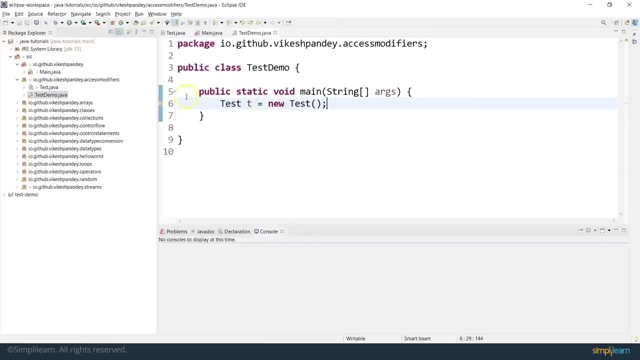 compilation error. yes, it works. it works because the test class and the test demo are in the same package and test class has a default access privilege. so let's go back to the test class and let's see what we can do here. so let's go back to the test. 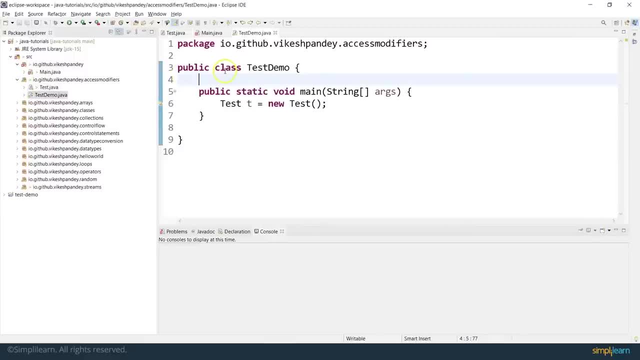 class and let's try to run one more variation of it to understand the usage of the private method better. going back to the test class, this display method has the default privilege right now. so, going by that logic, if i say t dot, i should be able to get access to the display method. and yes, 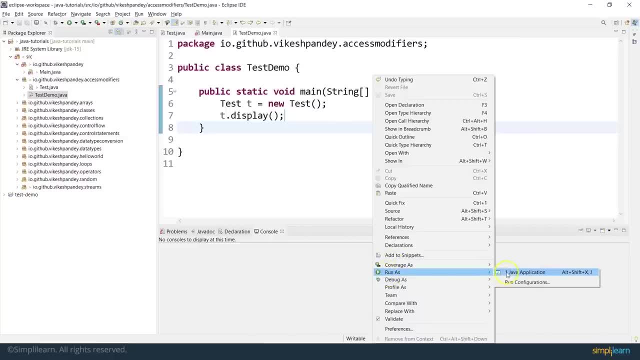 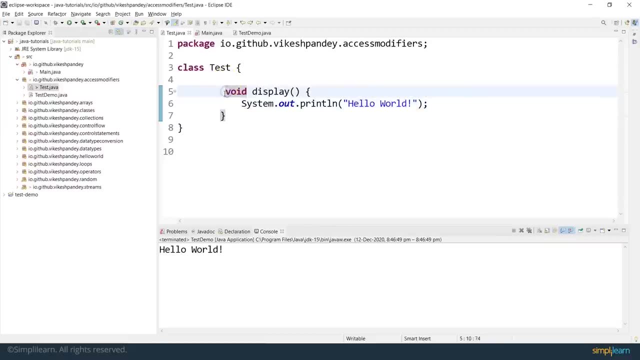 that is possible. if i run this particular program, i will be able to get whatever is given out by the display method, which is hello world. now let's try to make this particular method as private and let's try to activate the display method. and let's try to activate the display method. 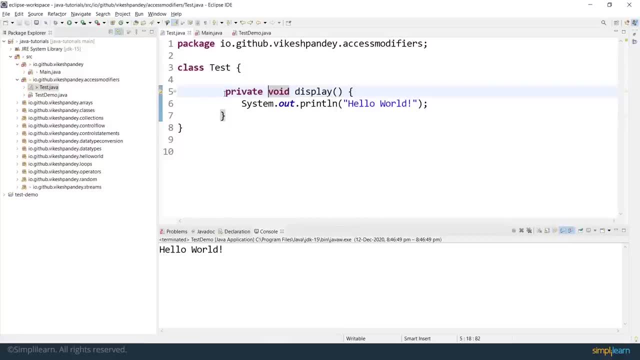 and let's try to activate the display method and access this method from one of the other class in the same package as of the test class. the class is default, the method is private and, if you see, this class has already turned red. there is a compilation error because now the display method. 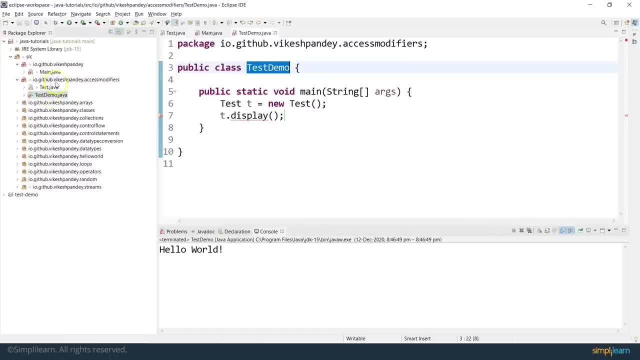 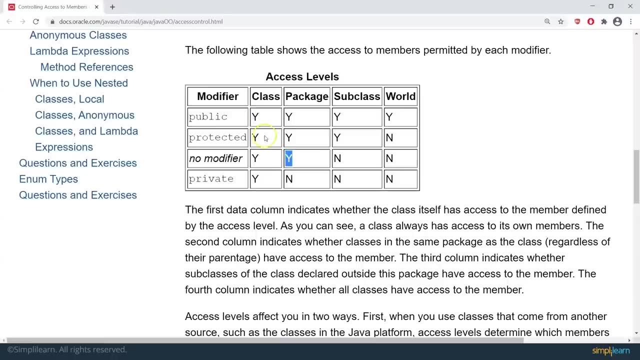 is not accessible to the test demo class, even if it was in the same package. it's not accessible because the display method's privilege or access modifier has gone to private- now exactly the same as explained here- because it has become private. so the package is private and the display method is. 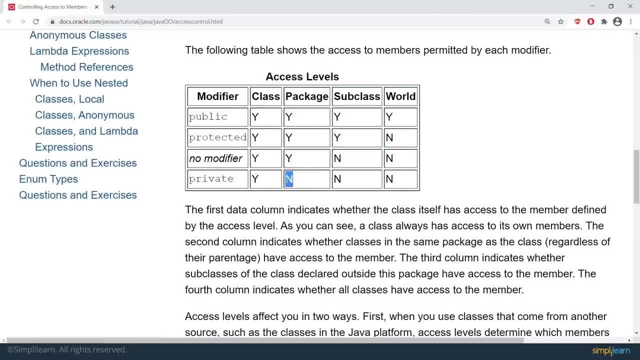 not accessible. so it's private and basically it's not accessible if you haven't already done it, and if you haven't already done it, then you haven't been a member of a large level members cannot access it. there's an n here, so this is- this was another variation to show you how you can. 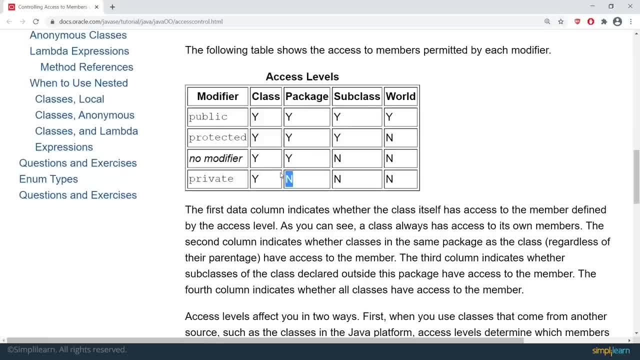 use public, protected and private together to only expose the members, methods and classes which are supposed to be exposed to the consumer. this is a very critical and very important concept to be used in java and it is used from a very simple program to all the highly complex application. 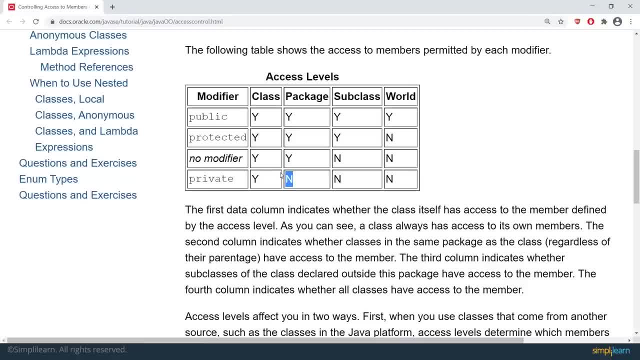 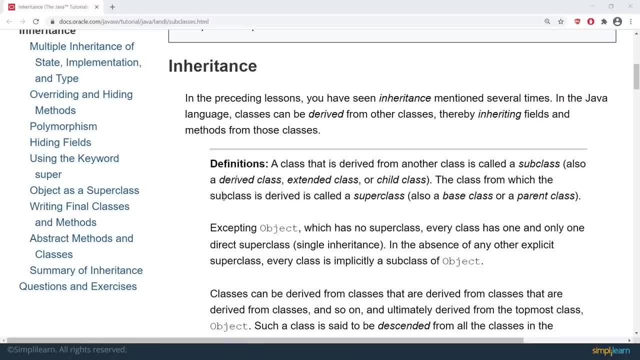 this is sort of the bare bone or the lean foundation for any kind of basic security level which you need to build your application. let's get started with inheritance. so inheritance is basically one of the most important properties of any object-oriented programming language. it's basically a concept and the concept says that what if you have a scenario where you want multiple? 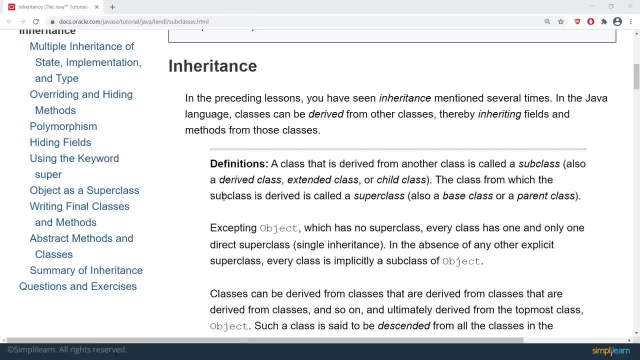 classes to share similar behavior and similar properties. let's understand this with the help of an example. let's take the example of a bank. when you go to a bank to open an account, there are multiple types of accounts. there can be a savings account. it can be a type of current. 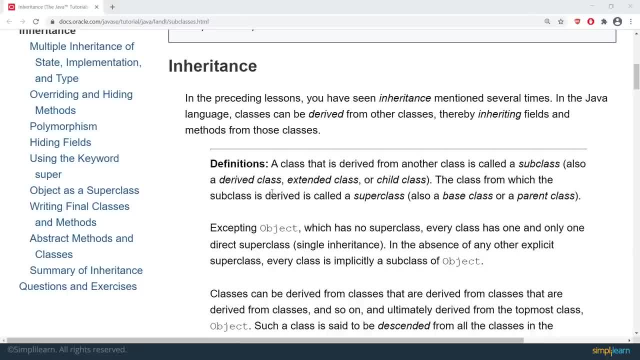 account. there can also be a different offering for personal account and commercial account, such as for businesses. then you may also have loan accounts, which are having different kind of properties. so all of these types of accounts are still technically accounts and they will share some similar properties. for example, all of them will have to maintain some sort of an interest. 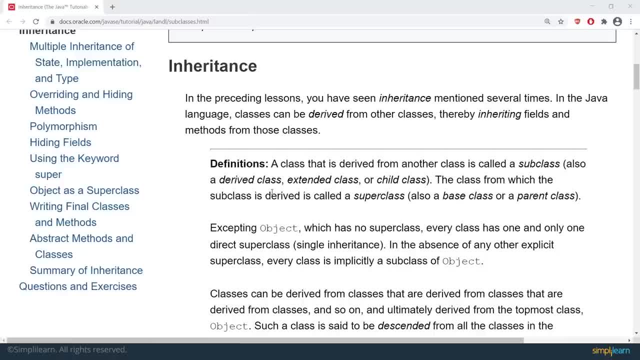 rate, for example. all of them will be. you use to either deposit money or withdraw money, so there would be some kind of similarity across all of these types of account classes, but at the same time there will also be some sort of differentiality amongst these classes. the way you will calculate the interest rate for a current account will be. 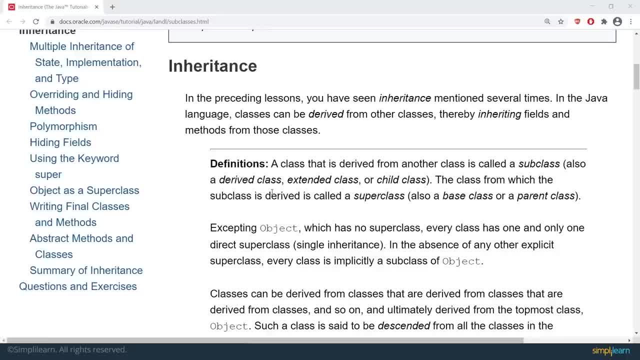 different from the way you will calculate the interest rate for a savings account, and the same applies for commercial account, personal account, loan account, etc. so you see that we have some common behavior, but at the same time we also have some common behavior, which is that we have to. 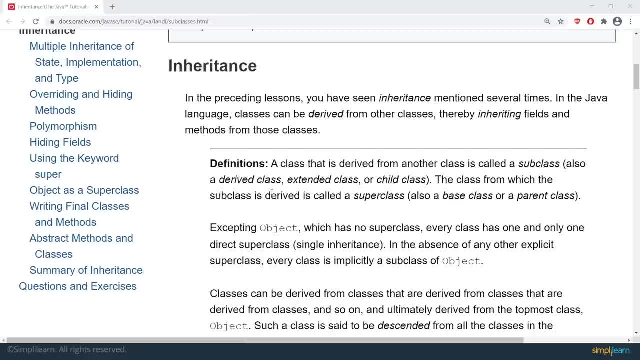 have some different behavior. so whenever you have such scenario, always think about applying the concept of inheritance in your application. there's another simple way to spot whether inheritance can be used at a particular place or not. inheritance is also called ISA relationship, so whenever you read the requirements from a customer, just try to find the words which use this. 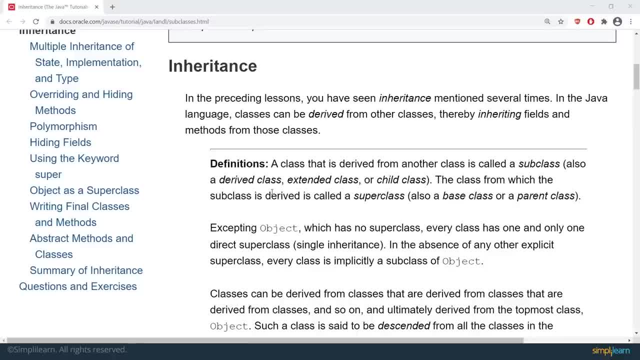 particular phrase is a, for example, car is a vehicle. savings account is available. here are two ways by which to spot whether the includes a type of account. similarly, you will find many other types of similar examples. so whenever you will see that is a relationship between two different kinds of objects or two different 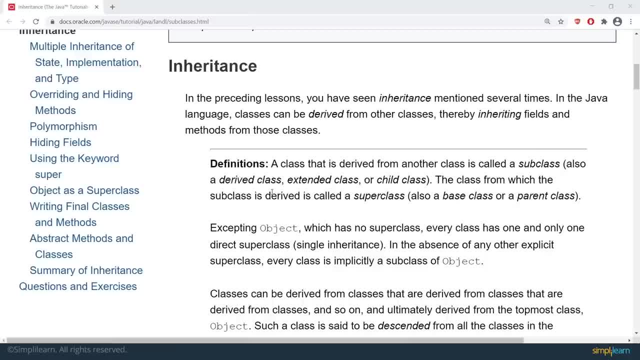 kind of entities. that means that there might be an inheritance relationship being applied between them, and that's how you will spot the usage of inheritance. so so far we have understood this concept that there would be some sort of relationship between the two classes. what will be this relationship? the relationship will be of parent- child type. there will be a parent. 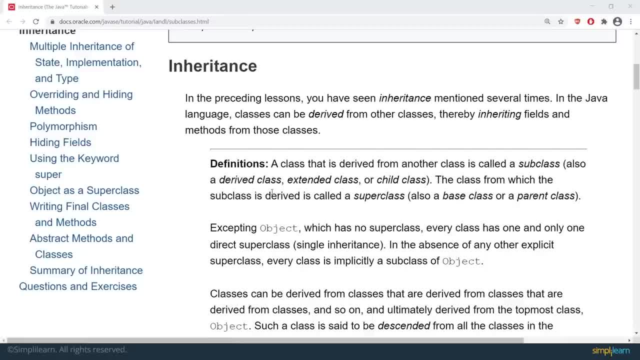 class- some people also call that as base class- and then there will be a child class, so the child class will be inheriting the properties and the behaviors from the base class or from the parent class. i will be using base class and parent class terms interchangeably during this session, but the 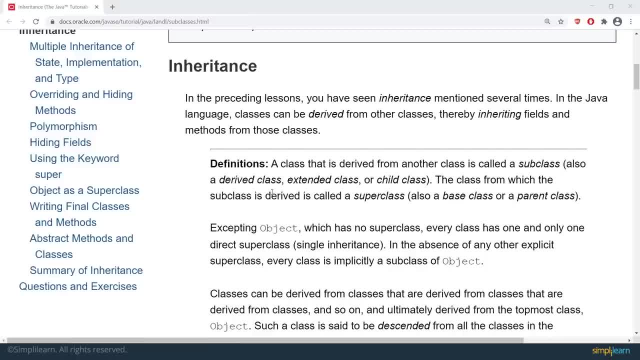 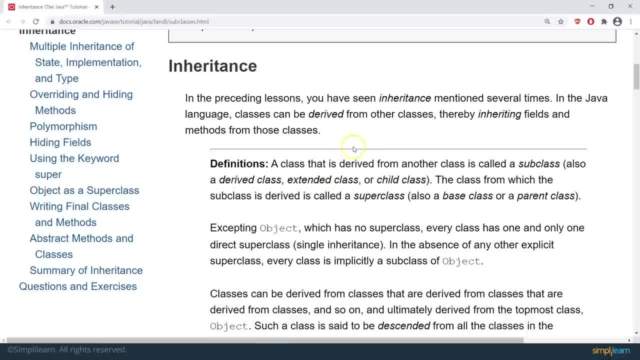 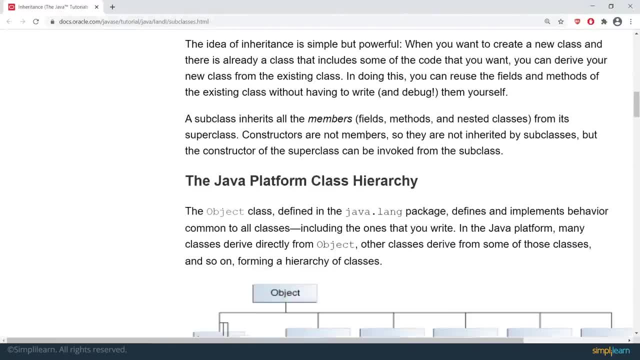 going to use that and I've just shown you the. what you see here is basically the official definition which is given by a Java docs. here we can read the definition as well, and the basic idea which I told you lies in the parent and child relationship and this is how you can conceptualize it, that you will have. 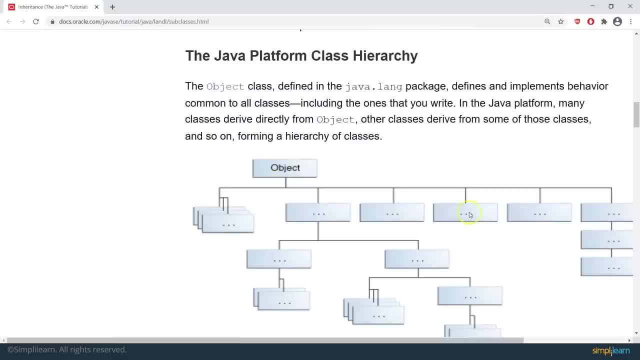 a base class or a parent class, and then you will, you can have multiple children of it, and then those children can again have their own children, and so on, so forth. so this hierarchy, this whole inheritance hierarchy, can go as deep as you want it to be, and that's the basic idea and basic conceptualization of how. 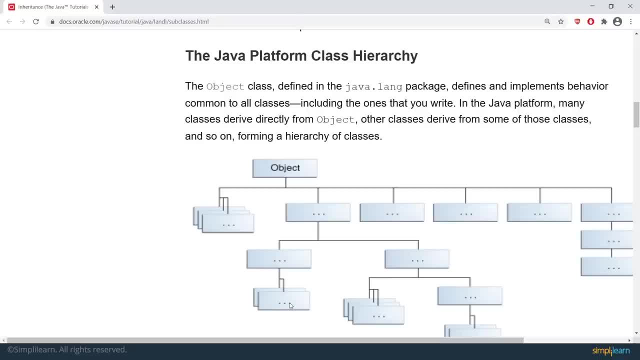 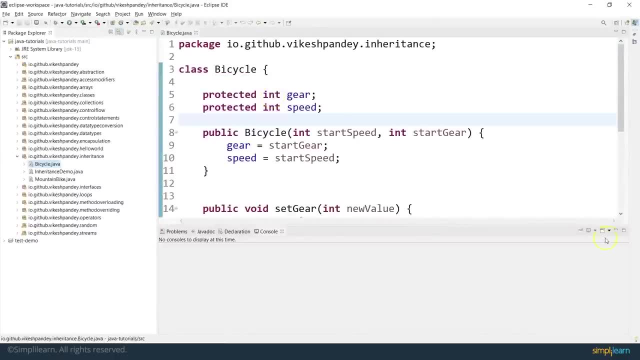 you understand and how you visualize inheritance. now let's move to Eclipse IDE and try to understand this with the help of an example. so, for this particular case, I have created a set of classes, basically, which we will be using to demonstrate a few basic concepts in the case of an example. so, for this particular case, I have created a set of classes, basically, which we will be using to demonstrate. 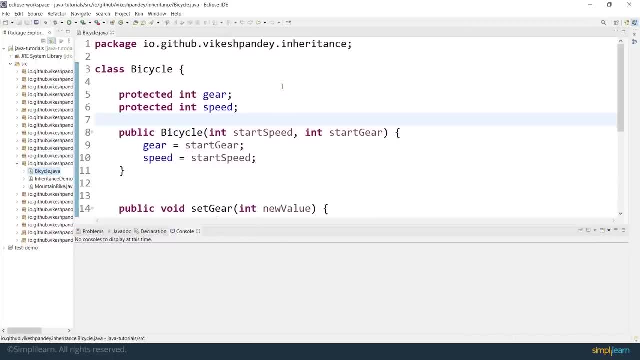 the relationship of inheritance, and I've taken the simple example of a bicycle. so a bicycle is again a very generic definition of any two-wheeler, and bicycles can have multiple types. there can be an all-terrain bike, there can be a mountain bike, there can be a city bike, there can be a bike which 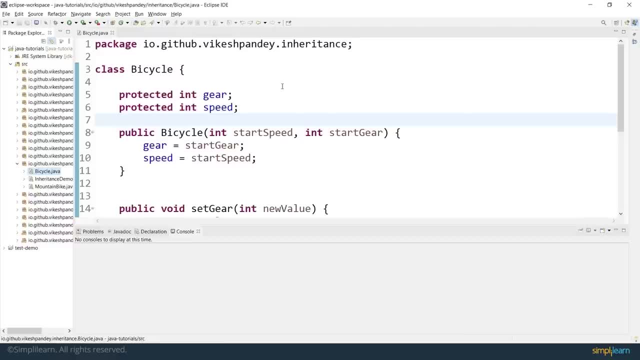 is specific, specifically made for ladies, and similarly, there can be multiple different types of bikes, but all of these bikes will have some similar properties. for example, all of them will have two wheels, all of them will have a seat, all of them will have brake, all of them will have some. 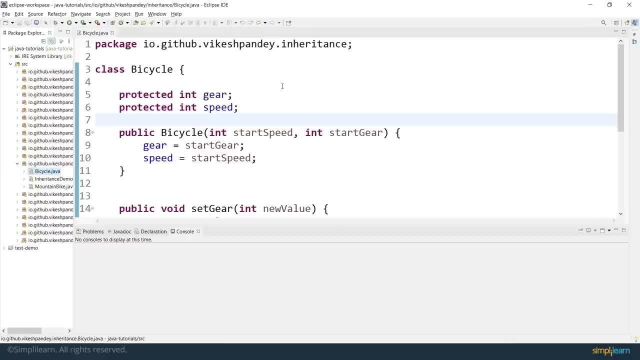 sort of of some sort of a speeding mechanism, whether they can accelerate or de-accelerate. so there will be some commonality but at the same time a mountain bike's features might be very different from a city bike feature. a mountain bike features might feature a mountain bike might have. 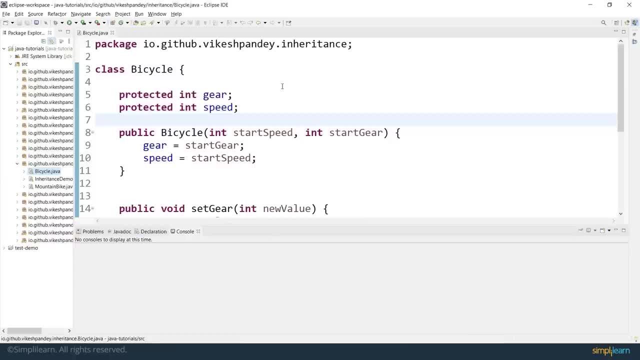 gears, for example, whereas a city bike might not have gears because you don't need that much of a variation in in inclination and declination when you drive down the road. so I'm trying to conceptualize the same example here, where I've created a class called bicycle and this is my base class. I define two. 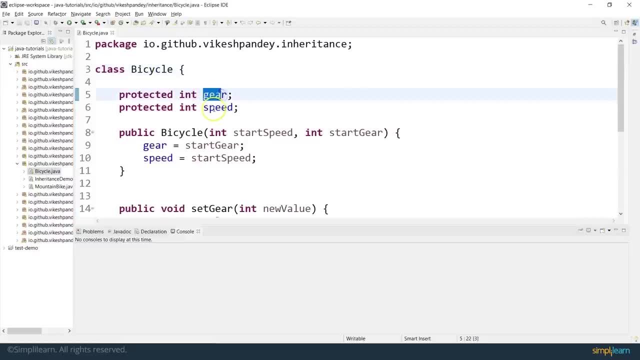 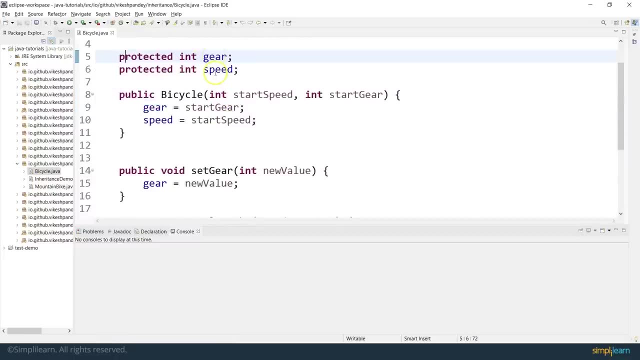 properties in the in the bicycle class, which is gear and speed. we will come back to protected in a while, but let's, let's leave that there. so I have two properties, which is gear and speed. I have a constructor where I'm initializing the starting speed and the starting gear, and then I have three. 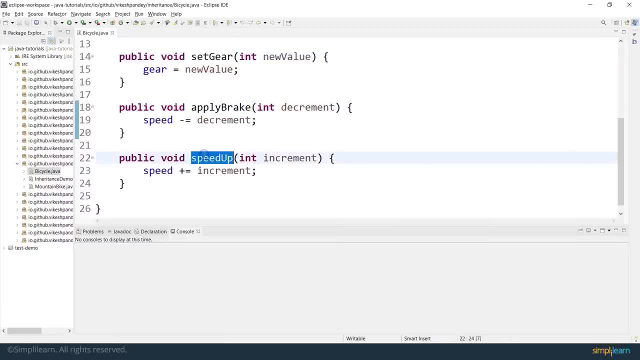 properties, which is set gear, apply brake and speed up. when I apply brake, the speed is going to get reduced. so that's why you see minus- equal to unary operator, and when I'm trying to speed up, the speed is going to increase. that's why I'm using the plus- equal to unary operator. so when you use the method speed up, the speed is going to be increased by the value you supply in the method. similarly, when you apply the brake, the speed is going to get reduced by the amount you supply in the method. so that's why you see minus- equal to unary operator, and when I'm trying to speed up, the speed is going to increase. that's why I'm using the plus- equal to unary operator. so when you use the method speed up, the speed is going to be increased by the value you supply in the method. similarly, when you apply the brake, the speed is going to get reduced by the amount you supply in the method. so that's why you see minus- equal to unary operator, and when I'm trying to speed up, the speed is going to increase. that's why I'm using the plus. 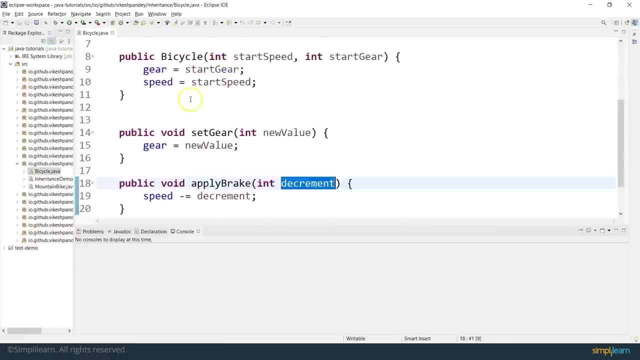 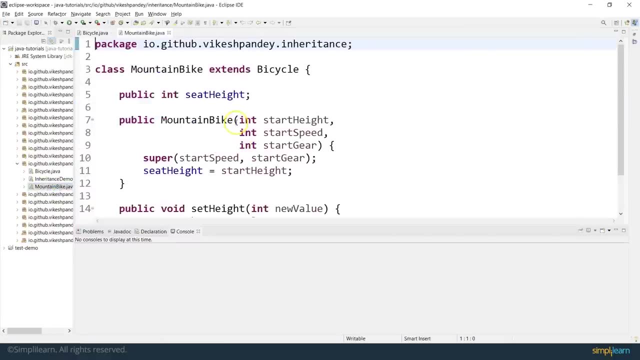 and that is my base class: bicycle gear speed and three methods. now let's have a look at the child class. so the way you will define the inheritance relationship in java is by using this extends keyword. remember, I told you to remember the extends keyword. so what you will do, 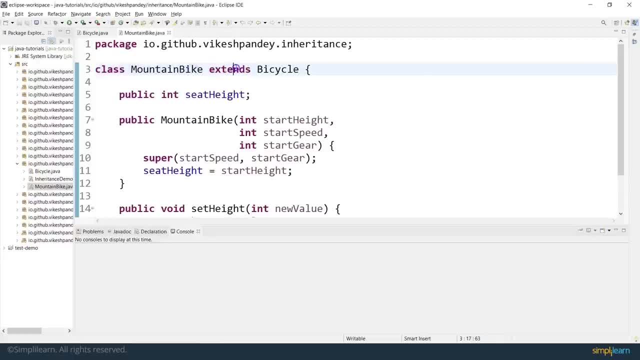 that you will write your class name as usual and then you will use extends keyword and then you will use the parent class name or the base class name. so here I'm saying class mountain bike extends bicycle and here i am providing an additional property. remember the whole commonality. 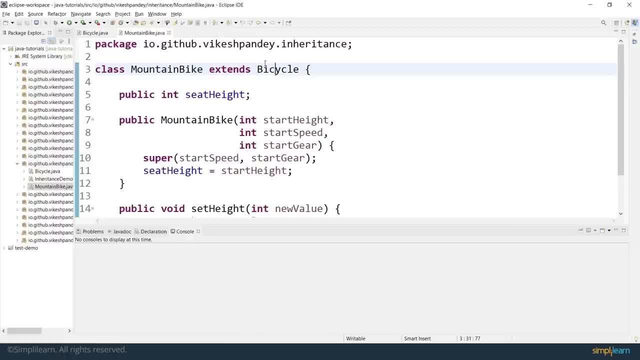 versus differentiality equation. so a mountain bike might have an extra property to adjust the seat height. so that's the extra property which mountain bike is having. and then, since this mountain bike is extending the bicycle class, this mountain bike class has the responsibility to initialize the bicycle class as well, and the way it will fulfill that responsibility. 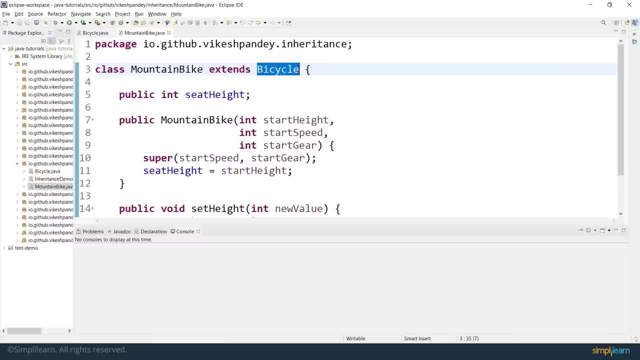 is by taking all the arguments of bicycle class plus the mountain bike class in its constructor, and that's why you see three different properties here. you see the start height property, which is the property of this particular class, which is the seat height, and then you see the start speed. 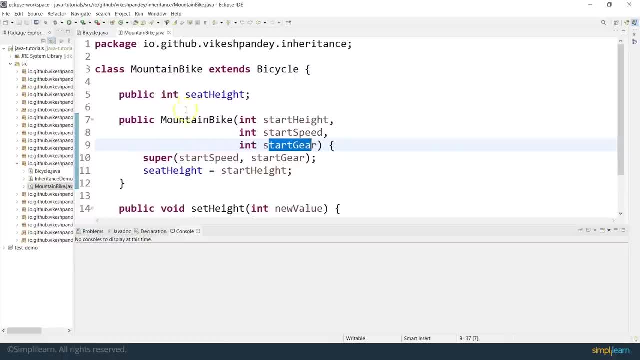 and start gear property which directly are not available in this class. but this class is inheriting those properties from the base class. remember the keyword inheritance here and then, once you do that, how do you initialize the base class constructor is by calling the super method. this is again a keyword in java and you will use this super keyword to refer to the 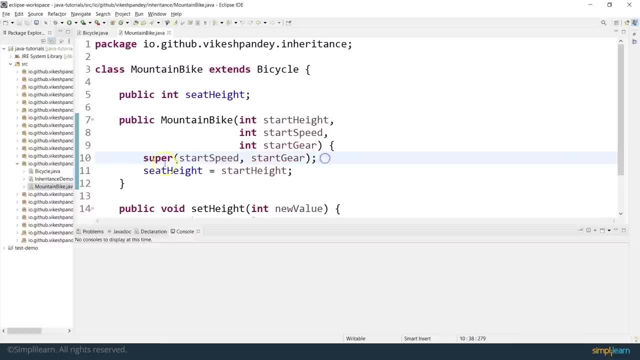 base class constructor in this way. so what you will do technically is that you will write super and you will supply the arguments which is required by the base class constructor. if i go back, the base class constructor requires two arguments: start speed and start gear. so i write super and 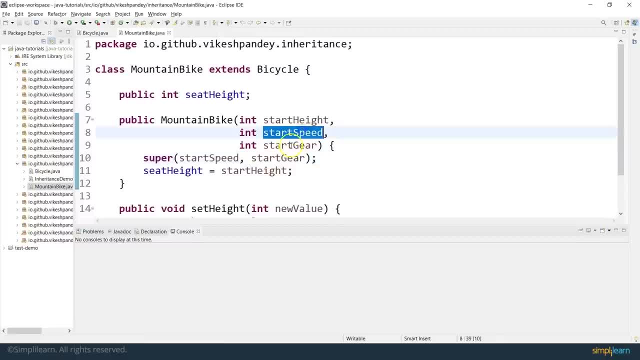 then i write start speed and start gear. so, whatever i got from here in the constructor of mountain bike, i'm supplying those values as is to super, and java will automatically take care of invoking this particular constructor the moment it it encounters this kind of statement. another another thing to notice is that this super keyword or super statement has to be the first. 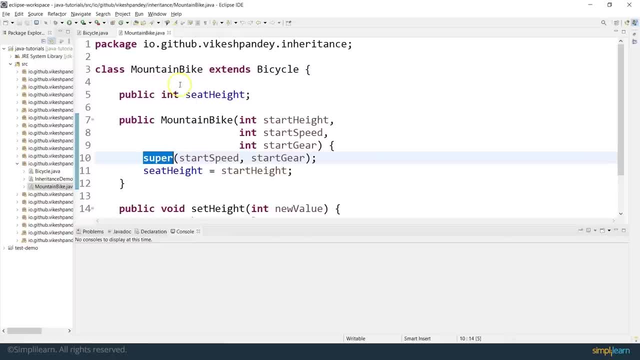 statement inside your constructor. remember that whenever you are dealing with inheritance and whenever you have to initialize the super class constructor or the base class constructor, use the super constructor invocation as the very first statement inside your child class constructor, otherwise java will not compile the program and then you will initialize the local. 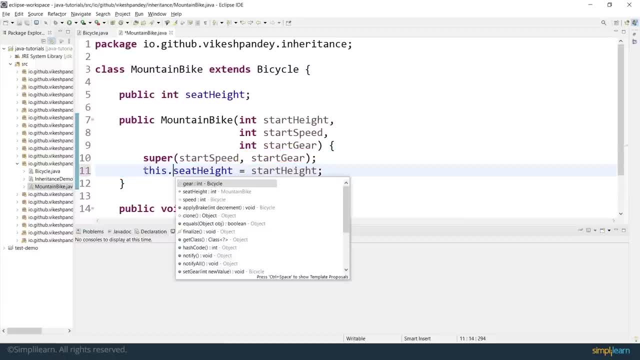 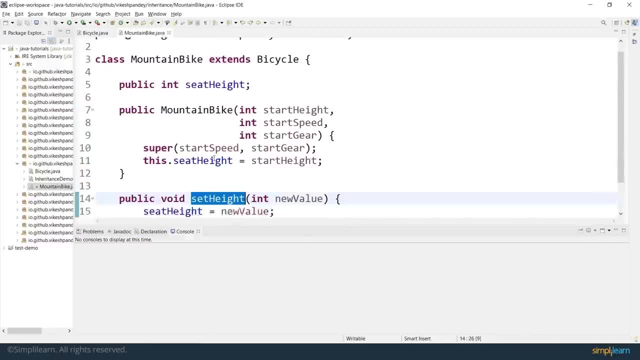 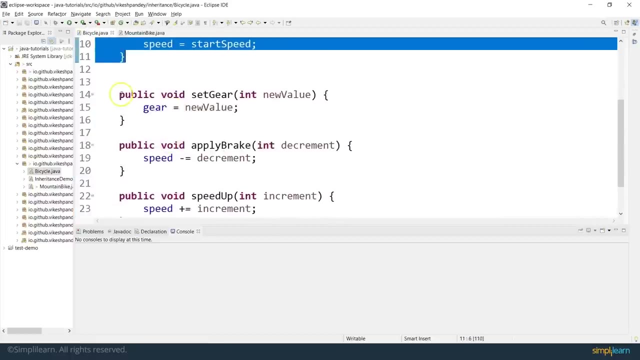 variable. i should call this as this, remember i we discussed about this in this in the classes session, okay, and then it just has a method of set height. so there's no extra method which this mountain bike is providing, but this mountain bike will have access to all the methods which have been provided. 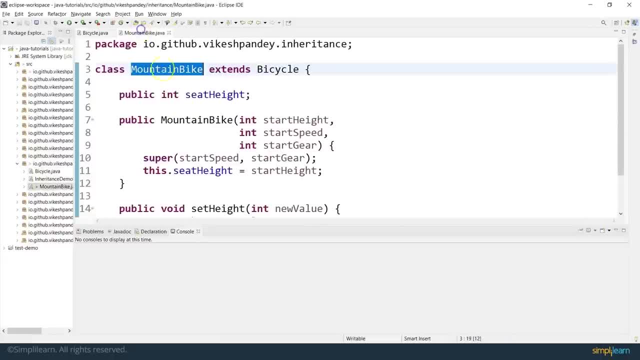 here and all the properties which have been provided here. this mountain bike can access everything from the bicycle class and that's the whole idea of inheritance: that the child class can access the properties of the base class by extending the base class. now let's look at how do. 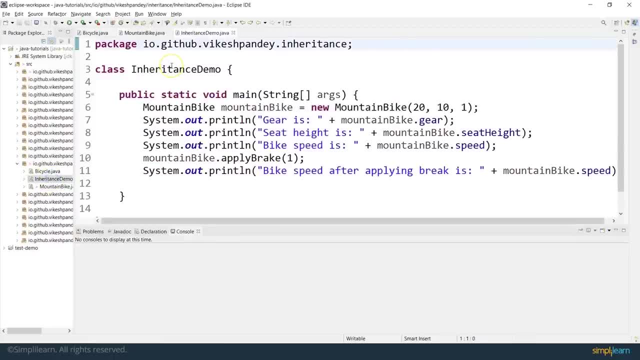 we invoke this particular class. so for that i have a set height method and i have a set height method and i have a simple class name as inheritance demo, which has a public static point main method, and then i am initializing the mountain bike class. i'm supplying three values as 20, 10 and 1. 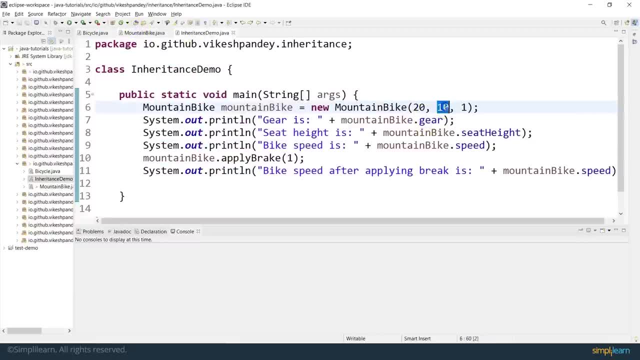 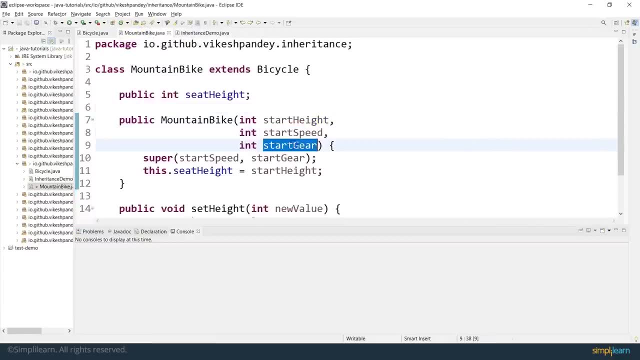 so the 20 goes to start height, the 10 here goes to start speed and one here goes to gear or the start gear, and that's how i'm setting the values. so when i call this particular constructor here the mountain bike constructor, i'm going to call this constructor here the mountain bike constructor. 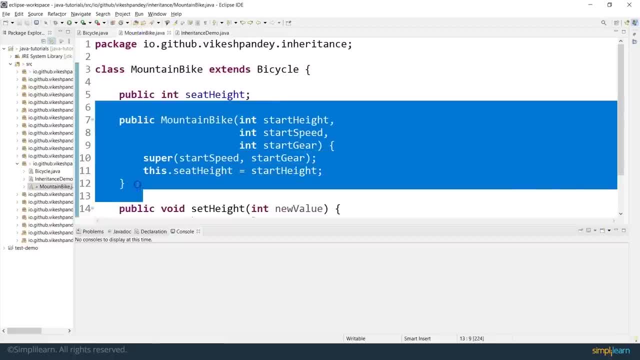 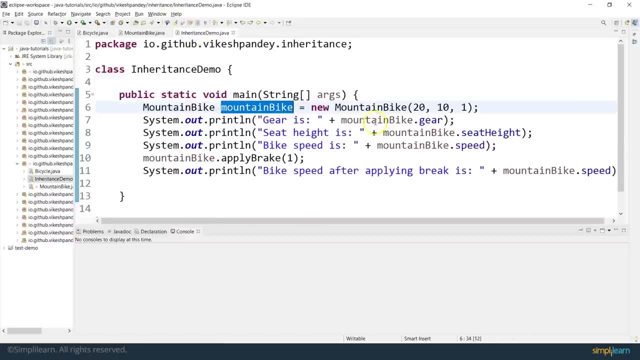 is going to this mountain bike constructor is going to get called, and which in turn, is going to call the base class bicycle class constructor as well, and everything will be set accordingly. and then let's try to access the gear property. remember, gear is not directly available in the 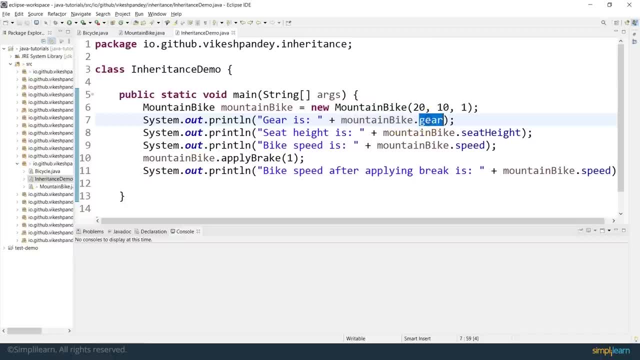 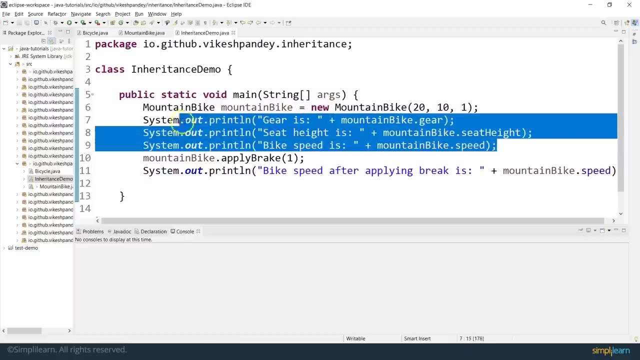 mountain bike class, but i'm still able to do mountain bike dot gear because child class can access the parents class properties. similarly, the same thing goes for speed as well, and seat height is the local property of this particular class mountain bike, so it will anyways be accessible, so i can access all the properties of the base class and the child class itself. 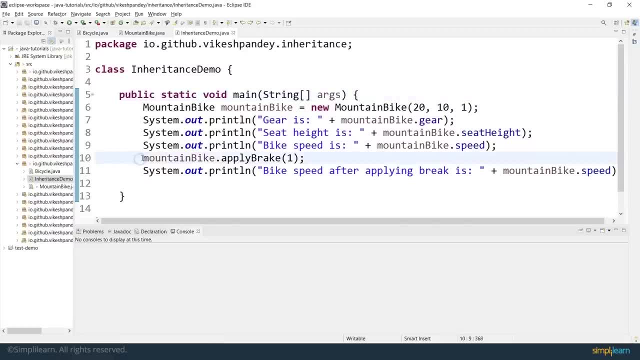 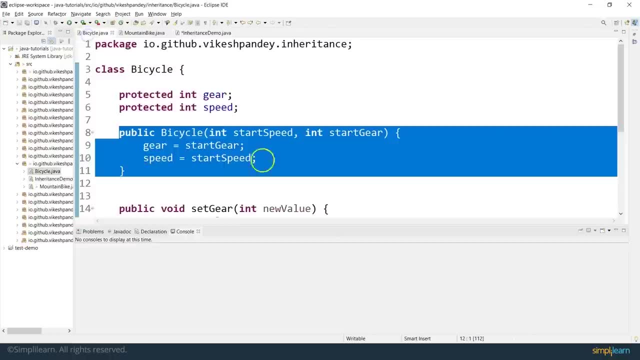 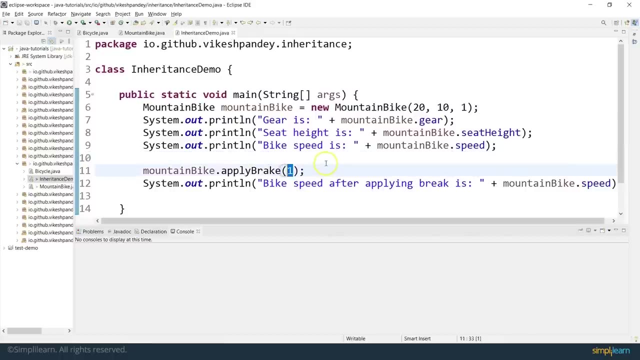 seamlessly, without any differentiation. now let's try to call a method. so here i'm calling the method apply brake. remember, apply brake was defined in the base class, not in the child class. it's defined here. so i'm calling the apply brake method and i want to reduce the speed, the current speed, by 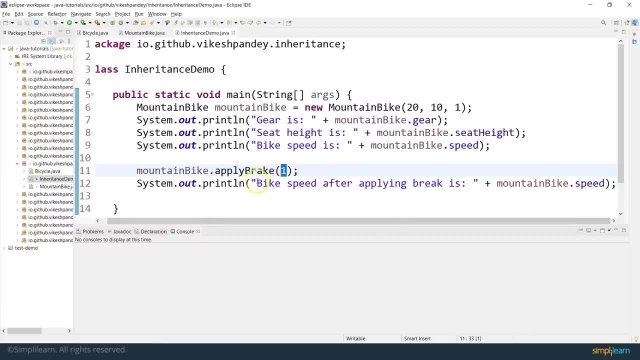 one, and then i'm printing the current speed, saying that bike speed after applying the brake is mountain bike dot speed. so let's run this particular program and observe the outputs. okay, so the the first statement which gets printed is at line number seven, which says: gear is. 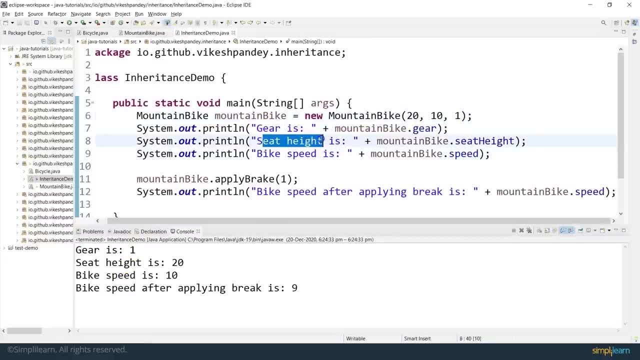 one because it's coming from here. then the seat height is mountain bike dot seat height, which is 20, which is the first argument here, and then the bike speed is 10, which is coming as here and getting printed here. and then, when i apply the break, let's go back to 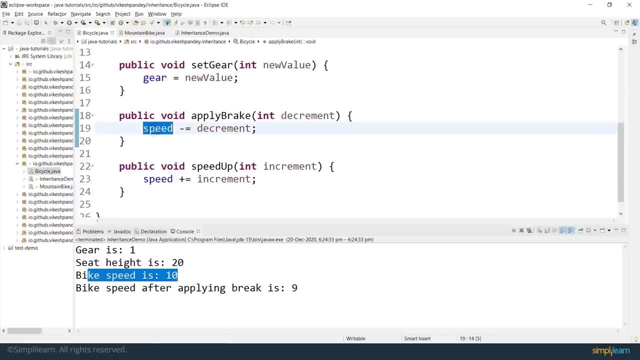 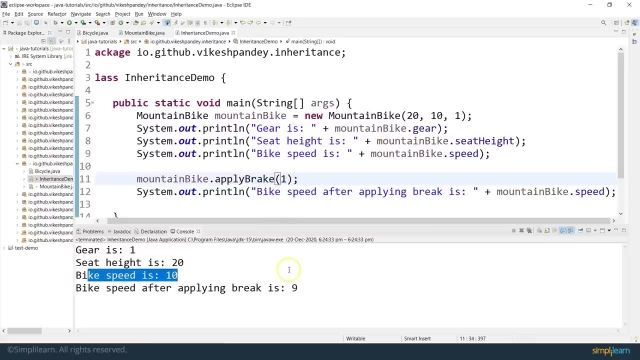 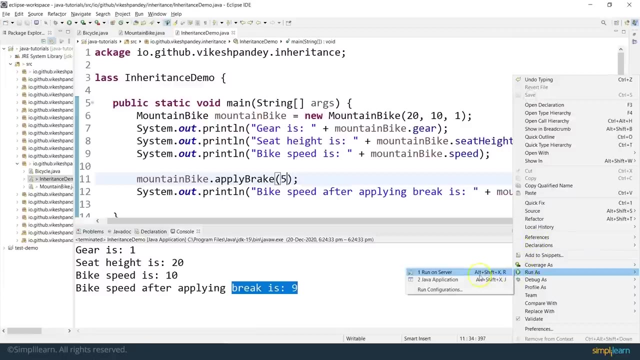 the apply break method. the logic is that whatever is the current speed, reduce it by the value i supply in the method. so if i supply 1, 10 minus 1 becomes 9 and that becomes the current speed. if i supply 5 here, the current speed will be 10 minus 5, equal to 5.. let's assert that particular. 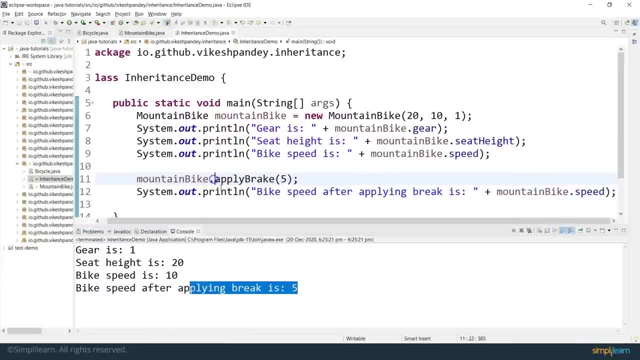 assumption as well. yes, we can see that and similarly you can access other methods of the base class as well, if i just do control space here and you can see: apply. break is accessible. set gear: set height: speed up. all the methods which are defined in the base class are accessible in. 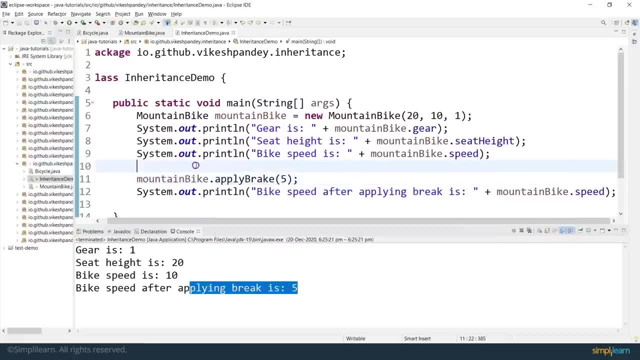 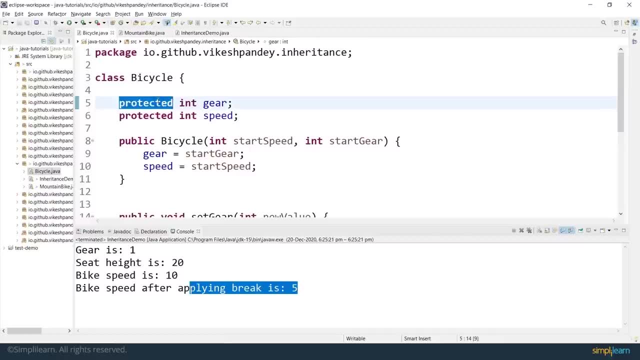 the child class as well. this is the power of inheritance. one more thing which i said i will come back to is around the usage of protected access modifier. remember, when we discussed about the access modifiers in the previous session, i said that protected is used when you are dealing. 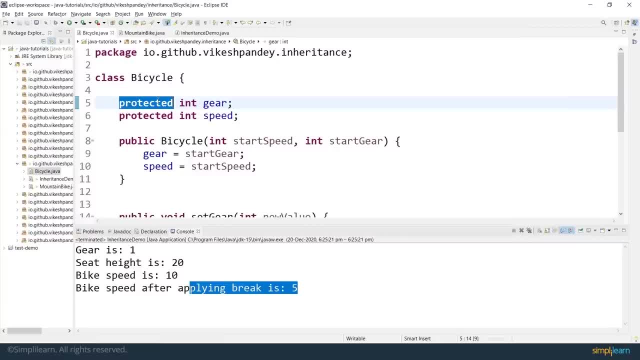 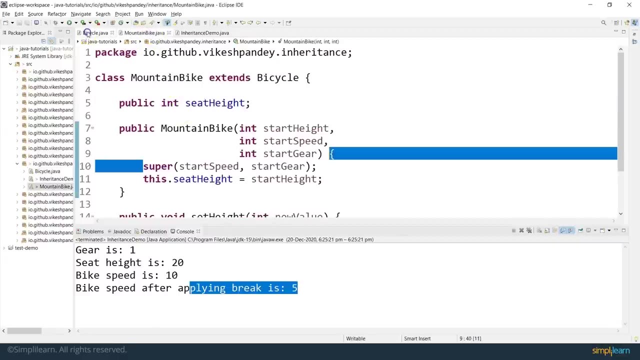 with inheritance that whenever you define something as protected, it will be available to be accessible in the child classes of the base class. so if i define this particular variable as as protected, then this particular property will be accessible in the child class mountain bike as well. let's play around this. let's 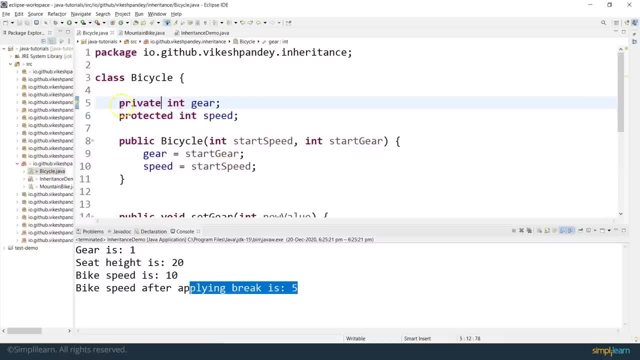 make this as private and see what happens. so if i make this private now, when, when i say private, the scope of this particular variable is within the class only and nobody outside the class will be able to see it and you can see the effect of it, i can see an error being coming here in my 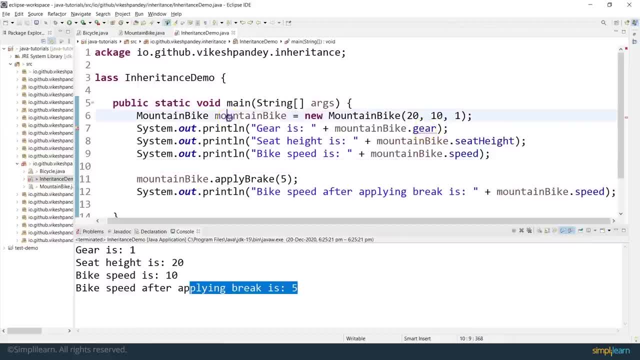 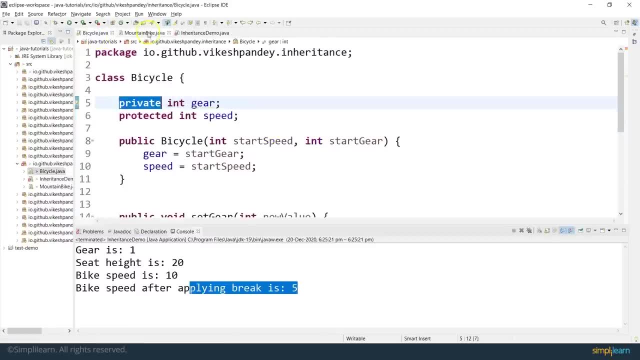 inheritance demo class, because i can't see the effect of it and i can see an error being coming here in my inheritance demo class, because because now mountain bike object cannot access the gear property, because the gear property is defined in the base class and now it is private. that's why the child class now mountain bike class. 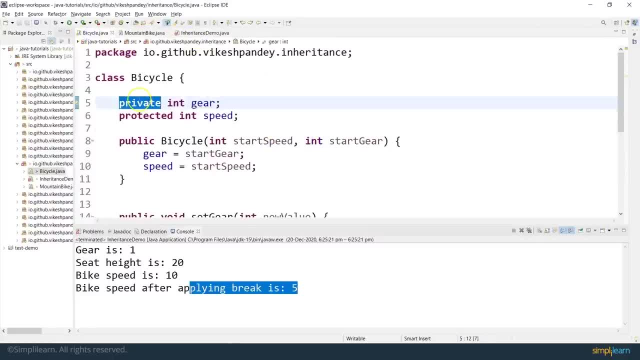 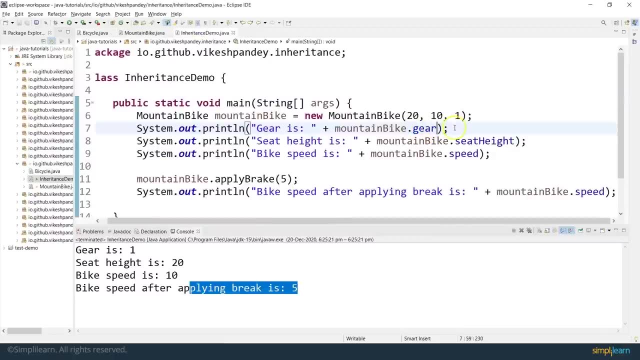 cannot access the property gear and the moment you make make it back to protected, it will be accessible. the error is gone. there's no red line here. so that's how you can. you can use the protected access modifiers. it is always, always recommended to use them when you, when you write any kind of 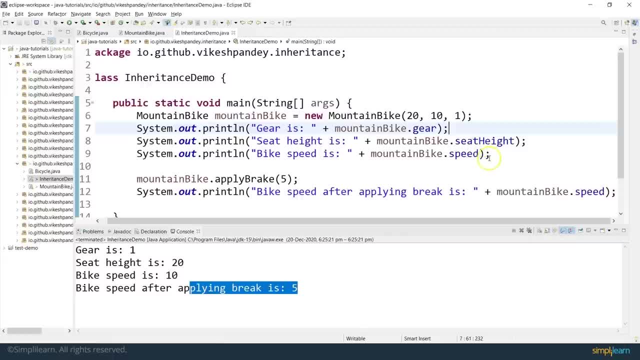 property and in inheritance logic as well. intentionally, if you want to hide a particular property from the child classes, just make it private. and that's all i want to cover. in this particular session, where we dive deep into the concept of inheritance, we had a look at an example. 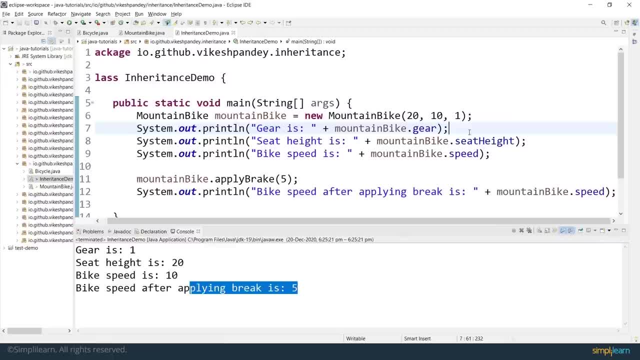 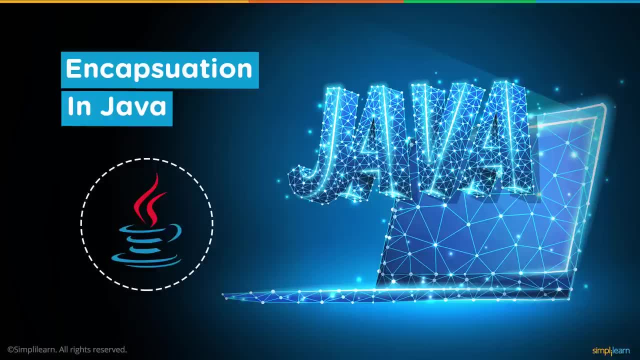 using the bicycle and mountain bike kind of construct and you can apply the same kind of construct on any kind of other other kind of business requirement. remember that is a relationship. let's get started with encapsulation. so again, let's understand what is encapsulation in general and then we will apply that concept to java encapsulation, if you try to break that word. 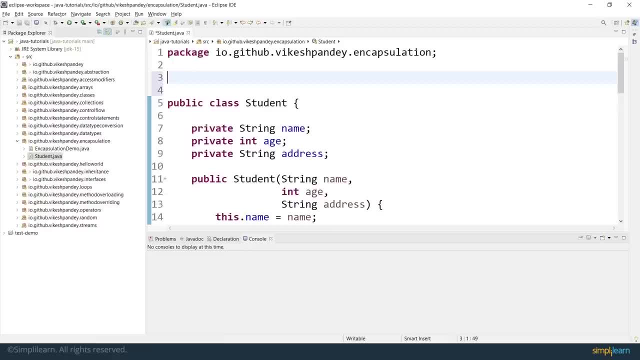 if i just write it here in the form of a comment, it's end encapsulation, just trying to break this word into to make it more visual. so you see, you see a word called capsule here. so if you try to imagine a capsule, why do you create that and what's the concept of a capsule? capsule tries. to pack a lot of things inside of a capsule and you can see what's happening inside this capsule. that's the specific state where they put them inside the CTL reliability model. so you can see inside the CTL reliability model they put all the components in there. they put poo rang C. 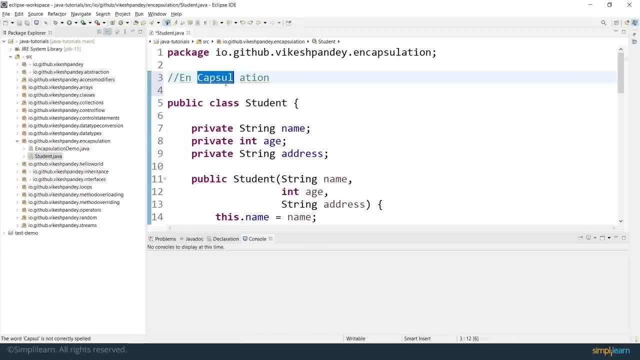 a small tube like shape and the concept of encapsulation is sort of inspired from that. not exactly, not literally, but that's the basic idea of of this root word which is called encapsulation. so encapsulation basically means to restrict accessing the properties of a class to the outside world. if you want to protect the properties of your class, how do you do that? you? 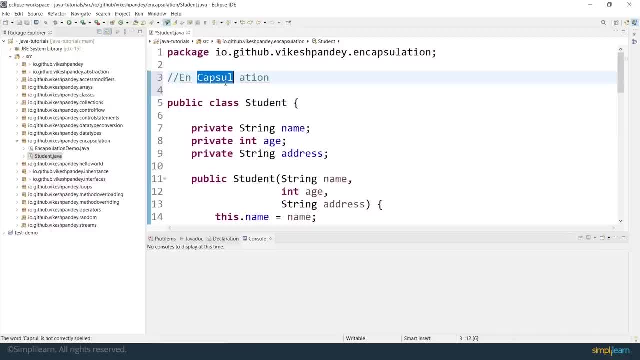 do that with the help of the concept called encapsulation. so here you. this is a sort of a security feature. you can think it of a think of it as a security feature that you want to protect the properties of your class and you will use encapsulation to protect the properties how you. 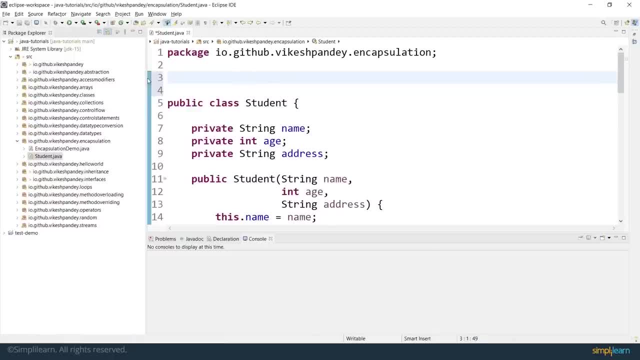 implement encapsulation. let's have a look at that now. so basic idea is to encapsulate the objects, create sort of a capsule around the object which can provide that protection to the class. and you can do that with the help of the concept called encapsulation layer and you will define how the outside world is going to access the properties of the class. 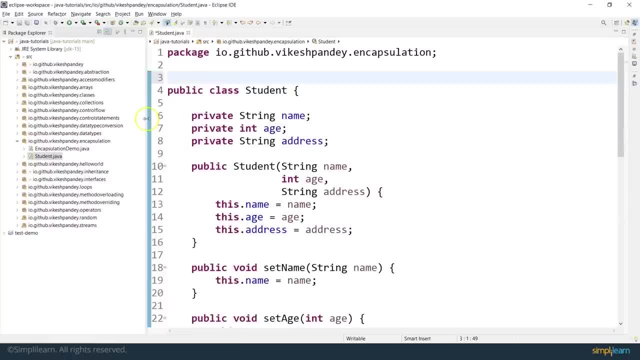 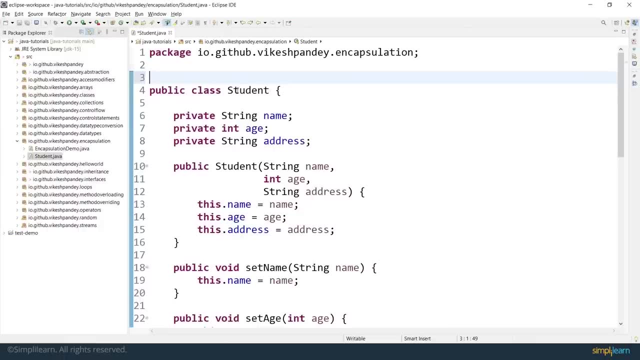 if needed. so i've created a simple class here and it's if you, if you remember one of the previous examples, when we discussed about classes, i used the same class, which was the student class, and i'm just using the same class for continuity. so i've created a student class here and i have 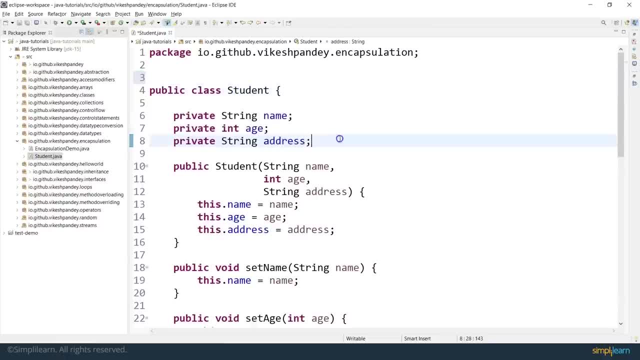 created three different properties of this particular class, which is name, name of the student and the class name of the class and the class name of the class and the class name of the student, age of the student and address of the student. you see, intentionally i have used the. 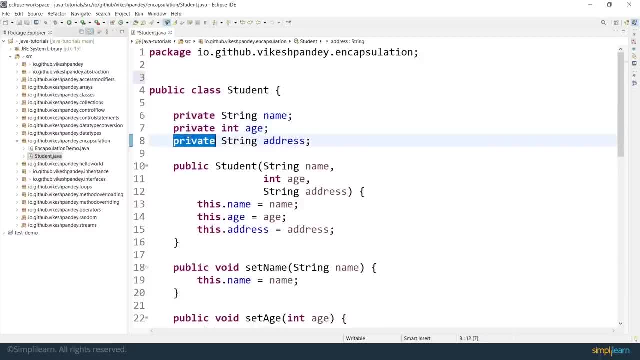 keyword private in front of these three properties. and that is the first thing which you need to do: to implement encapsulation on your object, that you hide all the properties from the outside world. remember, the moment you make anything as private, only the class, which is the student class itself. 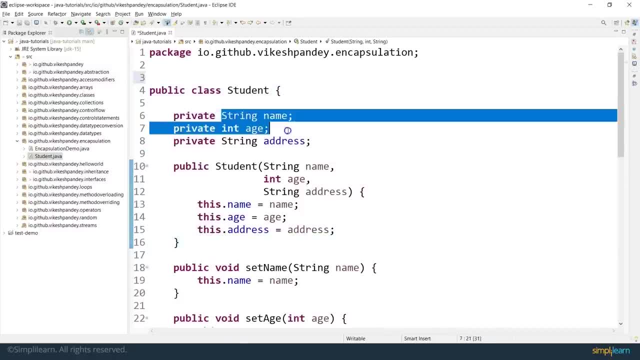 only the class itself can see these variables or these properties. nothing outside the student class will be able to access the name or age or the address directly from the student class. it's not possible. that's the whole idea of making it private, because you don't want the outside world to access these properties, so you make those 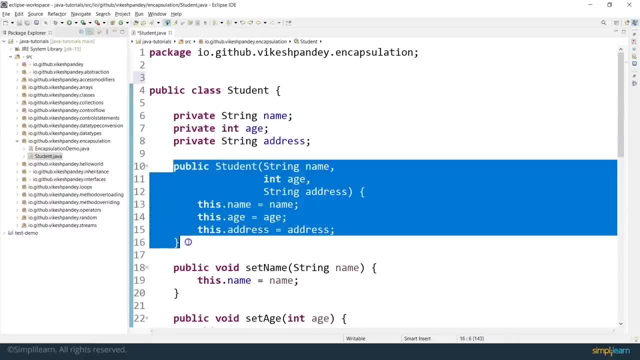 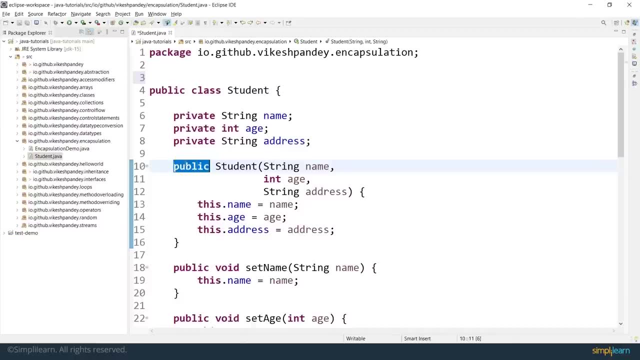 properties as private. then you create a constructor. the constructor has to be public so that anybody can initialize the student object, because you want your object to be accessible, remember. so you want the objects to be accessible, but you want the restriction on the access of the properties of the object. and these are the. 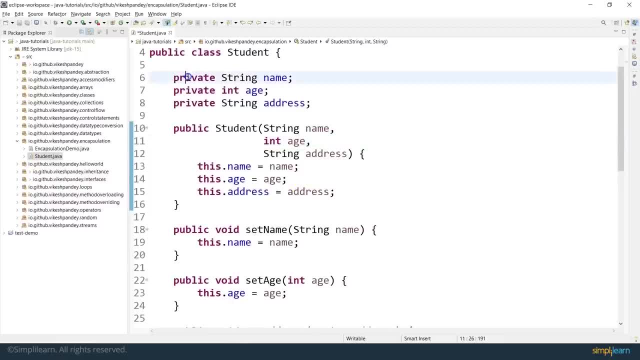 properties of the object. so you have restricted them by making it private. but that doesn't solve the problem, because there will be some illegitimate consumers of the student object which should not have access to the student properties, but there will also be some legitimate consumers of the 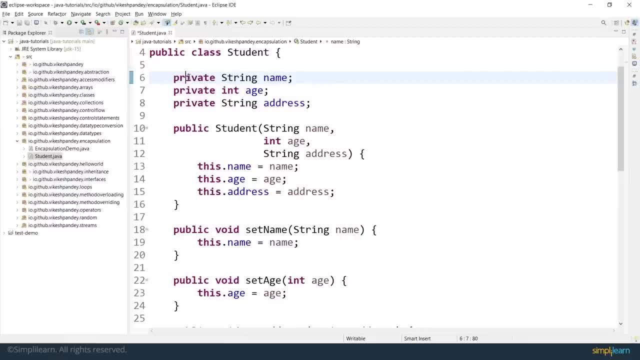 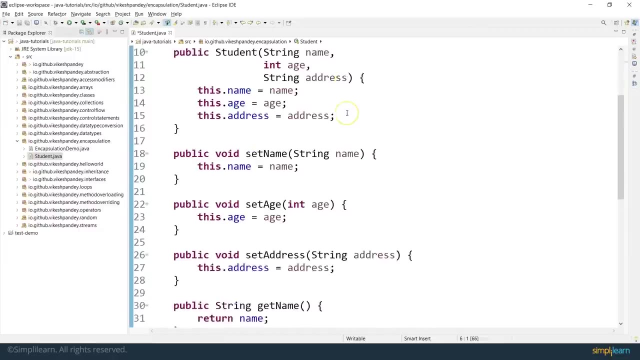 student object, which should be having access to the properties of the student object. for example, the payrolls application will need access to these particular properties. the examination application will require access to these particular properties. so how do you do that? you create getters. we call them getters because they 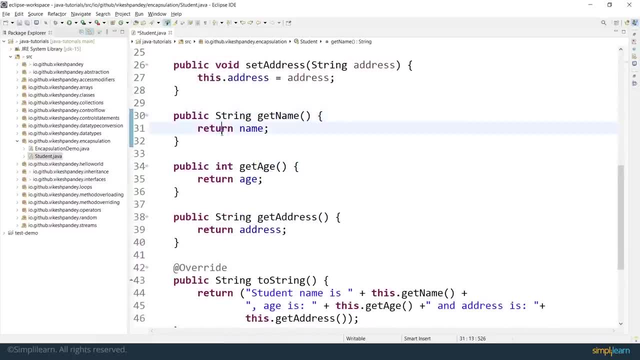 start with the keyword get. so you create a getter method. for each of the property you create the method called as get name, and this is the naming convention with java promotes that you write get and then you write the name of the property, in camel case. so you write get name and this: 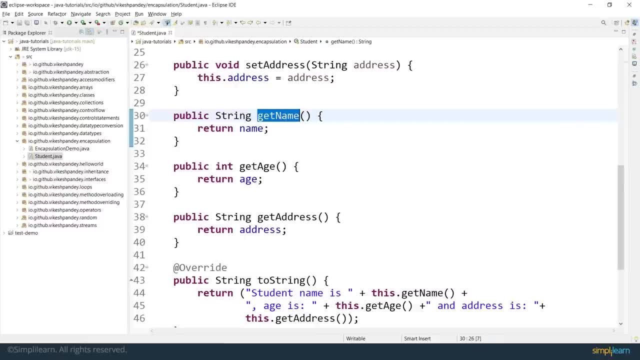 property is supposed to return the name property of this particular object. and you here, you say return name, so you are returning the, the name which is being stored by the current student object. whenever somebody calls student object, dot get name. and this is the way you have restricted. 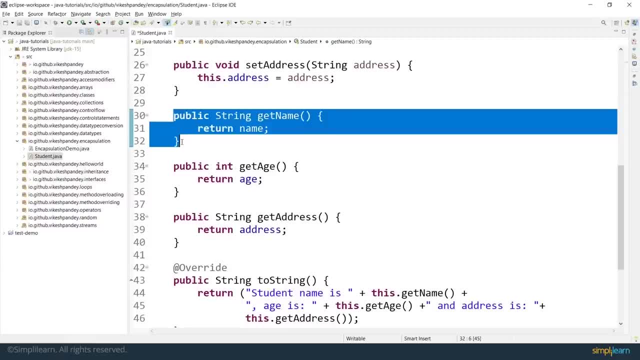 the access of this particular object as well. so remember, you made it private so that nobody can access it, and then you defined your own way of providing access to the name property of this particular class. now, if anybody wants to access the name value of your student object, 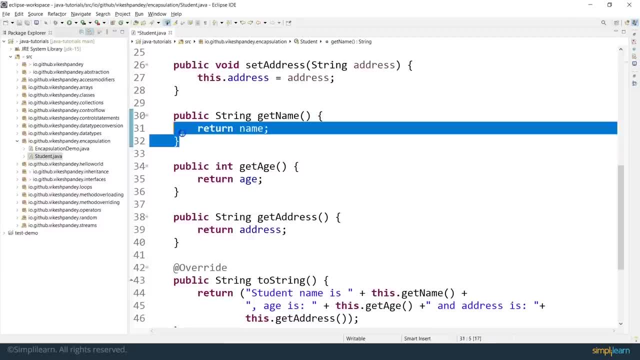 there's only one and one way to do that, which is via calling get name. so you have provided restrictions and you have also provided prescriptive guidance on how you are going to expose the properties of your class. that's the second uh thing which you need to do to. 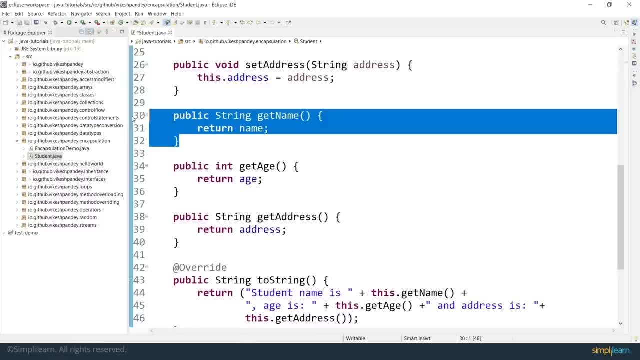 implement correct form of encapsulation on your object, that, that is, to provide the getter methods with the right visibility. you want to make them public so that anybody can call them, but since you are governing, which is what is written inside the method- you have full control on what kind of exposure you want to give for this particular property. similarly, you create a getter. 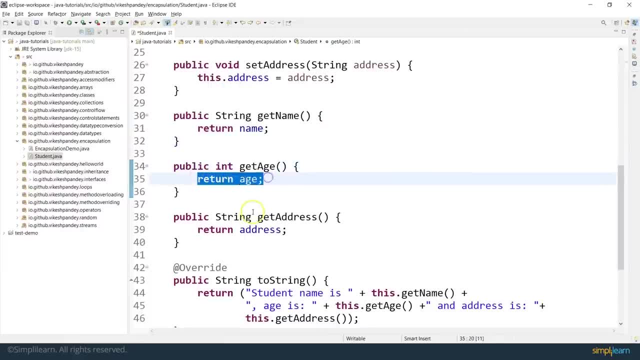 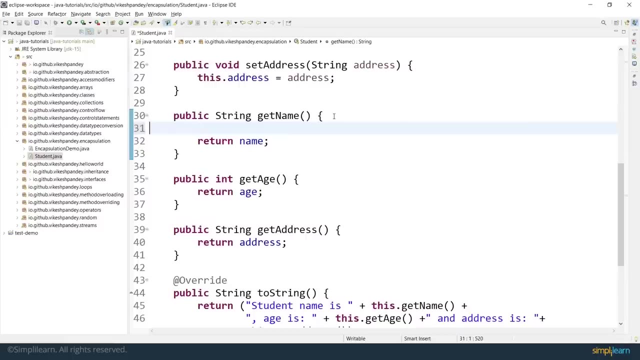 for age, calling get age, which returns the age, and then you call get ad, you write get address and return the address. here it is simply returning it, but if you want to do more stuff here, feel free to do that. like i said, you govern the control of how do you want to return the name. maybe you don't. 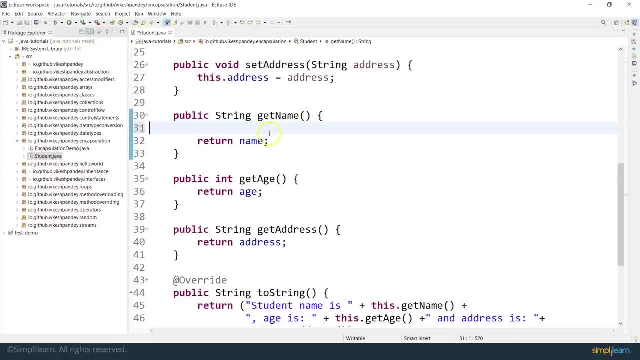 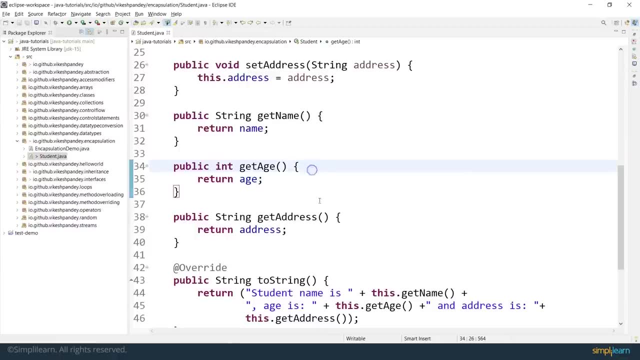 want to return the complete name and you want to just return the initials, then you can split the string, trim the string and return only the initials. so that's the basic idea of getters. now, after you have created the object, there might be use cases where somebody needs to overwrite. 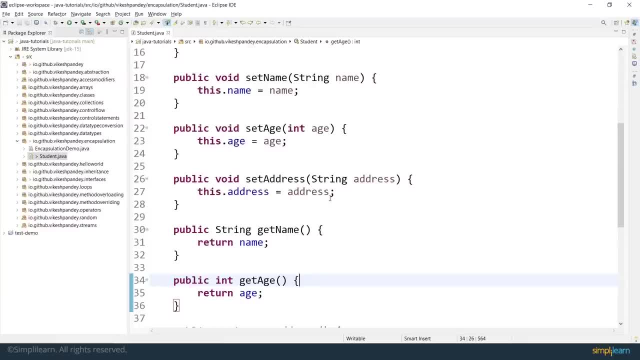 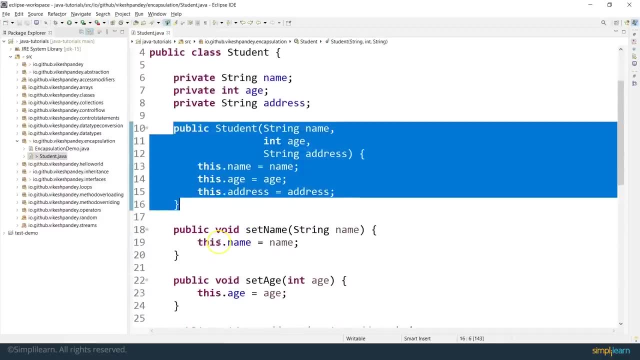 the values of the getter, so you can create a getter for each of these objects and then you can use the properties like name, age or address. what if a student's name was incorrectly mentioned when they called the constructor and now they want to overwrite the name or fix the name? so 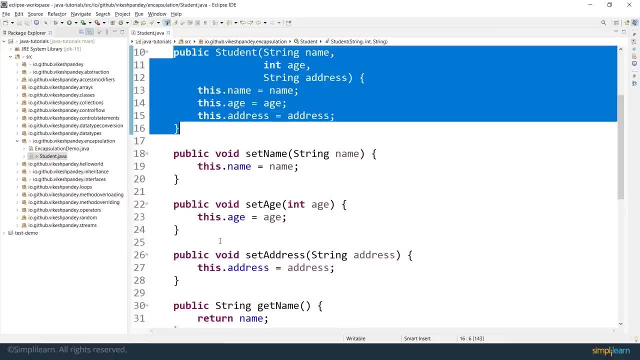 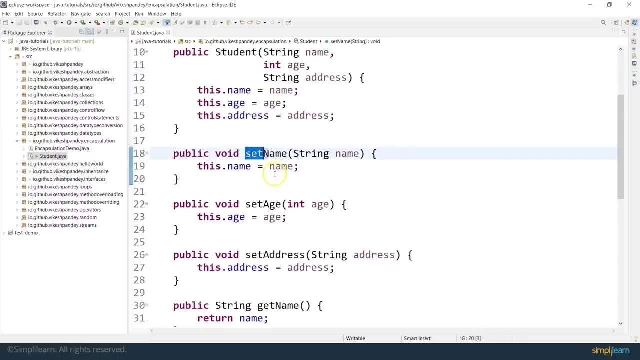 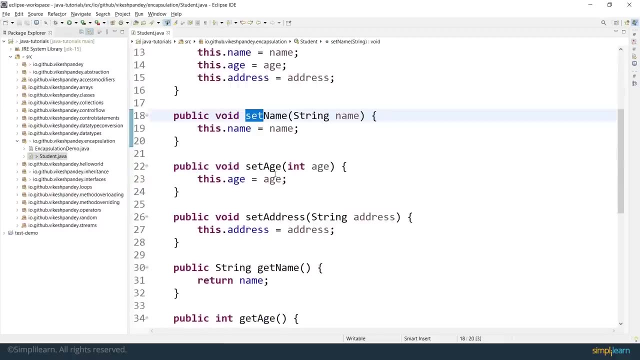 basically, they have to replace the existing value of the name with a new name. so in that case you need to provide what we call as setters, and they start with set. that's why we call them setters and we follow the same kind of logic that you provide the setters for all the properties of your class. 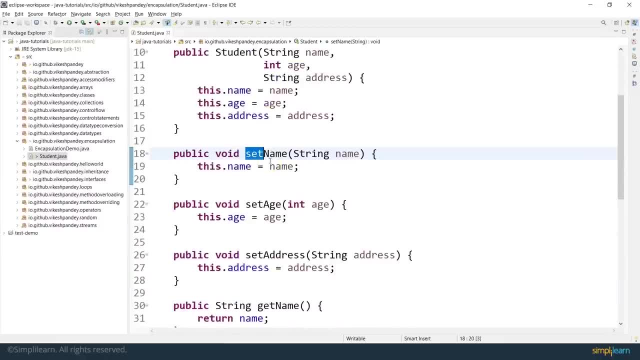 so you had three properties, which were name, age and address, and you provided the setters for all three of them, and how do you provide that you write? you again, make them as public because you want the outside world to access this setter method to overwrite the values of the name. 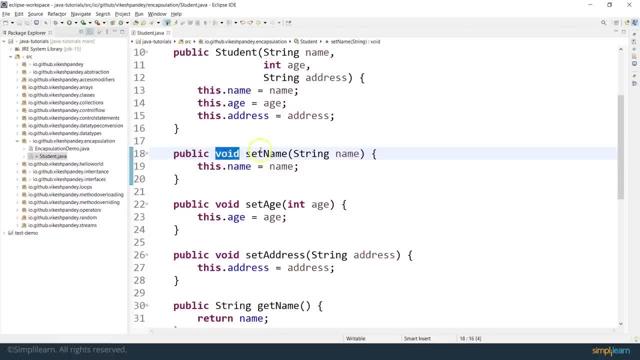 this method is not going to return anything, so it is going to be void. then you write the name of the method which starts with set, and then the property name, in camel case, and then you provide the new value, which is the value which should be, which should be the new. 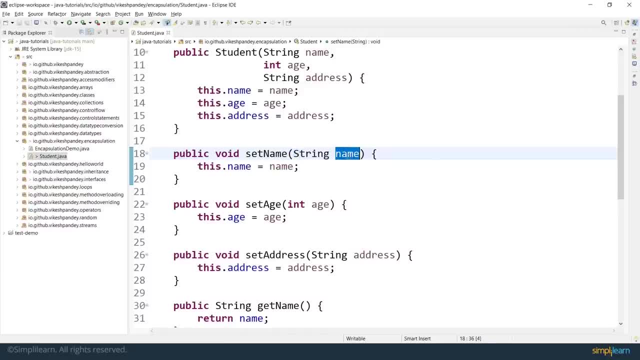 value, and this is the value which should replace the existing value. so whatever new value you want to supply, you supply that as the argument of the setter methods for set name, for set age or for set address, and then you write this particular line which says: set the current. 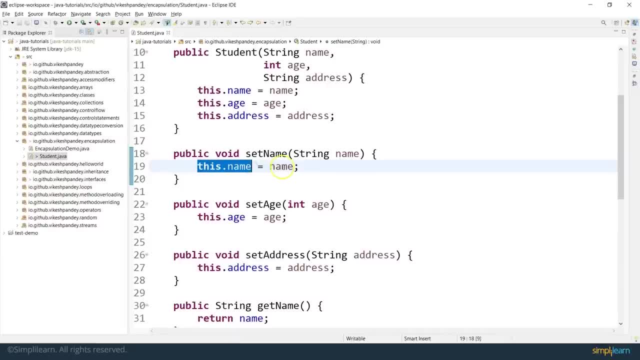 name property of this particular object with the name which is coming in from the argument. so this dot name- remember this dot name- represents the current object's property because this represents the current object. so whatever is the current object property value of the name is just overwrite that value. with the argument coming in, do the 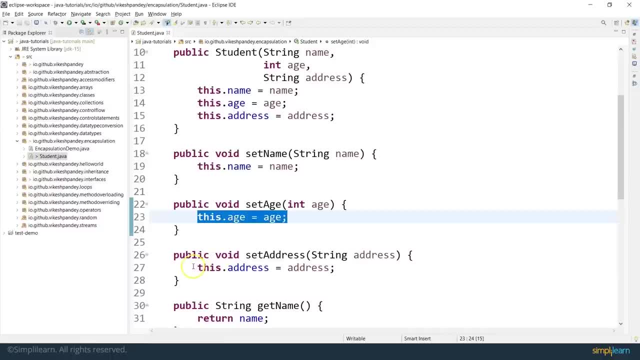 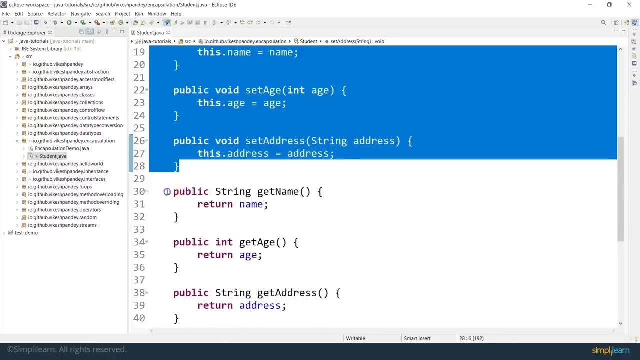 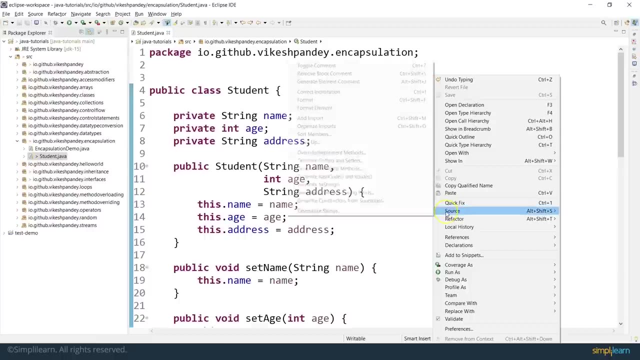 same thing for age in set age method and do the same thing for set address in the in the set address method. so this is how you are going to provide the setters and the getters. so setters and getters can also be generated in smart ids like like eclipse. so you just right click, you go. 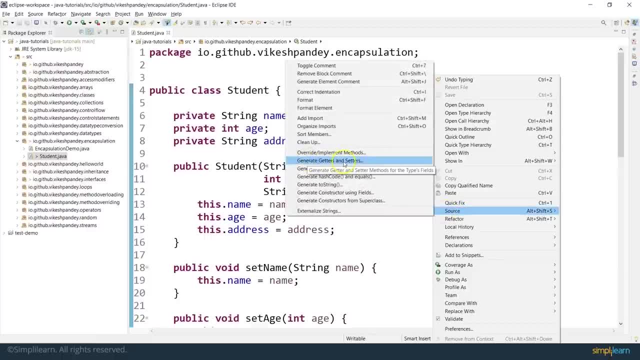 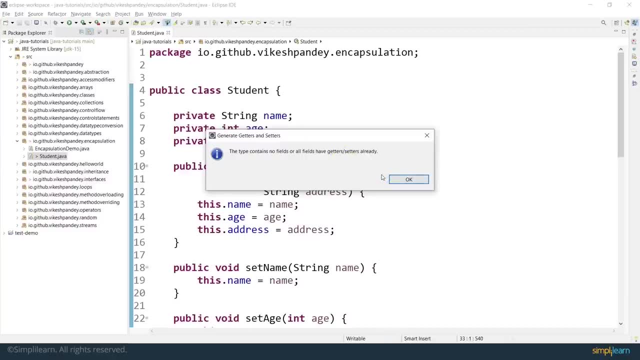 to source and here you will see the option of generate getters and setters. if you click on this, it will give you the list of the fields which are available to be had to be having getters and setters currently. it says no fields or all fields have getters and setters already. yes, because they. 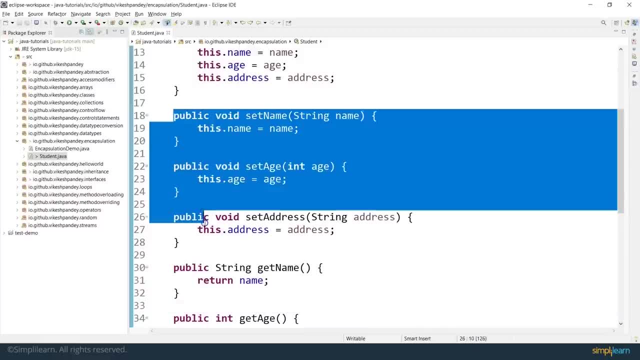 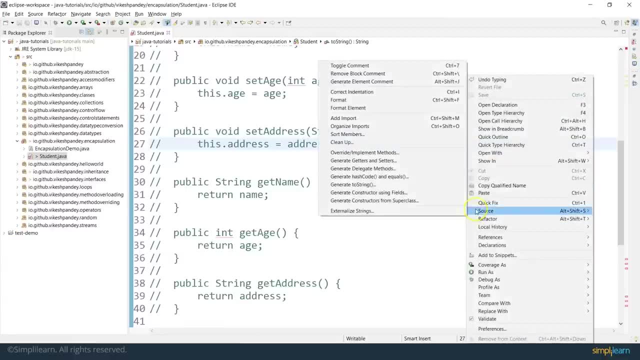 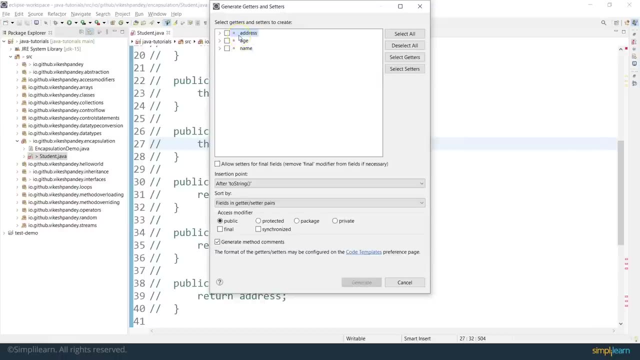 have it. let me just comment this and show this how this work. so, for example, let me comment all the getters and setters, so i'm commenting them, and if i right click source, generate getters and setters, i get all the fields available for which setters and getters can be generated, so you can select them. 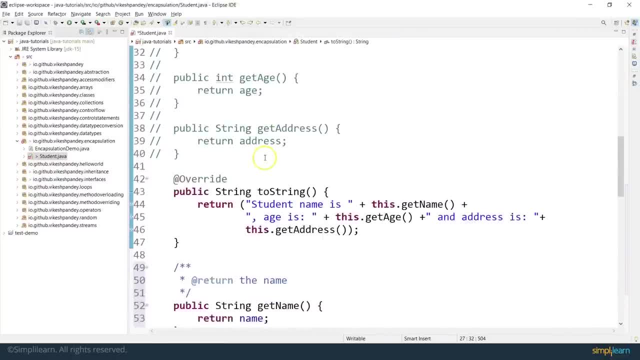 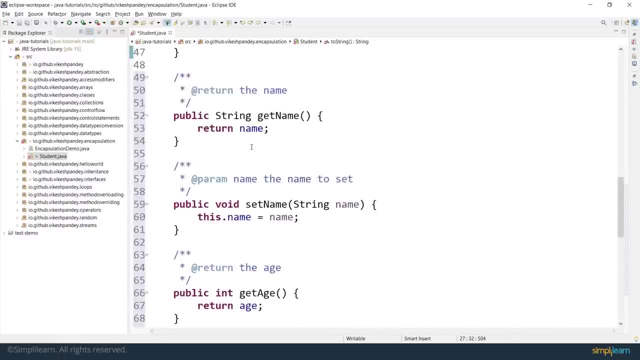 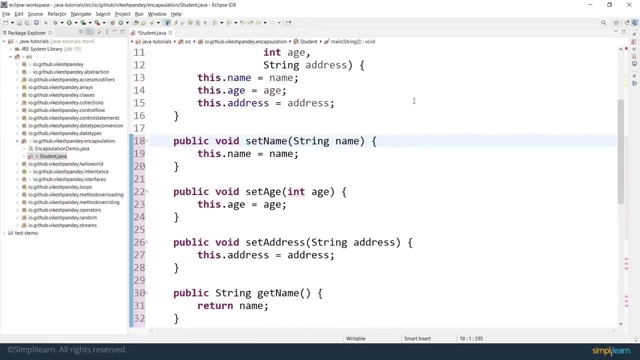 and leave everything as default. it generate, and it is automatically going to generate the getters and the setter. you see, all the code of the getter and setter is automatically generated, you don't even need to write it, and this is the power of the smart ids. let me just, uh, revert what i did, so. 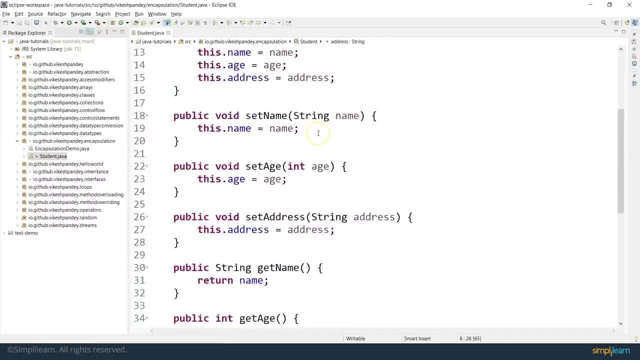 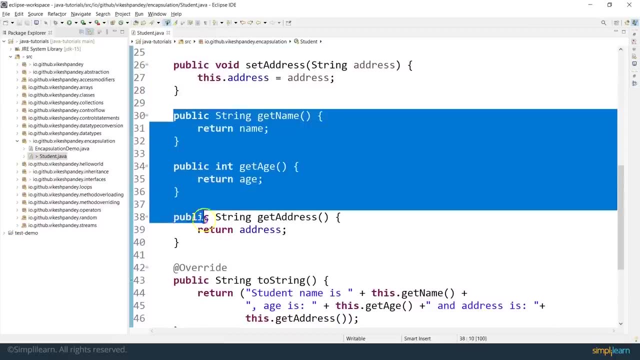 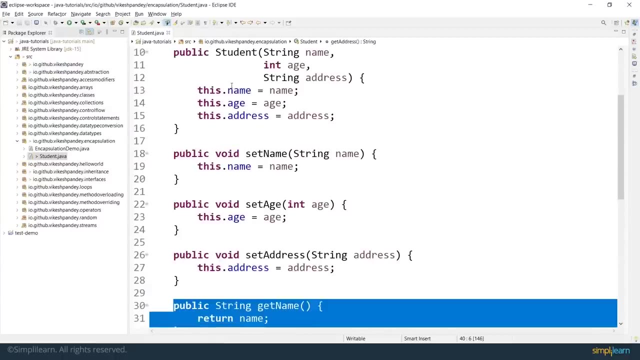 you created everything as all the properties as private. you define how you want to replace the values by providing the setters and you define how you want the outside world to access your properties. so you have full control of the class now you you control the visibility, you control how they are going to get initialized. 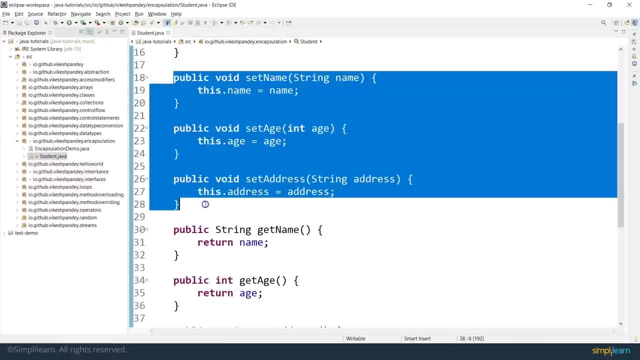 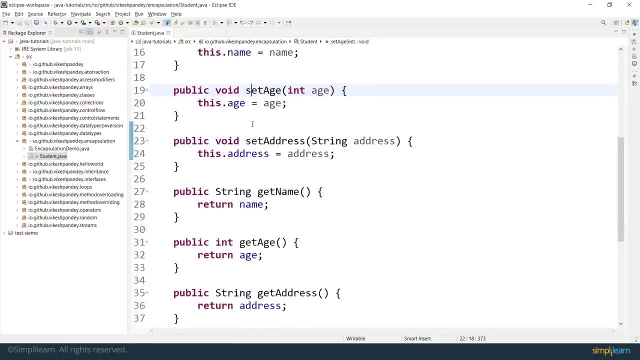 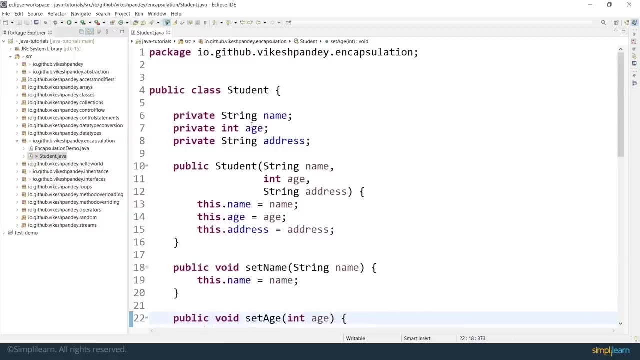 you. you are controlling how the properties are going to be overwritten or set and you control how the properties are going to be returned, so you have complete control of the class. so you have created a perfect capsule here, a perfect form of encapsulation in this class, and this is how you can implement encapsulation. let's get started with abstraction. 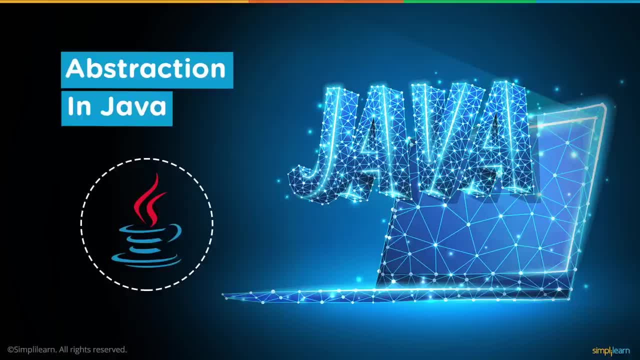 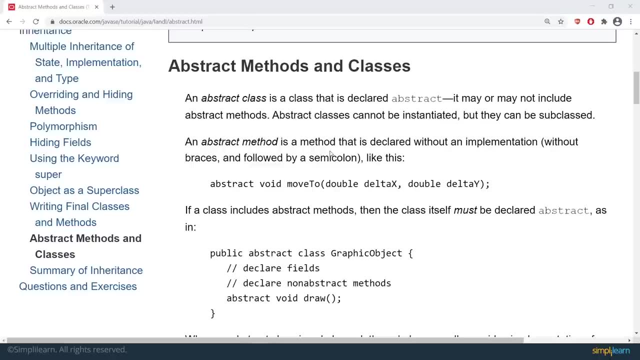 let's first understand the definition of abstraction before we relate this to java. abstraction generally means hiding something. when you want to hide some details of of a particular object from the outside world, you apply the concept of abstraction. for example, when you drive a particular car. you just hit the accelerator and the car speeds up. 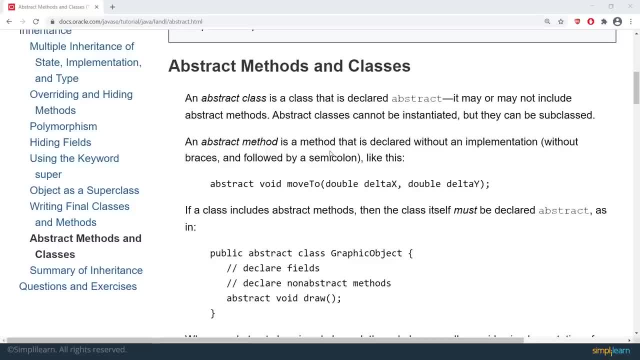 now, it's not only one action. when you hit the accelerator, the whole machinery of the car and all the components, different parts of the car work together to speed up. there would be engine, there would be propulsion, there would be fuel, there would be- there might be some if it's an electric. 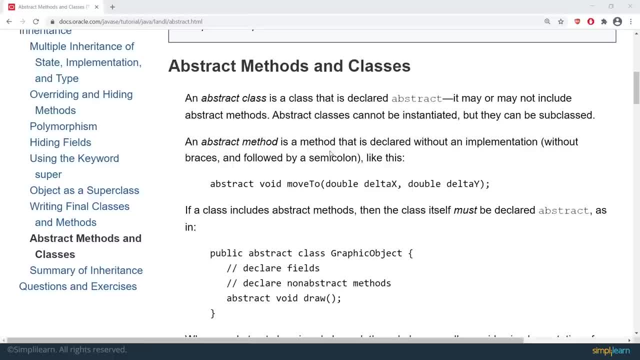 car. they would batteries, uh, there would be whole different kinds of pistons and plugs which will make the car speed up. it's not only a single component, it's a lot of different components under the hood, and that's the concept of abstraction that we only show. 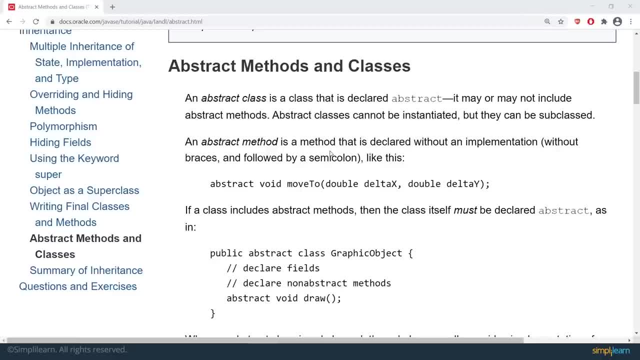 the relevant parts to the user and we hide all the internal details from the user. that's the basic idea of abstraction. so a car manufacturer abstracts away all the inner technical details from the driver and just gives the driver a single pedal to speed up the car. for a user it's a very good experience because he doesn't need. 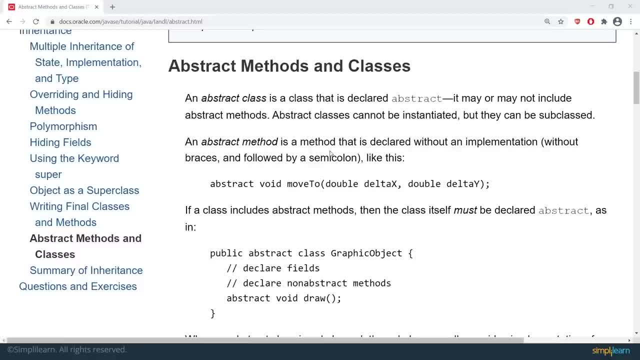 to know about all the internals of the car, but the car manufacturer can hide all the details and provide a very simple interface for the driver to interact with a gas pedal. and that's the basic idea of abstraction. and we try to apply the same kind of concept to Java in the form of abstraction, and Java provides this kind. 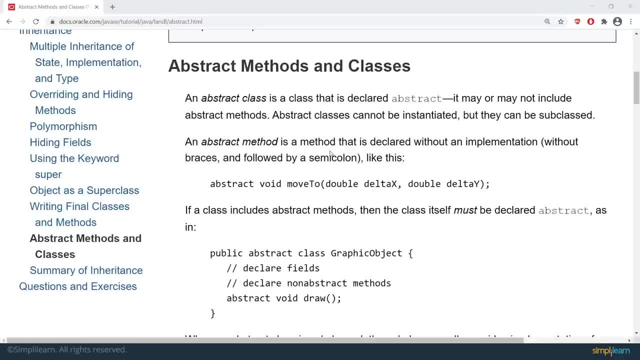 of concept implementation with the help of a keyword which is called abstract. now, abstract is a keyword which can be used in front of a class or a method. when you use it in front of a class, the whole class becomes abstract. abstract class is a type of class, so the class itself becomes an abstract class. one of 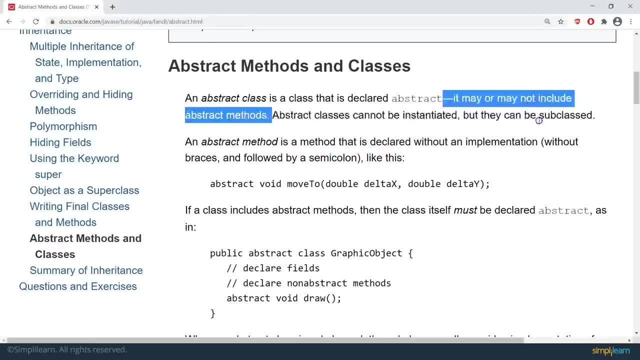 the things to remember is that abstract class cannot be instantiated but can be subclassed. remember we talked about the concept of subclass and the parent class when we talked about inheritance. so if you make a class as abstract class, you cannot call the constructor of the class because you cannot instantiate it. but 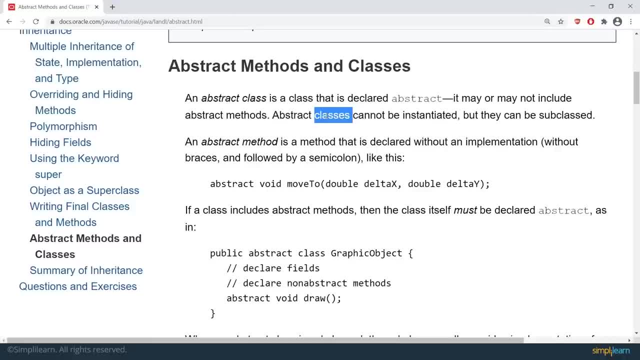 you can extend the abstract class and create a child class class out of it. that's the concept of abstract class. another concept is abstract method. you can also use the abstract keyword in front of a method, and when you use abstract keyword in front of a method, then that method is only declared without an implementation. you are not. 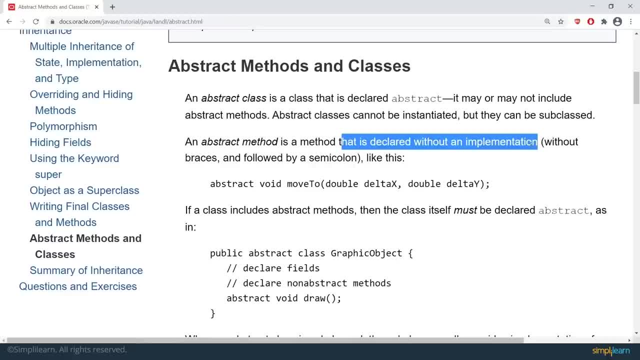 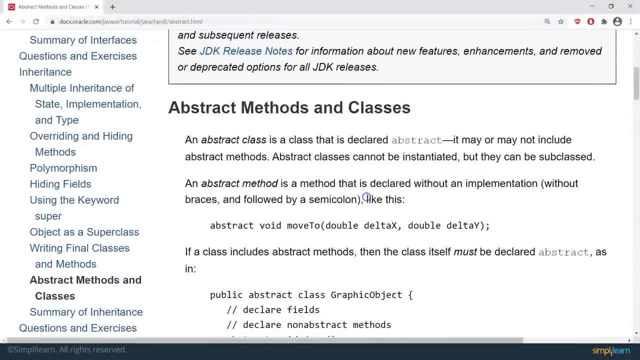 going to provide any implementation of the method and you're just going to declare the method, something like this. we will see a similar example in the in the hands-on as well, but that's the basic idea: that you just declare the method. you are not providing an implementation as to what does move to. 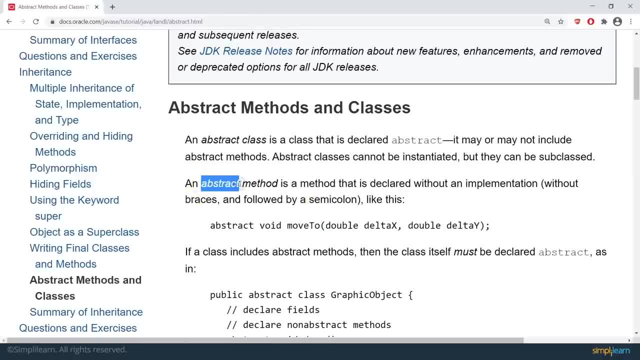 method actually does, because that's the whole concept of abstraction and it is the responsibility of the child classes which inherit the particular class in which the abstract method would be sitting, so that child class will be having the responsibility to provide a concrete implementation of the declared method. let's understand this better with the help of an example. so here I have. 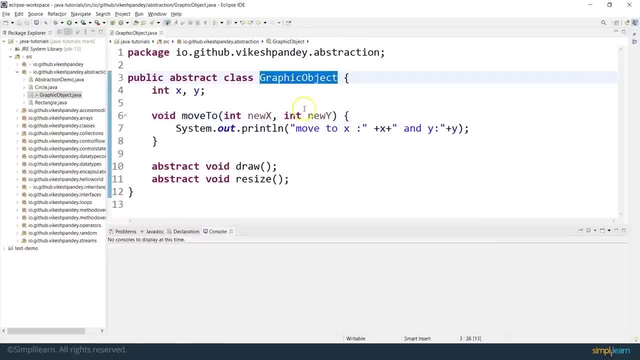 created a class called graphic object and I have made the class as abstract class. this is the keyword which you need to use in front before the class keyword and the class becomes an abstract class. now, when you create an abstract class, it automatically gets some properties. the first property is that this particular 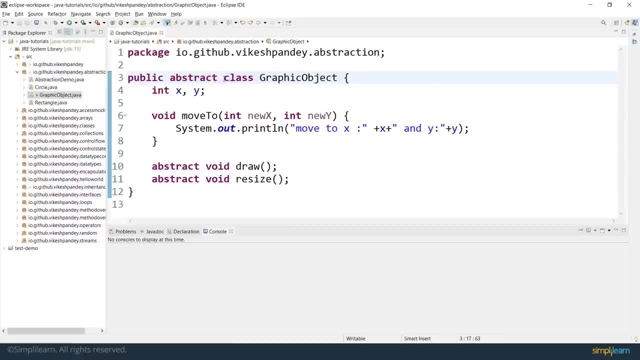 class must have at least one abstract method. and this is how you define the abstract methods, where you just provide the declaration but you do not provide the implementation of the draw method or the resize method. and the way you will create the abstract methods is by using the abstract keyword and the abstract. 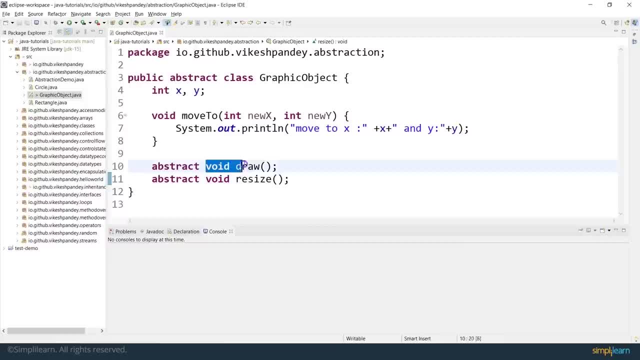 method before the actual method declaration starts. so general method declaration would look like this, and if you use abstract in front of it, this becomes an abstract method declaration. abstract class can also have concrete methods. so that is the Liberty which abstract class gives you: that you can have abstract methods which are just declared, but you can also have normal. 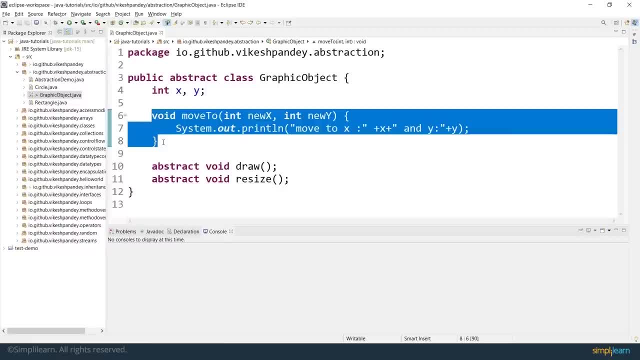 methods, which are which where you can also provide the implementation. so you can have normal methods and a stack methods as well in an abstract class. Now, if you want to explain this, select abstract methods and start the declaration here. so this is the abstract class. now, if, if you want to provide an implementation of the draw and 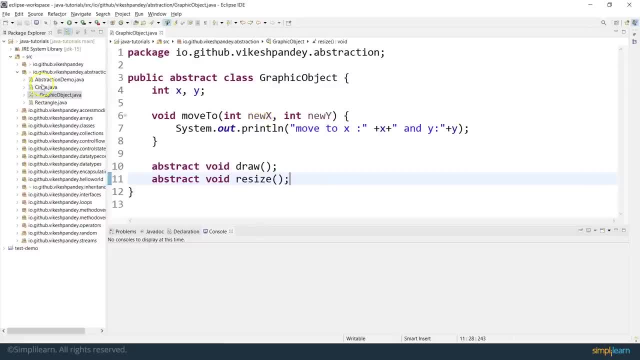 resize method, you have to extend this abstract class. so we extend this abstract class by creating two child classes out of this particular abstract class, which is circlejava, where you can see, i create a normal class and i use the extends keyword for inheritance, and i'm saying that. 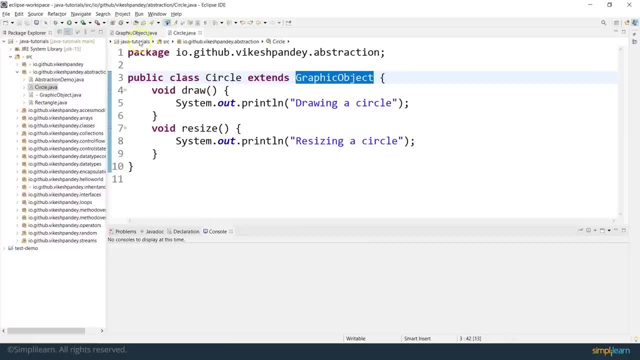 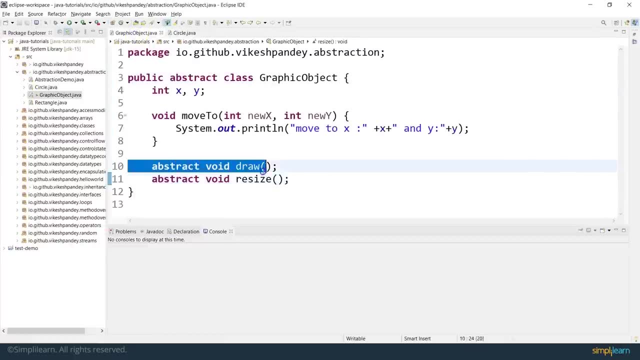 circle class is inheriting from the graphic object class, which was my abstract class, and once i use this extends keyword, then i have the responsibility of providing the implementation of the abstract methods. actually, java will force me to provide the implementation of these two methods if i do not provide all the declared methods. so there are two declared methods here. 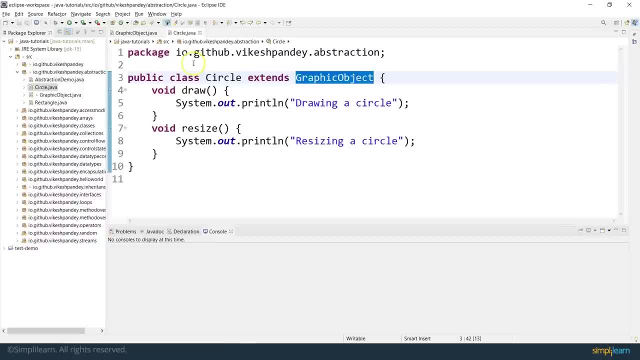 so if the circle class does not provide that- the implementation for both draw and resize methods- then java will throw an error and it will ask you to take an action, which can be either define all the methods, meaning provide implementation for all the methods- or make the circle class itself as abstract. let's see: if i just comment this particular out, i get an error. 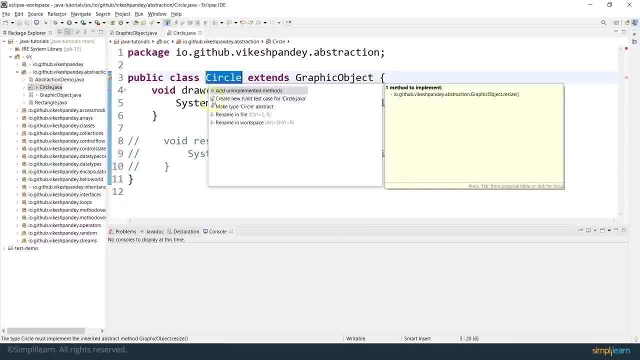 you see a red line here and if you click on this particular balloon here it will say: either you can add the unimplemented methods or you can make the circle type as abstracts. these are are the two options which you will get to fix this particular error so an abstract class can. 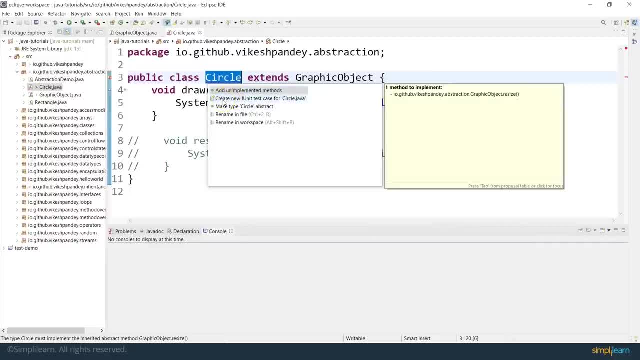 be extended by another abstract class if the child abstract class is not implementing all the methods of the parent. if you want to implement all the methods, then just implement them and keep at. keep it as a normal class, and that's what i've done here. i've just created a normal class here and 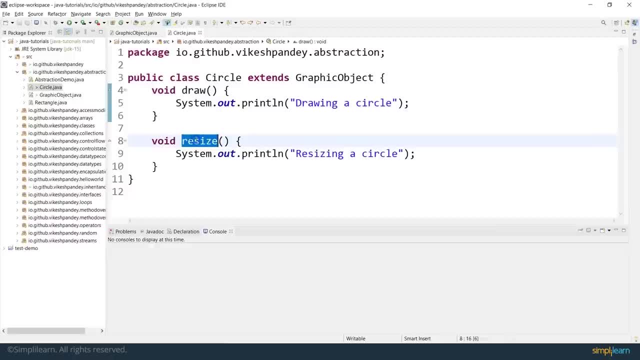 provided the implementation, and once you provide the implementation of both of the methods, the error is gone. similarly, i have also provided another child class because it's uh, there can be, uh, there can be multiple children of a particular parent. so rectangle also extends from the graphic object and it also provides its own implementation of drawing and resize, because generally the way 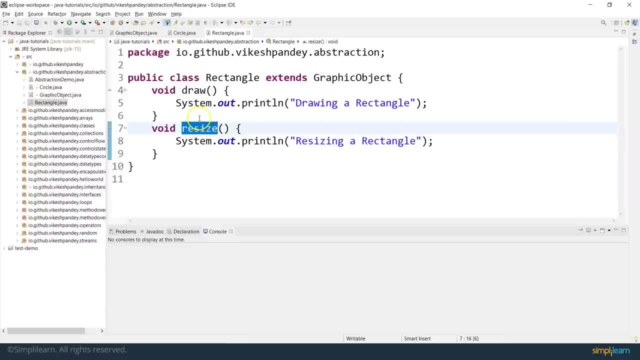 you will draw a rectangle and you resize a rectangle will be different than drawing or resizing a circle. here i'm not doing anything in the methods because this is just to show you the demonstration. i'm just printing a sysout saying drawing a circle and resizing. drawing a rectangle and resizing a rectangle and in the circle class, drawing a. 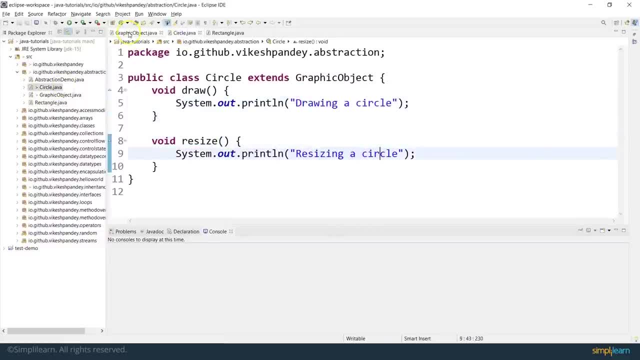 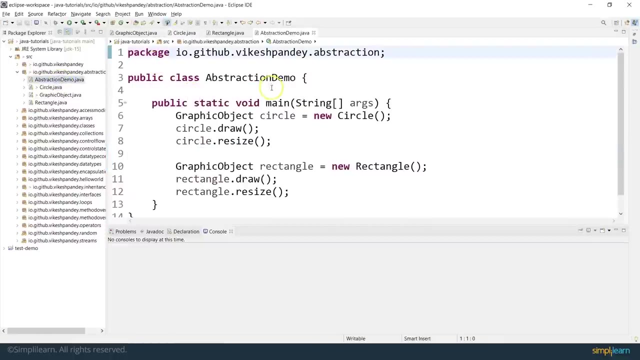 circle and resizing a circle. so one abstract class is the parent class, which is the graphic object, and two children, circle and rectangle, both providing the implementation of the abstract methods which were declared in the base class. now let's go to the main class, where i've defined 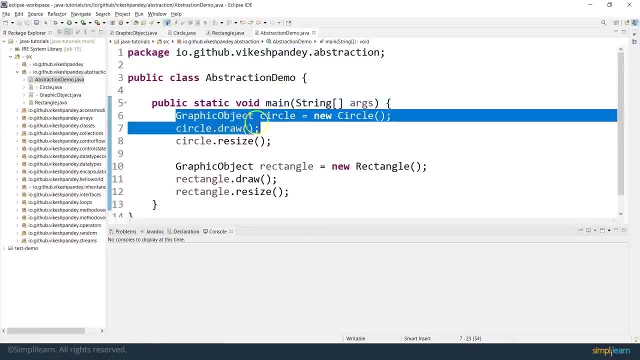 define the public static void main method. and here you see, i have created two different kind of blocks of code here. one block is where i'm saying graphic object, creating a reference of the graphic object named as circle and initializing the circle object. now you see a difference here. here is the. 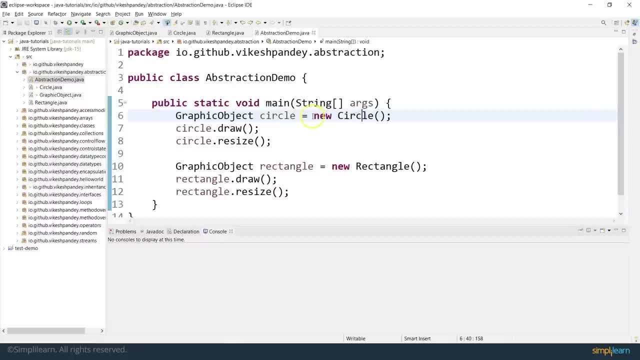 abstract class and here is the concrete class. so whatever you define on the right hand side, whatever is the type of object, will be the type of methods being caught. so if you created a circle object and then if you call the draw method and resize method, these methods will be called from the 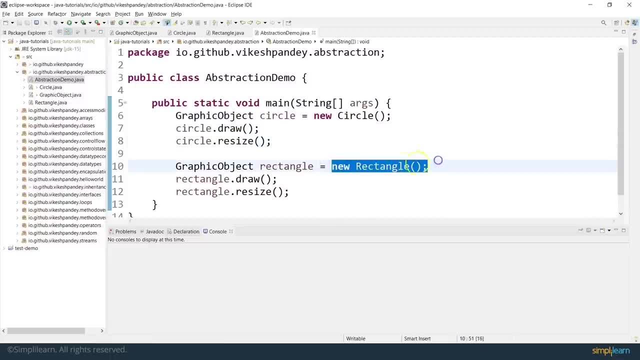 rectangle class. if you initialized it as new rectangle, then you are creating a rectangle class object and then the draw and the resize method will be called from the rectangle class. that's the basic construct and that's how you will initialize a particular class which is using an abstract class. so i i call a graphic object circle new circle and i call circledraw and 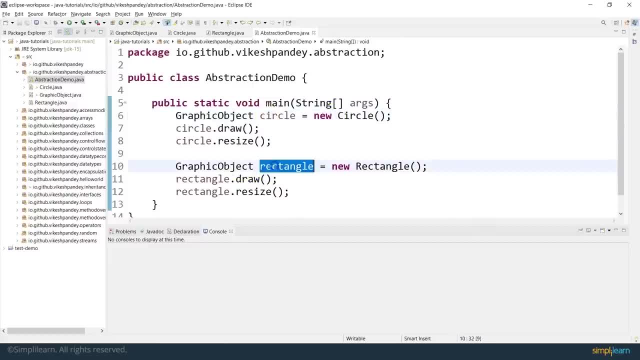 circleresize similarly: graphic object: rectangle equal to new rectangle and rectangleresize: rectangledraw- rectangleresize. let's run this program and observe the output. so when i call this particular block of code, circle object gets initialized and then circledraw method prints drawing a circle and circleresize method prints drawing resizing a circle. similarly, when i create 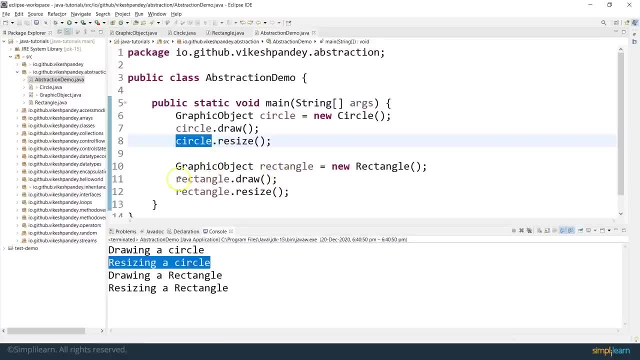 the rectangle class object, referencing it with the graphic object class. rectangledraw prints this particular line drawing a rectangle and rectangleresize prints this particular line which is resizing a rectangle. and this is how you will use the concept of abstraction. there's another very interesting thing, which which is which is going on here. 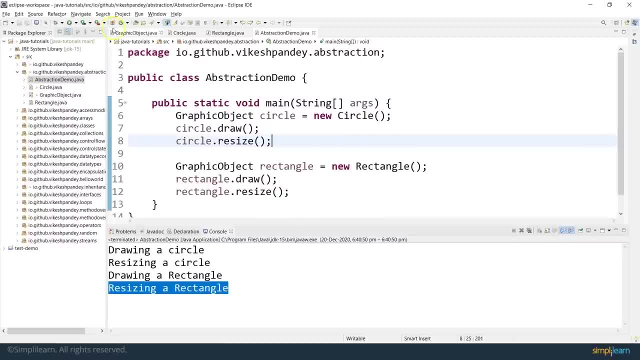 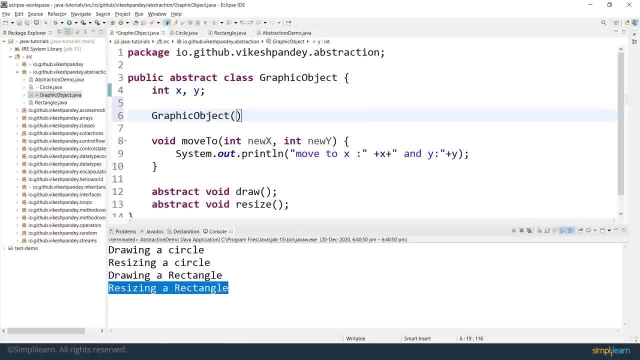 remember i told you that the abstract classes cannot be instantiated. so if i go here and i try to create a constructor of the graphic object class, let's see what happens. if i do this and i i create, i just put a system out here- base abstract class. so if i do this, 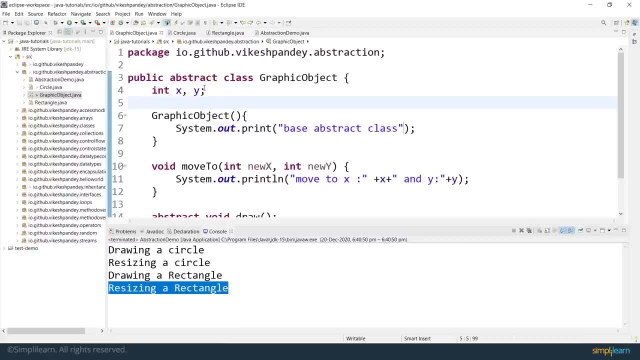 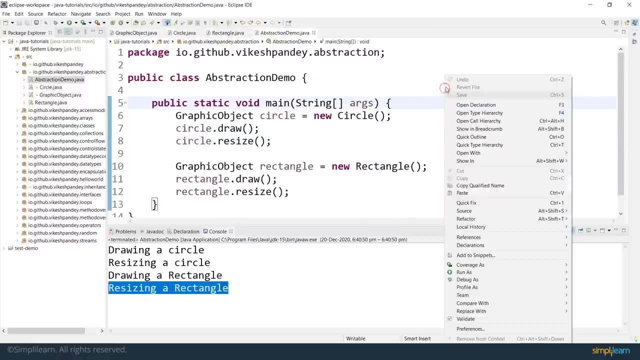 here. if i create, if i still write a constructor- though java says that it cannot be instantiated- if i still write a constructor of it and i do not do any changes here- and if i run this particular program, let's see what happens. you'll see the base abstract class being called here. let me just 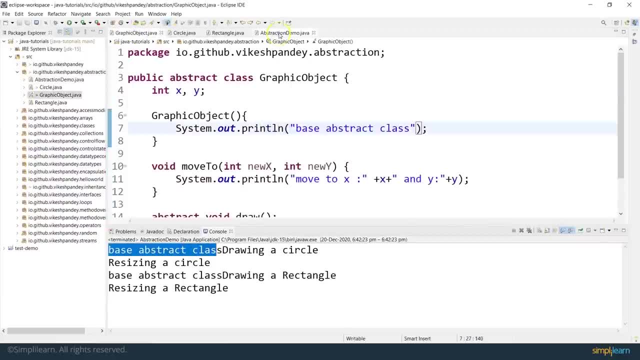 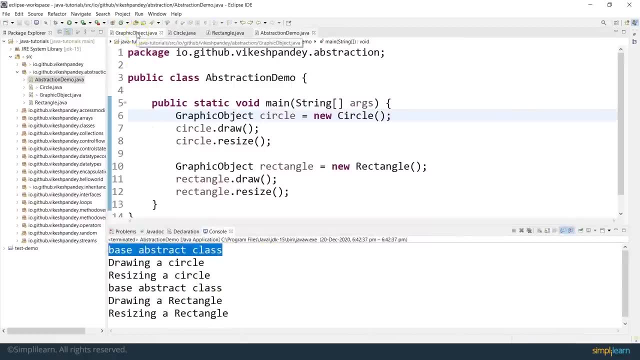 reformat it by putting l n here so that we get a better output. so if i run this particular program, you see base abstract class is getting printed, somehow, though we said that abstract classes cannot be instantiated, but still it will be instantiated. so if i do this here, if i do this, 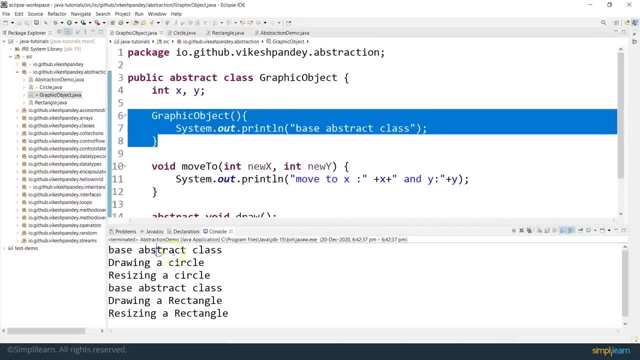 here. if i do this here, it will be instantiated. but still, the constructor of this is still getting called. somehow, when i create a circle class, the base class constructor gets called, and when i create a rectangle class, again, the base class constructor gets called. this is, this is the power. 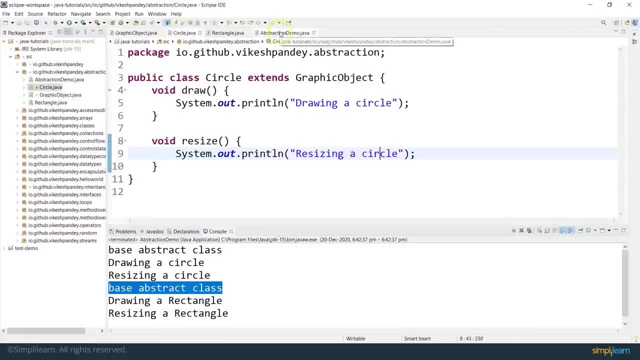 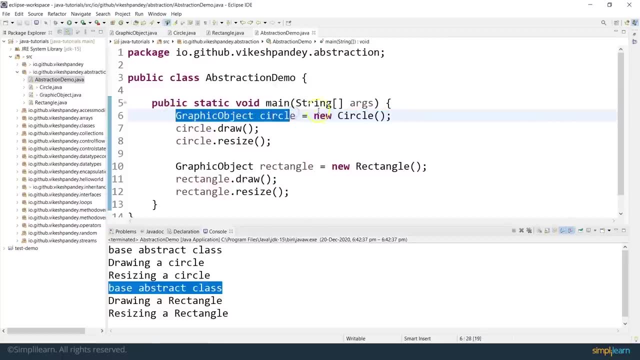 of inheritance, because in inheritance, remember how it works: when you call, when you initialize a particular child object, referencing it with the parent object, see the references of the parent class and the object is of the child class. so whenever you do it like this, first the default constructor, because i'm calling the default constructor here, the default constructor. 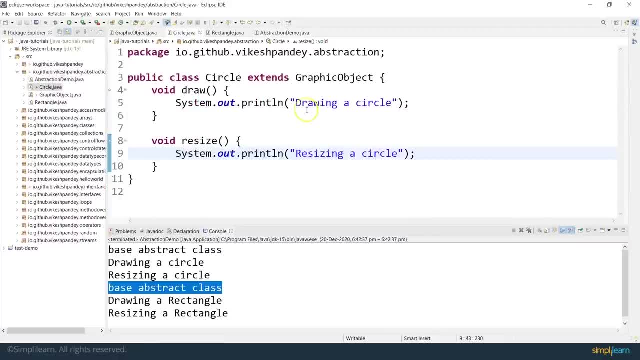 of the circle class will get called, which will go here. remember i told you that java provides the default constructor automatically if you don't provide it. so the default constructor of circle gets called, but java sees that you are writing this code here which says circle extends graphic object. so java is automatically going to call the parent class and going to initialize the. 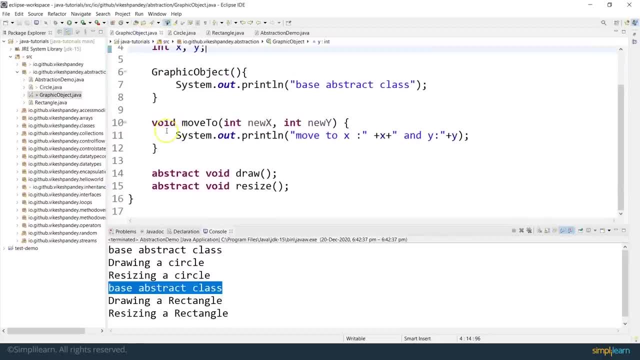 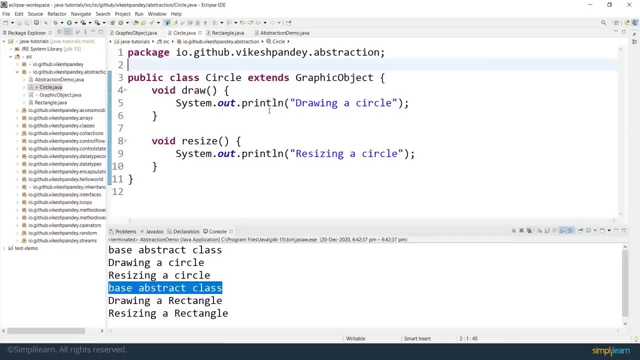 parent class as well, because that's how it will be able to see these methods, and so. so that's why it will automatically call the base class constructor, even if you don't call it explicitly. in fact, you cannot call it explicitly. java will not allow you to initialize the graphic. 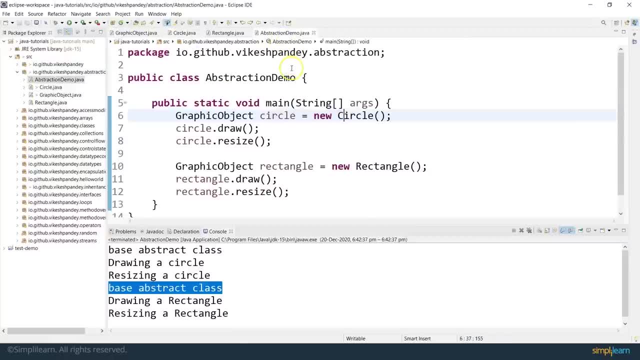 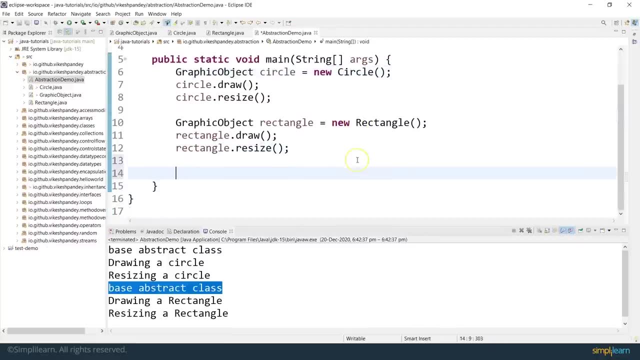 object class explicitly, it can only and only be called by java itself, indirectly, via the concept of inheritance. if you try to do this, let's try to do this for fun and and also for better understanding. so if i write graphic object, go equal to new graphic object. 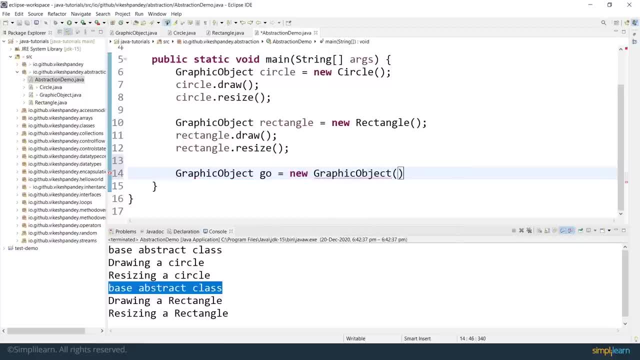 abstract. you see, i don't even get an option, but let's write it and let's see what happens. so you see that this particular it gives basically an error because it's not able to find the constructor of the graphic object class, though even i have defined the default constructor here, but still java is not able to find it, because 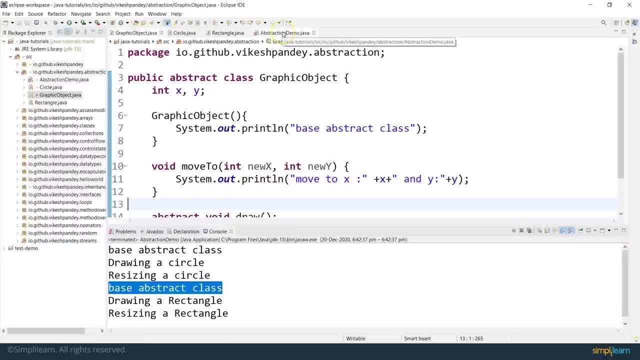 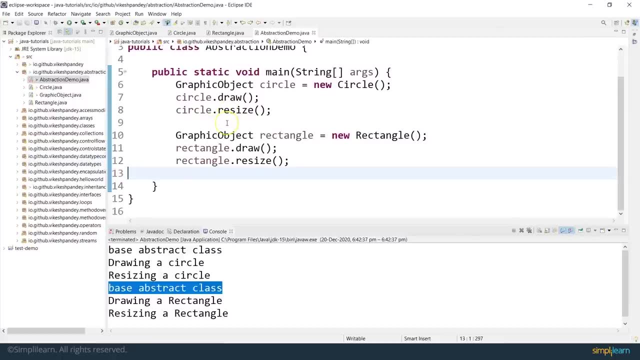 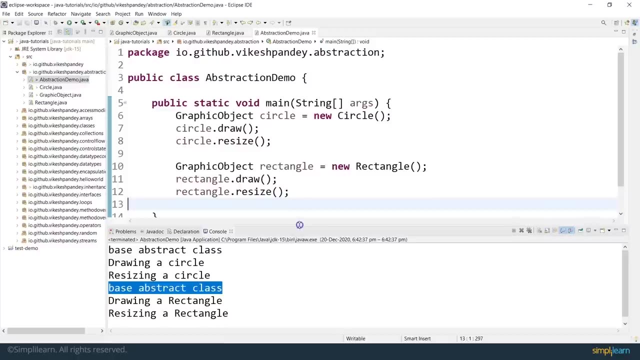 this class is abstract. so hence proved, abstract classes cannot be instantiated explicitly, they can only be instantiated by the child classes through the internal mechanisms of java itself. and that's all i want to talk about in this particular session where we looked in detail about the concept of abstraction, couple of more things which i did not cover in the previous. 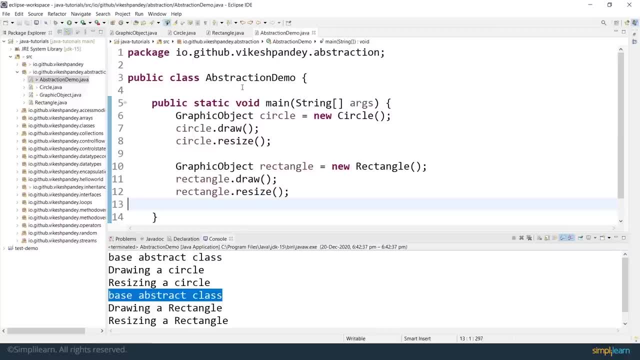 session. i just want to call them out for clarity. java does not support multiple inheritance. when i say multiple inheritance, what it means? that you will not have a scenario where a child will be extending from two base classes. java does not support it. it does support it with the, with the 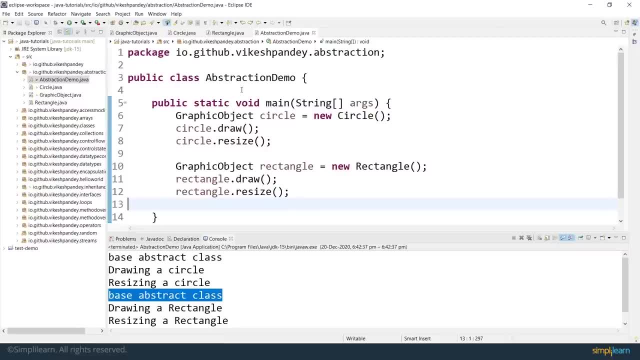 help of interfaces, but i will talk about interfaces in the coming sessions. but here just understand this: that you cannot use multiple inheritance with classes in java. a child cannot have two parent or two base classes in java. java will not allow that. it is also called the diamond. 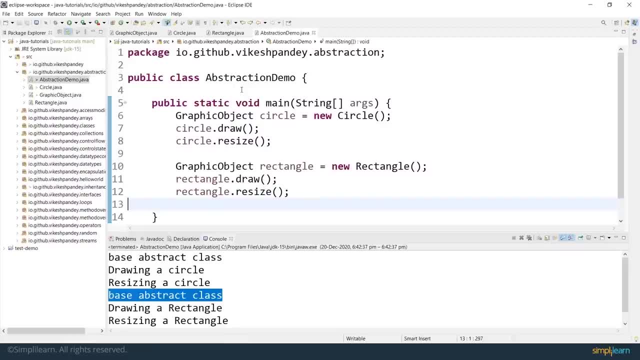 problem because the child class does not know whether to follow the route of base one class or the base two class. if it is, if it is extending from two different base one and base two classes. so a class can only extend from one class. in Java We can find a workaround of it by using the concept of interfaces. 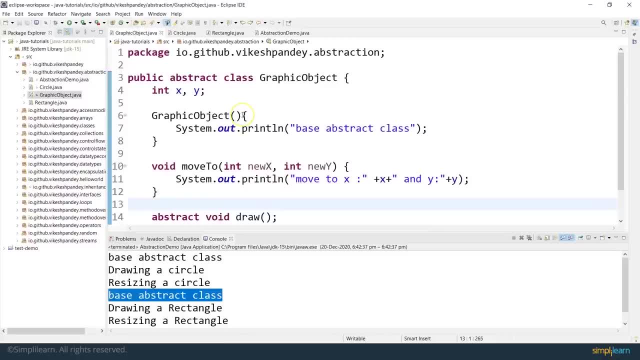 but that's something which will be coming later. Another thing to understand is that when you create an abstract class here- these variables- you can declare these variables as well, and these variables will be accessible by all the child classes as you access them. Let's get started. 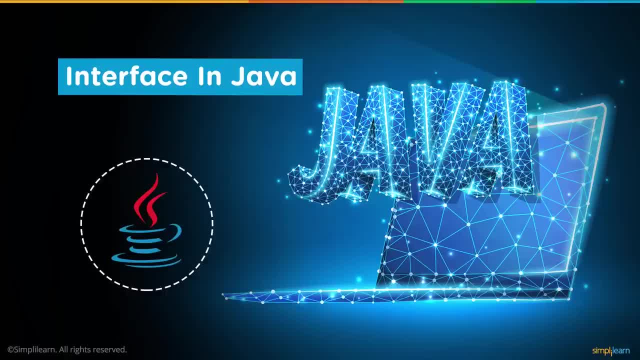 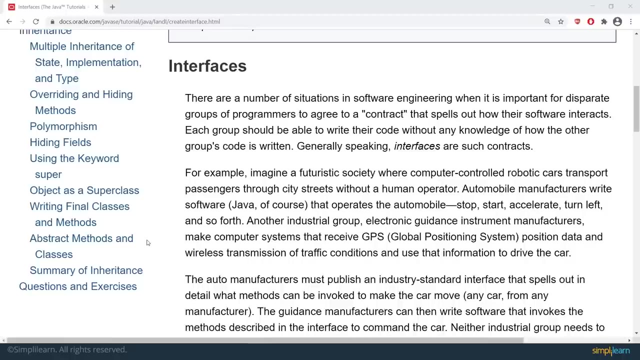 with interfaces in Java. Now again, let's understand what do we mean by an interface in general, and then we will see how do we apply the concept of interfaces in Java. So imagine let's, let's take the same example of vehicle industry, because that's something which we see every day around. 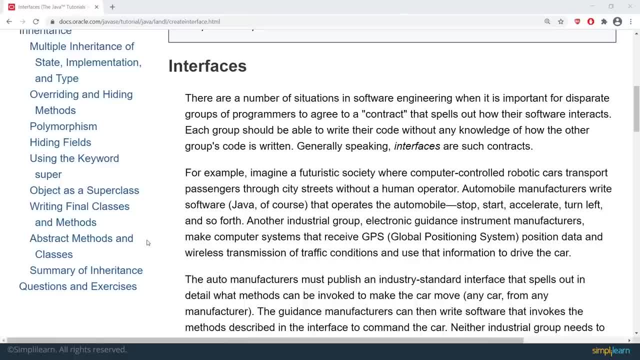 ourself and we can relate to it. So imagine if all the car manufacturers were creating a different way of driving a car. What if in one car you have a steering, but in other car you do not have a steering, but you have something else which is, which may be called something else, In one car? 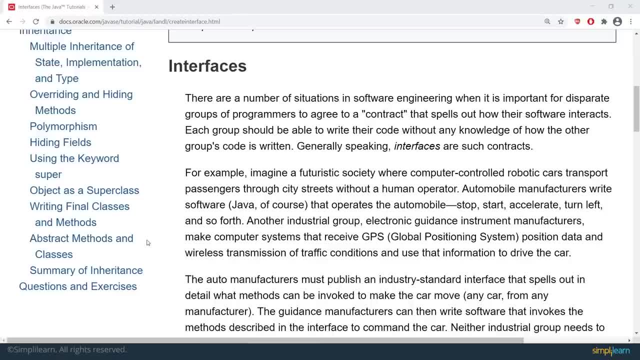 you have the gas Paddle to speed up. In other car you have a button to speed up. Similarly, in one car you may have different kind of doors and in other car you may have different kind of doors which are completely different looking. It's not even a single simple handle to open it. So you see the problem here. 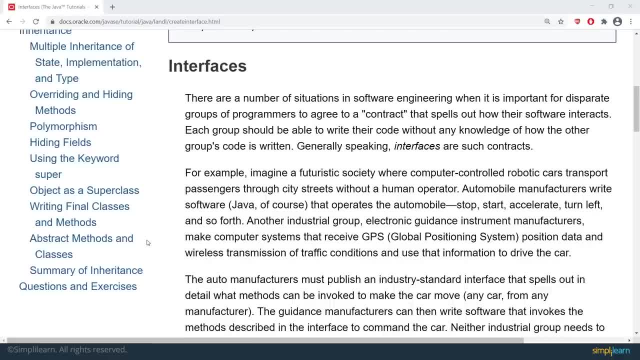 The problem here is that all the car manufacturers are not working on a single contract. They are not respecting a single interface, which will create a poor user experience, because the users have to buy a new car or they have to switch from one manufacturer to other manufacturer. They are 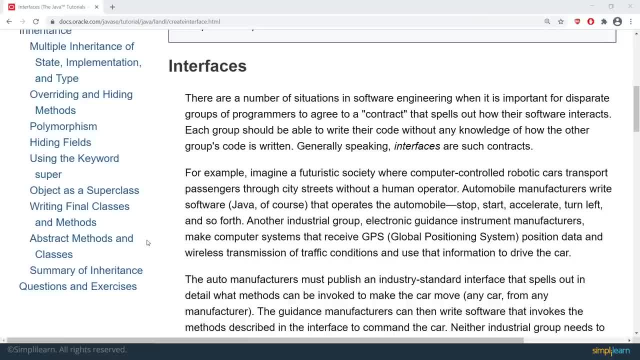 completely clueless as to how to drive that particular class, because the interface they were using in the previous car is completely different from the interface they are being shown in the other car, And that's that's the basic need for the concept of interface. Think of it as a contract. 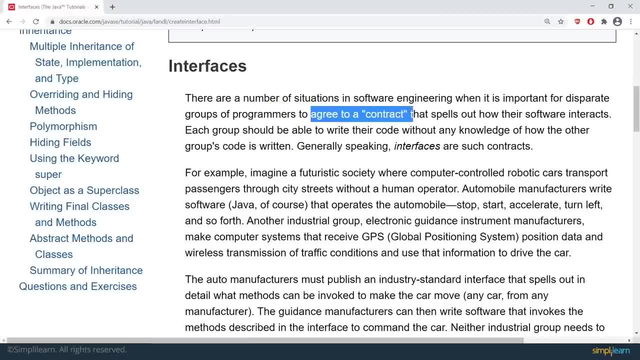 agreement. You see, it is also mentioned here that if you apply the same kind of concept to programming world, imagine if every programmer was writing their own logic in their own way, without following a single contract or a single guideline. Soon it is going to create a problem, and that's the kind of problem. 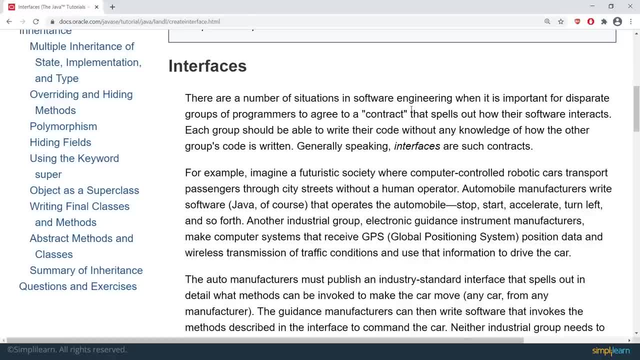 interfaces try to solve. So interface is again a keyword in Java, and the basic idea or the basic construct is that the interfaces are going to define the specifications of how a class would act. Let me repeat this in a more generic way: Interfaces are going to define the contract or the specification which is going to govern how an application or 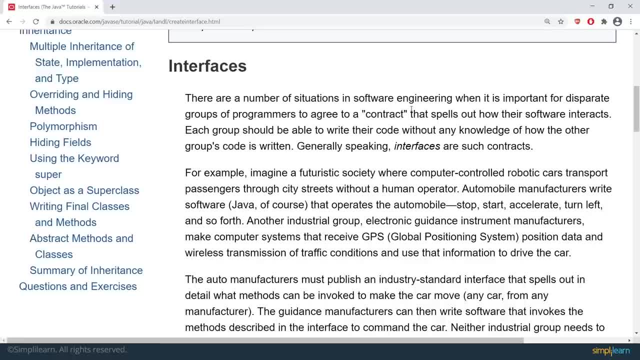 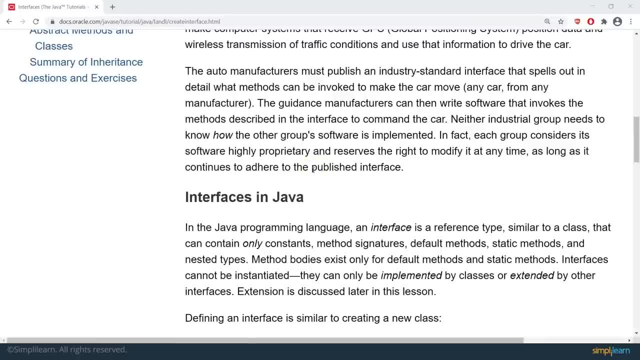 code or programming logic will behave. That's the basic idea of interfaces. So interfaces are their own type And the basic property of interface is that it can only contain constants, method declarations similar to abstract classes and some default methods, static methods or nested types. what is nested type? we will cover that later. default methods: 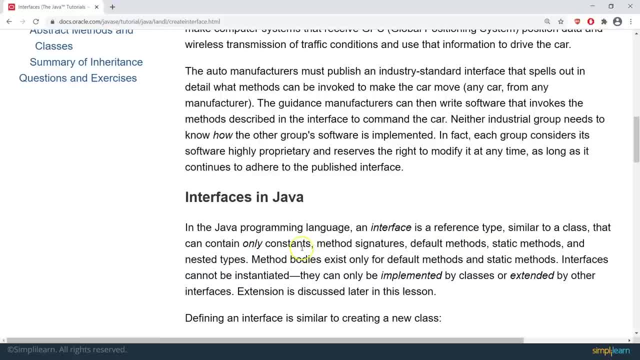 will touch upon a bit here and the static methods as well, but the basic idea is that when you create, when you create an interface in java, you cannot write anything concrete in terms of the behavior of the interface. when i say behavior, always think of that as method. so you cannot define a concrete. 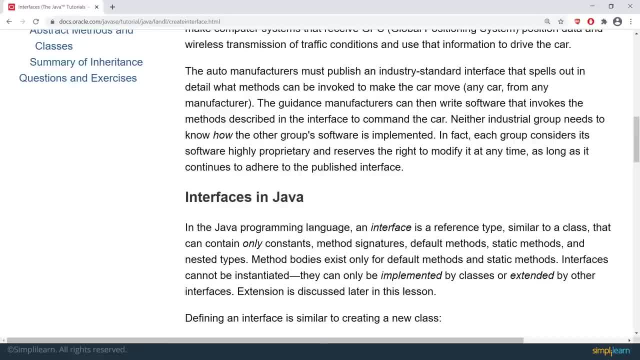 method in an interface. you can only declare methods. you can also declare constants. you can create a particular type of concrete method by using the default keyword, but use it in very special circumstances. you can also create static methods as well, which are only going to belong to the interface and nobody else. now let's look at an example. and and also before we go to the example, 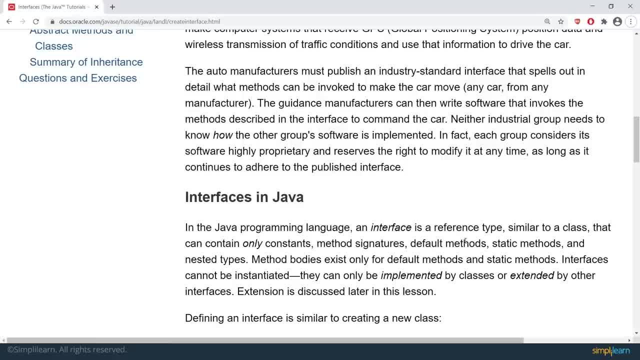 let me also phrase this here, that if an interface cannot define a concrete implementation of the methods, then naturally it will not be able to define a concrete implementation of the methods. the interface is going to be extended by a child class, a concrete class which is going to provide 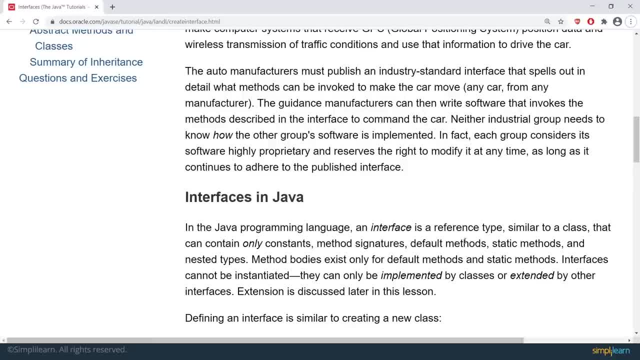 the implementation of the methods declared in the interface. it does sound like abstract classes, but there is a difference. let's understand the difference with the help of an example. this is how an interface will look like. i've used the same construct of bicycle and mountain bike, just. 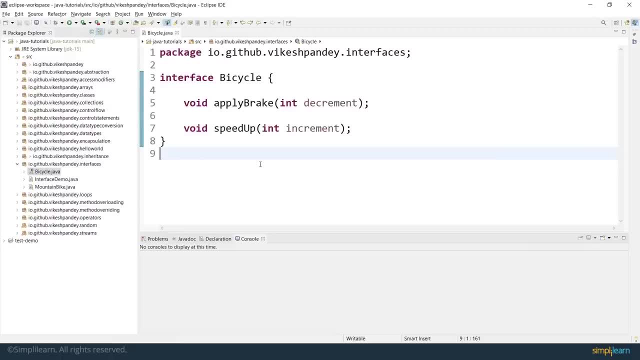 to maintain some continuity and less context switching. but this is how an interface would look like. you will not use the class keyword, but instead you will use the class keyword instead. instead of that, you will use the interface keyword. you can only declare methods. you cannot define methods. remember when we looked at the abstract classes example. 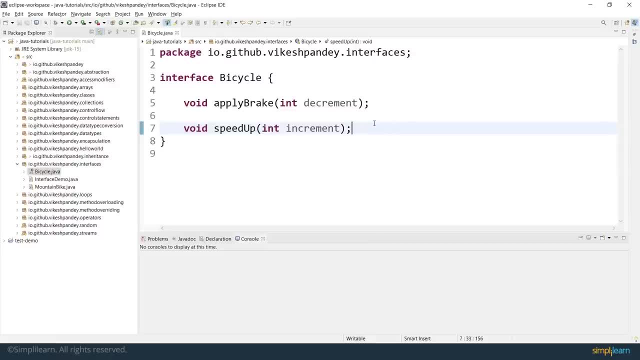 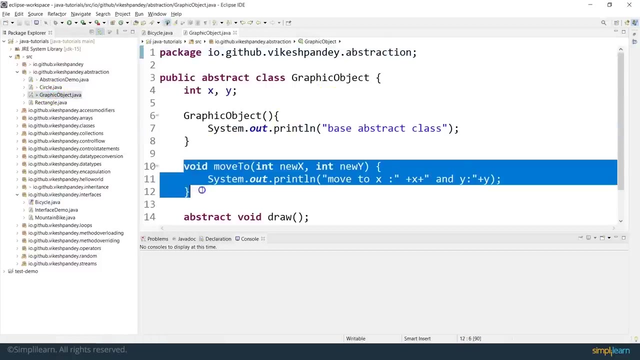 we were able to define concrete methods as well, but in interface that's a strict no-no. you cannot define concrete methods. let me show you the abstract class in the case of abstraction which we used. this was the abstract class and it did have a concrete method, right, but bicyclejava here. 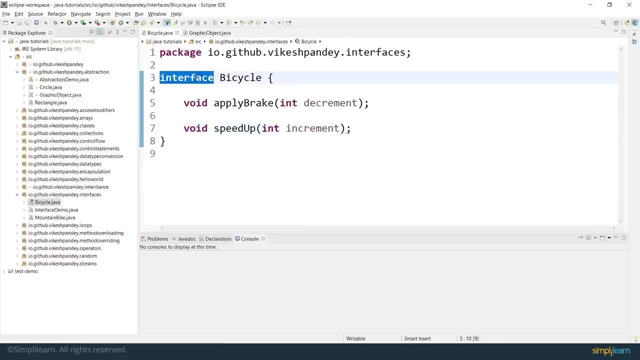 because it's an interface. it is not going to allow you to create a concrete method. another thing is that if you try to declare a variable inside the class, they will have to be constant. you cannot just declare them without any value, for example. i cannot do this. if i do this, it is. 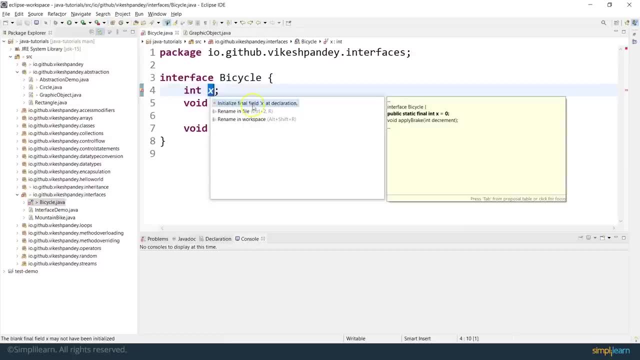 going to give an error. you see an error here and it says: initialize field x at declaration, something like this: public static final. so interface is going to force you to declare all variables as public static final with some value if you try to use them inside interface. so that is also something which interface will mandate. so you see, interfaces are more strict. 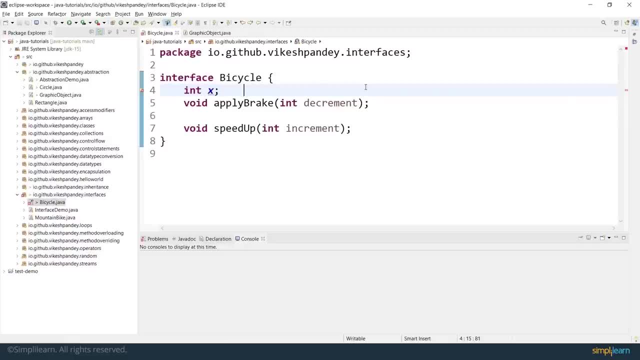 they are more strict in terms of what you can do. you can only declare public static final variables and you can only declare methods. you cannot define methods. so abstract class is less restrictive, interface is more restrictive and that is the differentiation which you have to keep in mind. 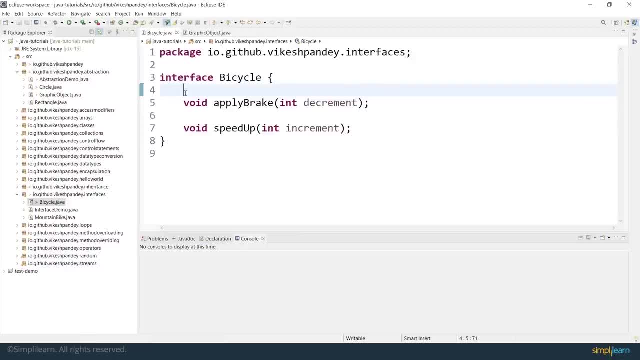 whether to use it or not. you can only declare public static final variables and you can only use abstract classes or whether to use interfaces. that is also a very common confusing question in the interviews as well, and remember that interfaces are only for contracts or specifications, where, in case of abstract class, you can write a concrete behavior as well in terms of a concrete 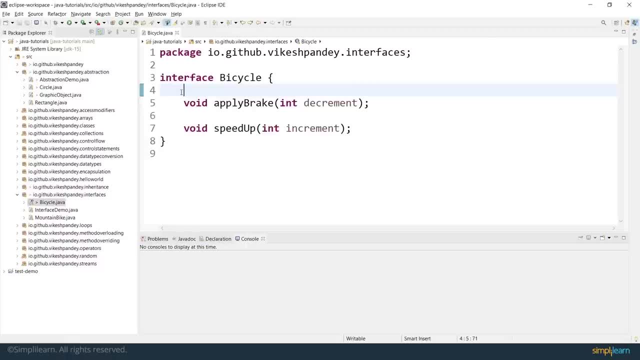 method in the base class interfaces. there is no concrete implementation in the base class. abstract classes: yes, there can be a concrete implementation in the base class. that's the basic difference. now, moving on, i have created a child class here which is again mountain bike, and it has three. 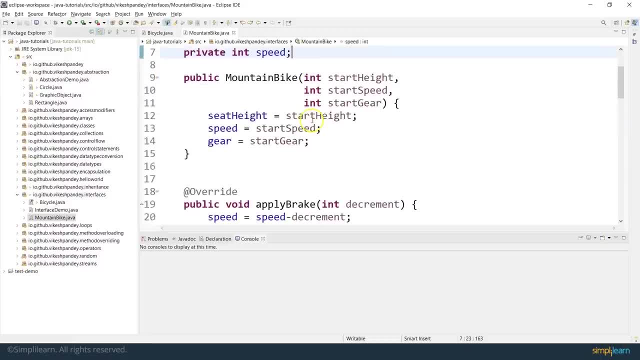 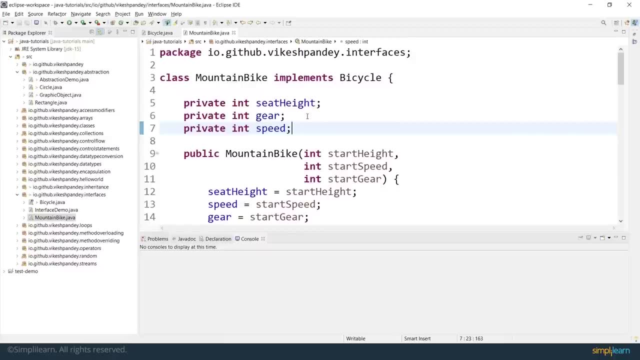 properties: seat height, gear and speed. similar to the previous example, it has a constructor. and remember in again, interfaces cannot be initialized directly. so you don't even need to call a super method here, because there is nothing to initialize. you initialize a class to create a state. state is: 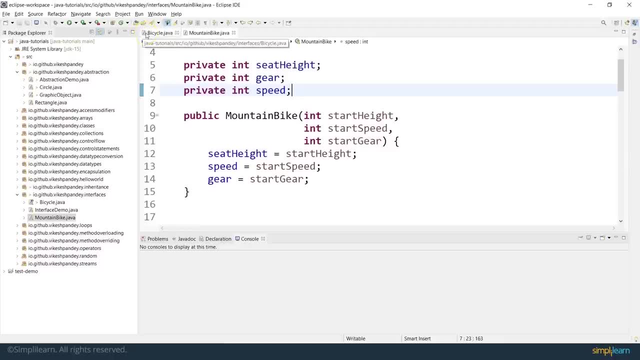 denoted by the properties. but interfaces will force you to write a public, static final property, its value, automatically. so you do not need a constructor for the interface because there is nothing to initialize. everything has been initialized in terms of the variables and the methods are anywhere, just declared. that's why you don't need to call super here after that. the 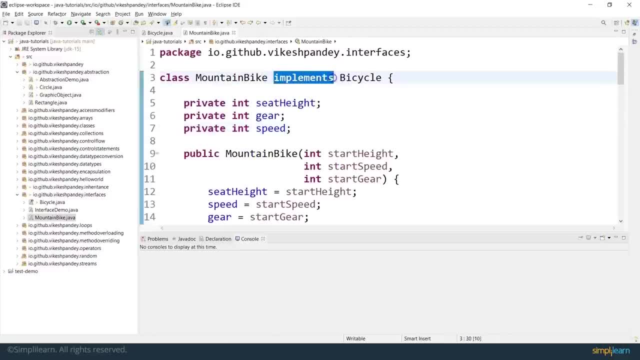 moment you write this particular keyword here- implements- and that is how you will basically extend from the, from the interface, you will use the implements bicycle keyword here implements is the keyword and bicycle is the name of the interface. if you write this here, then java is going to force you to provide the implementation of these two methods. if i, if i do this, implements. 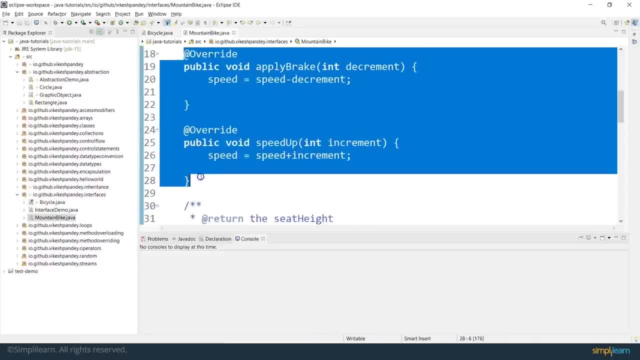 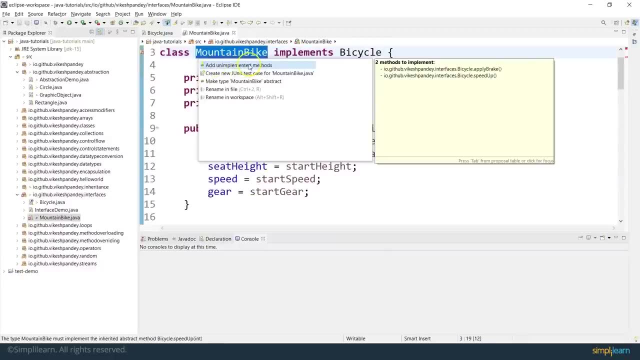 bicycle and if i comment out these two methods, which is coming from the base class, it is going to give an error. and if i read out this error, it says either you add the unimplemented methods or you make the mountain bike class as abstract. there are two ways to fix this particular class. 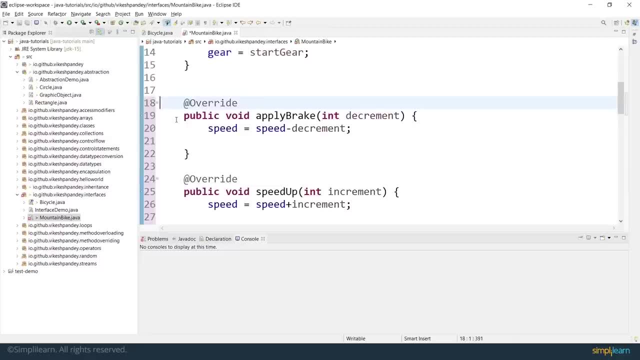 similar to abstract classes. it will force you to write the implementation of the base class declared methods. another thing which java will will suggest you and will will also force you via some ides as well, is that you use this particular annotation. we use this particular annotation to tell java that we are overriding this method from the base. 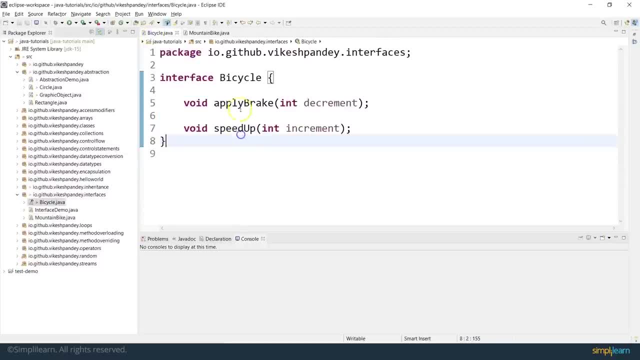 class, since apply, break and speed up methods were defined here in the base class, and this child class is supposed to provide the implementation of the methods by overriding them. overriding is again a concept which we will call overriding, and overriding is again a concept which we will call overriding. 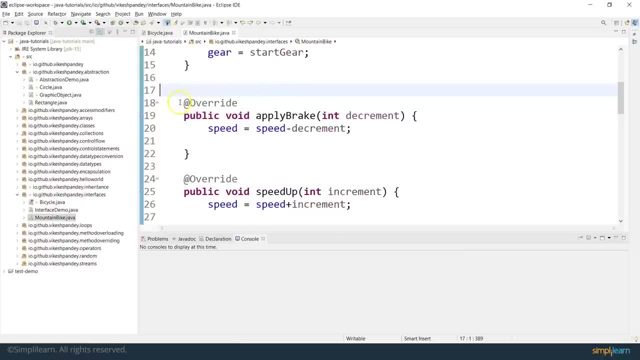 and overriding is again a concept which we will talk about in detail in the coming sessions, but for now, remember that you need to write this annotation here on the methods which have been taken from the base class to provide an implementation, and the implementation is similar to what we have seen before. so whatever value you supply in the apply break, the speed is. 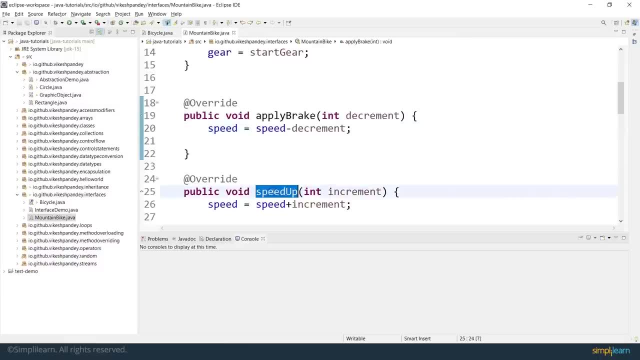 going to get decremented by that particular value and, in case of speed up, whatever value you supply in the argument, that value is going to be added to the current speed and the speed is going to go up. because we already received the answer when we were talking about, when we were talking about the 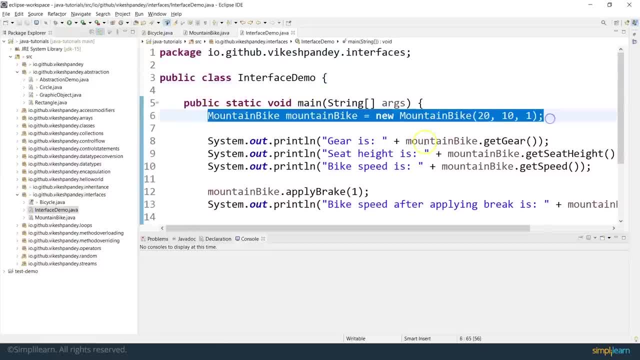 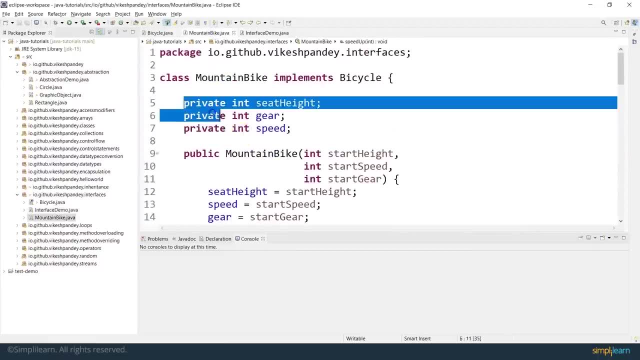 default value. what we were supposed to be looking for this time is the value we used, and this is going to be the value that we're going to get, so let's go back to our code. so what we're going to do is we're going to thread the input from the base class and we're going to create a interface. 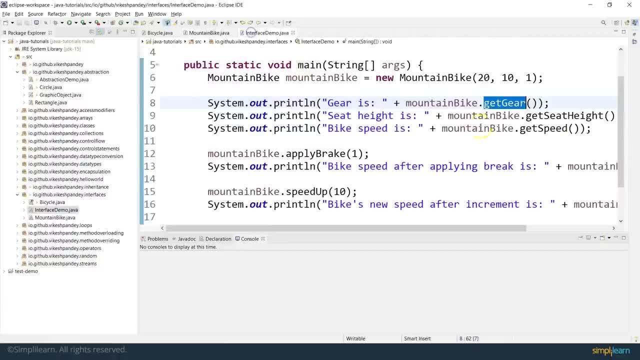 demo, which is going to be domain, and we're going to start the interface demo. we're going to create the main class here, which is called interface demo. it has a public static void main method. and here i'm, then i'm printing the current speed after applying the brakes. let me just expand this a bit more. 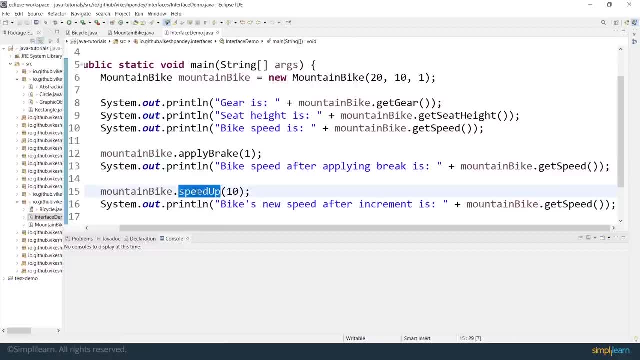 and then i'm using the speed up method, trying to increase the current speed of the bike by 10 and then printing the new speed again. so using the apply, break and speed up methods, which are concretely defined in the child class by using this override annotation. and these were the 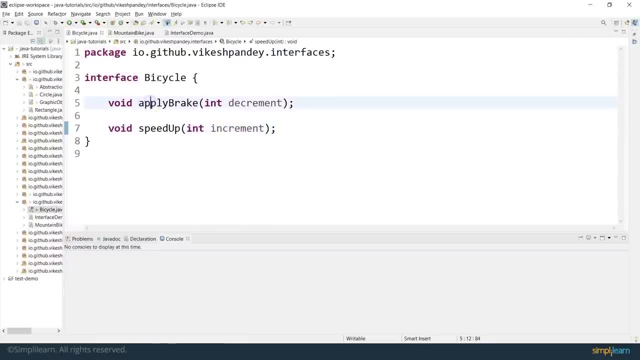 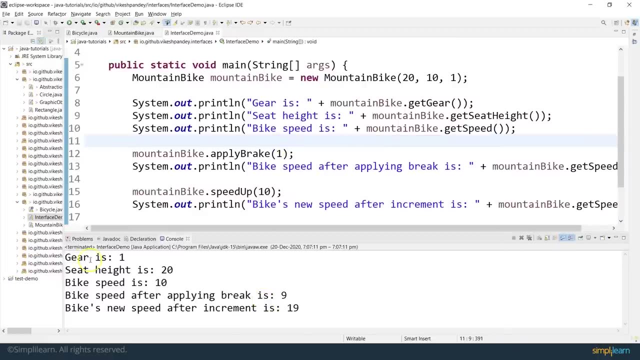 methods which were declared in the interface, in the base interface, and that's all which is happening in this particular class. let's run this particular program and these are the values i get. i get the gear as one which is coming from here. i get the seat height as 20, which is coming from. 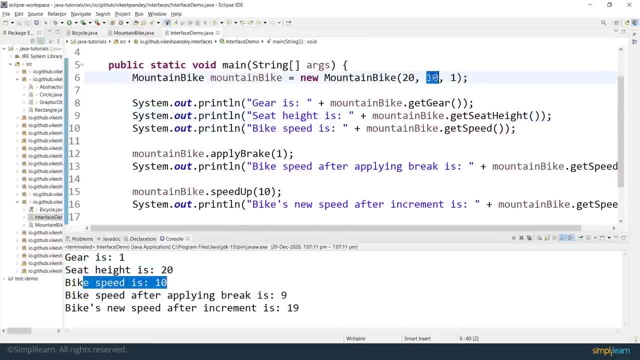 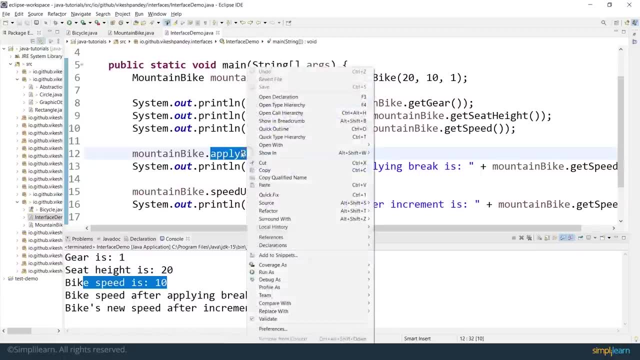 here i get the current bike speed as 10. this was the value which it was initialized with. then i'm applying the break and after applying the break, the speed of the bike gets reduced and it becomes 10 minus 1, which becomes 9, and that's what gets printed here. 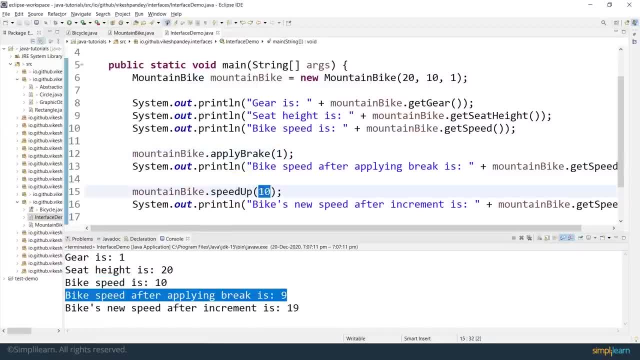 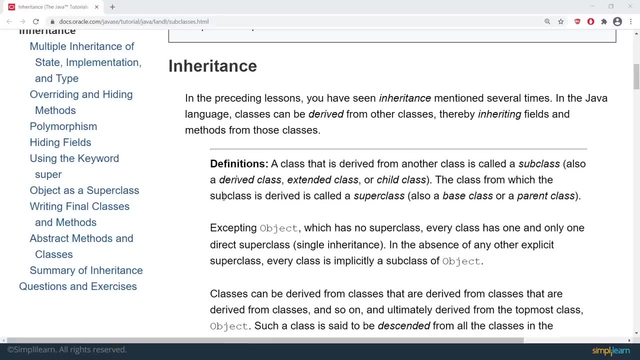 and then i'm speeding up the bike by 10. so the current value of the current value of the speed of the bike is 9, and if i incremented it by 10 it becomes 19, and that's what gets printed here. let's get started with inheritance. so inheritance is basically one of the 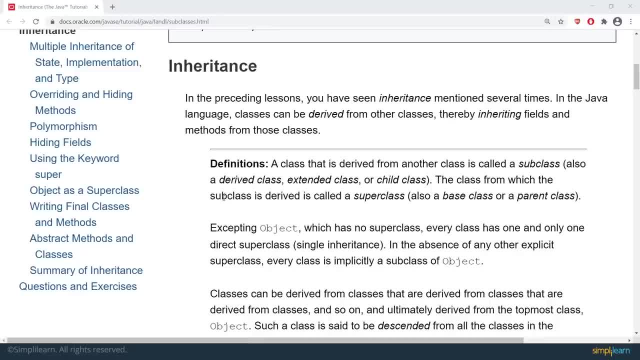 most important properties of any object oriented programming language. it's basically a concept and the concept says that what if you have a scenario where you want multiple classes to share similar behavior and similar properties? let's understand this with the help of an example. let's take the example of a bank. when you go to a bank to open an account, 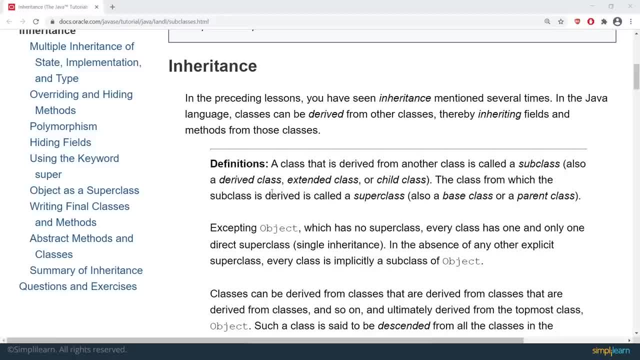 there are multiple types of accounts. there can be a savings account. it can be a type of current account. there can also be a different offering for personal account and commercial accounts, such as for businesses. then you may also have loan accounts, which are having different kind of properties. so 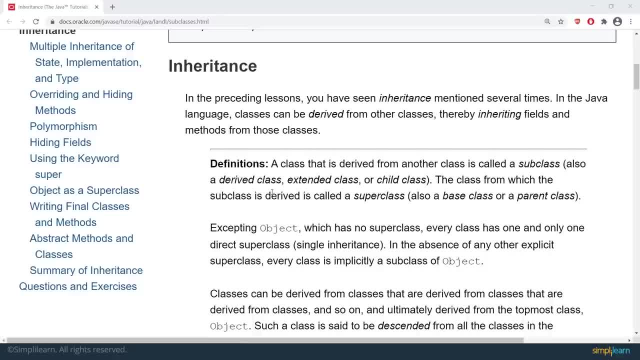 many accounts that are that are completely different types of accounts are still technically accounts and they will share some similar properties. for example, all of them will have to maintain some sort of an interest rate. for example, all of them will be used to either deposit money or withdraw money, so there would be some kind of similarity across all of these. 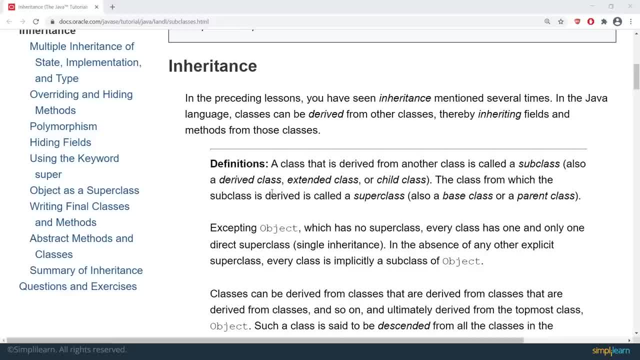 types of account classes, but at the same time there will also be some sort of differentiality amongst these classes: the way you will calculate the interest rate for, the way you will calculate the interest rate for a savings account, and the same applies for commercial account, personal account, loan account, etc. so you see that we have some common behavior. 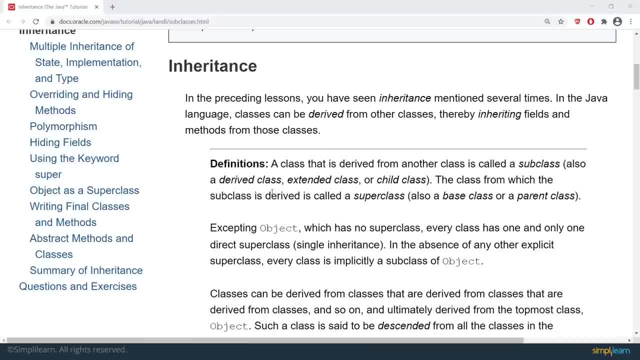 but at the same time, we also have some different behavior. so whenever you have such scenario, always think about applying the concept of inheritance in your application. there's another simple way to spot whether inheritance can be used at a particular place or not. inheritance is also called is a relationship. so whenever you read the requirements from a customer, 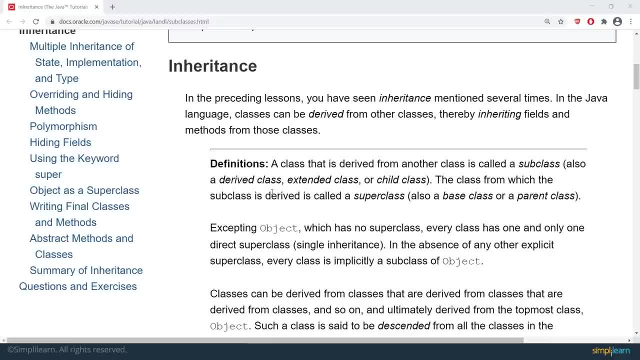 just try to find the words which use this particular phrase. is a, for example, car? is a vehicle, savings account is a type of account. similarly, you will find many other types of similar examples. so whenever you will see that is a relationship between two different kinds of objects or two different kind of entities. that means that there might 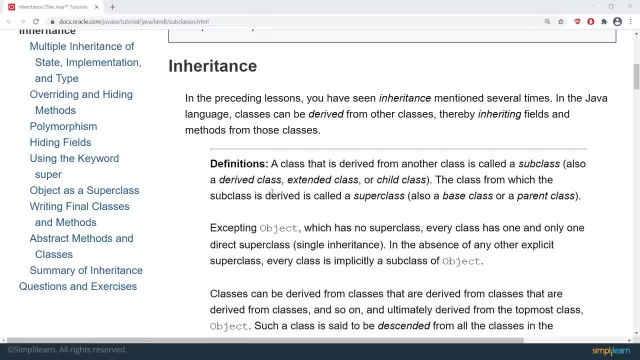 be an inheritance relationship being applied between them, and that's how you will spot the usage of inheritance. so so far we have understood this concept that there would be some sort of relationship between the two classes. what will be this relationship? the relationship will be of parent- child type. there will be a parent class- some people also call that as base class- and then 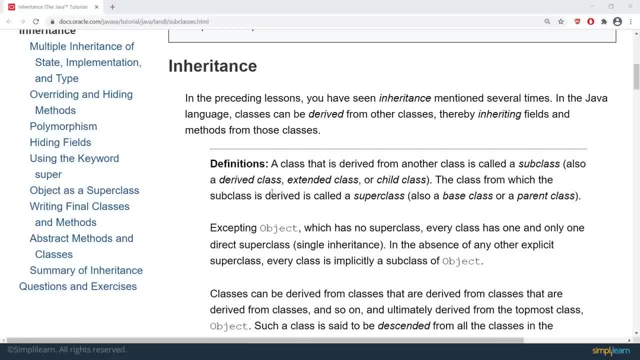 there will be a child class, so the child class will be inheriting the properties and the behaviors from the base class or from the parent class. i will be using base class and parent class terms interchangeably during this session, but the basic idea and basic premise is like that, only that there will be a 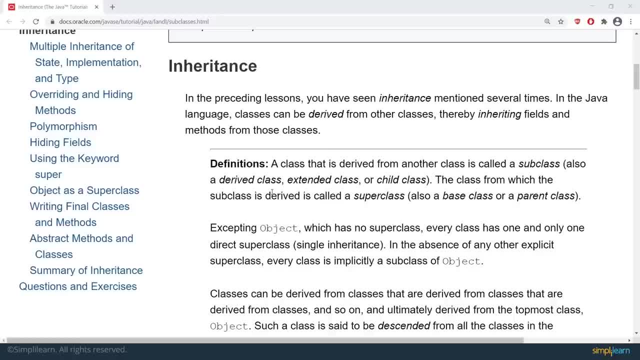 child class and there will be a parent class and the child class class is extending from the parents class. remember the word extend, because we are going to use that and i've just shown you the. what you see here is basically the official definition which is given by java docs here. 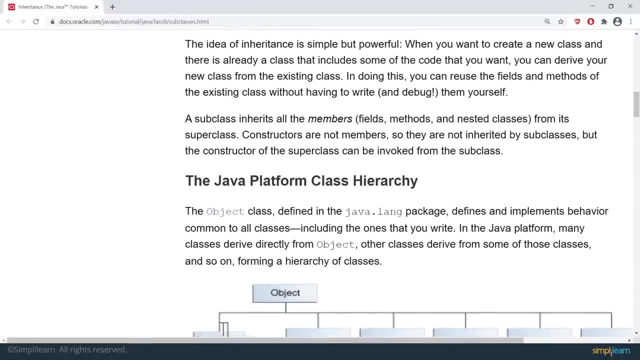 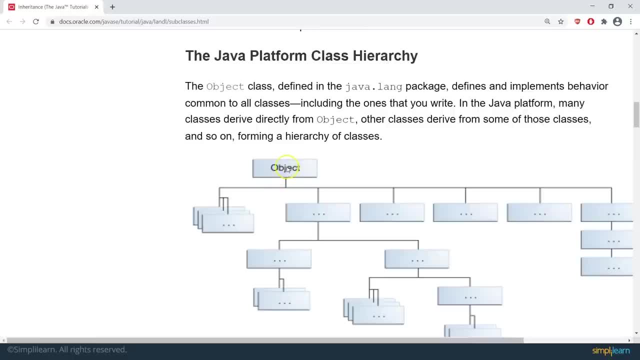 we can read the definition as well, and the basic idea which i told you lies in the parent and child relationship, and this is how you can conceptualize it: that you will have a base class or a parent class, and then you will, you can have multiple children of it, and then 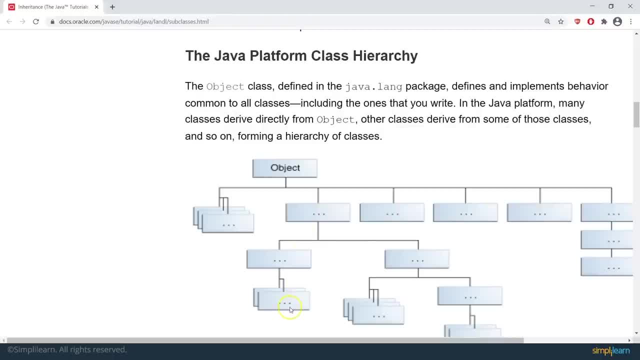 those children can again have their own children, and so on, so forth. so this hierarchy, this whole inheritance hierarchy, can go as deep as you want it to be, and that's the basic idea and basic conceptualization of how you understand and how you visualize inheritance. now let's move to eclipse. 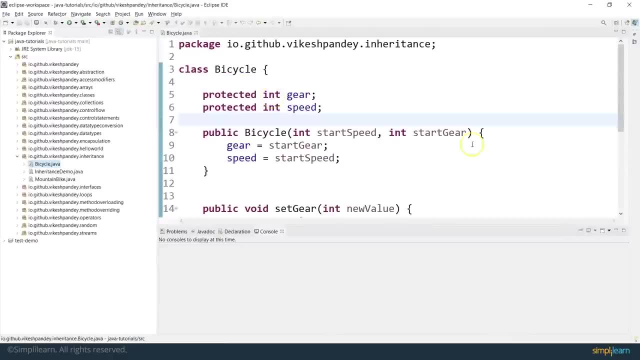 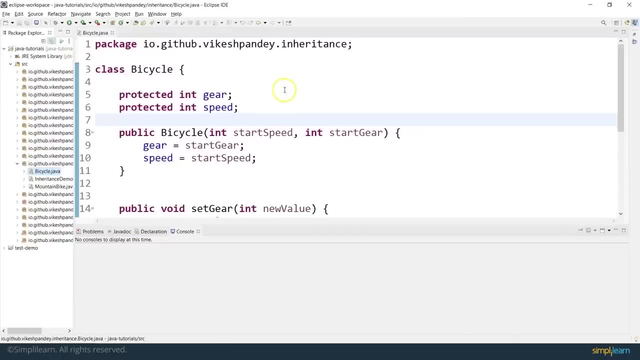 and see how you can understand the relationship between inheritance and child. this is very important and i will try to understand this with the help of an example. so, for this particular case, i have created a set of classes, basically, which we will be using to demonstrate the relationship. 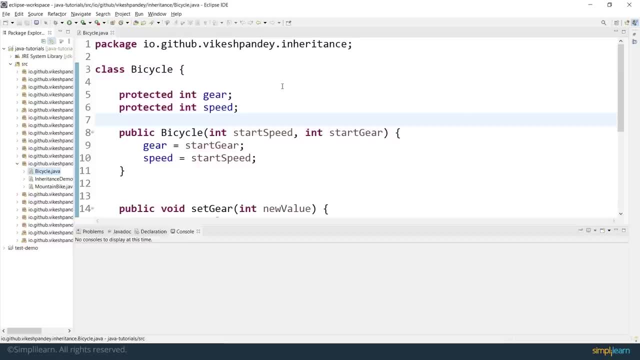 of inheritance and i've taken the simple example of a bicycle. so a bicycle is again a very generic definition of any two-wheeler, and bicycles can have multiple types. there can be an all-terrain bike, there can be a mountain bike, there can be a city bike. 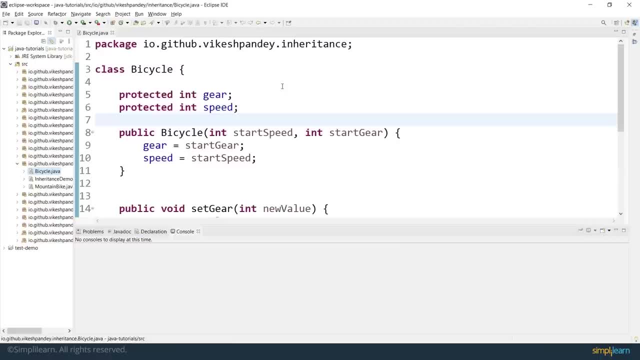 for ladies, and similarly, there can be multiple different types of bikes, but all of these bikes will have some similar properties. for example, all of them will have two wheels, all of them will have a seat, all of them will have brake, all of them will have some sort of of some sort of a speeding. 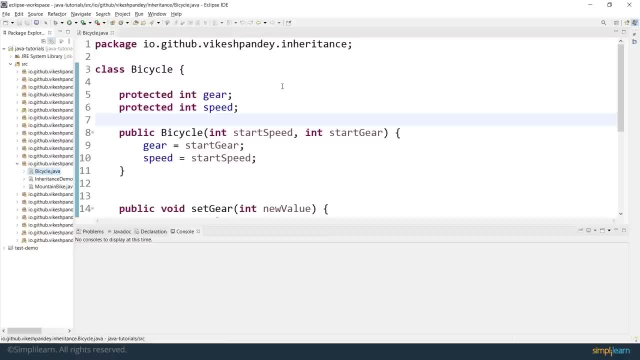 mechanism, whether they can accelerate or de-accelerate. so there will be some commonality, but at the same time a mountain bike's features might be very different from a city bike feature. a mountain bike features might feature, mountain bike might have gears, for example, whereas a city. 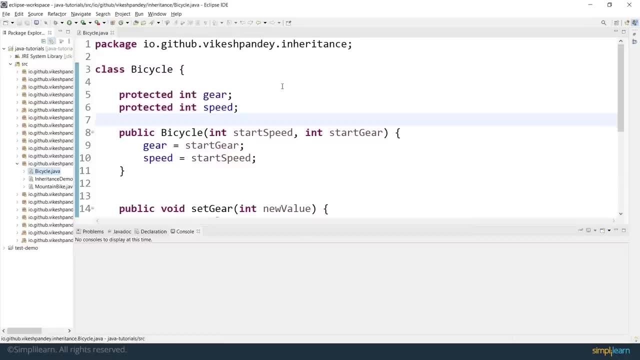 bike might not have gears, because you don't need that much of a variation in inclination and declination when you drive down the road. so i'm trying to conceptualize the same example here, where i've created a class called bicycle and this is my base class. i defined two properties in the 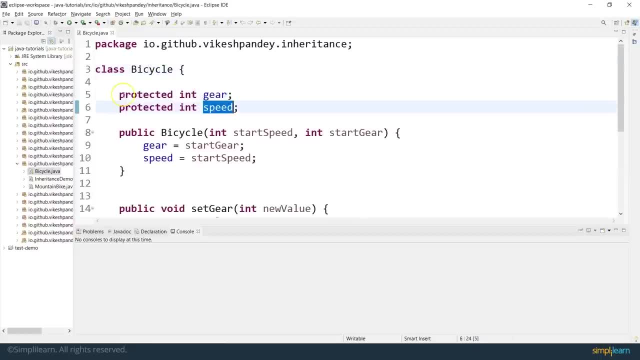 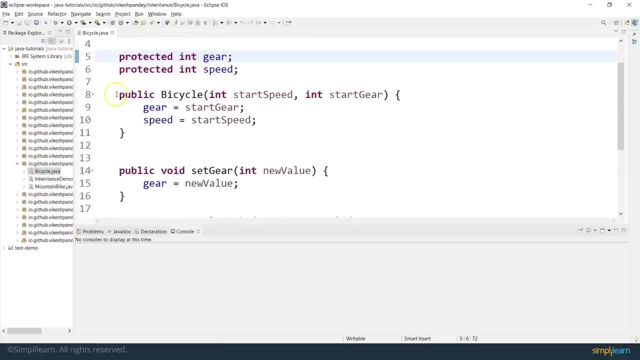 in the bicycle class, which is gear and speed. we will come back to protected in a while, but let's, let's leave that there. so i have two properties, which is gear and speed. i have a constructor where i'm initializing the starting speed and the starting gear and then i have three methods here. which says set gear. 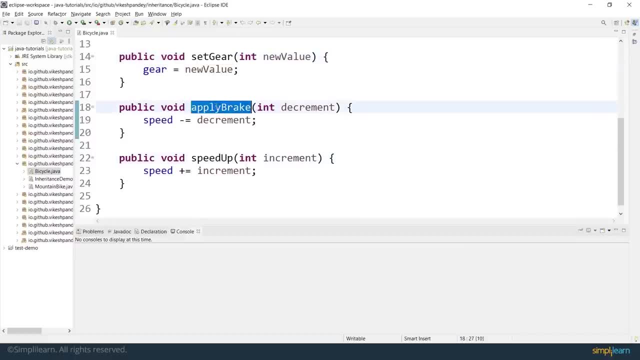 apply brake and speed up. when i apply brake, the speed is going to get reduced. so that's why you see minus, equal to unary operator. and when i'm trying to speed up, the speed is going to increase. that's why i'm using the plus, equal to unary operator. so when you use the method speed up, 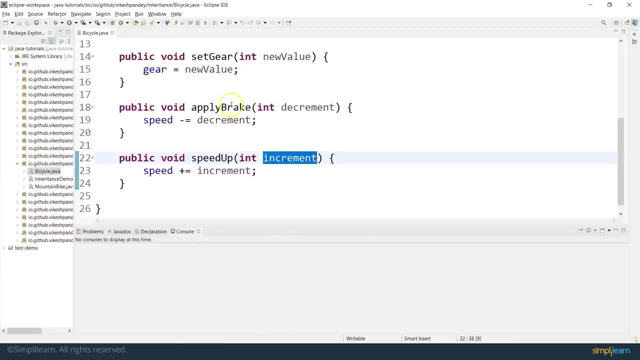 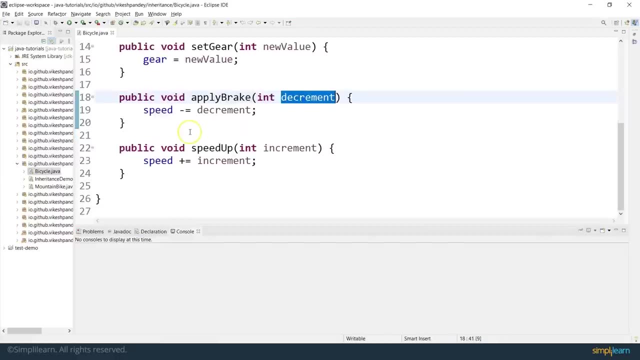 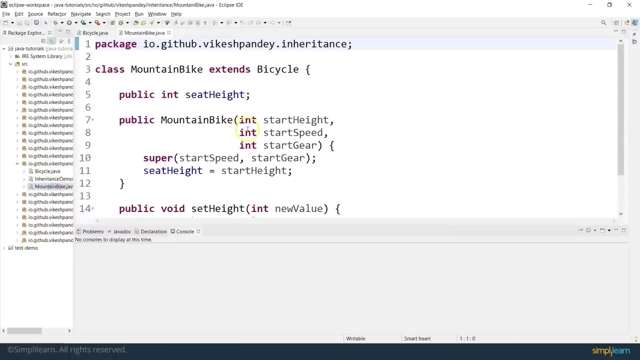 to be increased by the value you supply in the method. similarly, when you apply the break, the speed is going to get reduced by the amount you supply in the method argument. and that is my base class: bicycle gear speed and three methods. now let's have a look at the child class. so the way 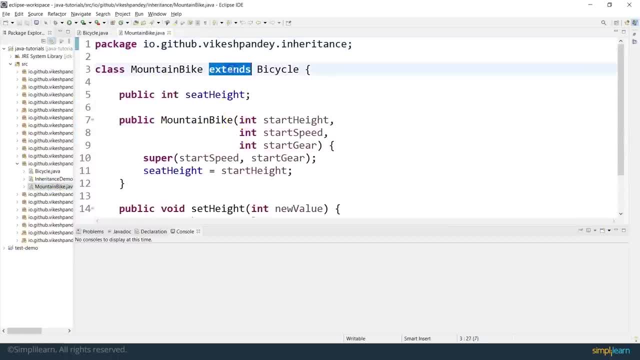 you will define the inheritance relationship in java is by using this extends keyword. remember, i told you to remember the extends keyword. so what you will do, that you will write your class name as usual and then you will use extends keyword and then you will use the parent class name, or 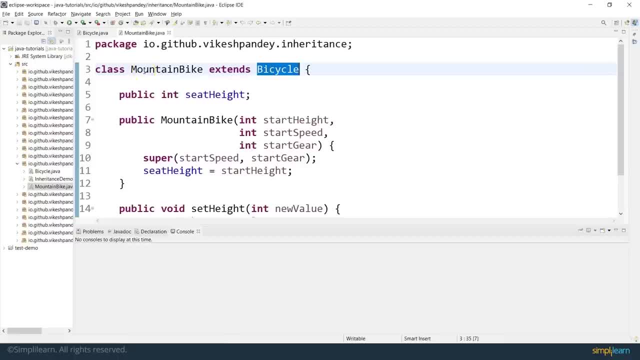 the base class name. so here i'm saying class: mountain bike extends bicycle. and here i'm providing an additional property. remember the whole commonality versus differentiality equation. so a mountain bike might have an extra property to adjust the seat height. so that's the extra property which mountain bike is having. and then, since this mountain bike, 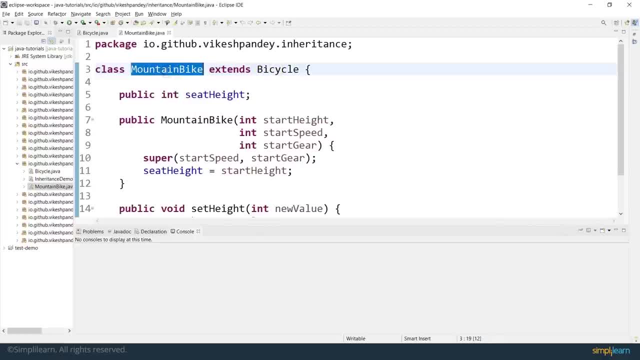 is extending the bicycle class. this mountain bike class has the responsibility to initialize the bicycle class as well, and the way it will fulfill that responsibility is by taking all the arguments of bicycle class plus the mountain bike class in its constructor, and that's why you see three different properties here. you see the start height property, which is the property of this. 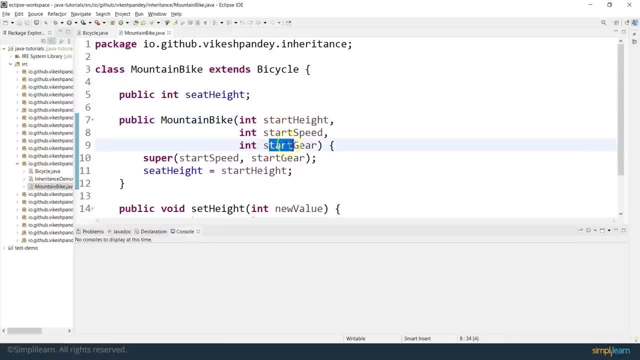 particular class, which is the seat height. and then you see the start speed and start gear property, which directly are not available in this class, but this class is inheriting those properties from the base class. remember the keyword inheritance here. and then, once you do that, how do you initialize the base class? constructor is by. 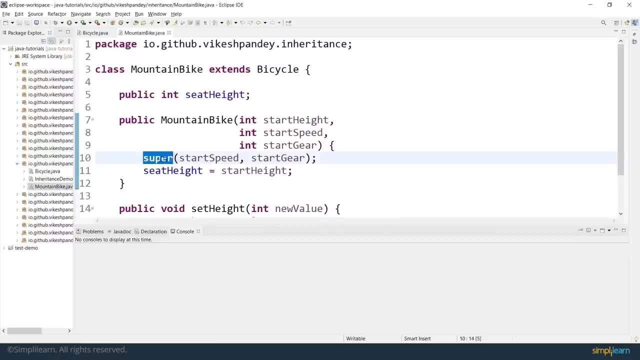 calling the super method. this is again a keyword in java and you will use this super keyword to refer to the base class constructor in this way. so what you will do technically is that you will write super and you will supply the arguments which is required by the base class constructor. if i go back, the base class 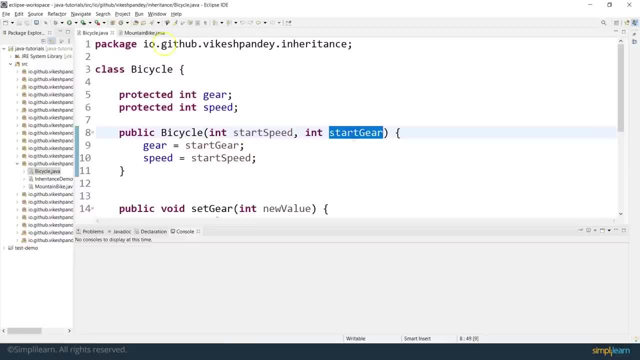 constructor requires two arguments: start speed and start gear. so i write super and then i write start speed and start gear. so whatever i got from here in the constructor of mountain bike, i'm supplying those values, as is to super, and java will automatically take care of invoking this. 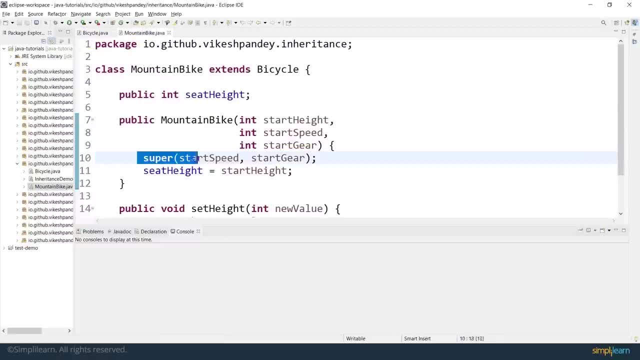 particular constructor the moment it it encounters this kind of statement. another another thing to notice is that the super keyword or super statement has to be the first statement inside your constructor. remember that whenever you are dealing with inheritance and whenever you have to initialize the super class constructor or the base class constructor. 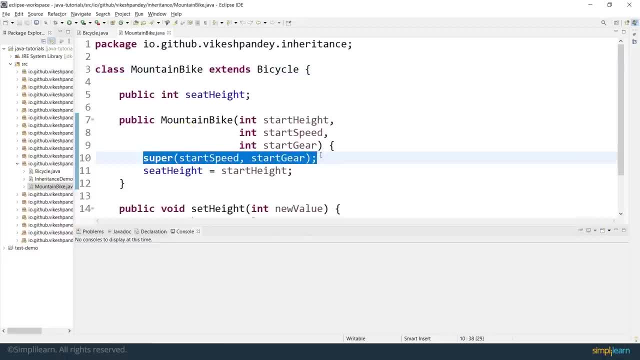 use the super constructor invocation as the very first statement inside your child class constructor, otherwise java will not compile the program and then you will initialize the local variable. i should this as this remember: i we discussed about this in this in the classes session. okay, and then it just 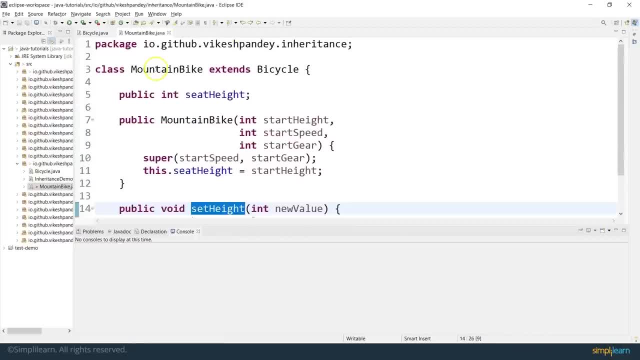 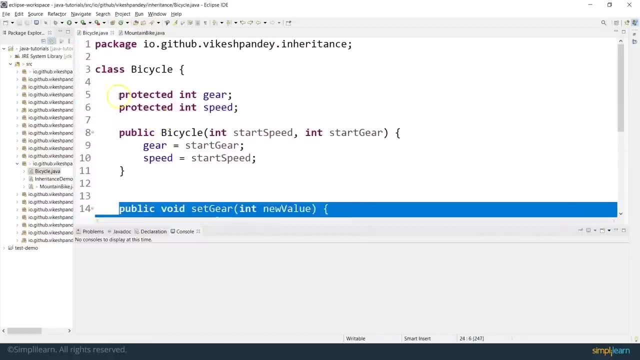 has a method of set height, so there's no extra method which this mountain bike is providing, but this mountain bike will have access to all the methods which have been provided here and all the properties which have been provided here. this mountain bike can access everything from the. 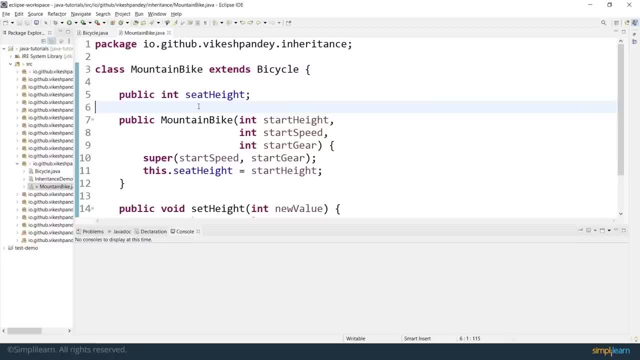 bicycle class. and that's the whole idea of inheritance: that the child class can access the properties of the base class by extending the base class. now let's look at how do we invoke this particular class. so for that i have a simple class name as inheritance. demo, which has a public static. 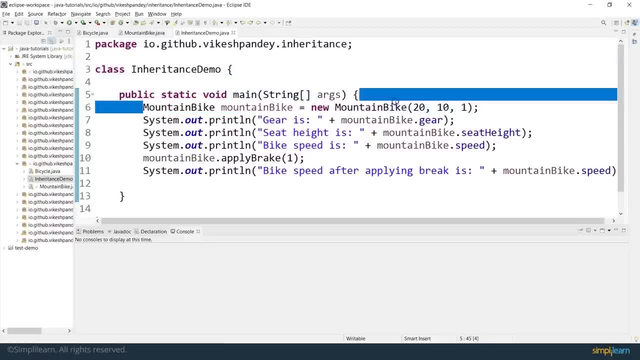 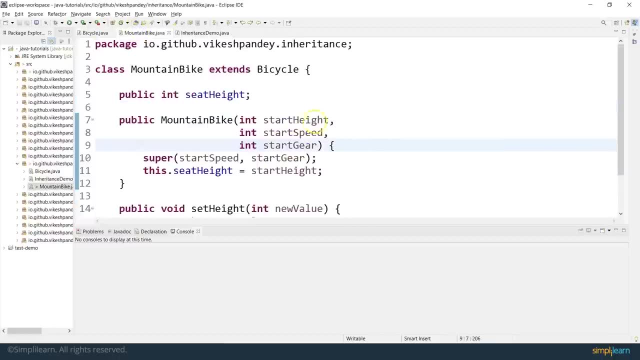 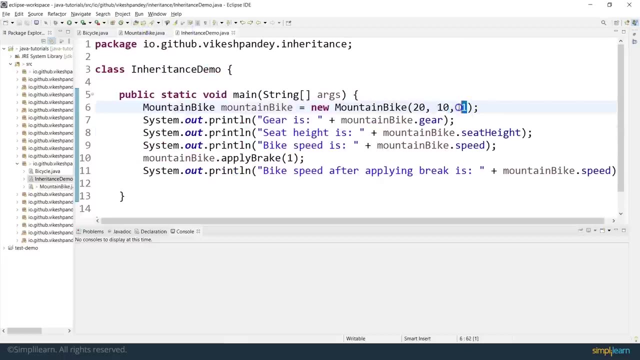 point, main method, and then i am initializing the mountain bike class. i'm supplying three values as 20, 10 and 1. so the 20 goes to start height, the 10 here goes to start speed and one here goes to gear or the start gear. and that's how i'm setting the values. so when i call this particular 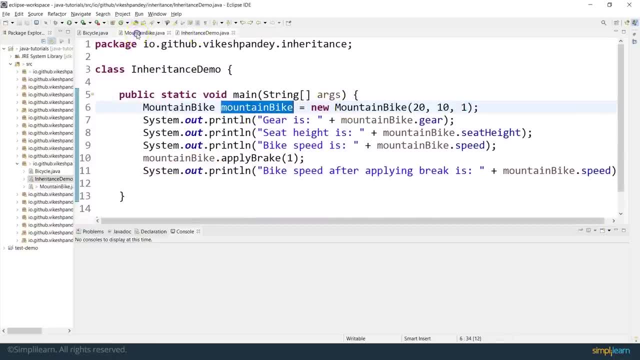 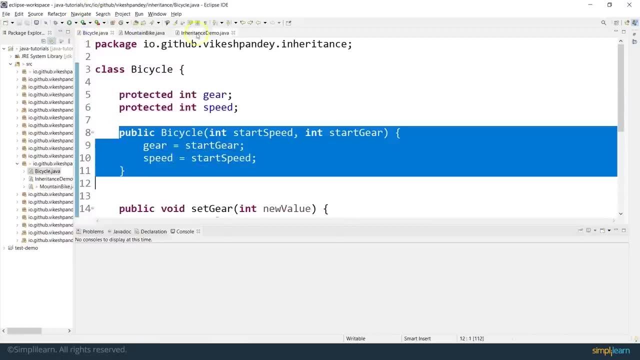 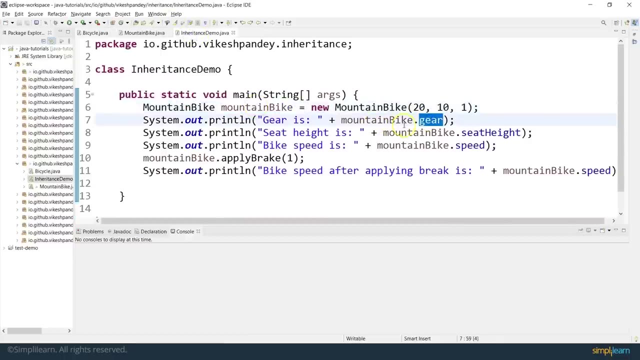 constructor. here the mountain bike constructor is going to. this mountain bike constructor is going to get called and which in turn is going to call the base class bicycle class constructor as well, and everything will be set accordingly. and then let's try to access the gear property. remember, gear is not directly available in the mountain bike class, but i'm still able. 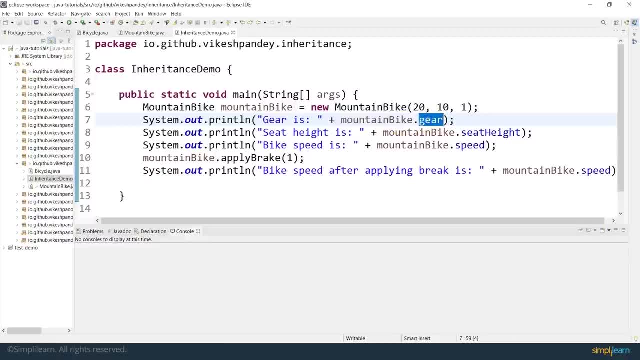 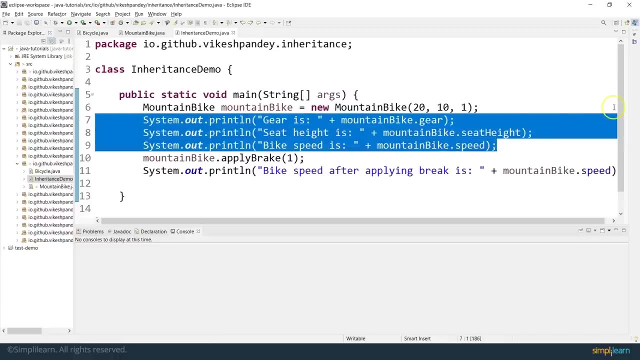 to do mountain bike dot gear, because child class can access the parents class properties similarly. the same thing goes for speed as well, and seat height is the local property of this particular class mountain bike, so it will anyways be accessible. so i can access all the properties of the base class and the child class itself seamlessly, without any differentiation. now let's. 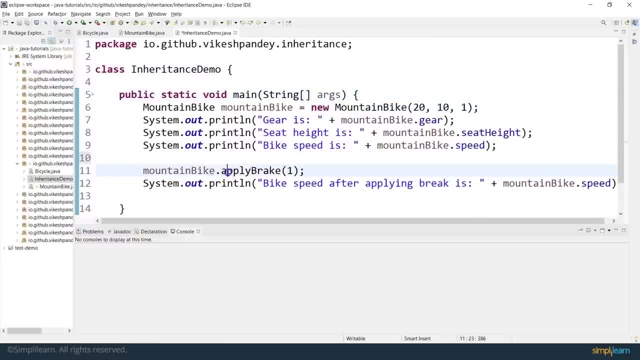 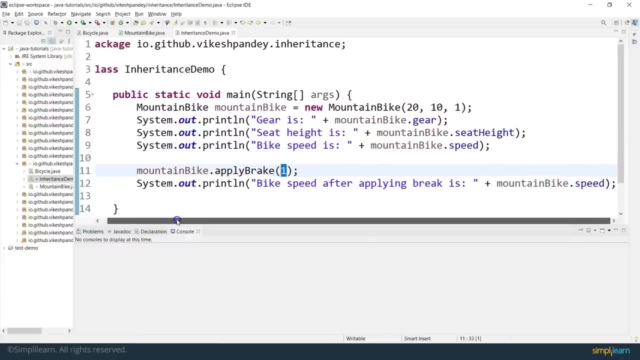 try to call a method. so here i'm calling the method apply break. remember, apply break was defined in the base class, not in the child class. it's defined here. so i'm calling the apply break and i want to reduce the speed, the current speed, by one, and then i'm printing the current speed. 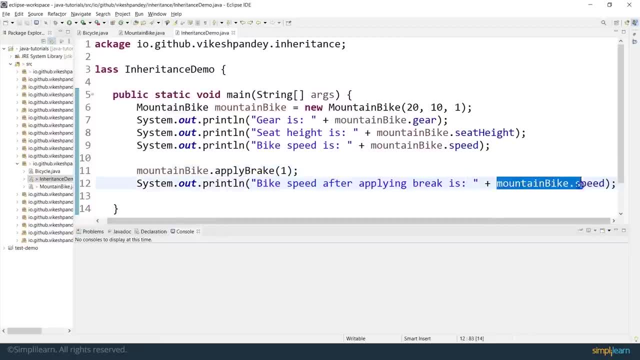 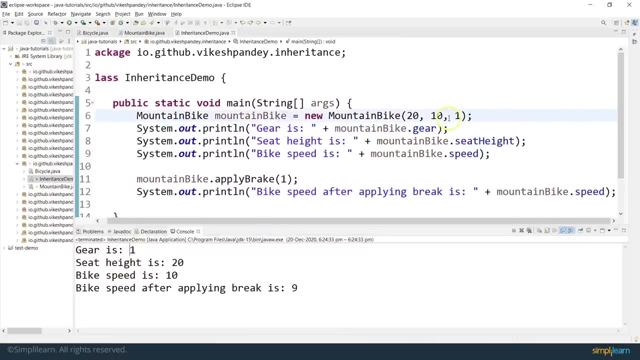 saying that bike speed after applying break is mountain bike dot speed. so let's run this particular program and observe the outputs. okay, so the the first statement which gets printed is at line number seven, which says: gear is one, because it's coming from here. then the seat height is mountain bike dot seat height, which is 20, which is the first argument here. 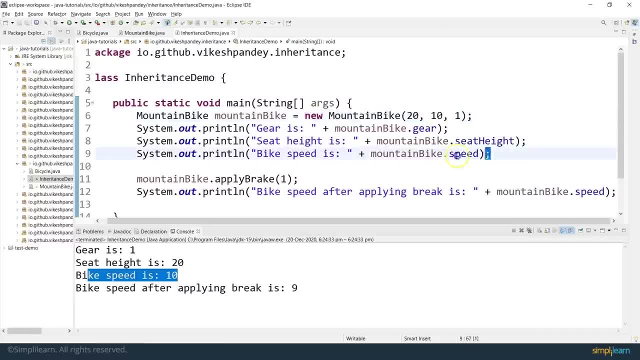 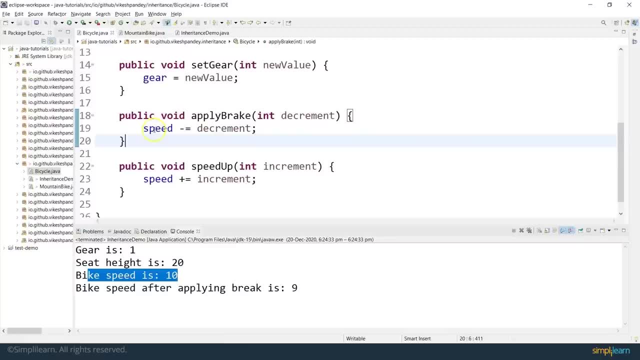 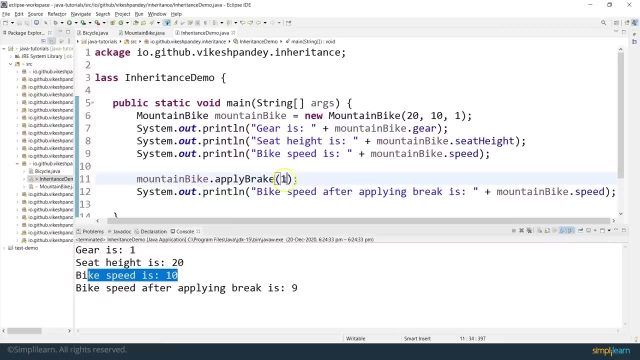 and then the bike speed is 10, which is coming as here and getting printed here, and then when i apply the break- let's go back to the apply break method. the logic is that whatever is the current speed, reduce it by the value i supply in the method. so if i supply 1, 10 minus 1 becomes 9. 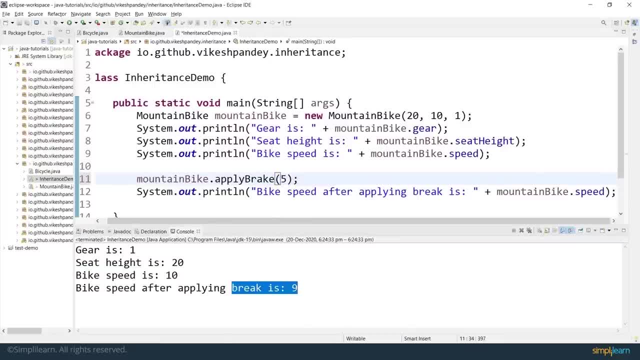 and that becomes the current speed. if i supply 5 here, the current speed will be 10 minus 5, equal to 5.. let's assert that particular assumption as well. yes, we can see that, and similarly you can access other methods of the base class as well. if i just do control space here and you 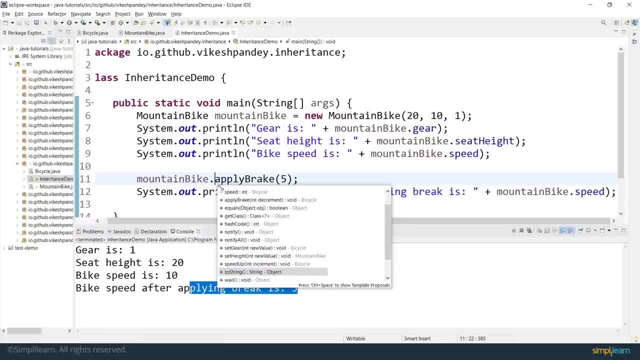 can see. apply break is accessible. set gear, set height, speed up. all the methods which are defined in the base class are accessible in the child class as well. this is the power of inheritance. one more thing which i said i will come back to is around the usage of protected access modifier. 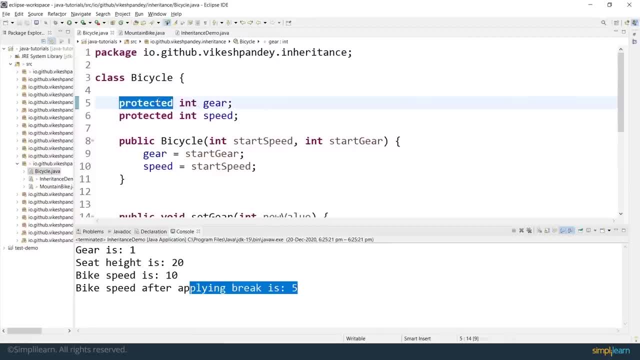 remember, when we discussed about the access modifiers in the previous session, i said that protected is used when you are dealing with inheritance, that whenever you define something as protected, it will be available to be accessible in the child classes of the base class. so if i define this particular variable as as protected, then this particular property will be accessible. 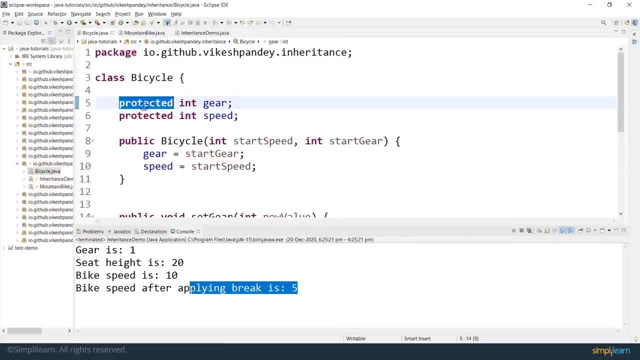 in the child class mountain bike as well. let's play around this. let's make this as private and see what happens. so if i make this private now, when, when i say private, the scope of this particular variable is within the class only and nobody outside the class has to be private. so let me. 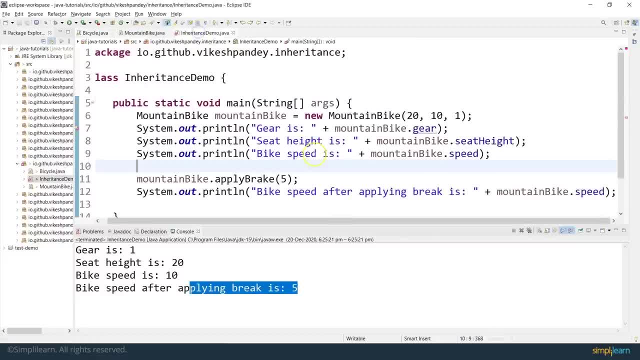 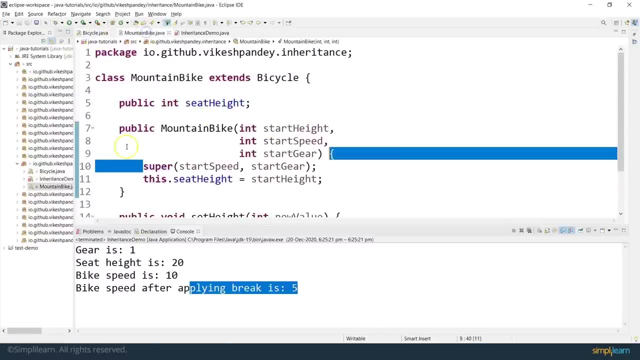 class will be able to see it and you can see the effect of it. i can see an error being coming here in my inheritance demo class because now mountain bike object cannot access the gear property because the gear property is defined in the base class and now it is private. that's why the child 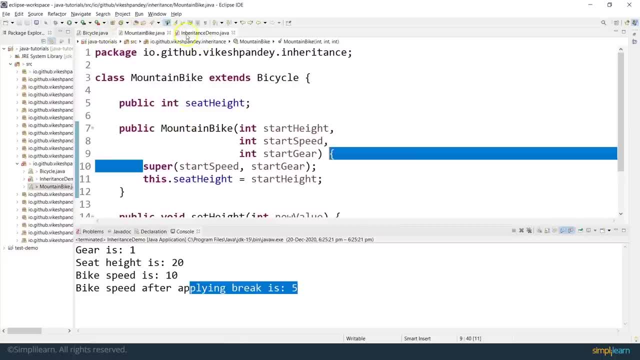 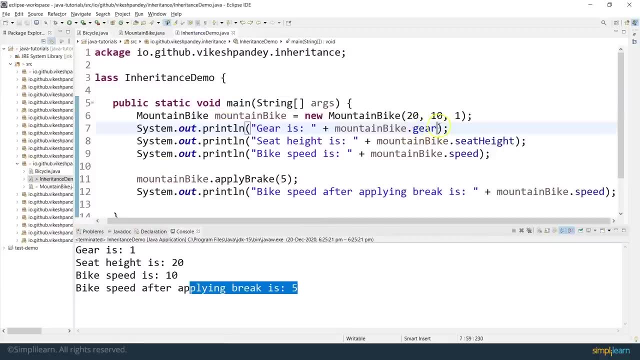 class- now mountain bike class- cannot access the property gear, and the moment you make make it back to protected, it will be accessible. the error is gone. there's no red line here. so that's how you can. you can use the protected access modifiers. it is always, always recommended to use them when you. 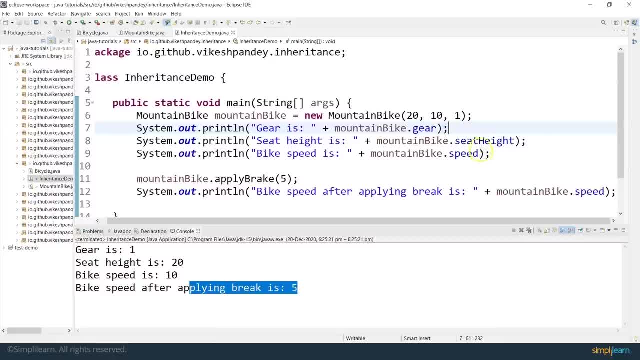 when you write any kind of inheritance logic- and in inheritance logic as well, intentionally, if you want to hide a particular property from the child classes, just make it private. and that's all i want to cover. in this particular session, where we dive deep into the concept of inheritance, we had a look. 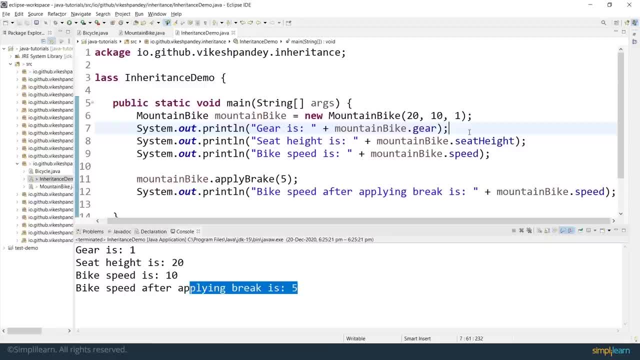 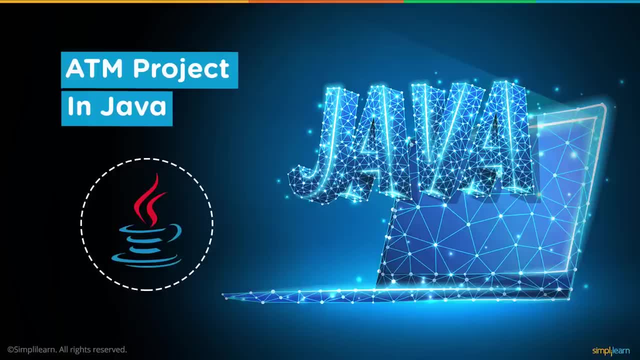 at an example using the bicycle and mountain bike kind of construct and you can apply the same kind of construct on any kind of other other kind of constructs. so that's all i want to cover in this kind of business requirement. remember that is a relationship. let's get started with walking. 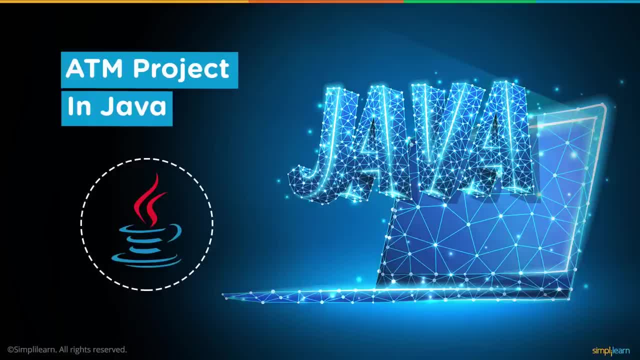 through a particular project, using all the concepts which we have learned so far. so in this session, we are going to focus on a particular project, and the project we are going to focus is is about an atm application, so you might have interacted with different atm stores in your cities. 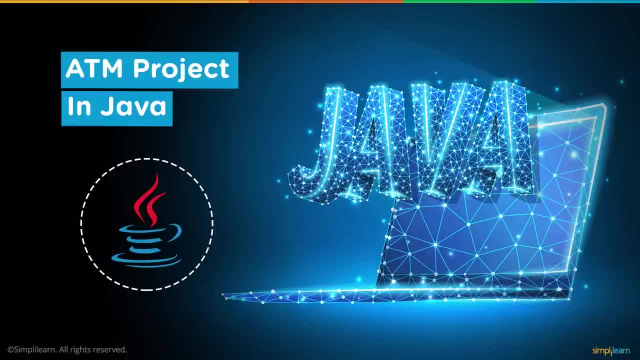 where you go in, you insert your card, you enter your pin and then you can view the balance. you can withdraw some amount. you can also deposit some amount from the atm. so we will try to look at it from that perspective and we will see what kind of different uh java and 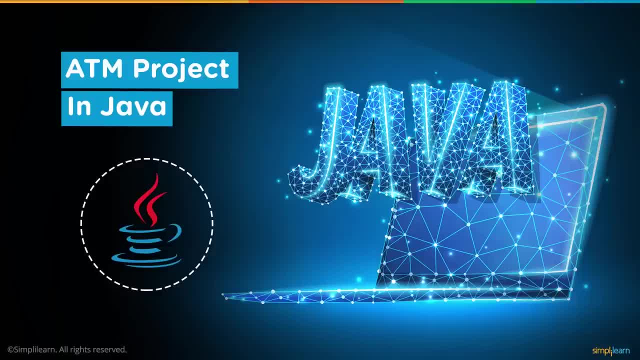 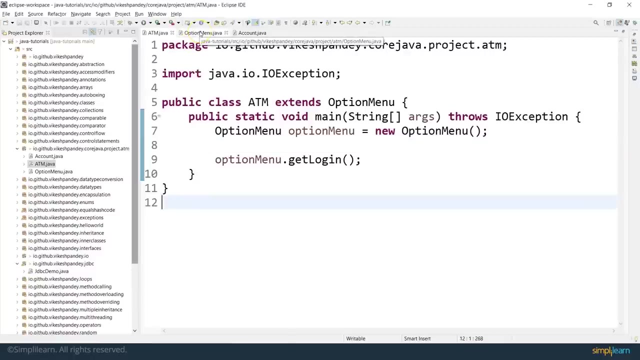 oops concepts we can use to build such atm application. this is not a super versatile application, but but this is just to give you the idea of how to use those oops concepts to build a simple or a complex java application. so let's start from the options menu class, because that 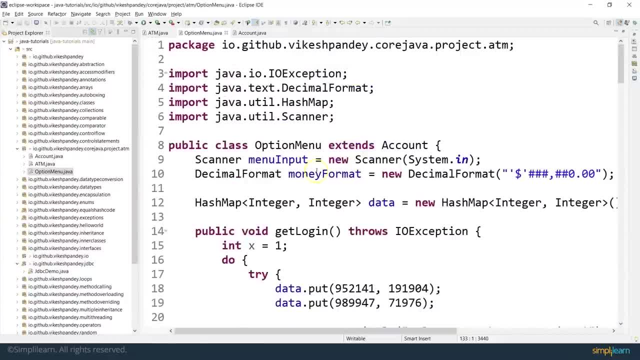 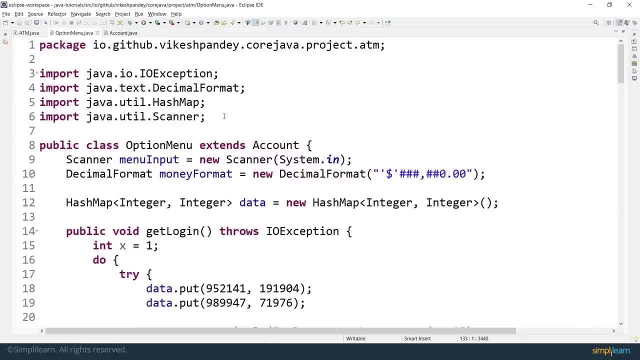 concepts which i which i have taught you so far in this particular series. so, for example, we are using the iu exception, we are using the hash map class, we are also using the scanner class, which is used to take input from the command line. so this option menu class is extending the account class. 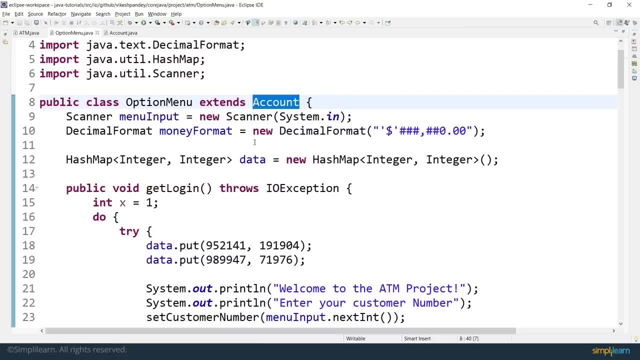 and i will come to the account class in a while. but let's see what this option menu class is doing. this particular class has, uh, it is using a decimal format, money format class, which is to denote what mat of money you have. then we have a hash map which is storing a couple of records of account. 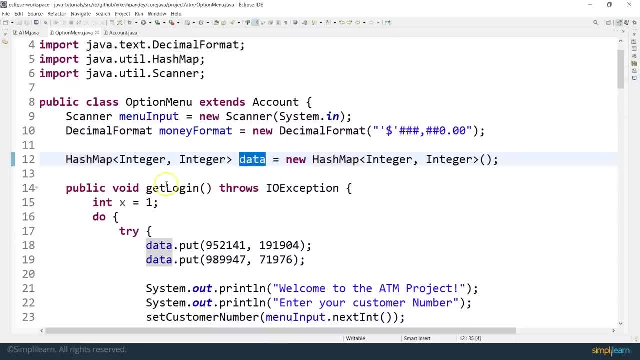 number to pin mapping. so we create a map and inside the get login method we add couple of entries to the map. here the first entry, the first integer, is pointing to the customer number and the second integer is pointing to the pin of the account of this particular customer number. so 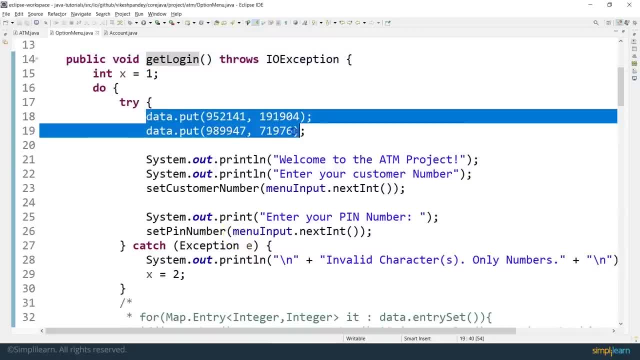 if we call the get login method, this method will insert the data. after that, it will ask the customer to enter the customer number, which has to be one of these two. if you provide any other value, then there should be a logic in the application to reject the input. 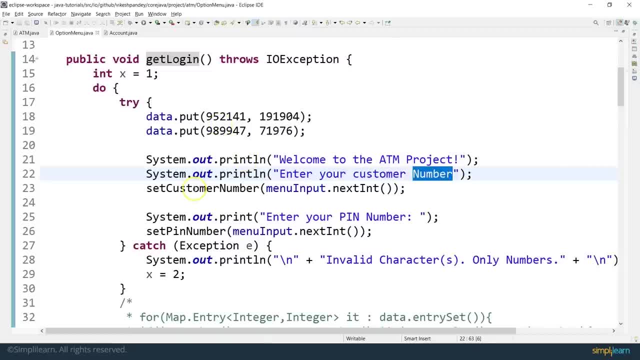 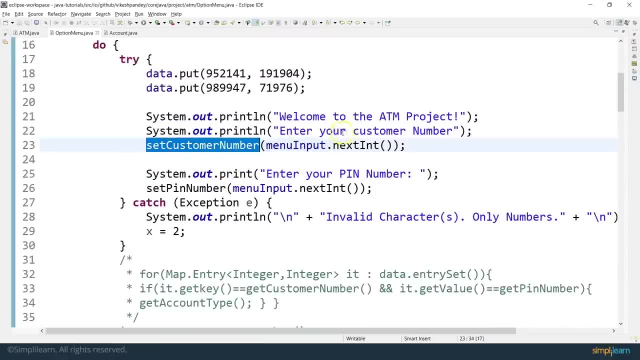 so whatever, in a customer number, the customer inputs, we pass that inside this particular method called set customer number. again i will come back to that. and once we have provided a valid customer number, then this method is going to ask you to enter a pin number, and remember i told you this is the customer number to the pin number mapping. so whatever. 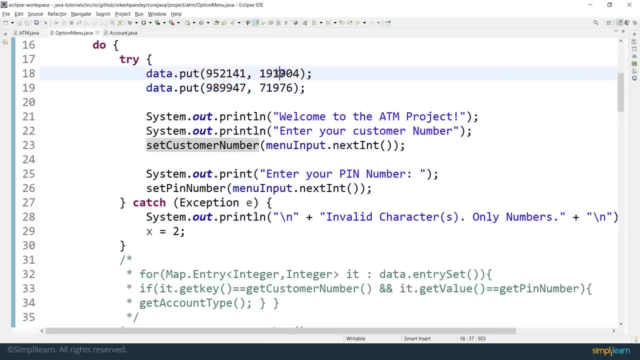 number you select from here, you will be providing the corresponding pin number and again, if you provide an invalid pin number, you will get an error. so that will all happen inside this try block and if you enter any invalid characters in the pin number or the atm customer number. 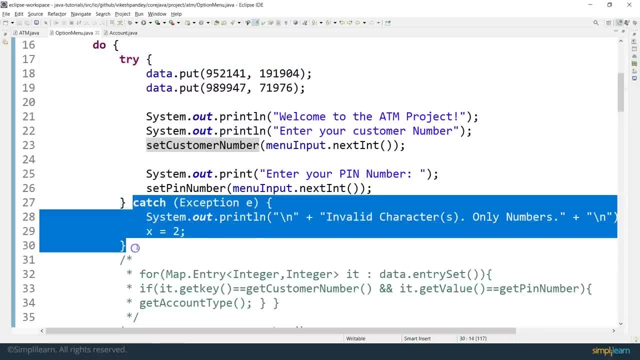 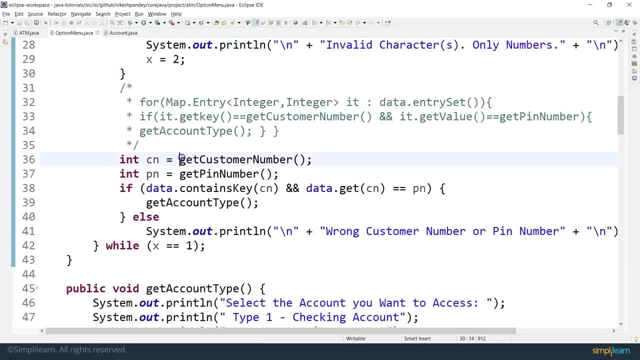 then you will get an exception which i am writing inside the catch block. this is all what we have seen so far. after the successful enter of the customer number and the pin number, i fetch those values from these two methods. again, i will talk about what these methods are doing. 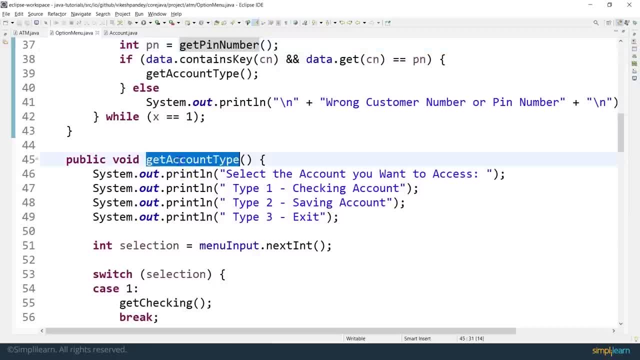 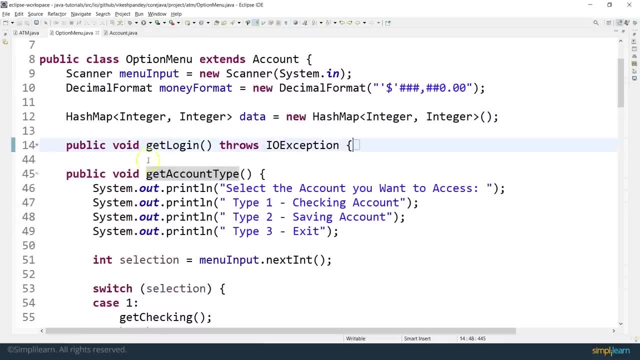 and again i'm doing some basic validation checks. but things get interesting in this method. so what we covered so far was the get login method. let me close this method here. so we covered the get login method. the second method which is defined in this particular class is the account type. 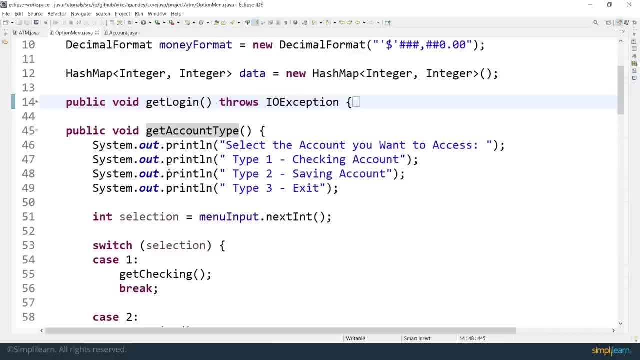 so here the we will ask the. once the customer has provided the customer number and the pin number, we will ask the customer to provide the account type. this application supports two different account types, which are checking account or a savings account. so whatever. so the customer has to. 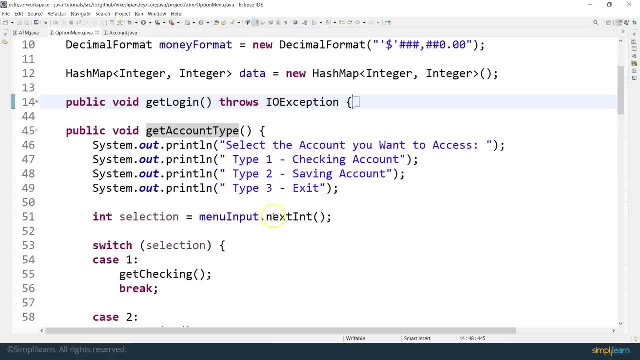 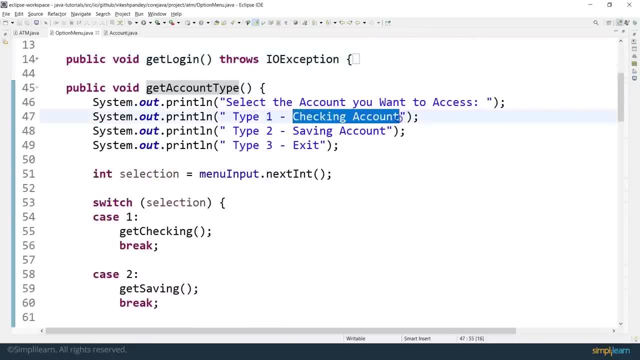 choose one of them. again, we will be taking the input from the command line using the scanner class and then i'm using a switch case. if the customer entered one, then i will execute some code for the checking account which is defined here in the case one. and if the customer entered, 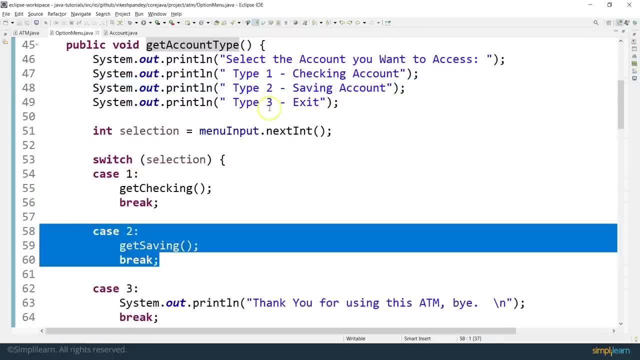 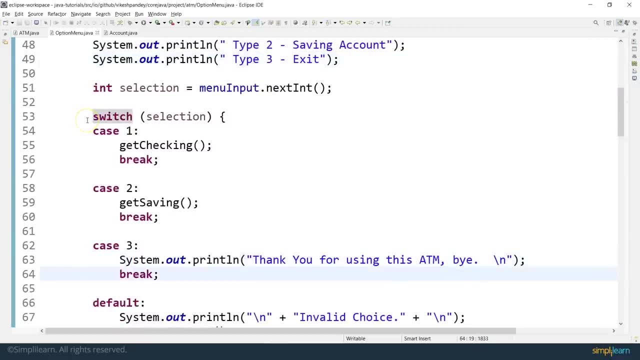 two, then the case two will be executed, and if the if it enters three, then i will exit the application by just printing assist out. so here i'm using the switch case construct to provide different options to the customer. there's also a default case specified here which says in: 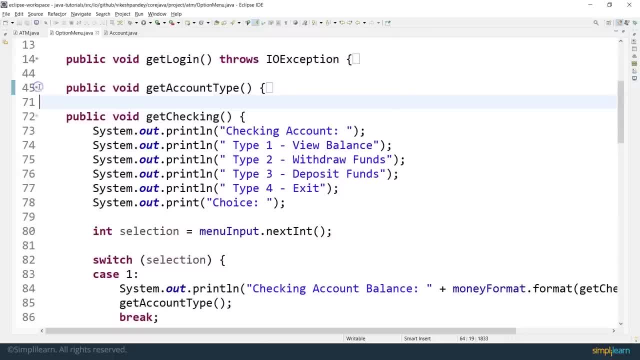 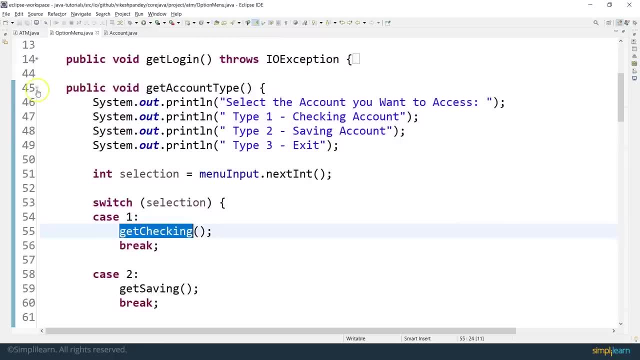 case two, that they have entered the same account type. and if they have entered their account type, then with the option one, we will ask the customer to type in the same account type. so this is a valid choice. so this is what is happening in the get account type method. the 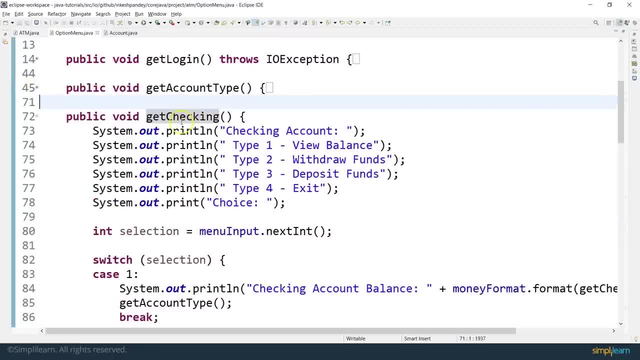 next method is: if the customer has used the option one, then we call the get checking method. so let's go to the get checking method, which is the next method which is defined in this particular class. so if the customer has selected a checking account, then we provide the following functionality: 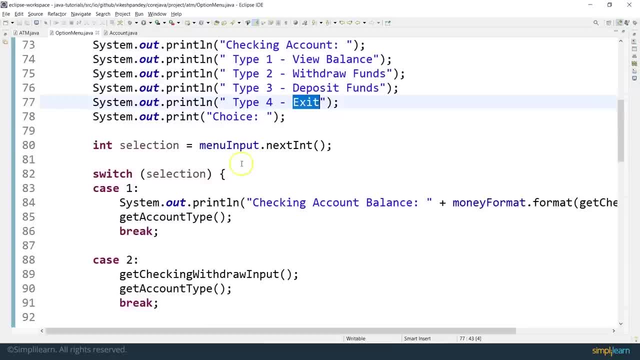 to the customer, which is the customer can view the balance using a switch case. here, based on the customer types- 1, 2, 3 or 4, the corresponding case block will be executed. for example, if the customer wants to view the balance, then this block will. 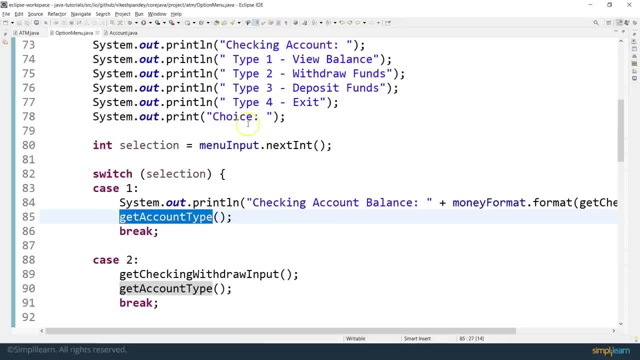 get executed and i call the get account type method. if the customer selects the 2 as the withdraw fund, then get checkings with withdraw input method gets called and then get account type gets called. similarly, if the customer enters 3, then we deposit the fund and for that also i 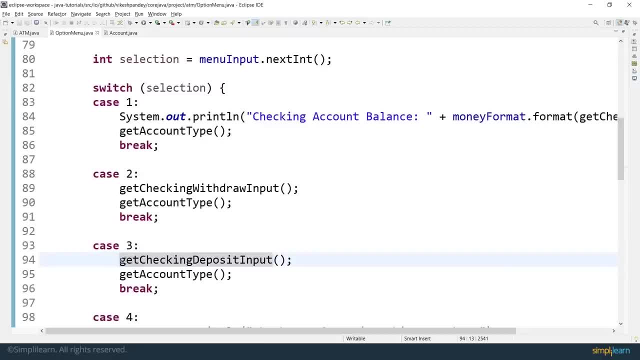 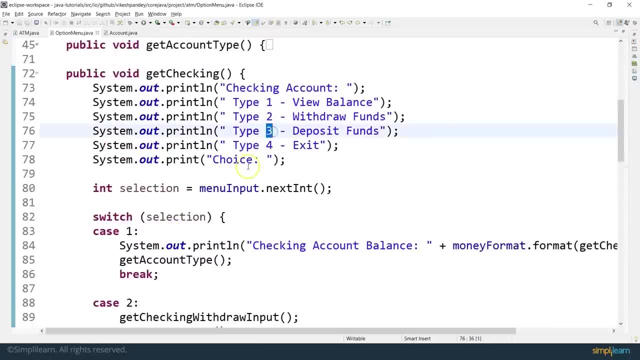 have defined a method. i will go to the definition of these methods as we go along, but right now we are just building the framework. so the get checking deposit input method will be called whenever the customer selects the option 3, and for option 4 we just exit the application. so this: 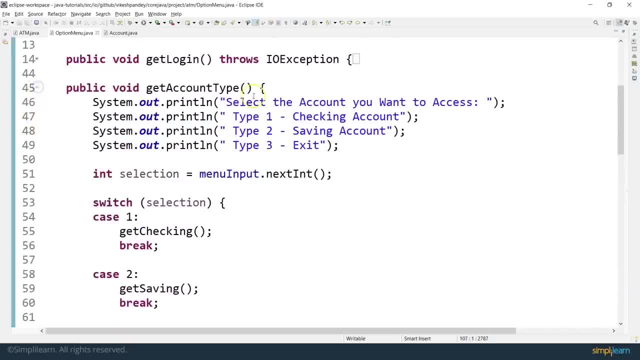 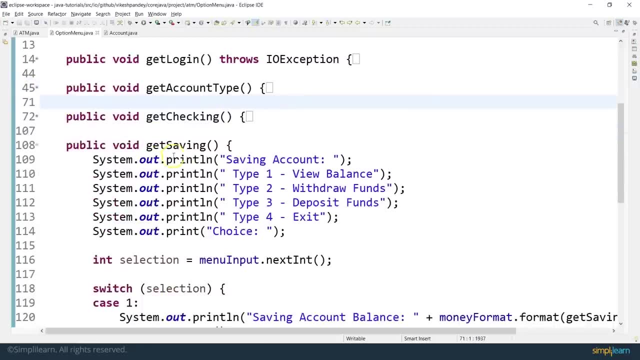 is what is happening in the get checking method now, if, from the account selection, if the customer selected second option, which was savings account, then we were calling get saving method. so this is where the get saving method is defined and again it is following the exact same format, as we saw. 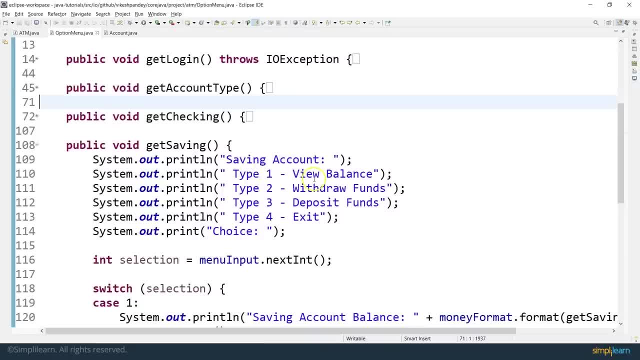 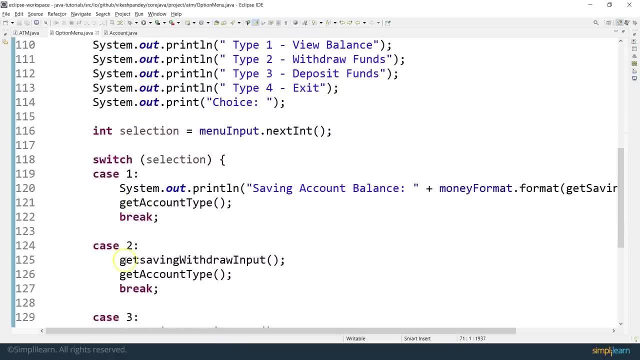 in the previous video. so this is where the get saving method is defined and again it is following the get checking method, where we present the following options like viewing balance, withdrawing the funds and depositing the funds in the savings account. and i have some methods defined here, for example, get saving withdraw input, get saving deposit input. so we define 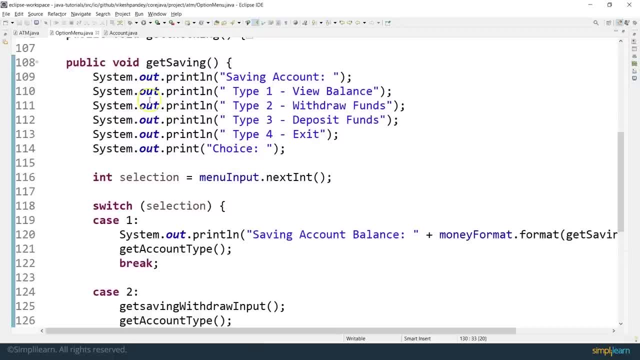 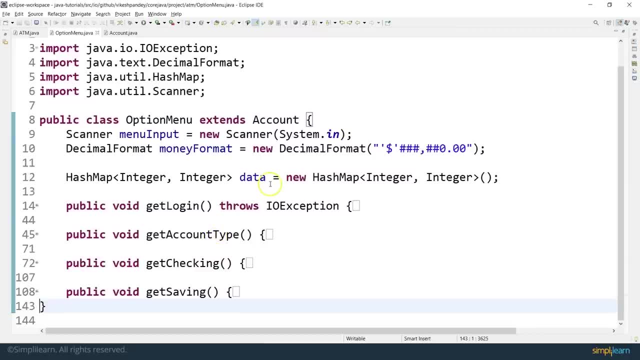 the switch case here, based on the customer's choices here, and that is what is happening in the get saving method. so let me close this method as well, and that's all what is defined inside the option menu class. so we ask the customer to enter the customer number, the pin number. 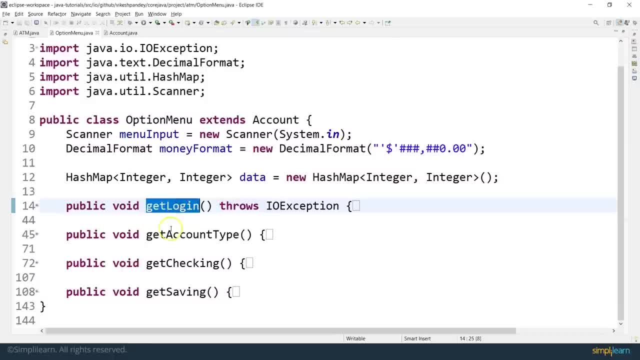 from this get login method. then, based on that, we provide the customer the options to choose the account type- whether they can choose the savings account or the checking account- and based on that, whatever account type they use, we call the get checking or get saving method and inside this, 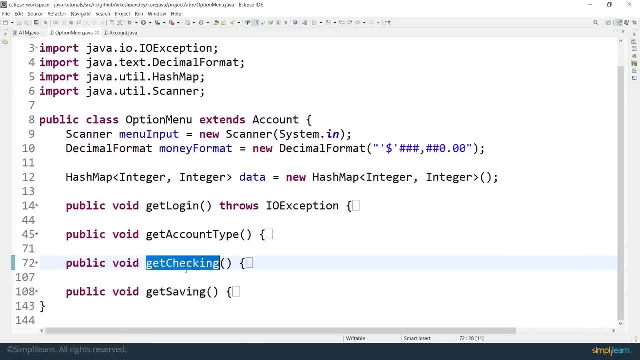 method. we provide the customer the other options to either withdraw the money, deposit the money or view the balance. that is what is happening inside this option menu class. now let's go to the account class and all the methods which we saw here will be provided a definition in the account class. you also see this option menu is extending the 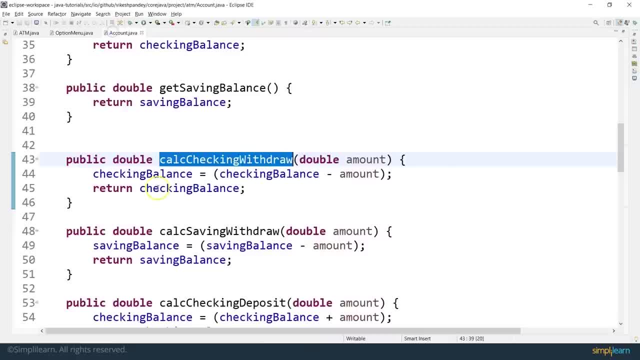 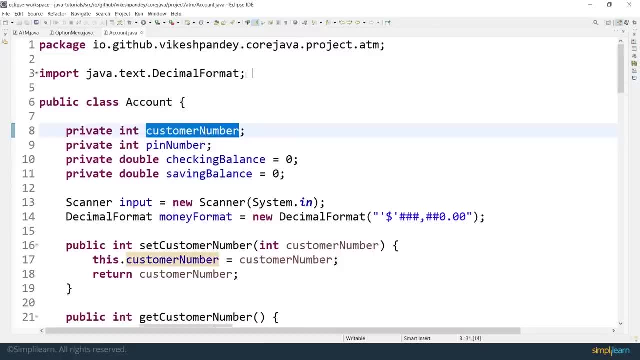 accounts class. so an inheritance concept is being used here. let's go to the account class now. so this is the account class where i have defined some private member variables like customer number. so now you will be familiar with the customer number, pin number which i just described, and also. 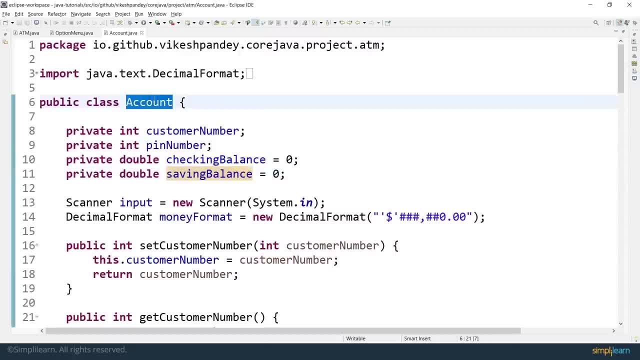 with the checking balance and the savings balance. you can also divide this account class into two child classes, where you have a savings account class and a checking account class, but for a room society i have kept it to one class. i'm initializing a scanner input which will be used. 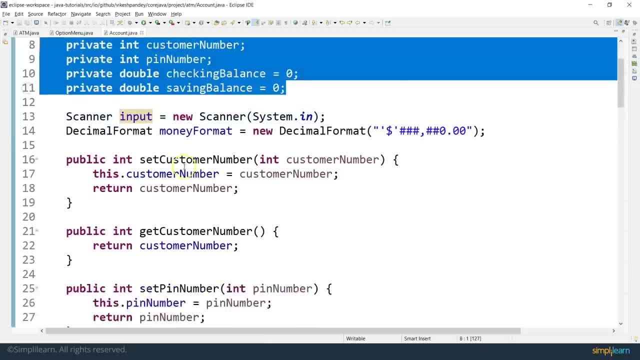 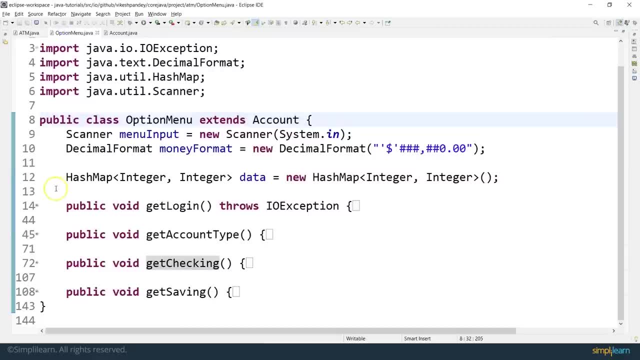 at multiple places. and then i have the setters and getters for these four member variables. so you see set customer number, get customer number. if you remember, this set customer number was called in the option menu class. if i go back to the get login, once we ask the customer to enter the 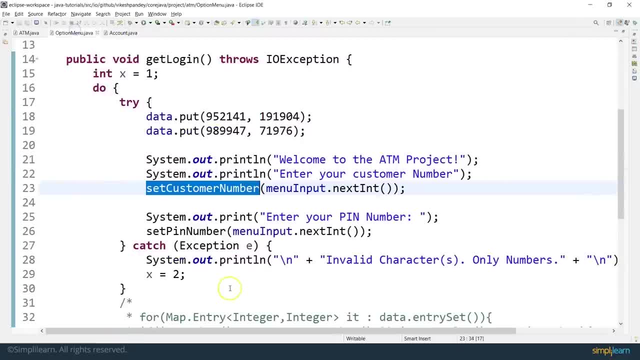 customer number. we call the set customer number, which gets called here similarly, we call the set pin number, which gets called here similarly. once we have said that, we then beautiful here and hit the write button again and we will see that the advanced program has one menu on the left and one set pm being a set 약간 number, which gets called here similarly, we call the set pin number, which gets called here similarly. once we have set that, we then allow the software to enter the business. and anyway, once we have caught survey, let us have a elimination in which we now have a solution. we 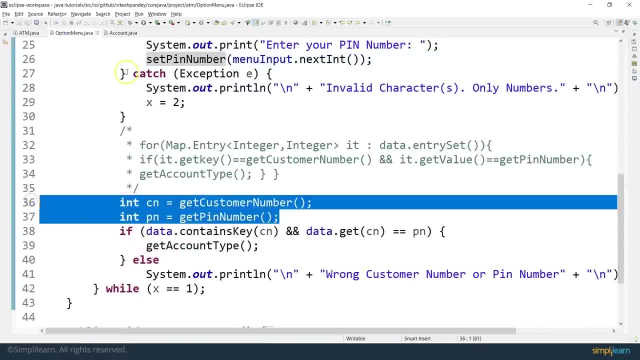 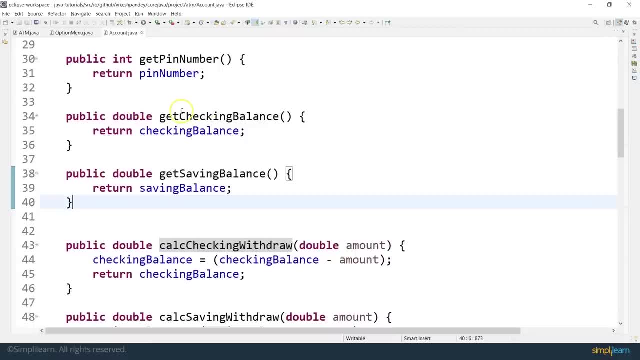 we were fetching the values using the get customer number and the get pin number, and that is that is also defined here in terms of the getters- get pin number and get customer number. Similarly, we also have the getters for the checking balance and the saving balance member variables. We do not 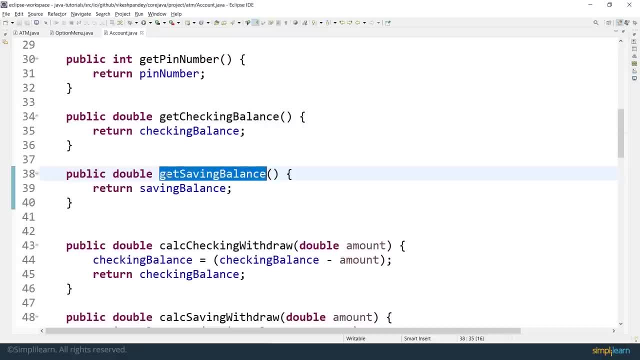 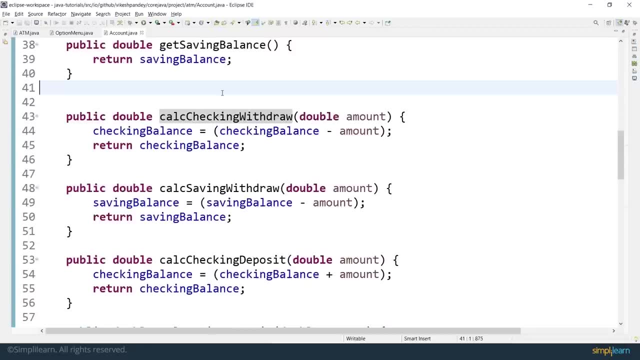 have the setters for them, because they are not technically setters, but we have to calculate the balance. It's not a simple setter where you can just return the value. So now let's look at some of the business functions of the account class. How do you deposit? How do you view the balance? 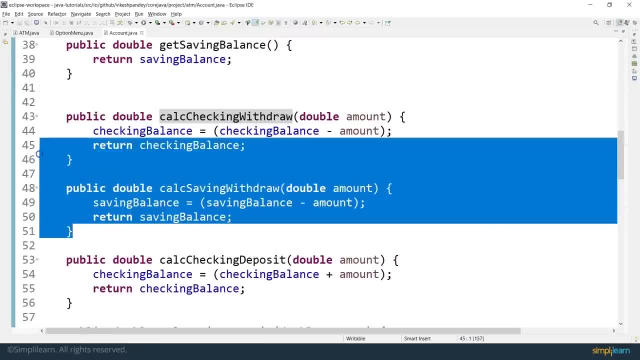 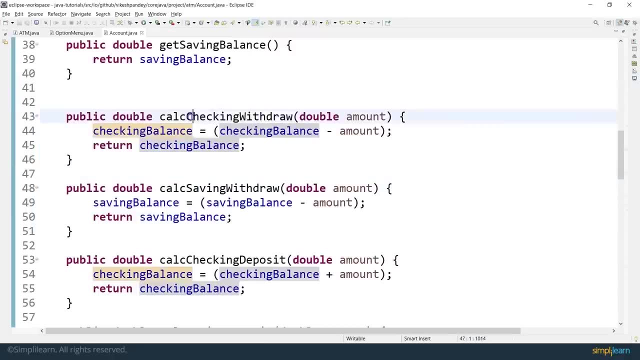 How do you withdraw the balance, etc. So you see these two methods which are specifically when the customer is trying to withdraw the money from their account, and these methods are basically called internally by other methods. So we will come to that. Let's see that. let's just understand. 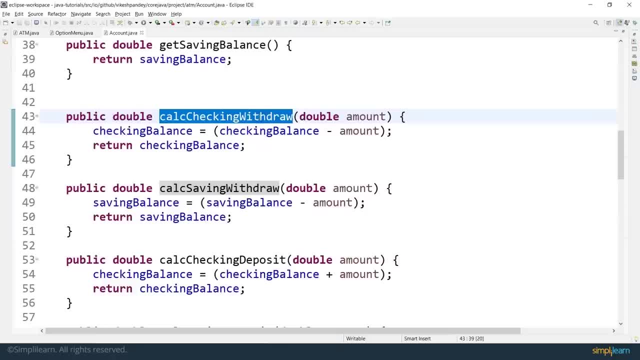 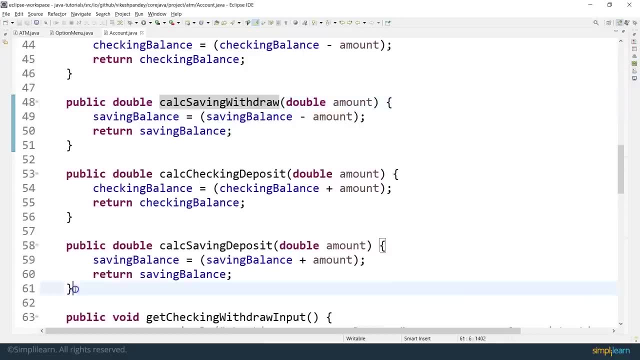 that we have two methods for calculating the withdrawable amount or executing the withdraw transaction for the checking account Account account and the withdraw transaction. So let's see how we can do that. So let's see how we can. and the savings account, Similarly, I have two more methods here which are calculating the 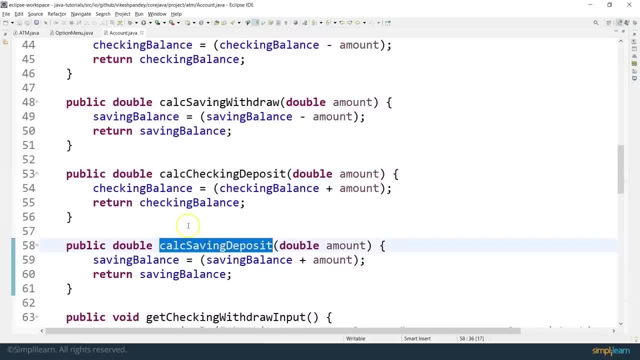 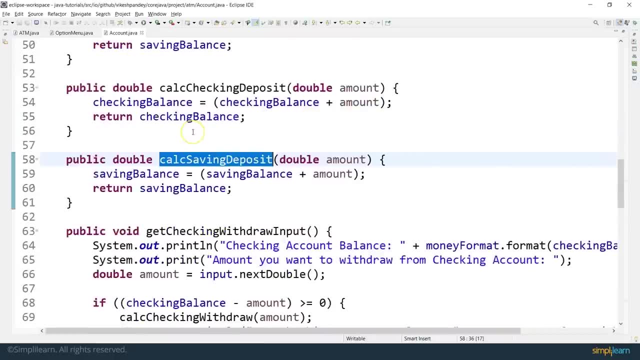 depositing for the checking account and calculating the depositing for the savings account. And then we get the bigger methods which are using these calculation methods. So I define four calculation methods so far: Calc checking withdraw, calc saving withdraw, calc checking deposit and calc. 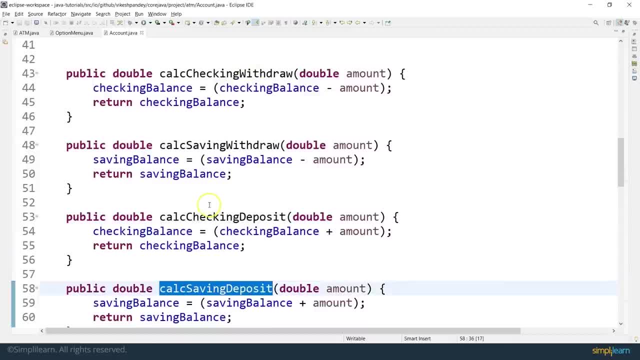 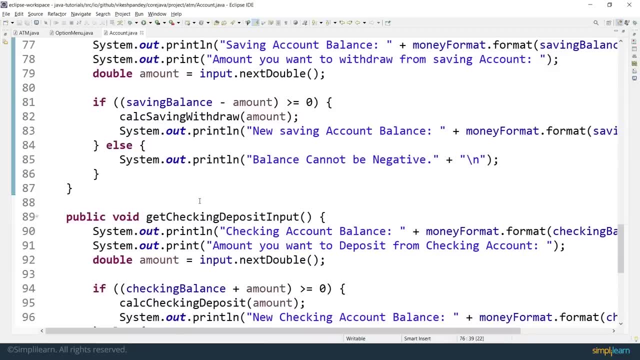 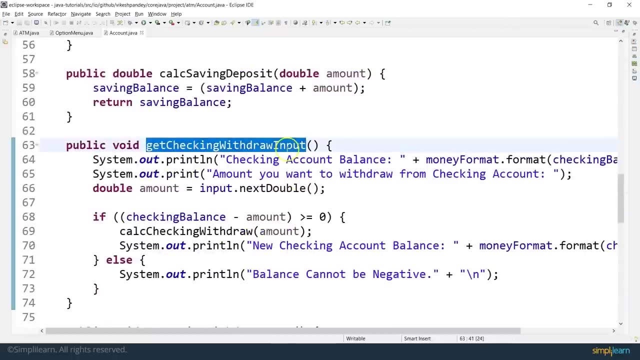 saving deposit, Basically withdrawing and deposit for both of the classes. And then we have these business functions called get checking withdraw input And get saving withdraw input, Get checking deposit input and get saving deposit input. So these getter methods are something which were being called from the option menu class, if you remember, If you go. 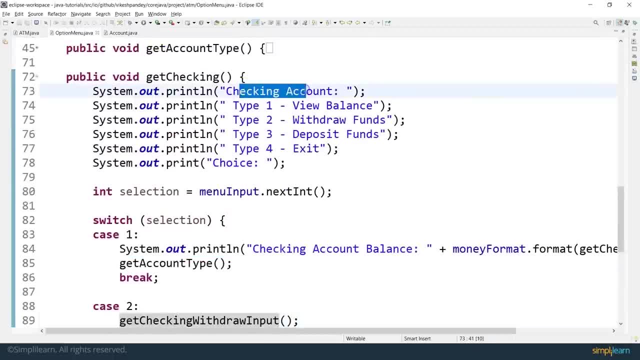 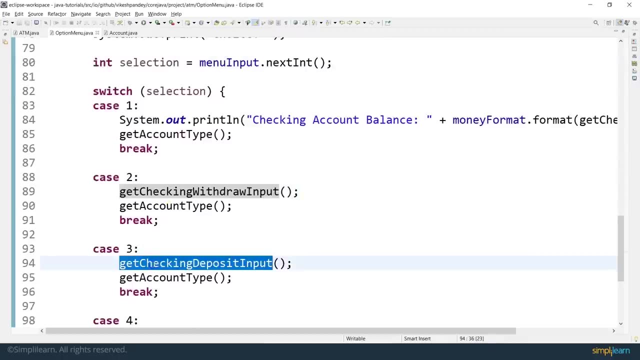 back to the option menu class and if you chose the checking account, you get these options. and let's say you chose option two, which was withdraw funds, or option three, which was deposit funds, Then the corresponding methods, which were being called, were get checking, withdraw input and get checking. 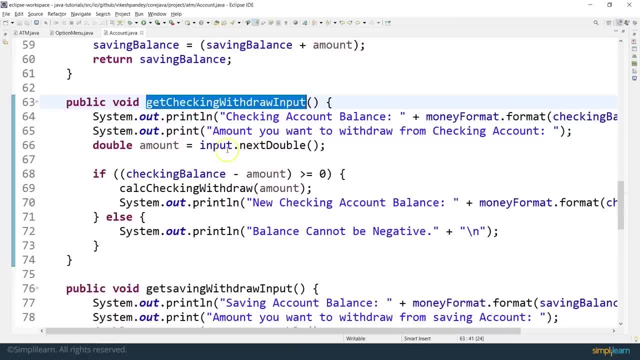 deposit input. And this is the exact same method: Get checking withdraw input and get checking deposit input. So if you see what is happening inside this particular method is couple of sysouts. Then we take the scanner input amount and we convert that amount to the double. After that we check if the 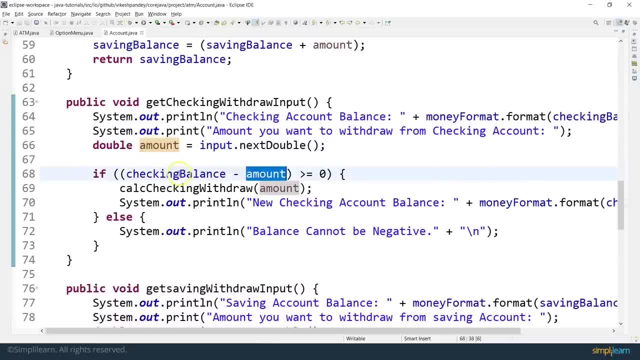 amount which the customer wants to withdraw is smaller than the checking balance or not. And I'm running this condition to check that If the amount is smaller than the checking balance, then we call the calc checking withdraw method, which was defined right here. Remember I told you that. 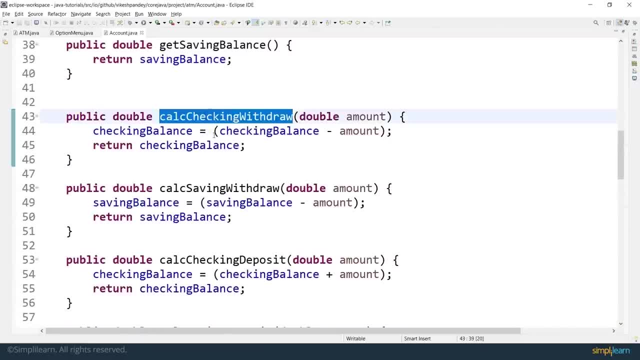 these four calc methods will be used and this is how they are used. So here I'm actually subtracting the value. So whatever amount the customer wants to withdraw, subtract that from the main balance and then return the new main balance. That's what you do, right? If you have thousand rupees and if 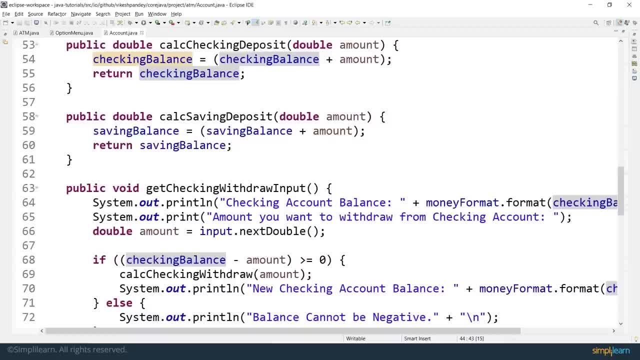 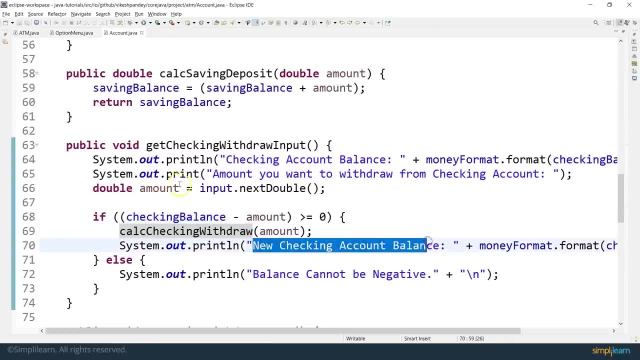 you want to withdraw 500, you subtract 500 from thousand and then you send back the remaining balance. So that is what is happening when we call this method and then we print the new checking balance. That is what is happening in the get checking- withdraw input method. Similarly, if you 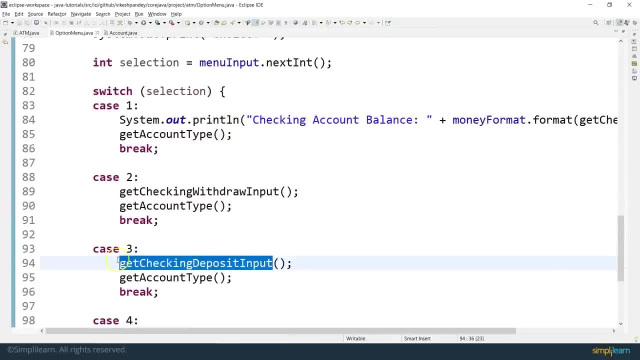 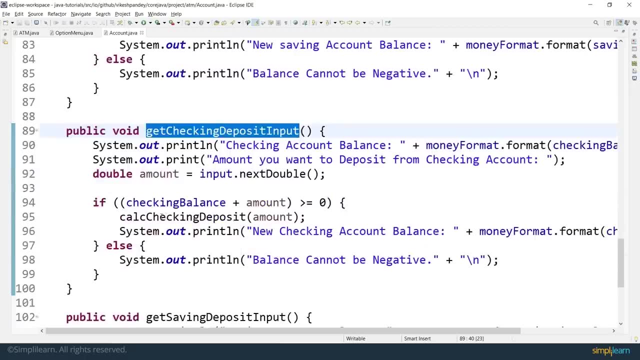 chose option three, which was depositing funds to the checking account. then get checking deposit input gets called and it is defined right here. Get checking deposit input and here, instead of subtraction, we are doing the addition. So here I'm again doing a condition: check that the current 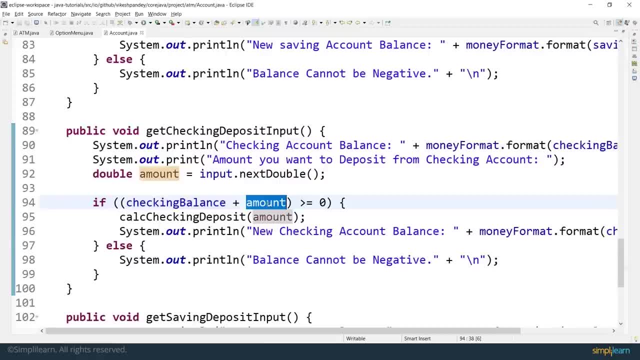 balance plus the new amount which has been supplied by the customer from the command line, the total customer entered an amount minus five thousand. I should not allow that. So that's the reason I'm putting this condition in place. and if the current balance plus the new amount which is supposed to 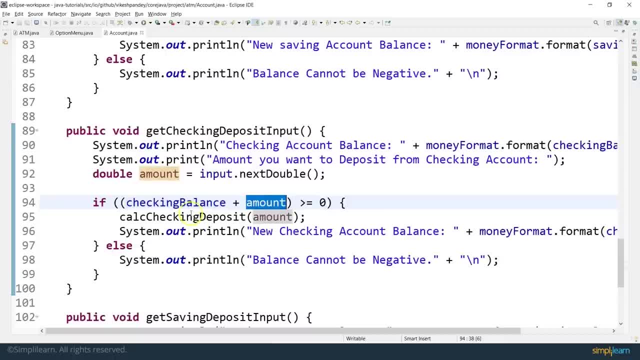 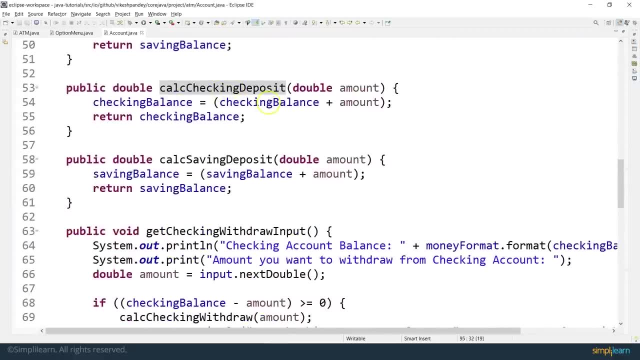 be deposited to the account. the sum of it is greater than zero, then call the calc checking deposit method. And this is where the calc checking deposit method is present and where I'm just doing present balance plus the new amount and returning the new balance. That's all which. 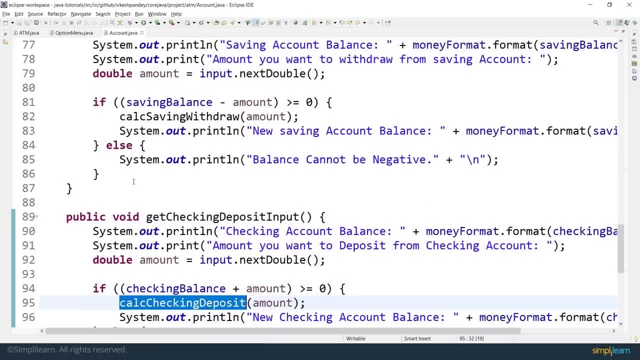 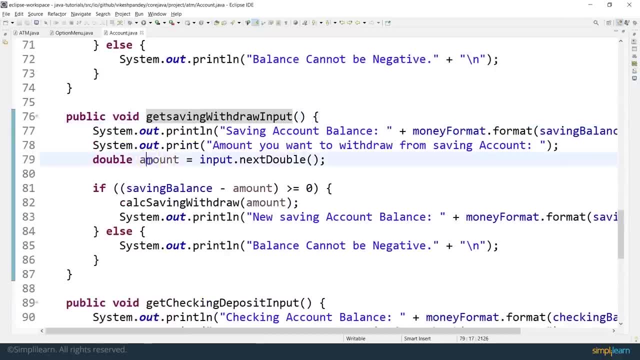 is being done here, And you will see exactly similar logic running for savings account as well If you look at the get saving withdraw input, which is used to withdraw money from the savings account. So I take the input from the command line and I run a condition. 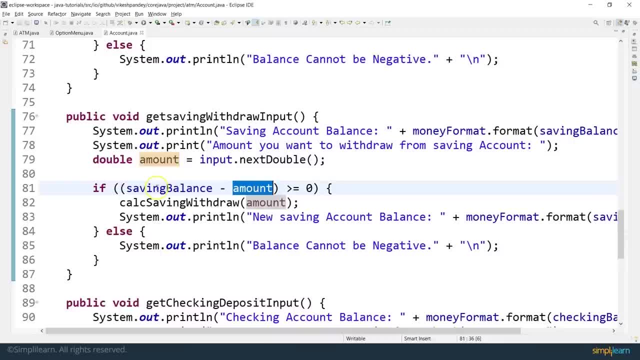 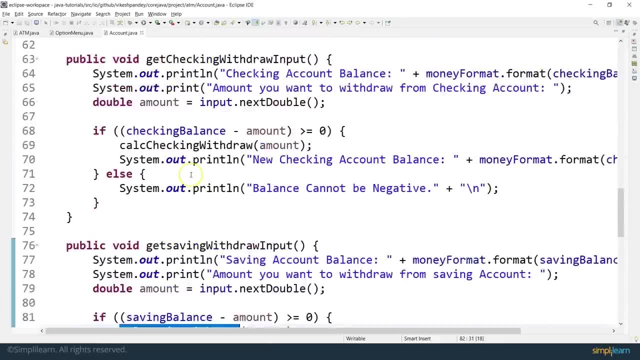 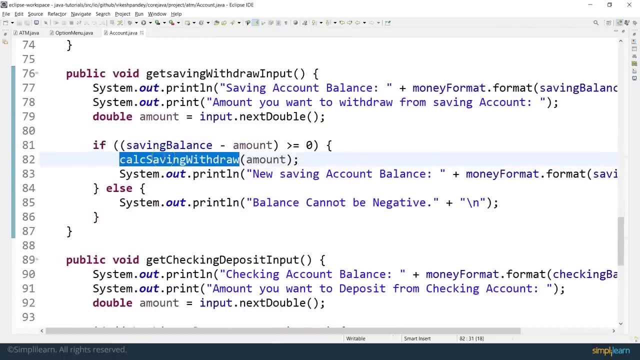 check that the amount which the customer wants to withdraw should be less than the current saving accounts balance. If yes, then call calc saving withdraw method, which is defined here, where I subtract the amount from the current balance and I return the new balance And similarly you will. 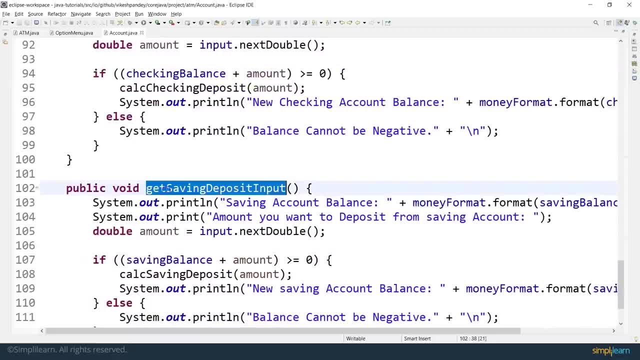 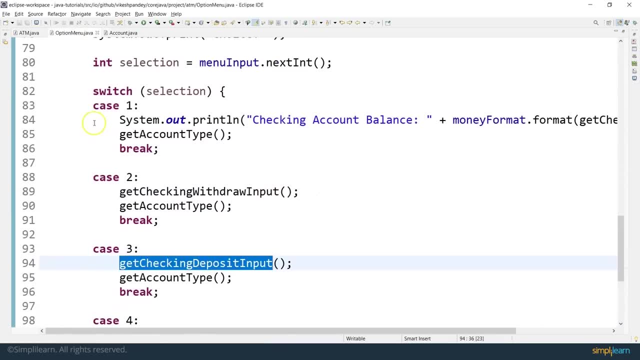 see the exact same functionality in the get saving deposit, where we add the money instead of subtracting the money, And this is all what is defined in the account class. So we talked about the option menu class, We talked about the account class and now we have the ATM class, which is the 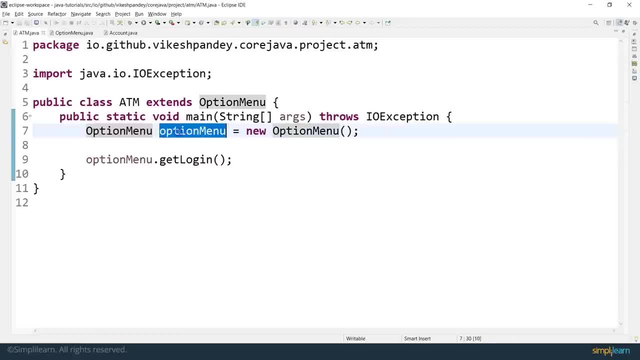 entry point which basically initializes the option menu class and calls the get login method. Remember, get login was the first method which asked you to provide the customer number and then get login called the method to choose the account type And the account type methods, then call the method to choose the option to withdraw deposit or exit. 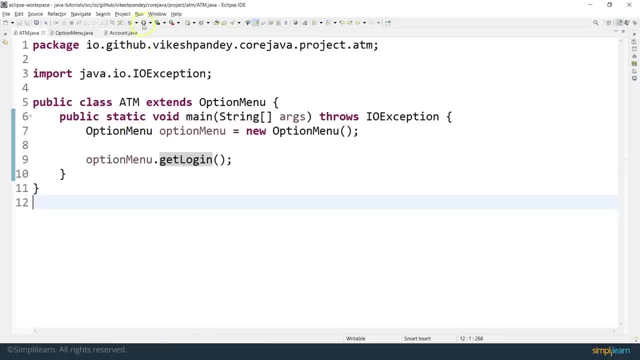 So now we have built a fair understanding of what is happening in this application, So let's run this application. So I just ran this application and let me bring the console here. It's first asking for a customer number. So I will go to the option menu class and I will pick up one of the customer. 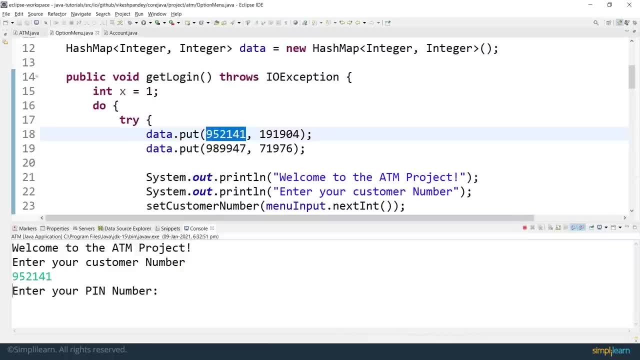 number which I have hard coded here. So I will provide that customer number and hit enter. Then it asks me for the pin number. So remember you have to provide the correct pin number corresponding to the customer number. So I'm taking this pin number, just copying it and pasting. 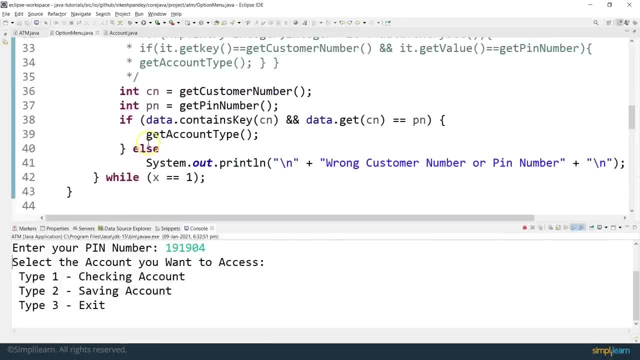 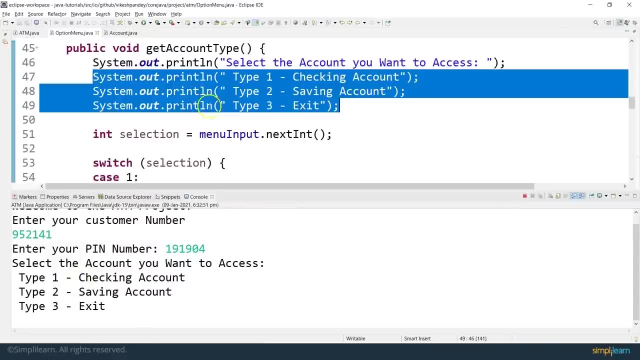 it here. Then this whole code got executed and then it called the get account type, and the get account type method provided you with these options which you see here on the screen. So, based on what you select, the case block will get executed. and let's say, I want to go for a. 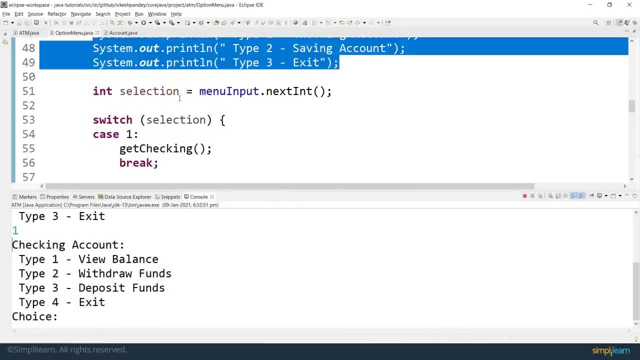 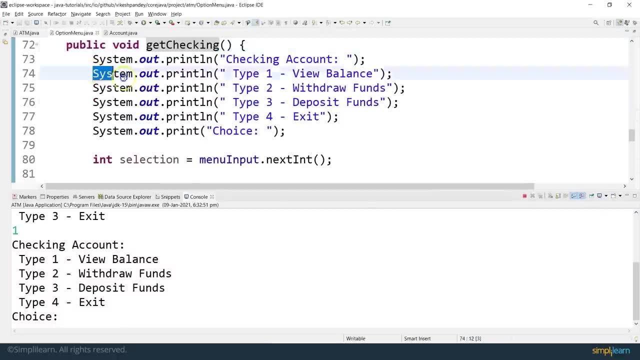 checking account. So I press 1 and I hit enter. Once you select the checking account, the case 1 gets selected and it calls the get checking method. and the get checking method again provides you with another menu to withdraw, view, view, withdraw or deposit or exit. So let's say: 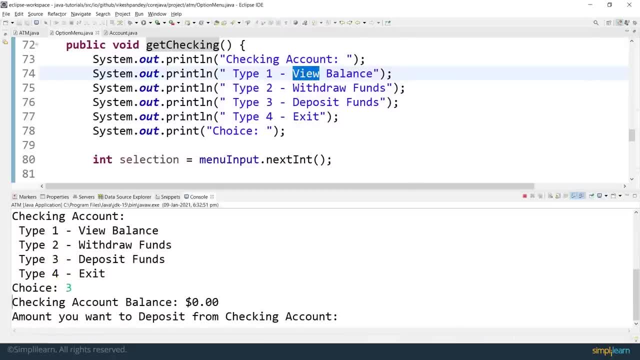 I want to deposit funds, So I press 3 and hit enter. It says the current balance is 0 and enter the amount you want to deposit. Let's say I want to deposit 500 and I hit enter. You get the message saying the new checking account balance is 500 and you have successfully deposited the money. 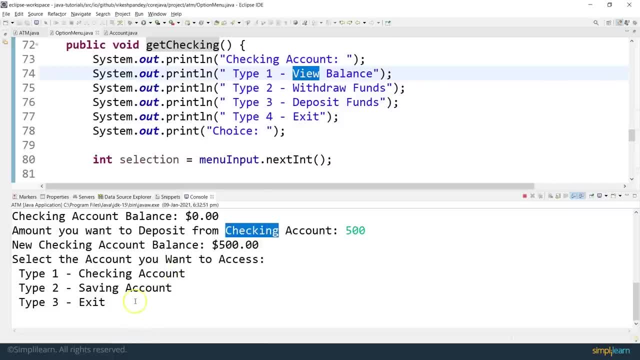 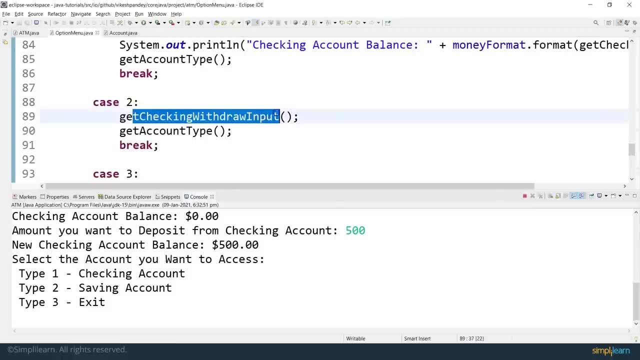 and that is what I did for the checking account. Now let's try to withdraw something from the checking account So you again get back the same option. because inside the get checking method we call the once we have successfully done the business operation, we again call the account type method to display the menu again to the user. So let's see again. 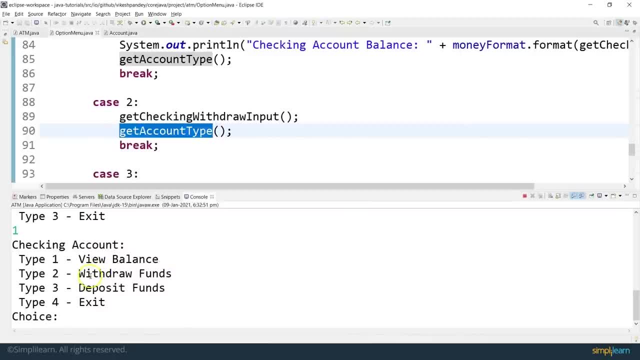 select the checking account class and this time I want to withdraw the funds. Remember, I've added 500 there. So let's say I want to withdraw. so I choose the option 2 as the choice. current balance is 500 and it's asking me the amount you want to withdraw from the checking account. So I enter. 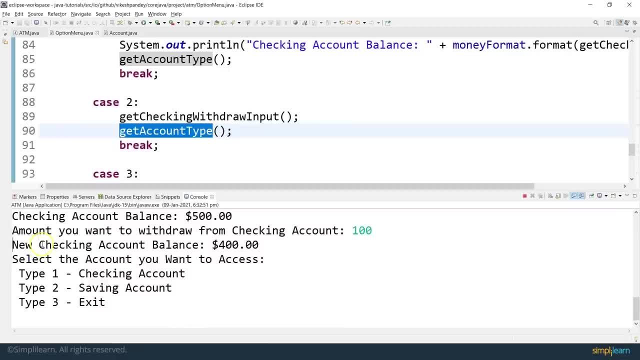 let's say 100, and I hit enter that the new checking account balance becomes 400. So the 100 got subtracted from the 500 and the new balance is shown to your screen. You can do exactly the same thing for the savings account. 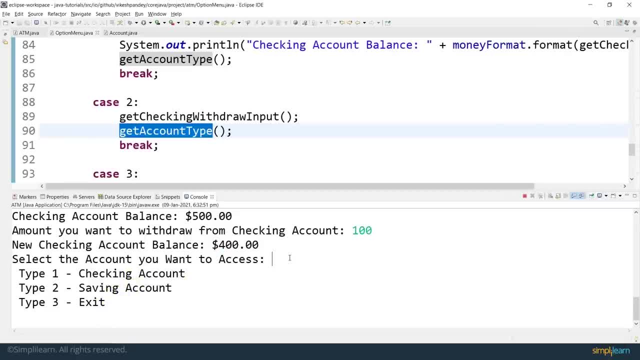 as well. and let's also run a negative condition. So I again select the checking account and I want to withdraw the funds, So I choose the option 2.. Current balance is 400 and I would like to withdraw 1000. What happens If you do that? we get a message saying balance cannot be negative. 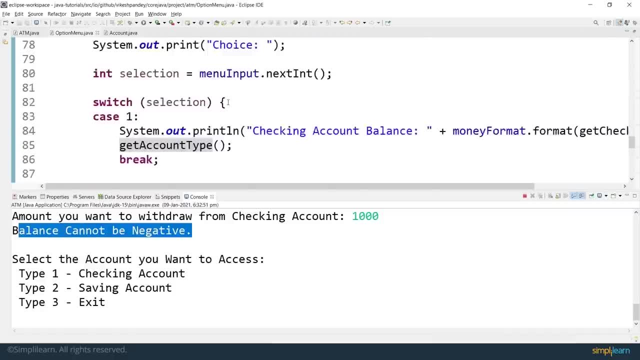 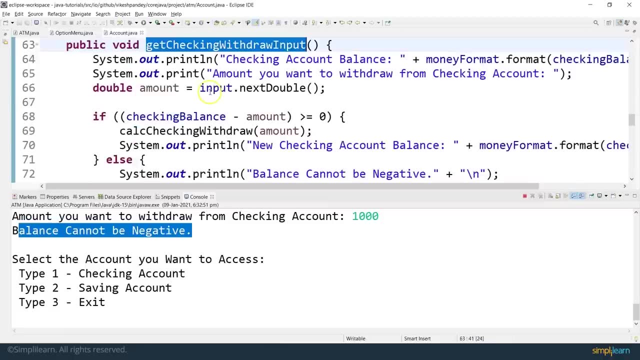 and this is coming from the calc checking method which is defined here. So what is happening? that I wanted to withdraw the funds from the checking account and here get checking withdraw input called Here. this condition was checked, So the checking balance was 400 and the amount I wanted. 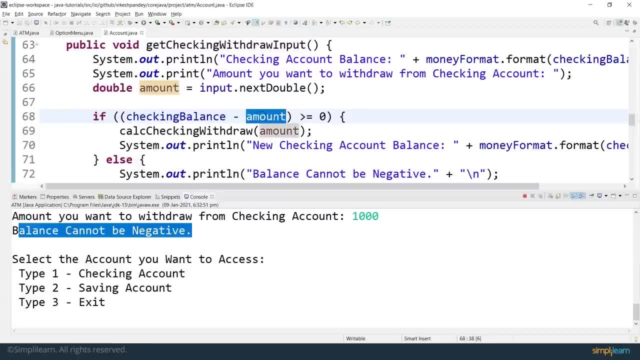 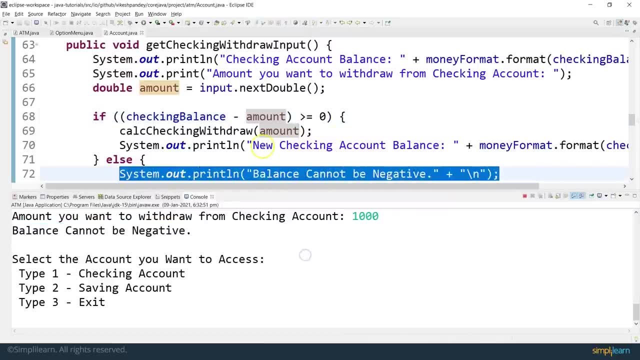 to withdraw was 1000. So 400 minus 1000 is not greater than equal to 0. So it jumped into the else block and it said: balance cannot be negative. So this is how you can also build some error conditions in your code. 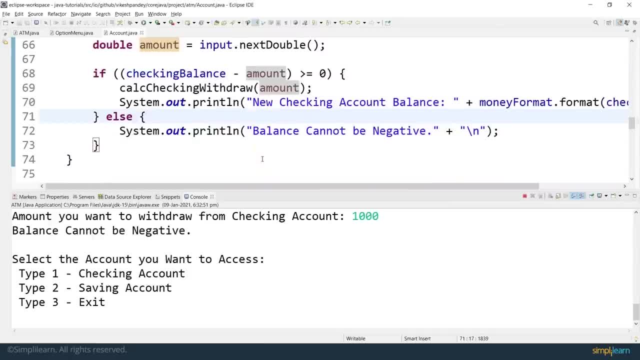 Which are mandatory and which should be built. otherwise your application will have a lot of bugs. We can also exit the application. So if you just type 3 and hit enter, you will exit from the application and it will come in. it will again call the login method where it will again ask you to. 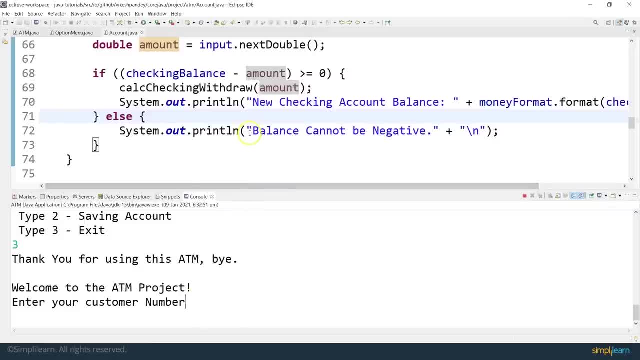 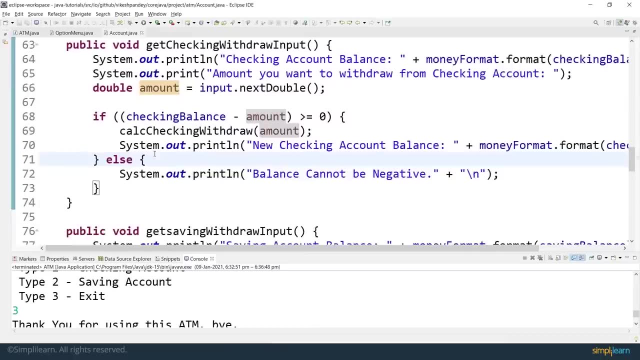 enter the customer number. So this is how you can run this application, and this is. this was a simple use case for you to show how you can use the different object-oriented concepts like classes, objects, methods, setters, getters, switch, case, etc. to build the application with the. 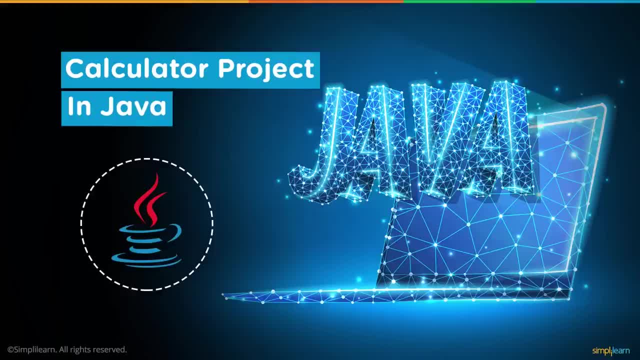 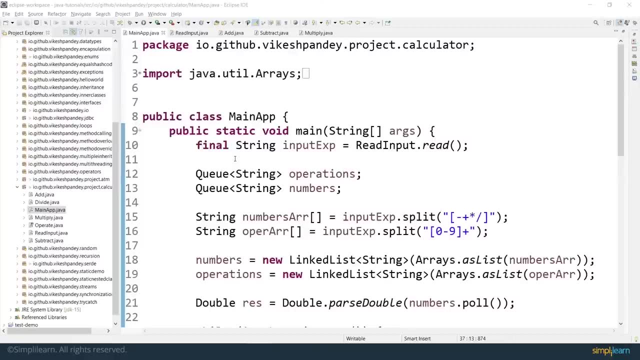 correct business logic. Let's get started with walking through a core java project using all the different oops concept we have learned so far. So in this example we are going to have a look at a calculator application, and this calculator application supports primarily four different operations. 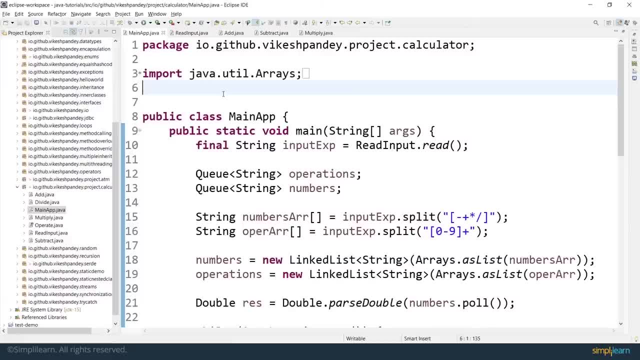 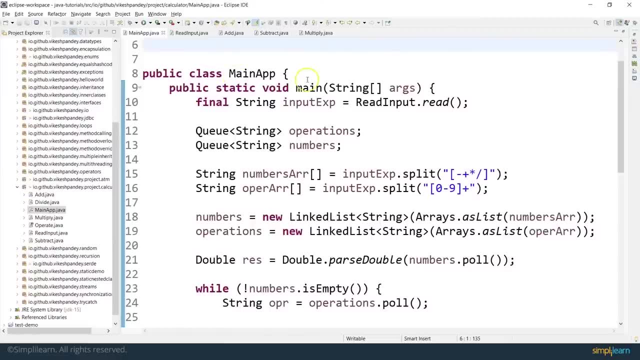 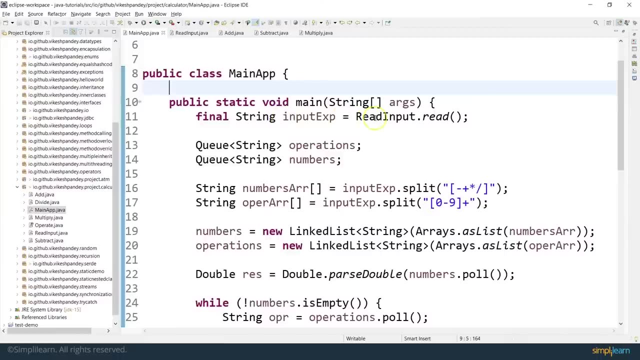 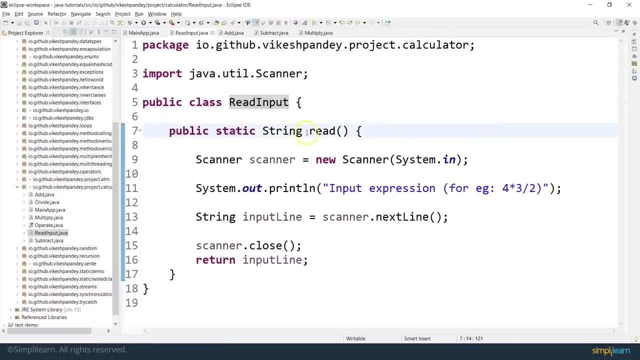 like addition, subtraction, multiplication and division. So let's see how do we build that app. So in front of me right now is open the main class. So I have a main app class here which is a main class. So we are going to add a public static void main method and the first thing we see is a read input class which is calling a read method. So if you go to the read input class, it has a simple static method here which is the read method, and it is using the scanner class. If you remember, I talked about the scanner class which is used to take inputs from the command line, from the user. So we initialize the scanner class and we start taking the inputs and whatever the user inputs in terms of the expression, let's say the user entered 4.0.0.0.0.0.0.0.0.0.0.0.0.0.0.0.0.0.0.0.0.0.0.0.0.0.0.0.0.0.0.0.0.0.0.0.0.0.0.0.0.0.0.0.0.0.0.0.0.0.0.0.0.0.0.. 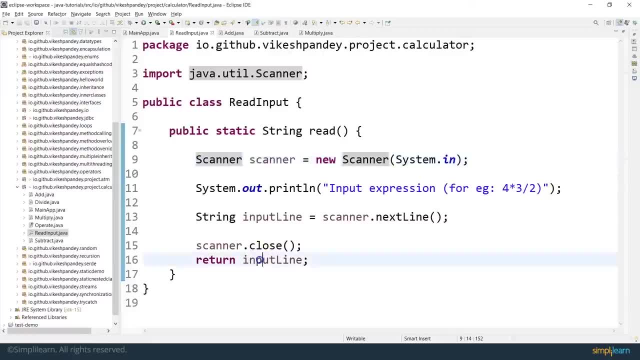 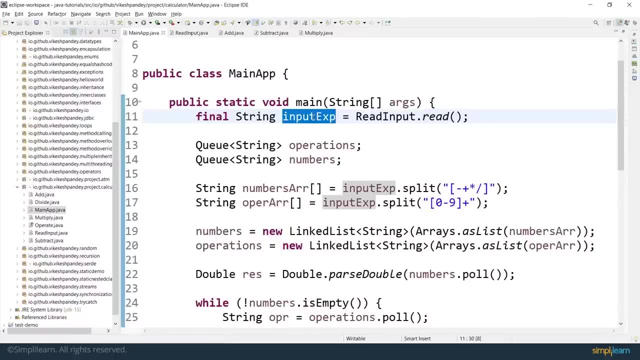 plus 5 or whatever. that whole expression gets sent back into this input line as a string and that comes back here in the input expression. once we have captured the input expression, the next thing we do is divide the input expression in the numbers and the operators. basically, an expression would be either something like 4 plus 5 into 3 divided by 2, let's say. let's. 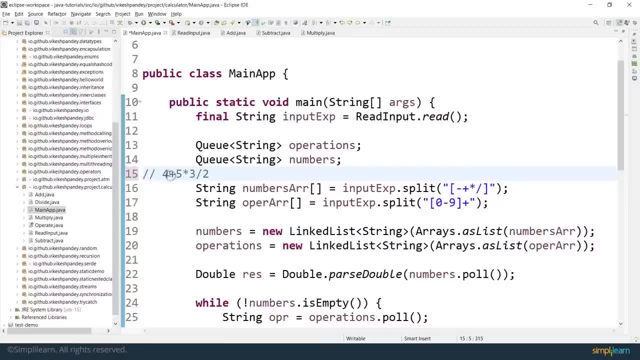 the user entered this expression, so this has either numbers or operators. so that's what we are doing here. we are using the split method of the string api, the string class, basically- and this split method is going to split the numbers and operators into two different string arrays. and here i'm providing the split expression that split at every time you encounter one of. 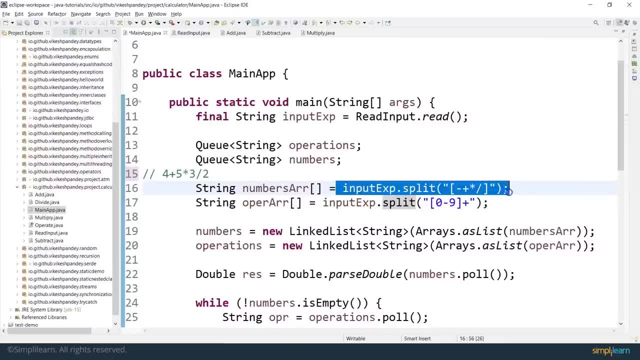 these symbols. so this: when you execute this particular statement, it is going to return a numbers array which will be created based on this expression. so you will get an array with 4, 5, 3 and 2, and similarly, in the operator array, you are going to split or pick out the elements every time you receive a number. so 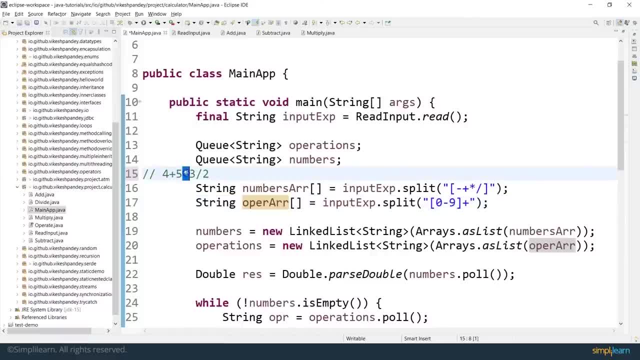 this operator array is going to hold this plus sign, this multiply sign and this divide sign. hope you get the understanding that we are just splitting the whole expression into two different arrays, where first array is holding only the numbers and no mathematical: 2, 1, 1. 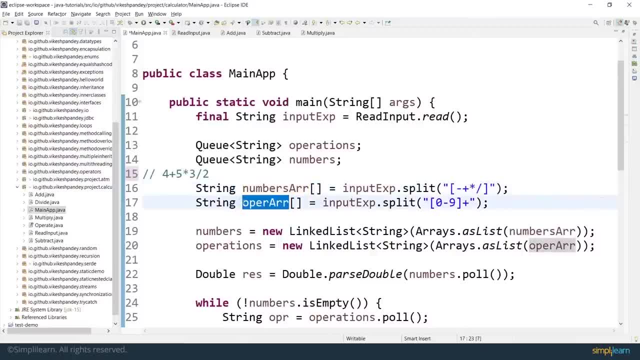 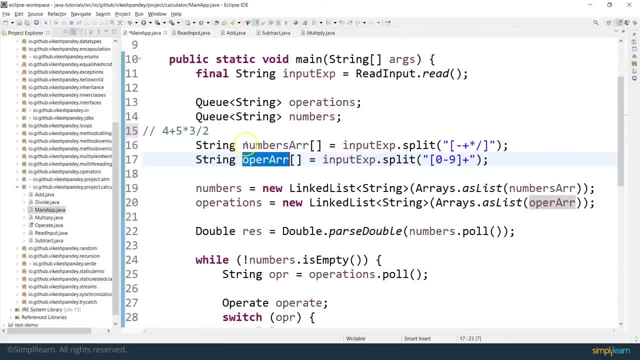 expressions. and second array is just holding the mathematical operators and no numbers, and we'll see why we need to do that in the upcoming lines. once i've created the string array, i just want to store or convert these string arrays into a queue. so i convert this array into a list by calling the. 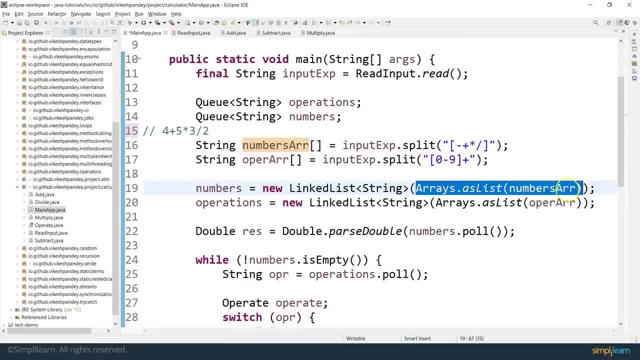 array dot as list. so this expression is going to return a list, and then i'm going to convert this normal list into a linked list and then going to store this linked list into the queue of numbers. and i'm going to do exactly the same thing for the operator array as well, converting this into 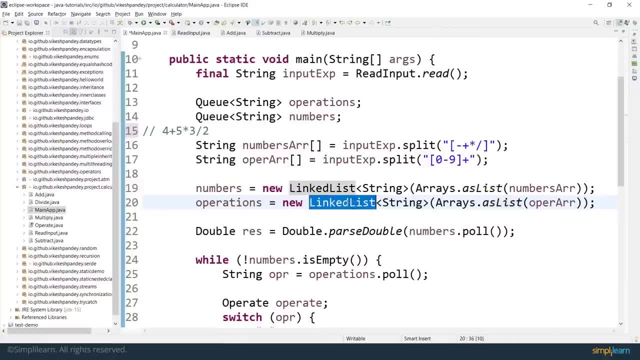 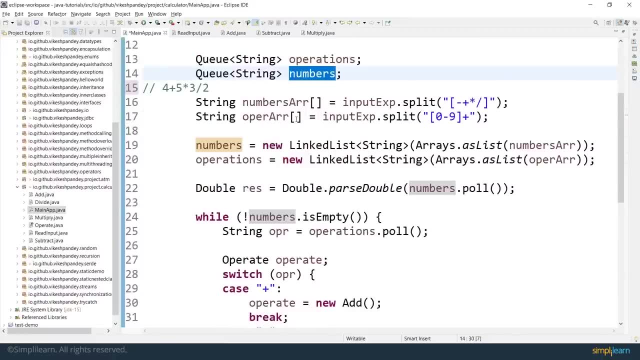 a generic list, converting that generic list into a linked list and then storing this linked list as a queue. so i have an operators queue and i have a numbers queue. both of them have been stored into a queue now, and then i'm using the poll method. if you remember, the poll method of the queue is: 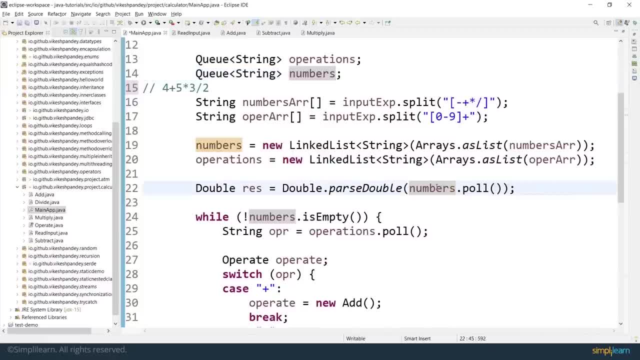 used when you want to fetch the first front element, the head element of the queue. so whichever element is sitting at the head of the queue will be taken out the moment you call. call the poll method. so i fetch the first number from the numbers queue. so in this case four will be fetched here in this variable and after. 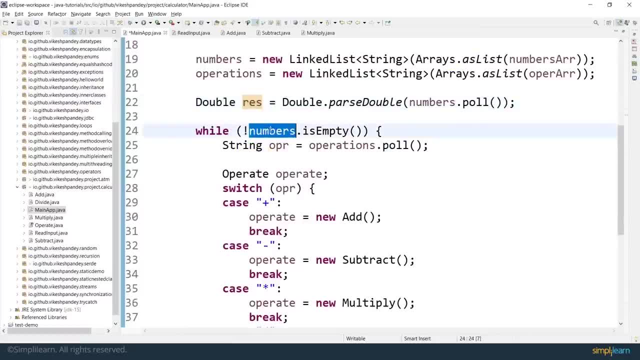 that i run a loop on the numbers queue and i'm going to run this particular loop till this particular queue is not empty, if you see there's a negation here. so i'm going to pick up numbers one by one from this numbers queue till the number queue becomes empty and inside the loop i do the exact same poll operation for the. 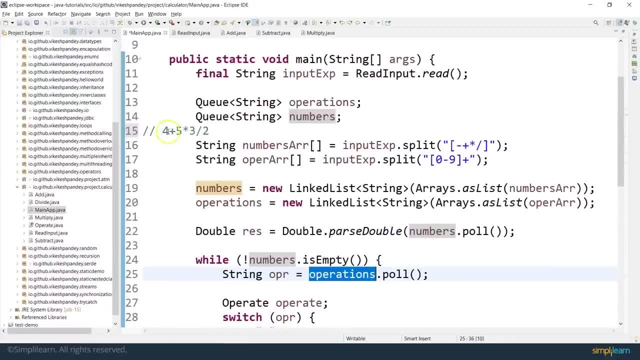 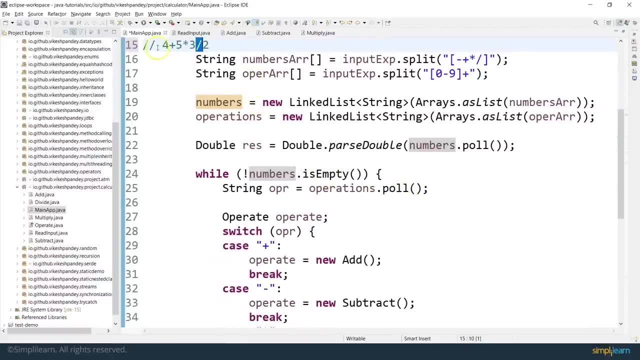 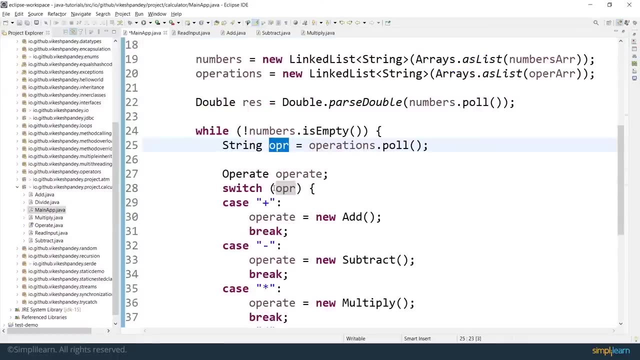 operations queue. so this operations queue is holding all these mathematical operations like plus, star and divide, so i'm going to pick the head of it. so in this case, plus will be picked up and will be stored in this variable called opr, and then i'm going to run a switch case on this opr. 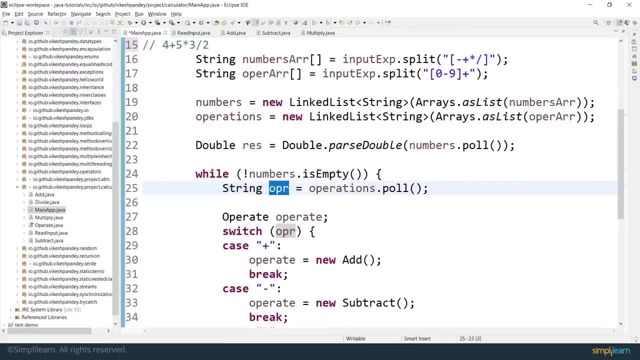 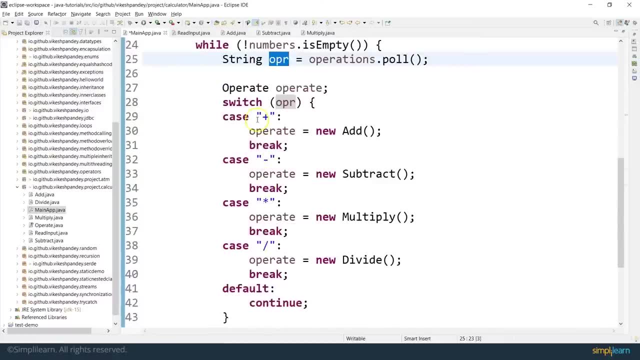 basically, as i told you, in this particular calculator application we are supporting four operations, which are addition, subtraction, multiplication and division. so i define a case for each of the mathematical expression. so you see there are four different cases here and for each case i'm initializing a class if it's a plus sign. then i'm initializing the add class if it's a. 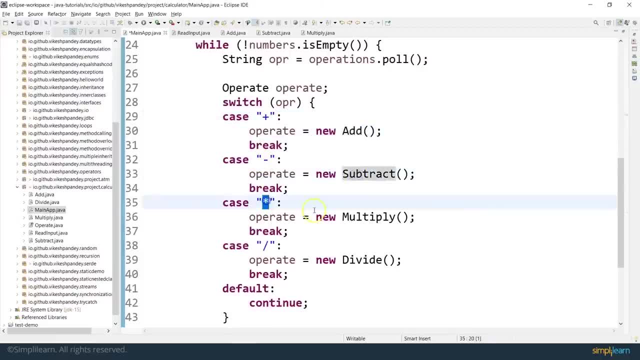 minus sign, then i'm initializing the subtract class. for multiplication, i have a class called divide, and for division, i have a class called divide. let's have a look at what these classes are containing. so if i go to the add class, first of all it is implementing an interface called 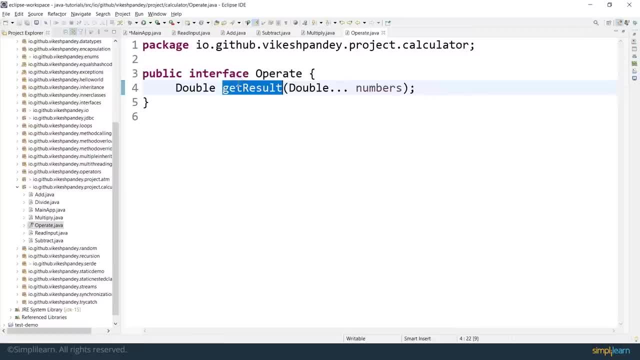 operate, and this operate interface has just a single method called get results, which is accepting a variable argument array. if you remember, i told you that you can also use a var arg array. this is called a var arg expression. this means that this numbers will be an array of arbitrary length. it 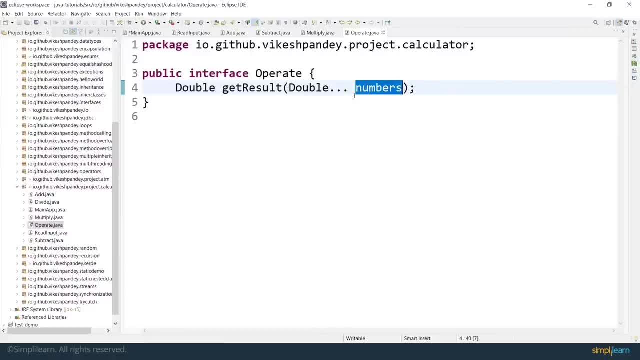 can be a one element array, or it can be a one element array, or it can be a one element array, it can be a two element array, it can be a four element array, or whatever you supply, but it is still going to be a fixed length array. but the length is going to be dependent upon how much. 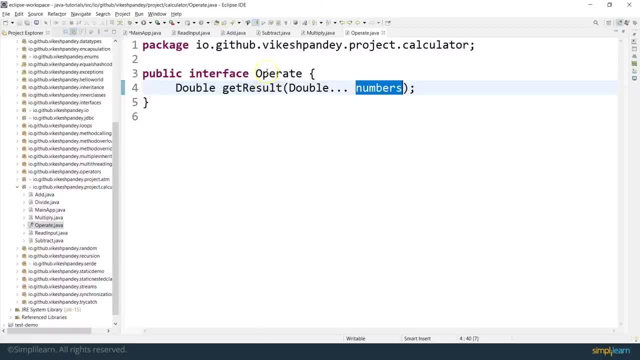 argument you supply to this particular method. so that is what this interface operate is doing. it just has one method declared, which is called get result, which is accepting an array of numbers. so if the add class is implementing the operate interface, then it has to override the get result. 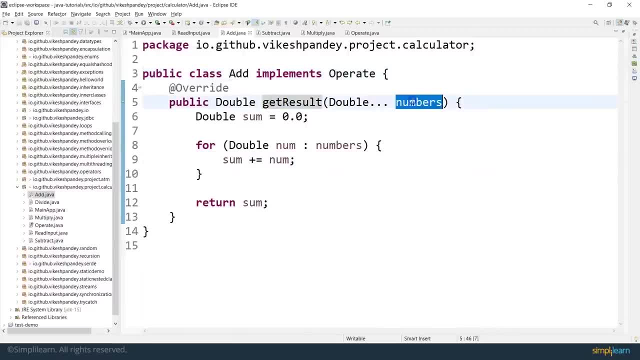 method- and here it is just doing a summation of all the numbers- which is accepting an array of numbers which have been supplied. so if you supply four numbers, it is just going to add up those four numbers and return the sum. and the exact same kind of logic, or similar logic, will be seen in other 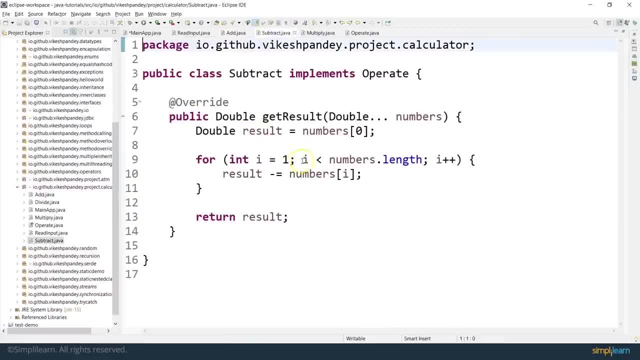 operate classes. so if i go to the subtract class, it runs the exact same operation but it subtracts the values. if i go to the multiply class, it is also implementing the operate interface and in the get result it is just multiplying all the values. similarly, in the divide class it is also implementing 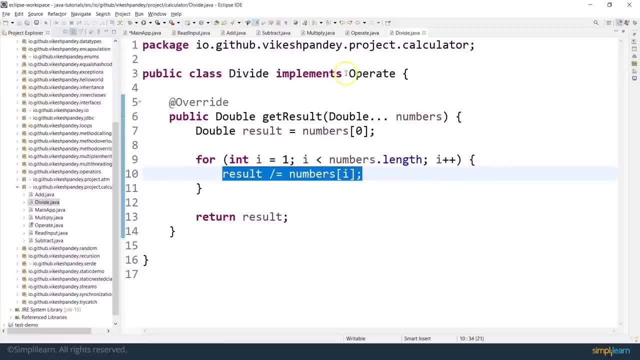 the operate interface dividing all the numbers one by one. so it's doing pretty much the same thing in terms of the expression and the logic. the only difference is whether you are using an add operation or a subtract, or multiply or a divide. so we have checked all these classes and the operate interface as 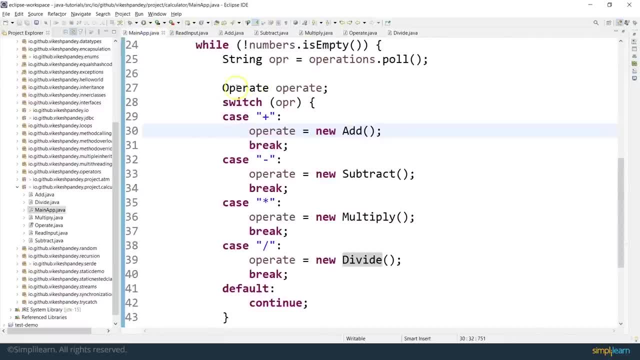 well, and let's go back to the main app now. now you also see that i've defined a reference of operate here and each of the switch case block i'm assigning the object type to this interface reference. so i'm using the concept of dynamic binding which we talked about when we talked 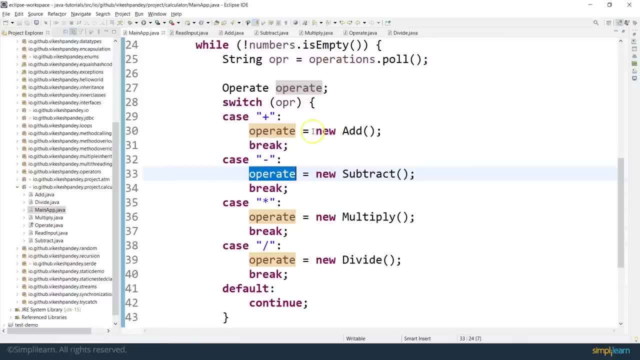 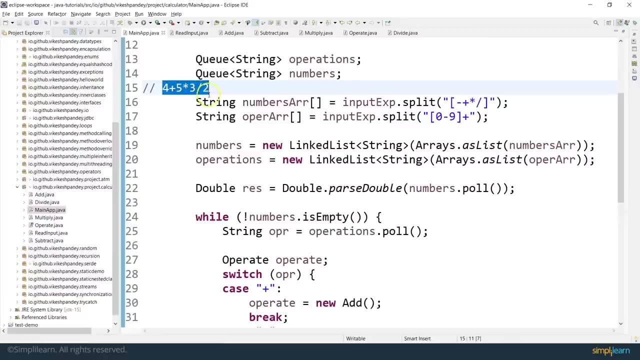 about interfaces that we can also do dynamic binding, where we can assign an object to an interface type and the object type will depend upon the expression. so once we have filled that based on the case, while filtering out this expression and picking up plus star and divide sequentially, then we go to the next line after outside the switch case block, which is to pick. 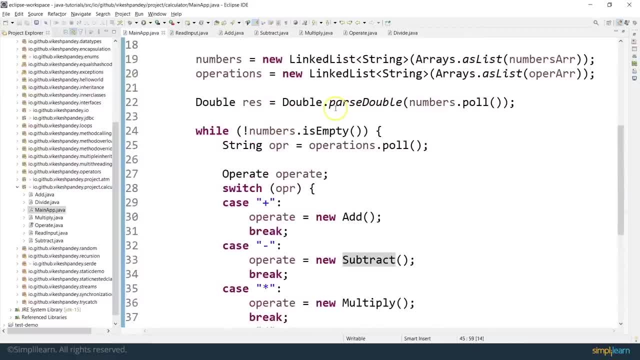 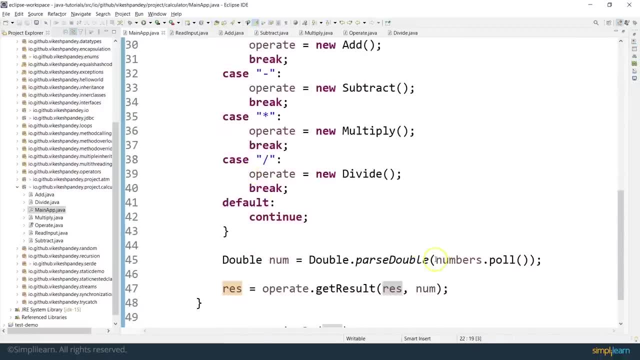 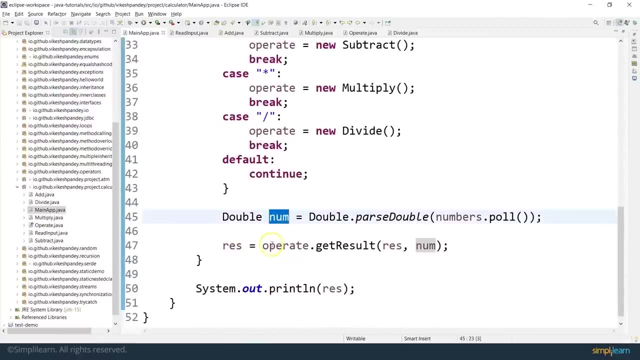 the next number from the queue. remember, we already did one pole here. so, as per this example, four was here in this res and now, when we do this number dot pole again, five will be picked up, because that will be the next head of the queue. so we pick up five here and then we call operate dot get. result now this: 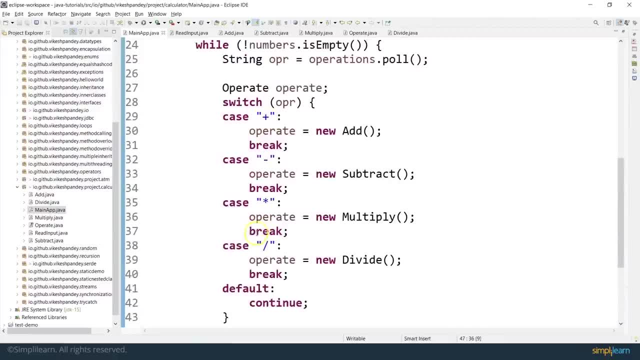 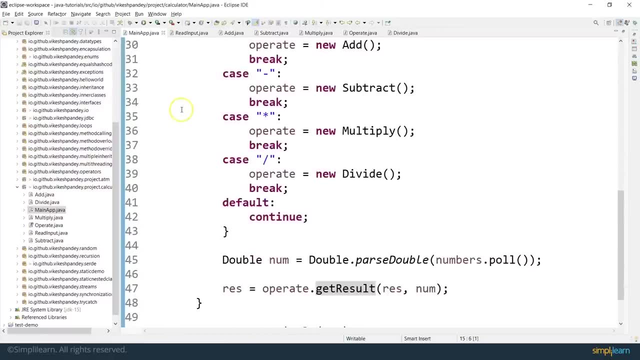 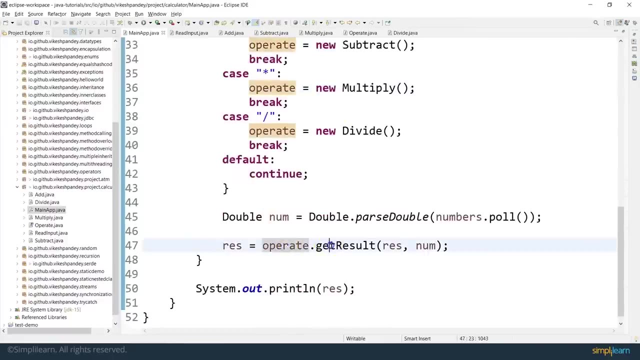 get result will be called based on the expression which was encountered first in the queue. again looking at the example, the first expression encountered will be plus, so the expression was plus. so the operate type object is of add type and when you call operate dot get result, the get result method of add class is going to get invoked and it is going to sum four and five. 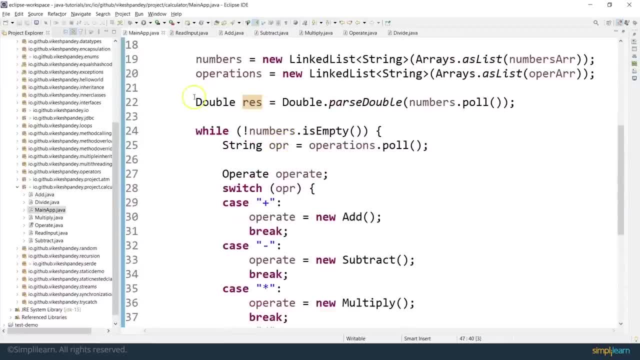 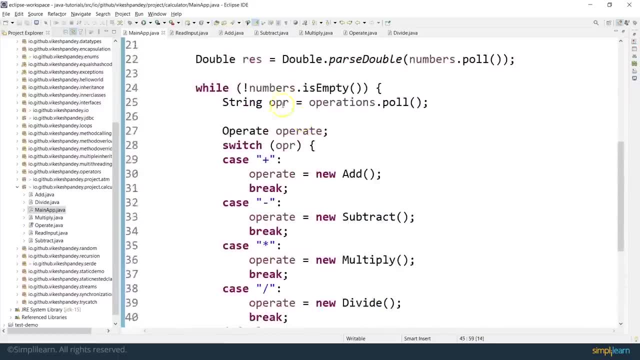 this res is holding four right now, based on what i described here, numbers, dot pole, and this num is holding the, the second operand, basically basically five here. so four plus five gets evaluated here in this case, and then it again goes to the next line after this expression was plus. so the operation. 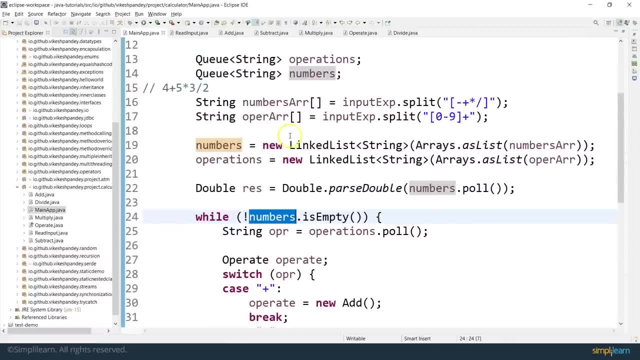 goes back here and it checks if the number queue is now empty. no, it is still not empty, because we still have three and two left there. so again it does the operations dot pole and it picks up multiply sign here. then it again runs the switch case. since it's a multiply sign, it will go here. 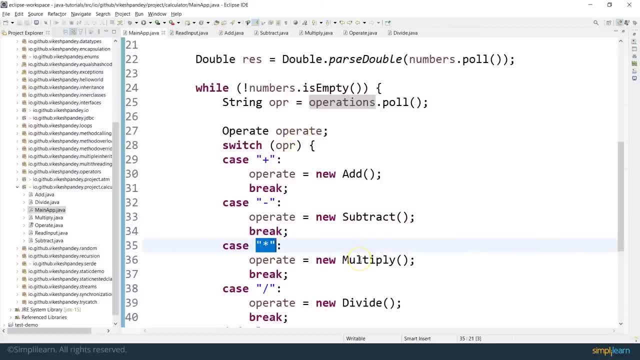 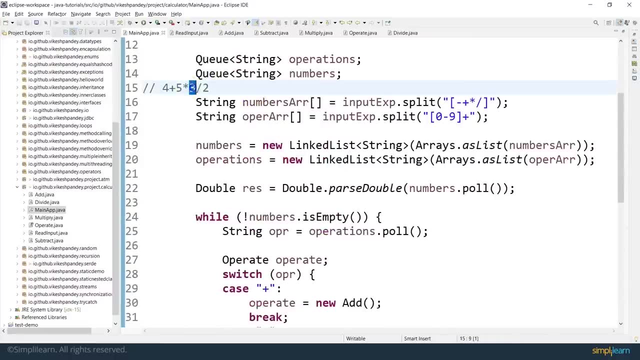 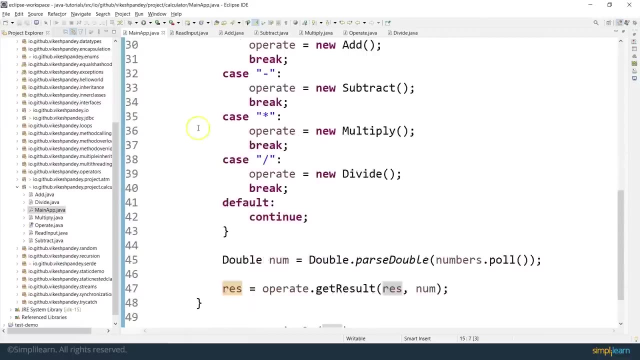 and it will initialize the operate interface reference as the object of multiply class. then, coming here, it will do a numbers dot pole and this time the numbers dot pole is going to pick up three. so three will be picked up here and then the current value of result, which is already nine. four plus five, was nine. the current 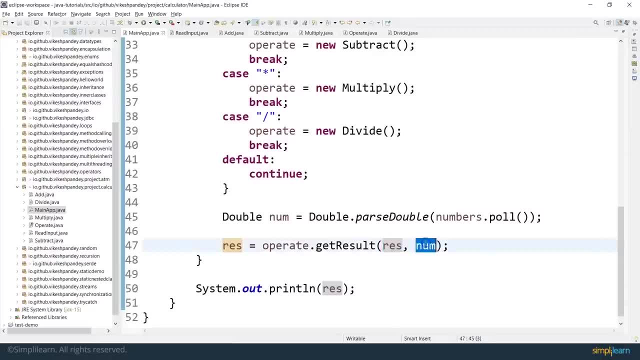 value of result will be updated here. so res will be nine here and num will be three here, and when you call operate dot get result, the multiply classes get result will get called and it will say nine into three, which will become 27. it will again go back here to this particular line and it 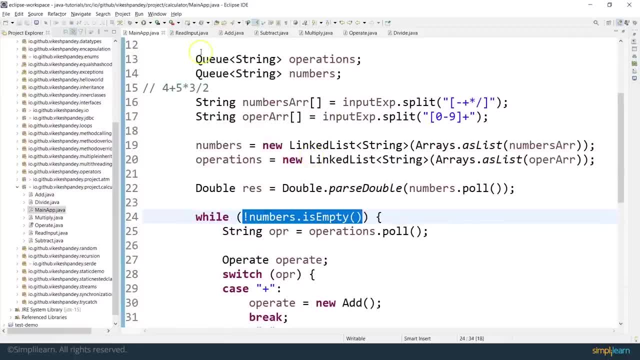 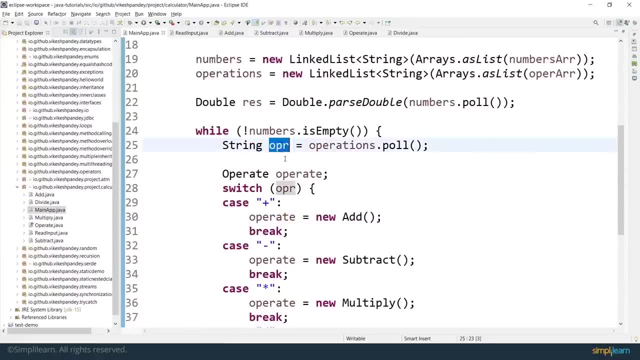 will check again if the numbers queue is now empty. no, it is still not empty, because we still have one element left. then it pulls the queue of the operations where the expression divide is present. there, which is the only element left in this particular operations queue, and since we have the opr value as divide, 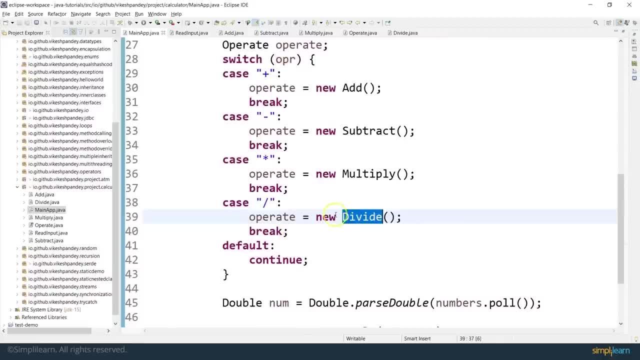 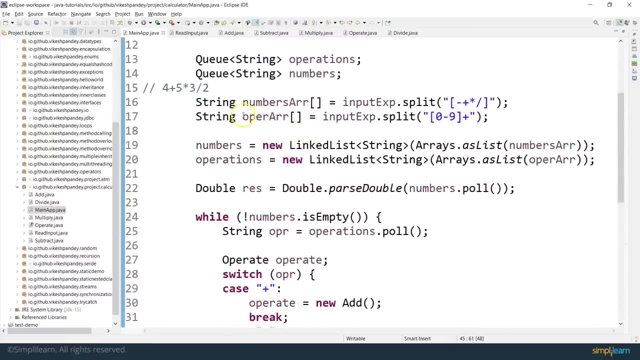 this case, block gets called and the new divide class gets initialized. the divide class basically gets initialized and we come here and we do numbers dot pole. now the last number which is available in this queue is two, which gets picked up here, and then we again call operate dot get. 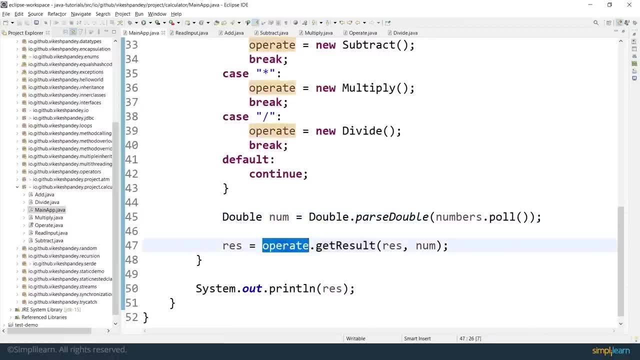 result. the operate object refer object: operate reference type was of divide class type. so when we call operate dot get result the divide operation or the get result method of the divide class, basically this method will get invoked and it will divide the current value of result, which was 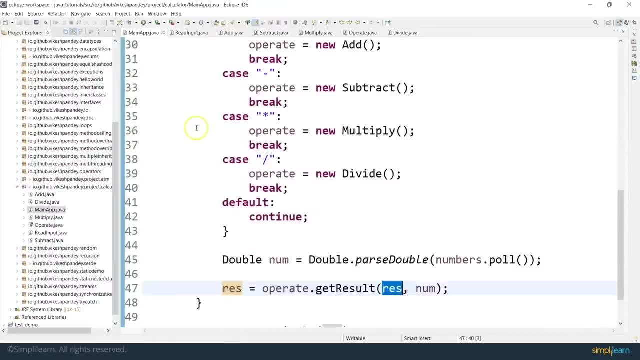 four plus five nine into three, which was 27. so it is going to divide 27 by two, which was the last value of the numbers dot pole. so it is, it is going to execute 27 by two and whatever value it gets, it is going to store the. 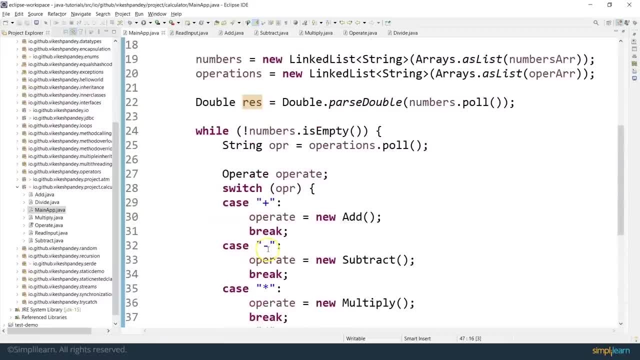 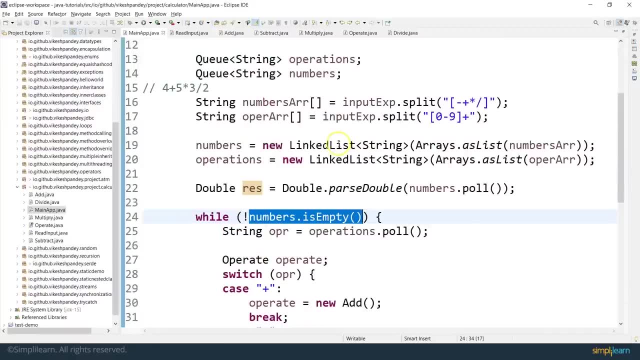 result value back into the rest variable and then it is again going to go back here and again going to check the condition if the numbers queue is not empty. but now the numbers queue is empty because two was the last element. so it is going to come out of the loop and it is going to print the final. 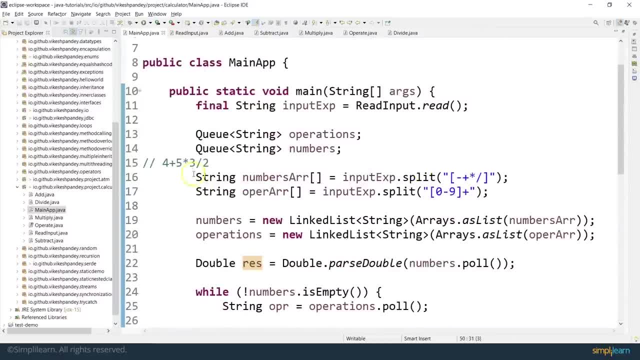 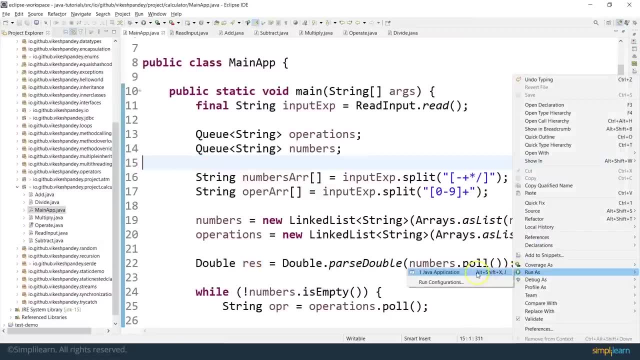 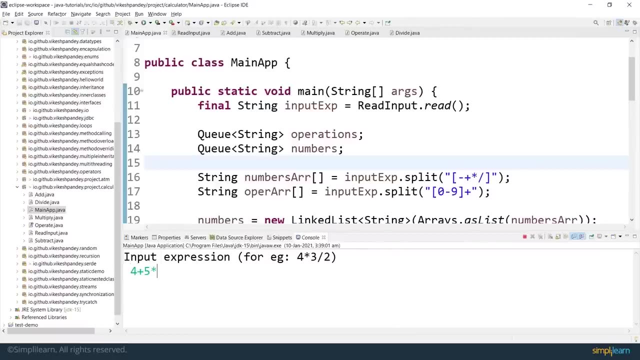 result. that is how this whole program is working. now let's try to see this in action and we'll try to execute the exact same expression. so if i right click and go to run as and run this as java application, and i supply an expression saying four plus five, star three divide two, and if i now hit enter, i get the value as 13.5, which 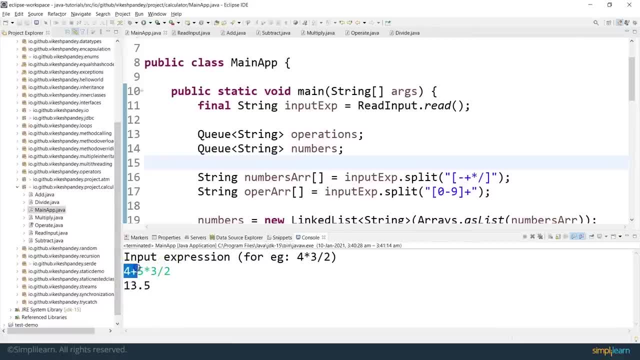 is exactly what we ran through, because four plus five will be evaluated first, which will result into nine, then nine into three, will be 27, and 27 divided by two will be 13.5- exactly so this is how this whole program is running, where we first take the inputs and then 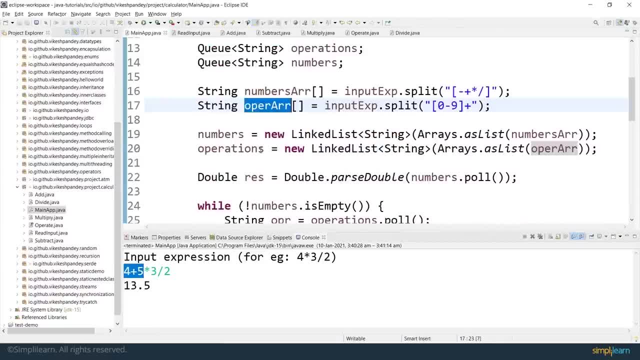 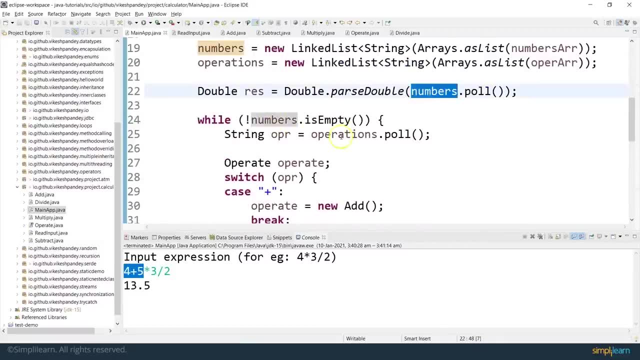 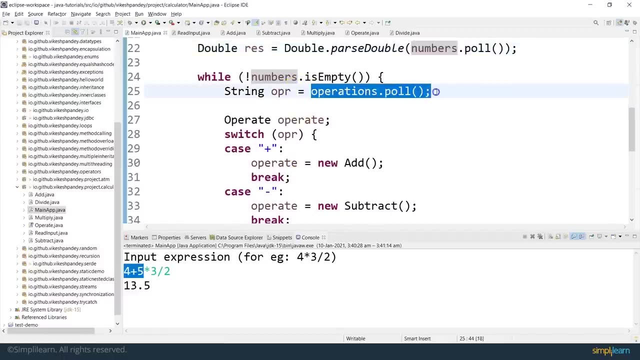 we divide the input into numbers and operation arrays or in fact queues, and once we have those queues built up, then we pick up the first number and we keep running this loop till the numbers queue is not empty inside the while loop. at each step we pick up the first expression or the operator. 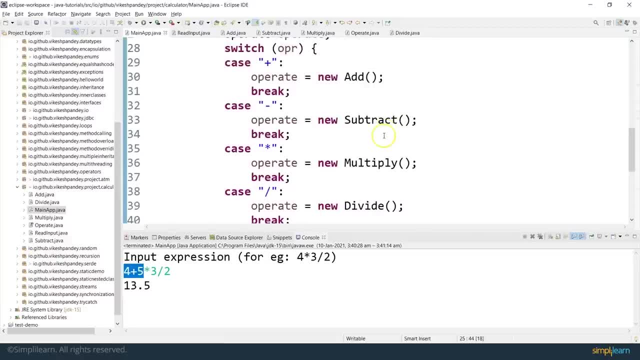 we check what is the operator, whether it is an addition, subtraction, multiplication or division of the operator. and whatever kind of operator we have, we initialize the corresponding class of it and then we fetch the next value in the numbers queue and then we call the get result based on the. 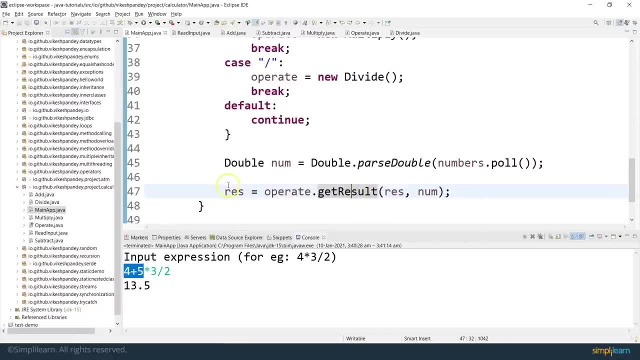 expression and whatever result we get from the get result, we store it back into the rest variable. so we keep updating the rest variable at every step. that's the reason the result of four plus five gets stored in the rest, and next time you are calling the get result for a multiply operation. 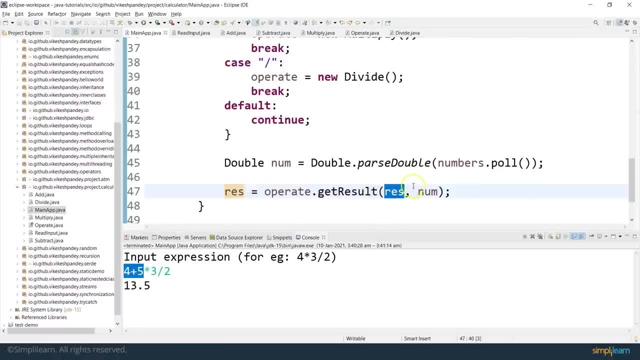 here is nine now and it says nine into three again. in the next time the rest value will be updated to 27, because we are storing the result back into the result variable. so this is all i want to cover in this particular session, where we looked at an example of a calculator application, purely from 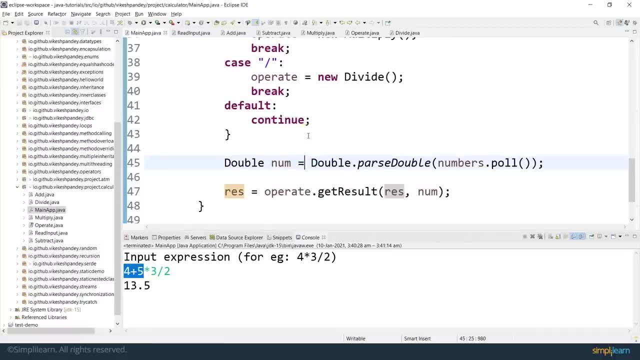 the console standpoint. obviously there can be a lot more stuff which we can do into this particular application: make it more error free and cover a lot of corner cases like validating the inputs etc. also looking at putting some conditions around the exception handling, handling the divide by zero. 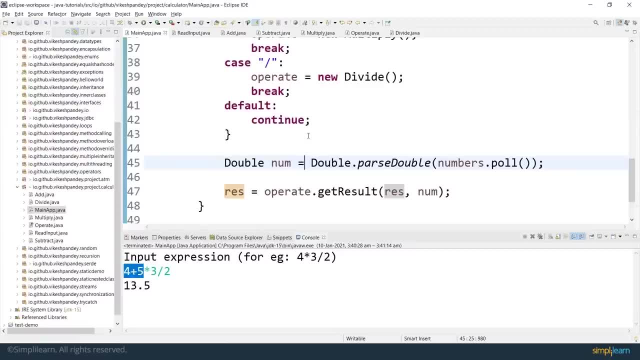 scenario etc. which is not here, but this is just to show you the basic idea of how you can build simple to complex cli applications using the core java concepts. so that's all i want to cover in this particular session. if you like this video, a thumbs up will be massively appreciated. thank you, and 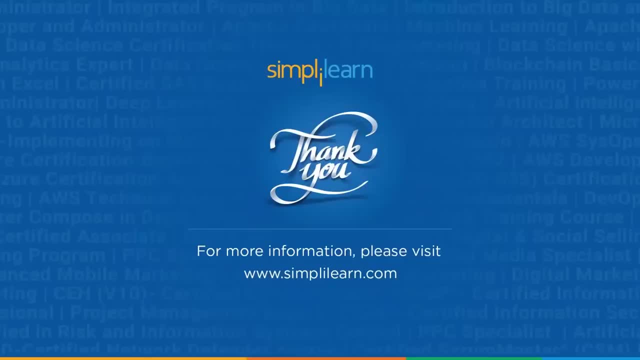 we'll meet again in the next session, and with that we have come to an end of this particular tutorial on object-oriented programming in java. if you have any queries regarding the topics covered in the session, then please feel free to ask them down in the comment section below our team of experts.